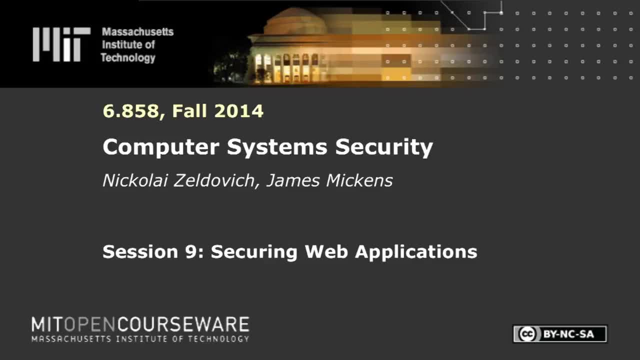 The following content is provided under a Creative Commons license. Your support will help MIT OpenCourseWare continue to offer high quality educational resources for free. To make a donation or to view additional materials from hundreds of MIT courses, visit MIT OpenCourseWare at ocwmitedu. 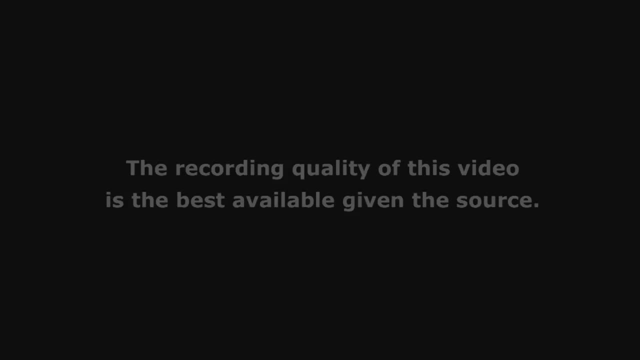 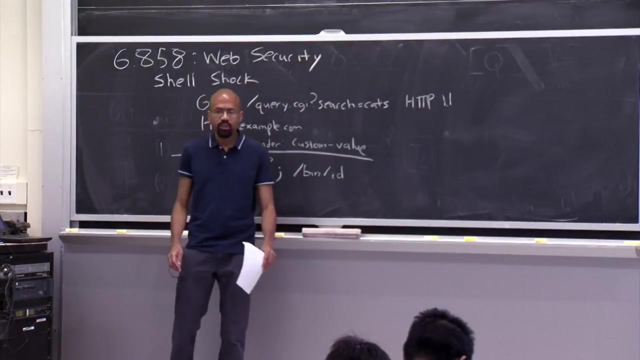 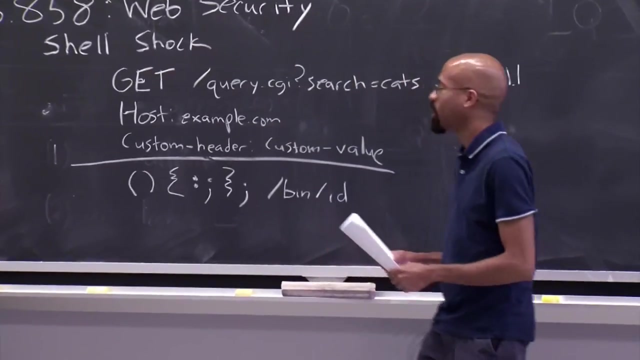 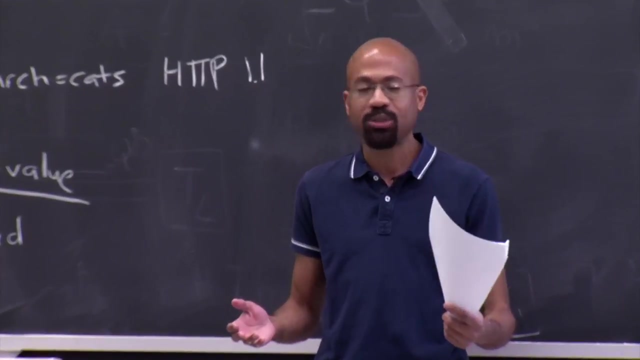 All right, So let's get started with the second lecture in our stunning series on web security. So to start off the class today, I actually want to go over some quick demos. So, as you know, demos almost never work, So hopefully you won't just be seeing my empty terminal up. 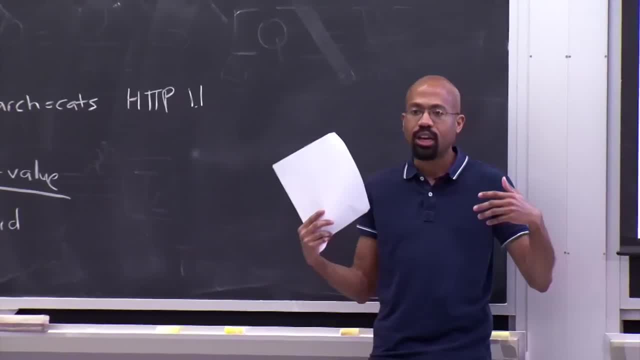 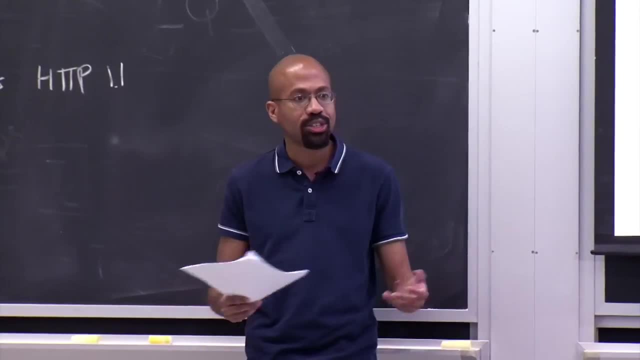 here, But the basic idea is That I first wanted to show you an example of the shell shock bug that you may have heard of. This has been pretty popular topic in the security literature And people were saying that Heartbleed was like a 10 out of 10 security bug. 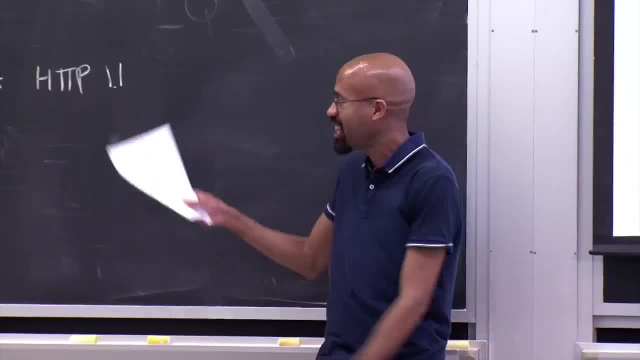 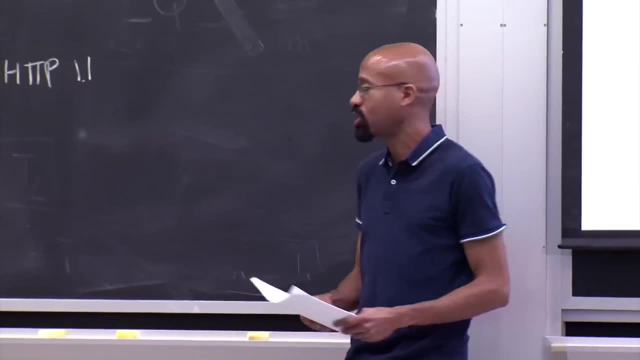 People were saying we should not have reserved 10 out of 10 for Heartbleed. This is potentially worse, And so I thought that this would be a great idea for you guys to see some living history and for you to tell your parents that they're getting their tuitions. 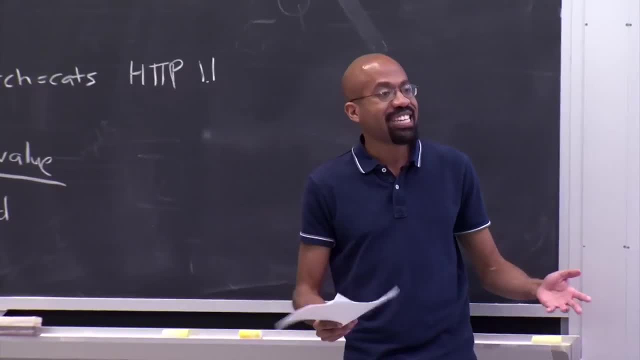 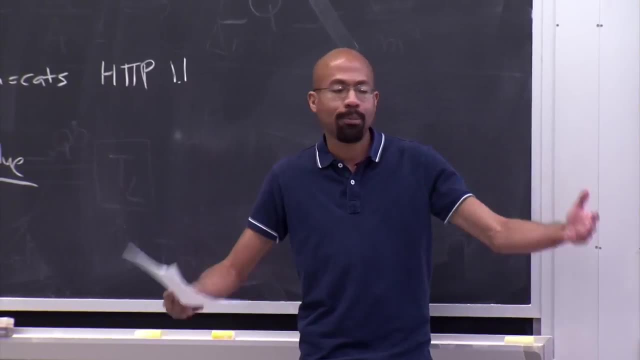 worth out of MIT. So what is the basic idea behind the shell shock bug? Well, it's a really great example of why it's so difficult to build secure web applications that span multiple technology stacks, multiple languages, multiple OS's, so on and so forth. 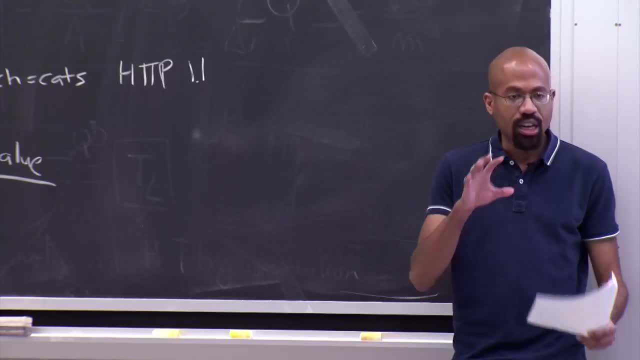 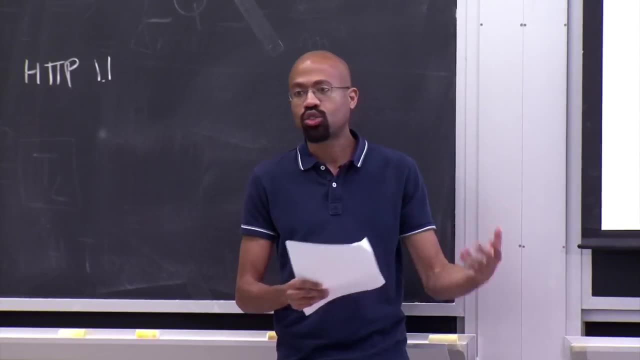 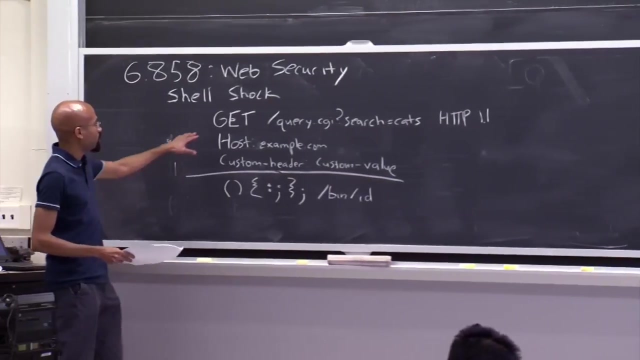 So the basic idea is that shell shock is going to take advantage of the fact that the attacker can craft a special HTTP request to a server and control the headers that are in that request, And so I've written an example up here. It's very simple. 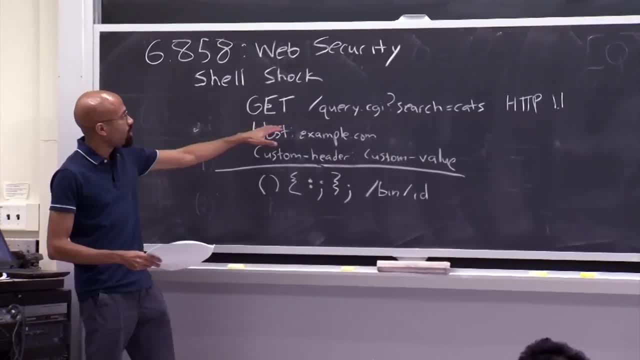 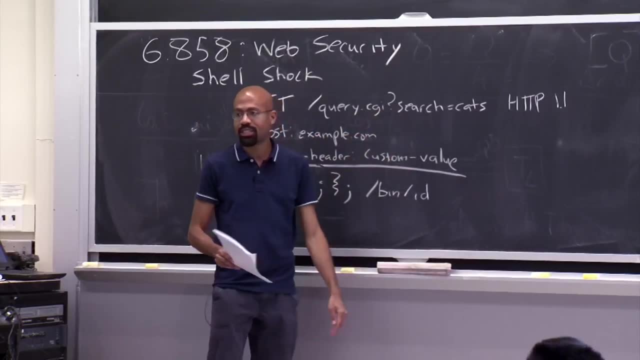 So let's say that the attacker wants to send some get query. They're going to send that query to some CGI interface And then there's going to be some question mark. The person wants to search for cats because that's all the people search for. 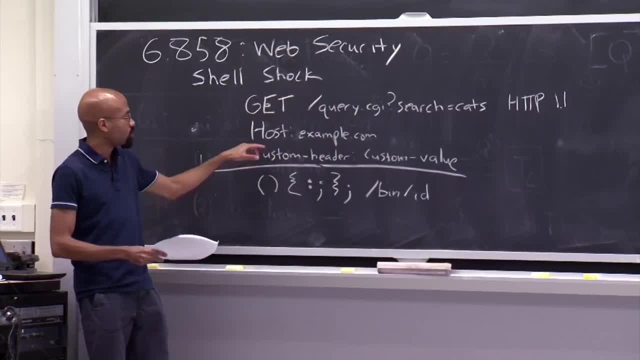 And then there's some standard headers here, like host for example. So this is saying that this URL here is hanging off of examplecom. Now note that the attacker can also specify custom headers. So the attacker can just say: I wanted to find some application specific header called. 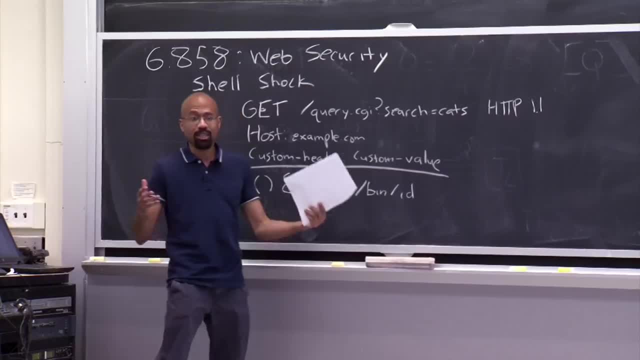 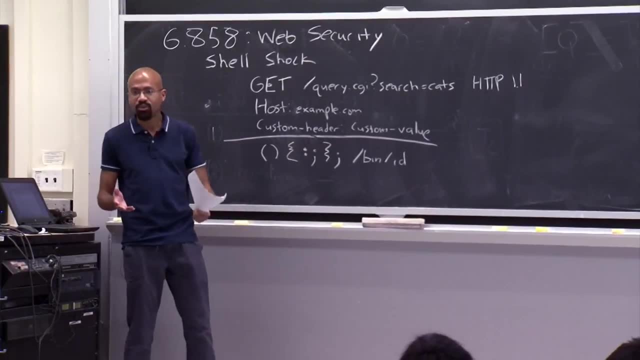 custom header And I want to specify some value there, Because you can imagine that a web application might define certain functionalities that can't be expressed using the simple predefined HTTP headers, So that all seems fairly innocuous. But what ends up happening is that in a lot of these CGI web, 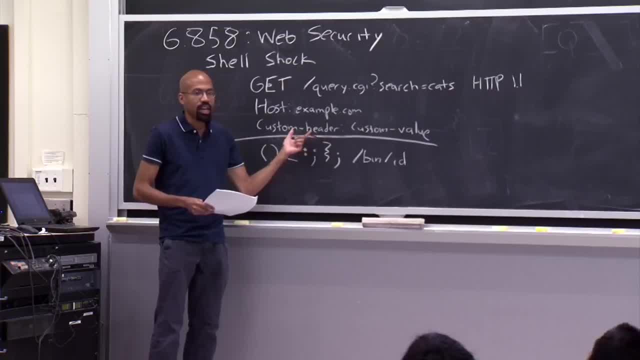 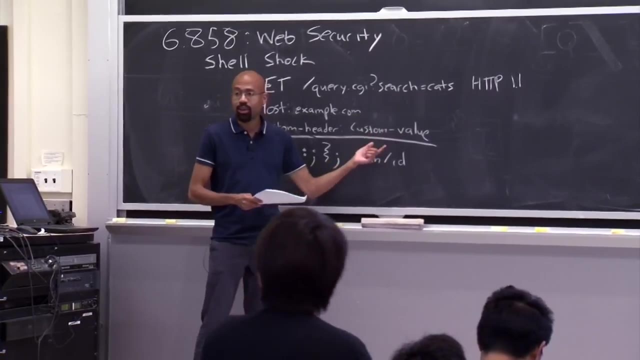 servers. they will actually take these custom header values and use them to set environment variables for bash. So they will use this header to create a bash variable named custom header. Then they will take this value here that the attacker has applied and use that to be the value of that bash variable. 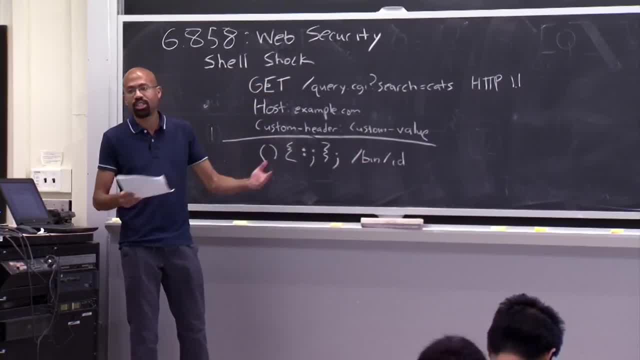 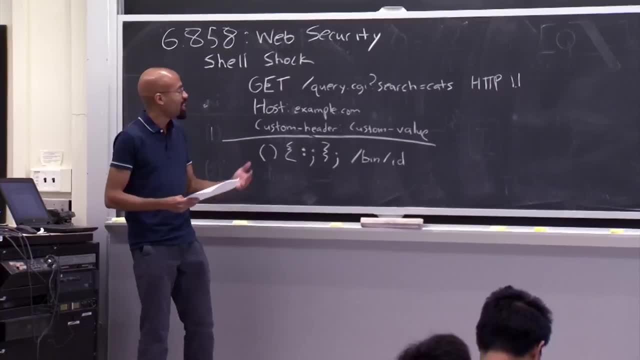 And then, once that variable is set up, then the CGI server will do some processing in the context of that environment. So this is clearly bad. You can probably see where this is going. Web servers should not be taking these arbitrary values from arbitrary, unwashed masses. 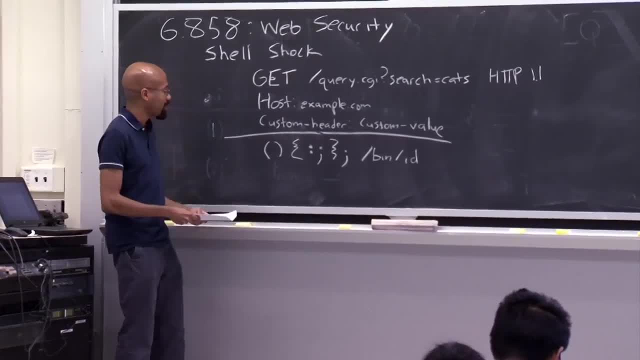 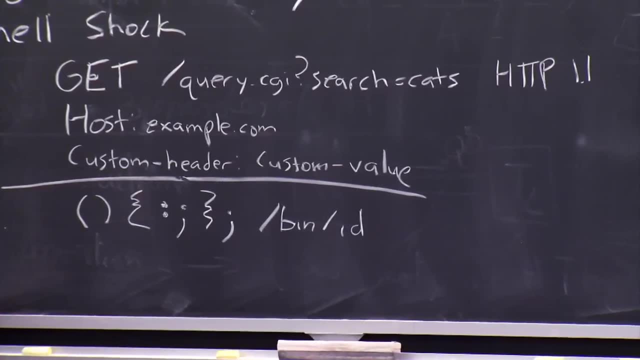 So in the particular example of the shell shock bug, what ended up happening is that if you set your bash variable to this, this kind of malformed, evil looking thing, then there's going to be insanity. that happens. Basically, this is a malformed function definition. 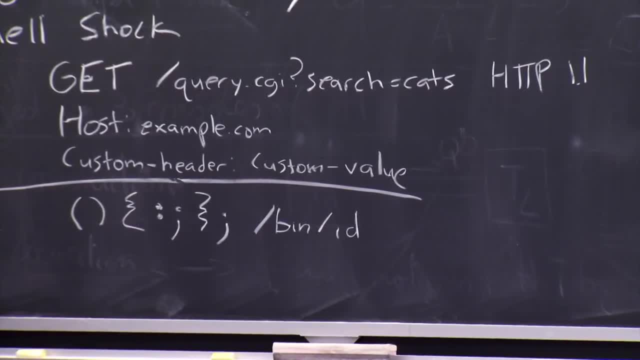 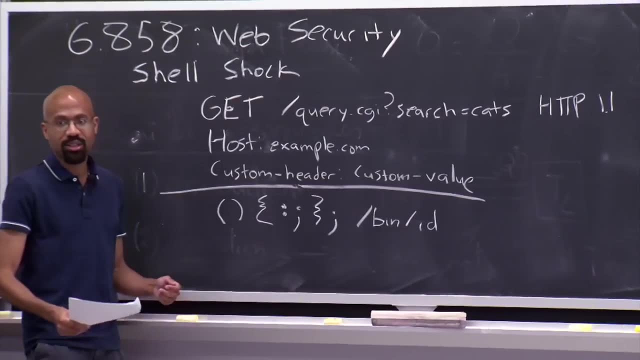 in the bash scripting language, You don't have to worry about the specifics of it. But what was intended to happen if bash were correct is that this part over here wouldn't be executed. So basically, you just define some stupid function here. 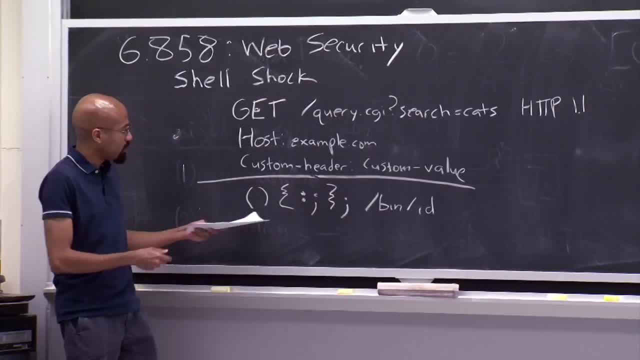 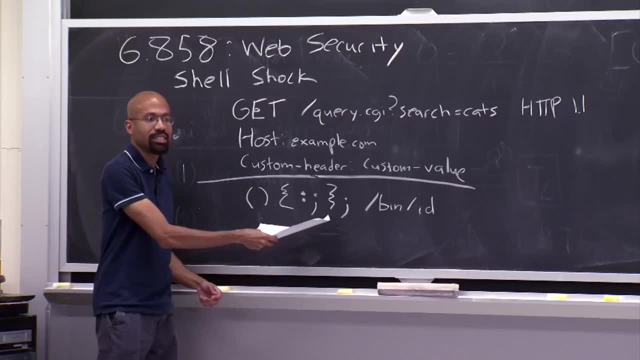 that doesn't do anything, And then the parsing would terminate here. But this sequence of characters actually confuses the Barsch parser, And so what ends up happening is that it sort of stumbles through this nonsense here And then it says, oh, I might as well keep on parsing. 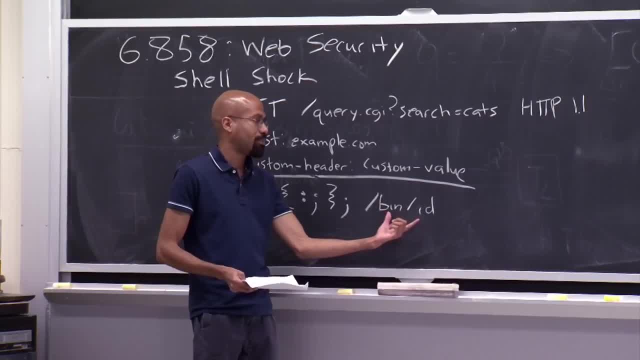 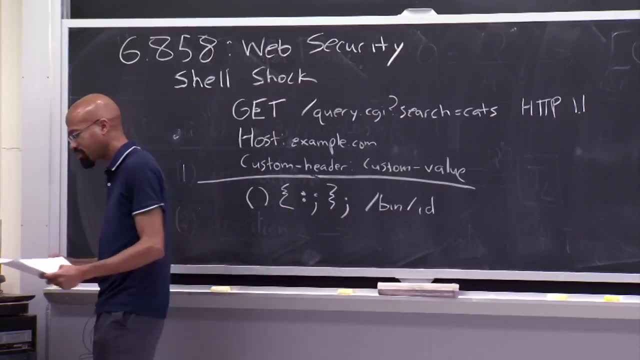 and execute some commands here, And so in this case this just does the bin slash ID command, which displays some information about the user. But this could be any code right here. So that's the part of the vulnerability. So I'll give you a very simple example here. 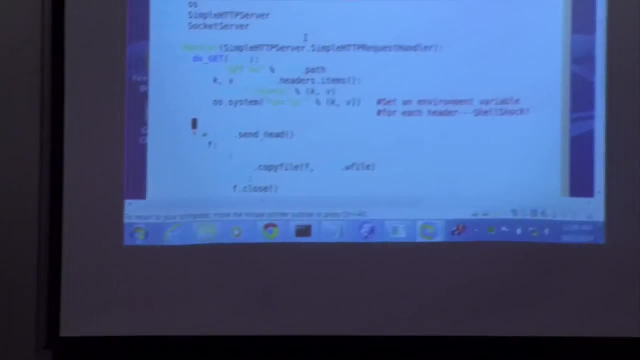 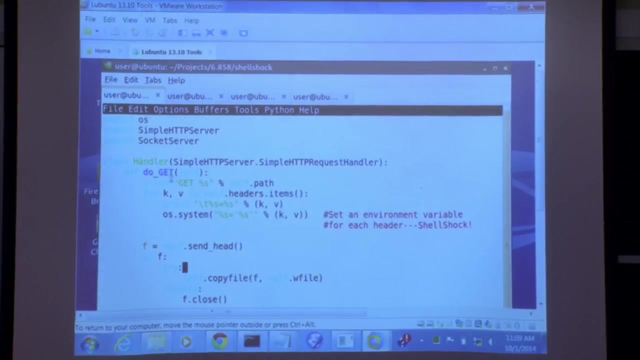 So you see up on the screen. So basically, you've got a very simple Python server here, Just the dumbest one you could possibly imagine. It's got this do get method And so with the do get method, is it's going to basically iterate through all of these? 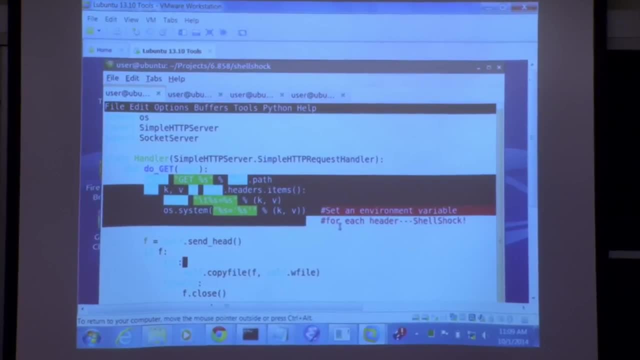 OK, All of the HTTP headers in the request. OK, So that's what this for- key value for the header and the value in this request, And then it'll just print out the headers that it finds And then, in this dirt simple example, 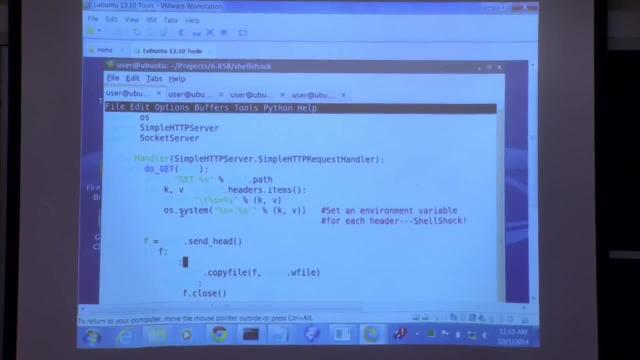 it's going to do something very dumb, which is execute the system call and just directly set the environment value to the value specified in the header. So that's the whole root of the vulnerability. So if I come over here and I start my victim web server, 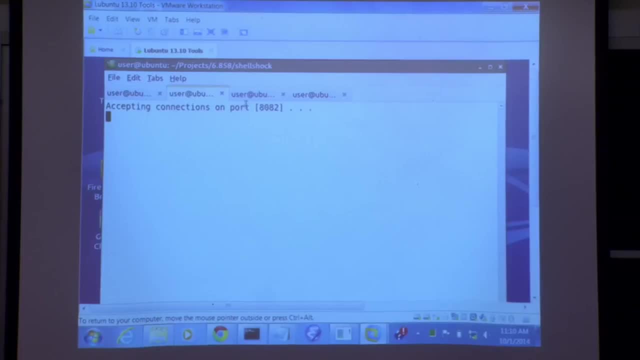 OK, So it's now ready to accept requests, And then I can write my special shell shock client, like so, And this is actually pretty dirt simple. So here I just define one of these malformed strings, So I have these kind of janky characters at the beginning. 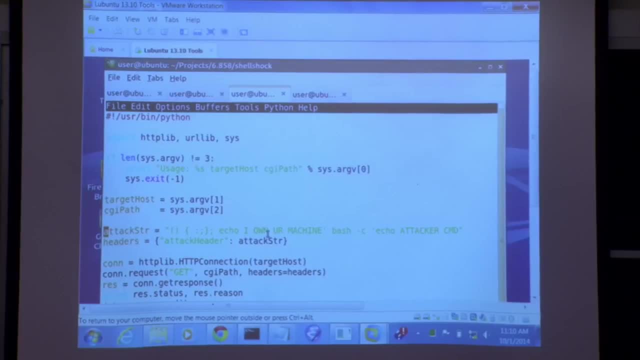 And then I know that everything after this is essentially going to be executed on my behalf on the server side. So in this case I picked something that was actually pretty innocuous. It just says: Echo, I own your machine, But this could be anything here. 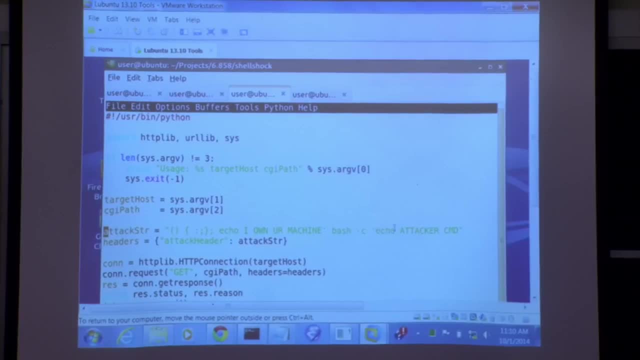 You could start another bash shell, you know, kind of like I do here, and then echo, you know attacker command, Where in the real world that could actually be something very dangerous. So then I set the headers and my custom request. 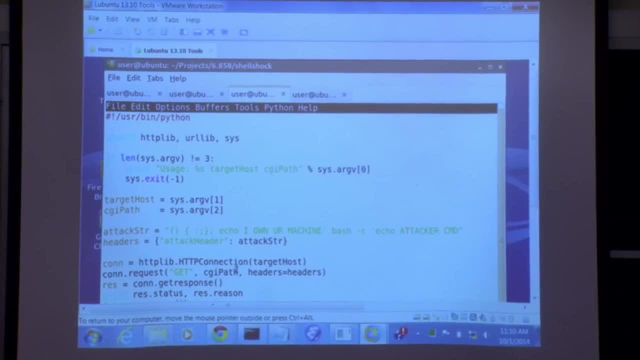 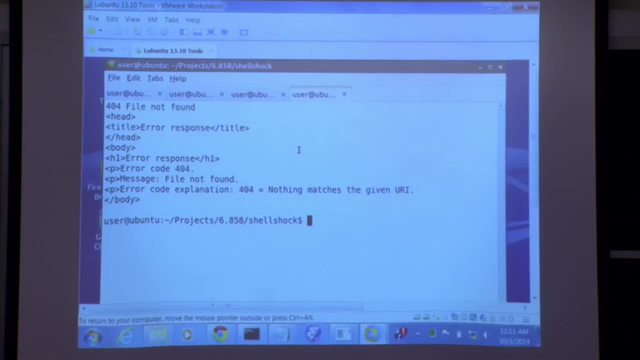 And then I just use Python to create an HTTP connection and just send it to the server. So what ends up happening? So I execute my shell shock client here. So it's saying that I had a 404 here, because it doesn't matter what file I requested, right? 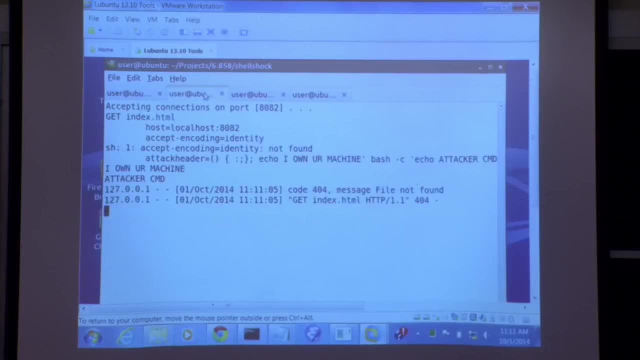 So I just put in some indexhtml that doesn't exist. But If we look over here, this is the output for the server right, And so what you see is that you have this output. I own your machine and attacker command right. 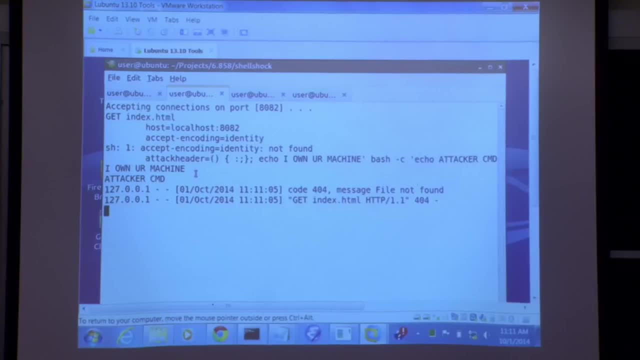 And that's because, as the server got that header, it set the bash variable, It set it with this weird thing here And, as a result, an attacker control command got the run. So does that all make sense? So does this happen like if the program is run under that? 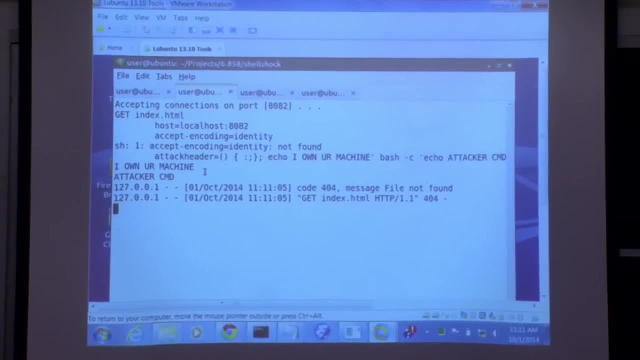 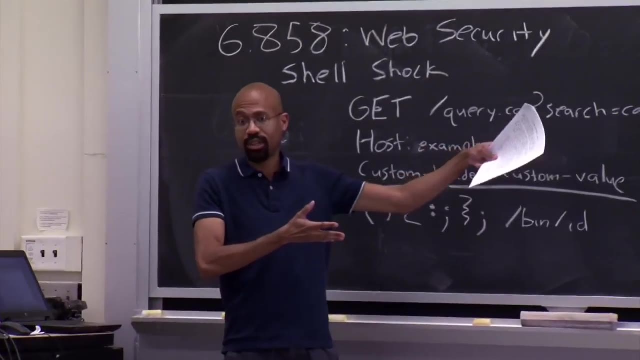 Do you have to invoke? I'm still unclear on like. Yeah, So the specifics of how the attack works actually depends on like. are you running Apache, Like what exactly your web server looks like? So, like in this example, it's a little bit contrived. 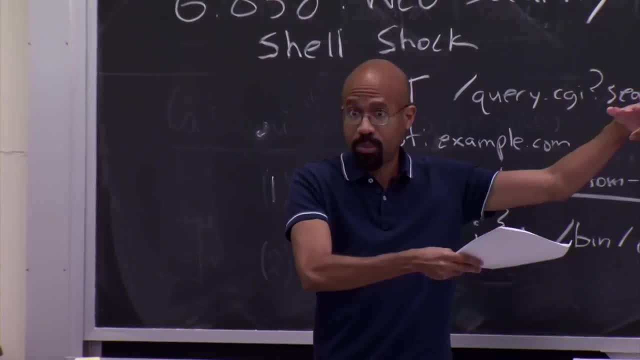 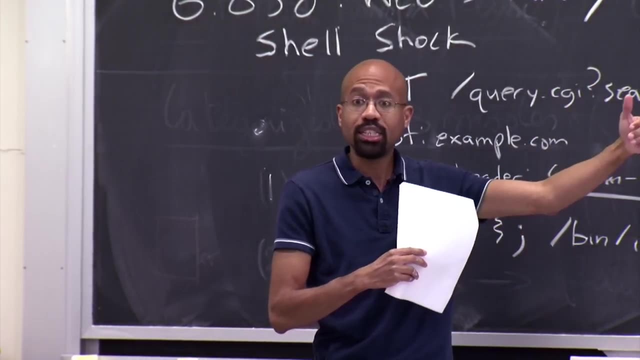 because I actually called ossystem, explicitly spawned off another bash shell, set the environment variable in there and then we were ready to go. But you can imagine that if you were spawning off a different process for each incoming connection, you could set the environment variable for that directly. 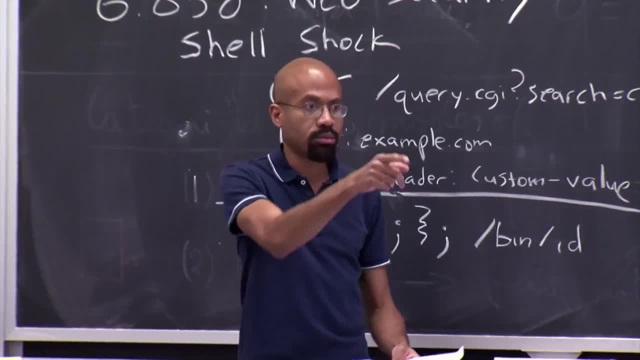 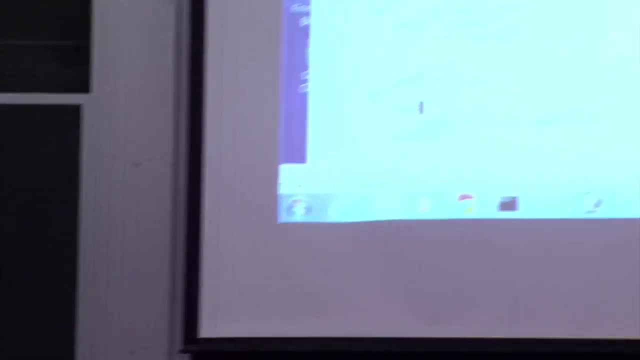 if that guy was living inside of a bash environment. So if you go back to your web server code, it means that you have a much worse vulnerability than the shell shock, because you're calling ossystem and I can execute a command just by setting the custom header. 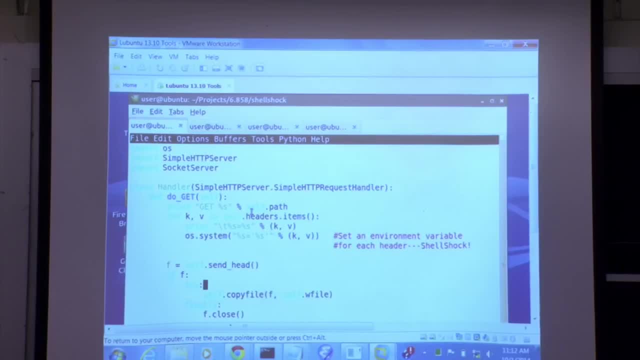 to something malicious, I don't have to use the shell shock. That's correct. That's correct. yeah, So in this particular web server, which is something I wrote just for sort of teaching value, yeah, this thing you shouldn't trust for anything. 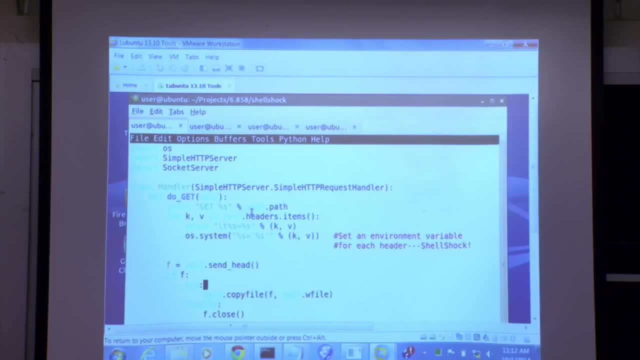 But the shell shock exploit was on assigning something malicious to an environment variable using setend or something like that. Oh yeah, yeah, So that gets back to his question. That's right. So if you had, let's say, Apache up here, 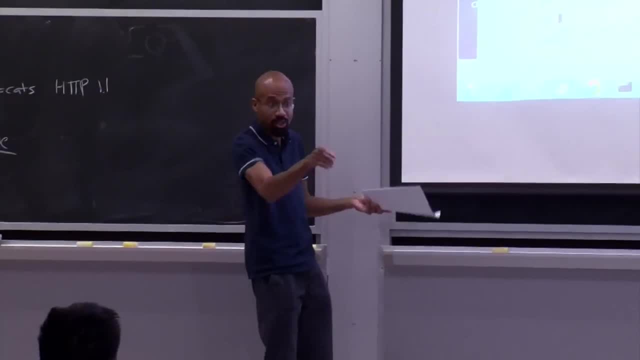 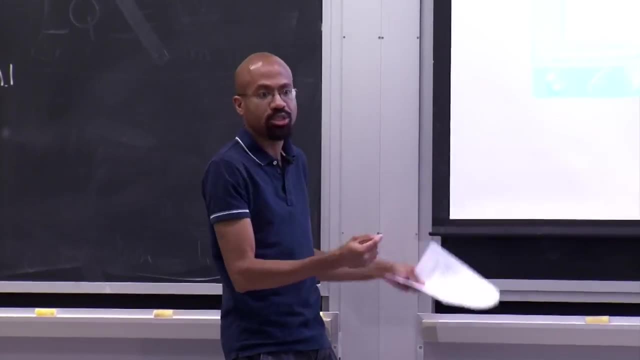 Apache is a little bit tricky to configure in a way. that's obviously what's going on, But you're exactly right. So Apache we call setend, which is another way that you can directly set the environment value for whatever particular server side process you have. But you also actually have some servers like this that you can imagine that they actually do a spawn of a separate process and do something very morally equivalent to this. But you're exactly right that the way that Apache, in particular, was violated was the way that you described. 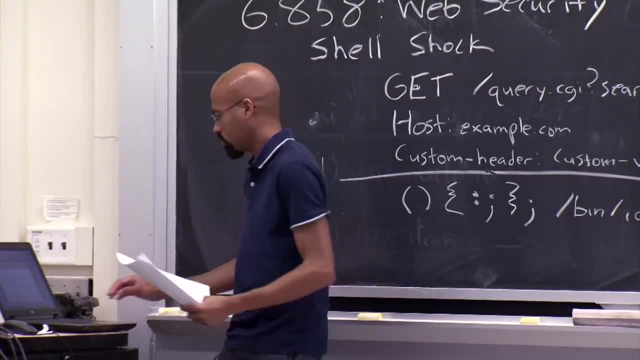 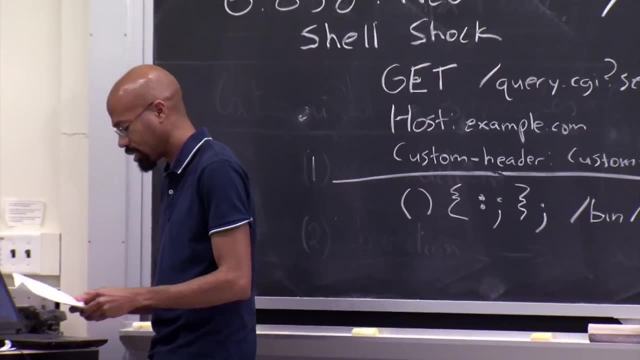 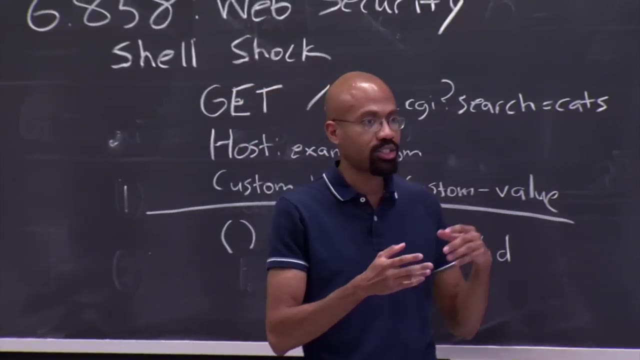 So does it all make sense? OK, So that's sort of a quick and dirty example of shell shock stuff, And so another example I wanted to give you was an example of cross-site scripting, And so the shell shock bug was sort of an example of how content sanitization is very important. 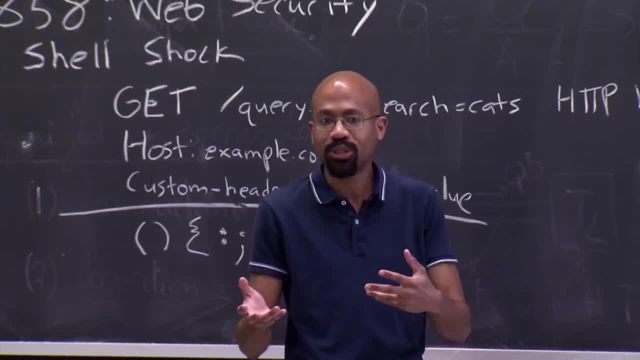 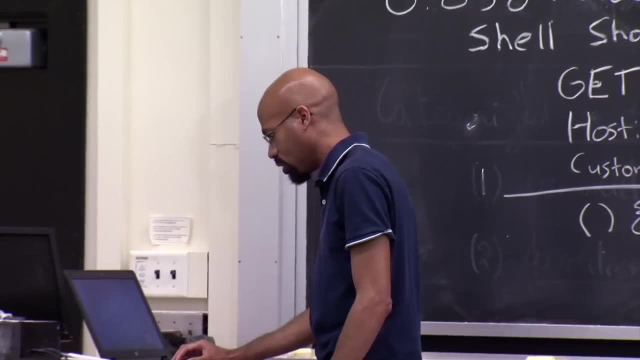 So, as we've just been discussing, you shouldn't just take inputs from an arbitrary person and then use them directly in commands of any type, And so cross-site scripting attacks are another example of how something can go wrong. So in this example I have another sort of dumb CGI server. 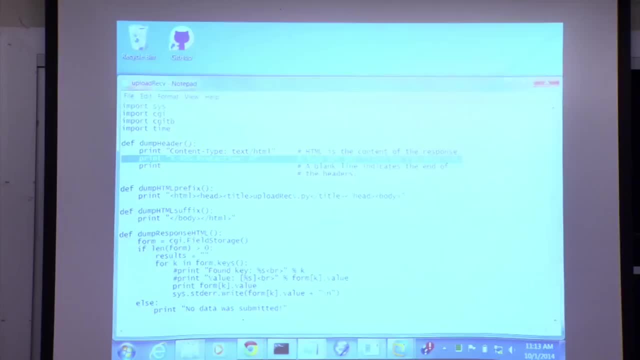 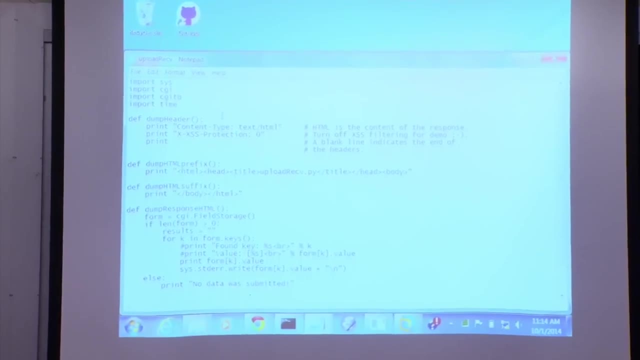 here, And if we look at this CGI server, so what is it going to do? So, once again, I've written something very simple in Python. This is going to be the handler that executes when a request comes in from the client, And so essentially what happens is that up here. 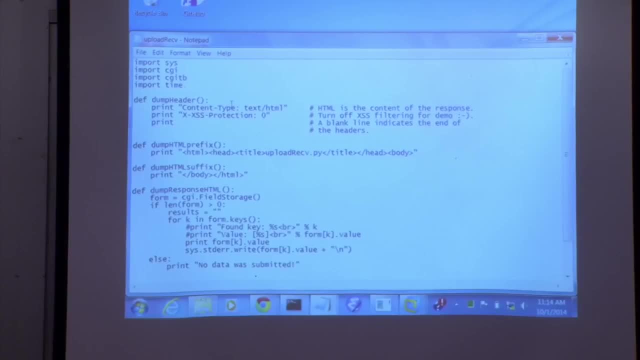 I'm going to print some headers for the response. Right, I'm going to say my response is going to be of type text, HTML. This line here will actually explain in a second. So, as it turns out, browsers have some security mechanisms to try to prevent the attack that I'm about to show you. 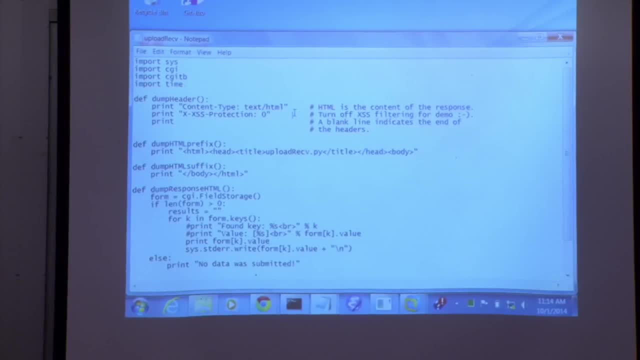 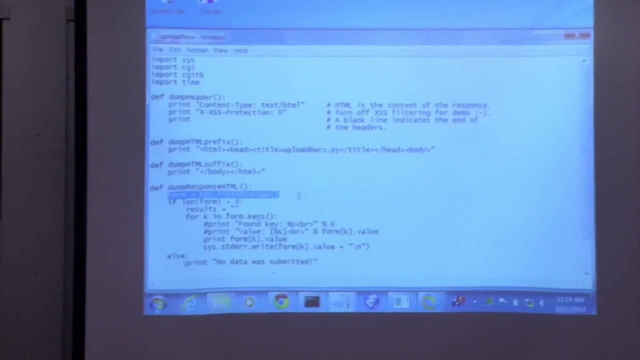 So I put that header line in there to turn some of those protections off. And then what the CGI script does is it gets access to all of the fields in the CGI request. So imagine that everything in a query string after this question mark like these header and value things. 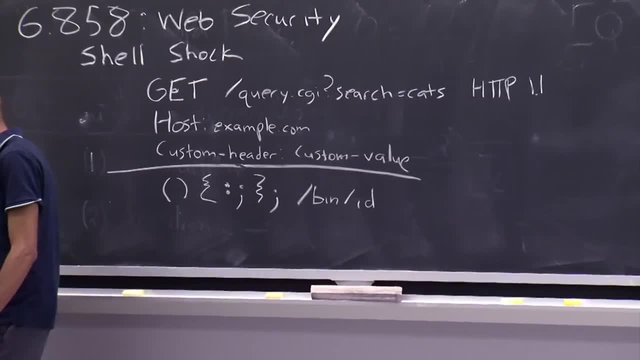 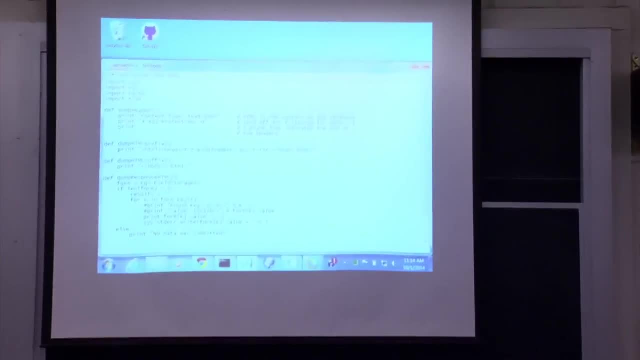 that's what I'm going to do. This is going to be the first query in the query string, And then what the CGI script does is something very simple: It just directly prints the value of something that was passed from the attacker. So same basic idea. 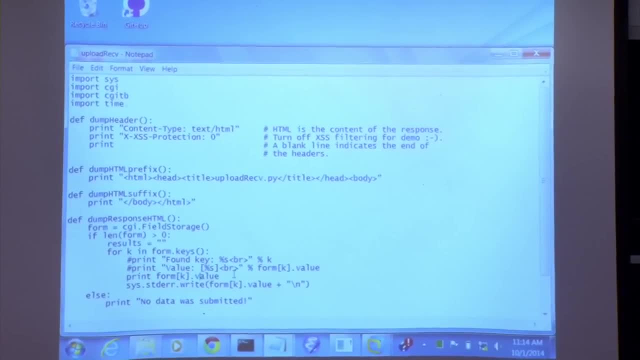 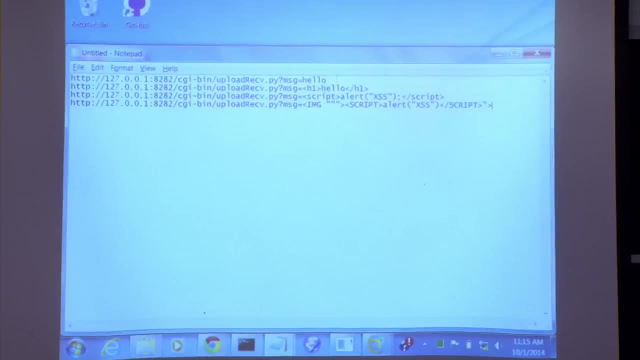 This is a bad idea because this print statement here it's printing directly into the HTML itself. So what can happen is as follows. So let's say that I have a bunch of queries I want to run, So in this first query here I'm just setting: 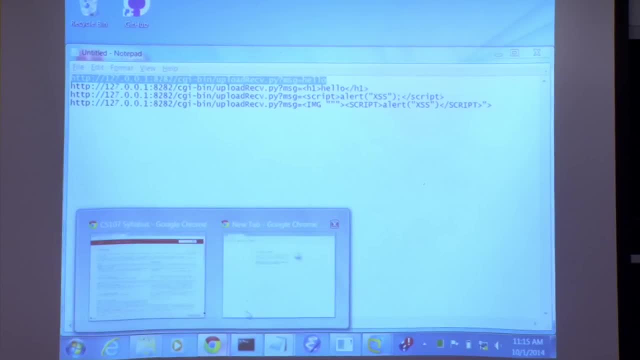 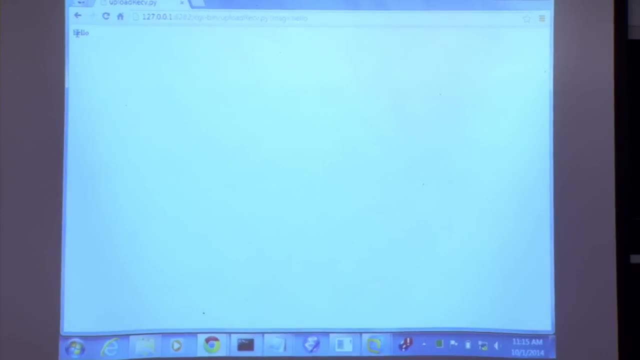 the message value to hello. So if I go over here and I run that page, well then you'll see that this hello shows up Because once again the server was taking directly what I passed to it and it prints hello. So no big surprises there. 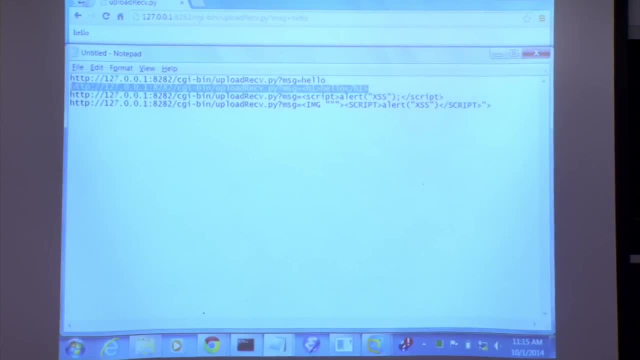 Now let's say, I realize that I can actually pass arbitrary HTML in there. So now I actually try to embed some styling in there. So I say to h1, and then hello, then slash h1.. So that worked Because once again we're printing directly into the page. 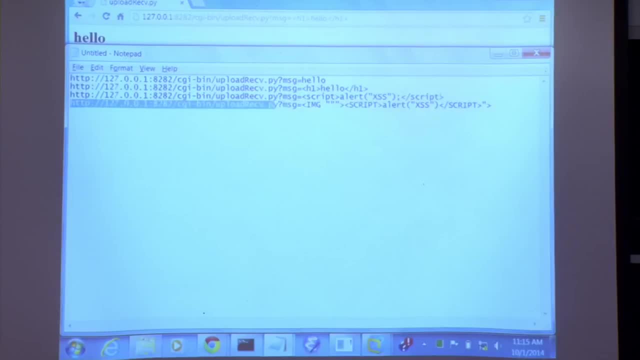 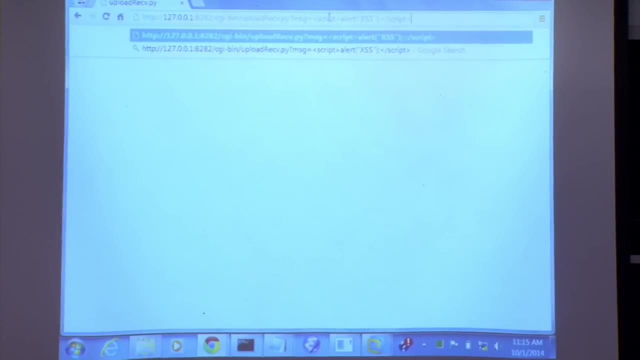 So now you might be thinking: OK, we're in business, now This is cool, So let's just directly embed some JavaScript code in there. And so I do this, And here I've actually just put in for the message I put: script. 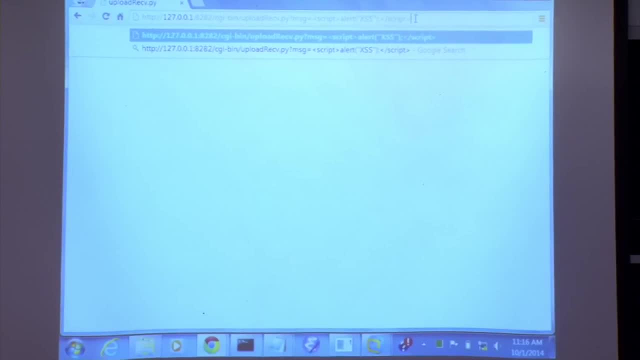 Then I want to just alert xss and then script. So now that's interesting. So it seems like something didn't quite work. So I don't see any output. I didn't see the alert either, And if I actually look at the output for the web server, 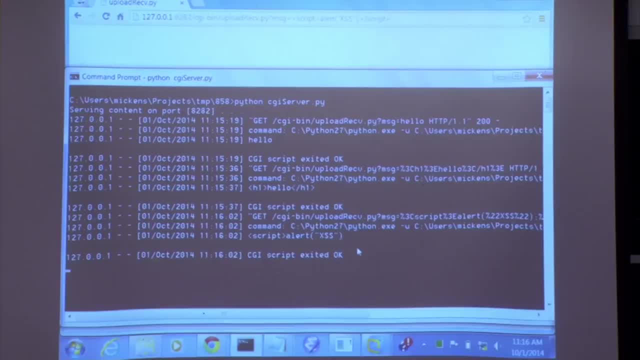 then what I see is that here the web server itself didn't actually get that trailing script tag, So it seems like the browser itself has somehow detected something evil, even though I tried to disable the xsx filter. So that's interesting. We're going to come to this defense mechanism. 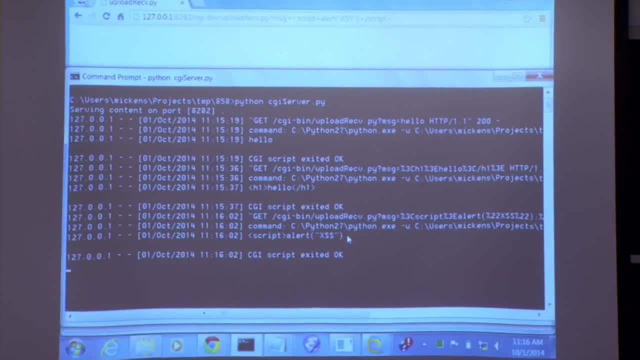 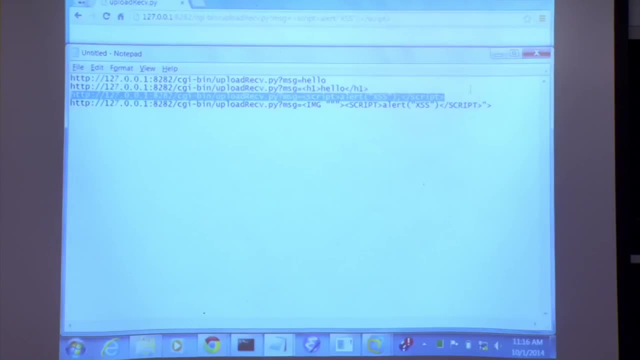 a bit in the lecture, But suffice it to say it seems like the browser is trying to resist this cross-site scripting attack, But of course, what we can take advantage of is the fact that HTML, CSS and JavaScript are extremely complex languages. 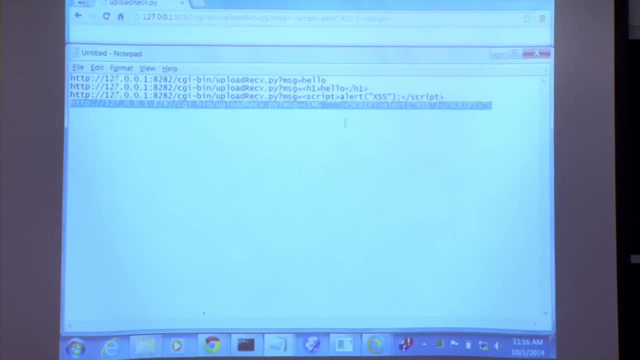 And they compose in these very difficult to understand ways. So here this is what I'm setting my attack string to. here This is malformed URL. I'm saying image and then three quotation marks in a row and then a script tag. 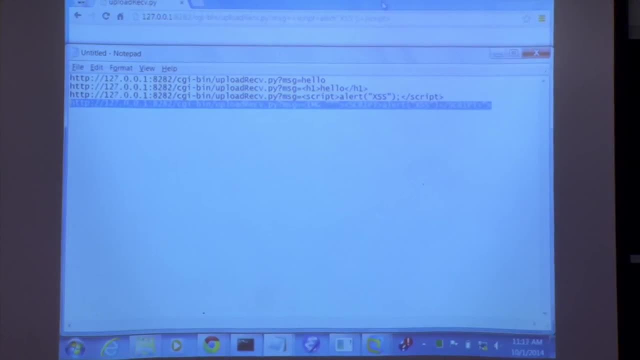 This shouldn't actually parse, But what's going to end up happening is that the browser is going to get confused here, So it's built-in cross-site scripting detection actually fails here, And so what ends up happening is that now you see the alert. 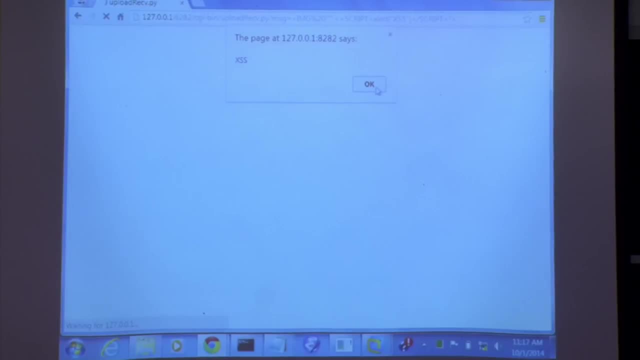 And what's interesting is that if you actually look at the contents of the page now, it's kind of messed up. Where did this quotation mark and brace come in? If we do a Control-U, we can see that this does not make the browser happy in some way. 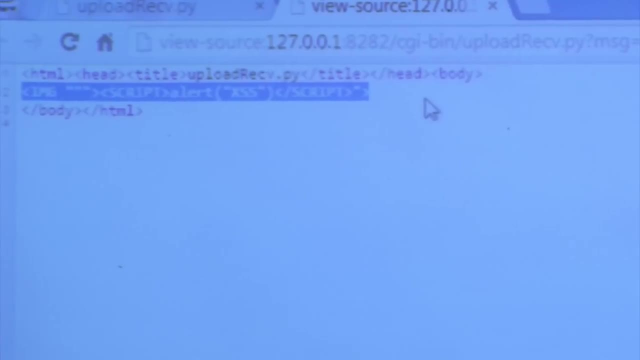 That's a little bit unclear, But it doesn't matter. if we're the attacker- We saw that alert- That means that our code got the run. And from the perspective of the attacker, who cares if the page is messed up now Because I could have used that code to steal the cookie? 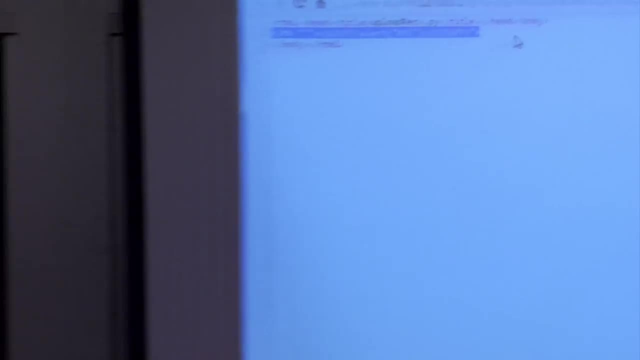 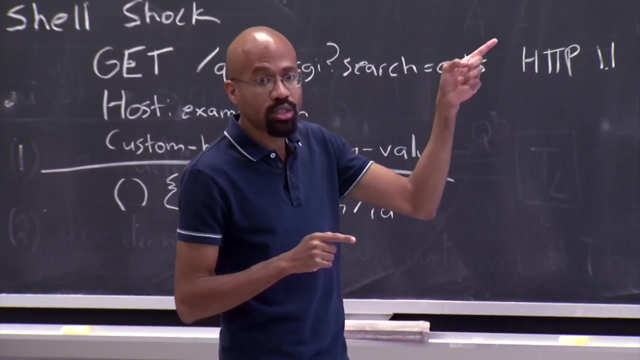 or things like that. So does that all make sense? Yeah, What's the cross-site aspect of this? So the cross-site aspect is that if the attacker can convince the user to go to a URL like this, then the attacker is the one who's specifying. 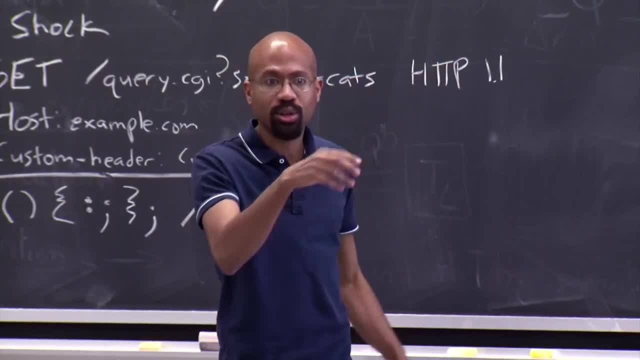 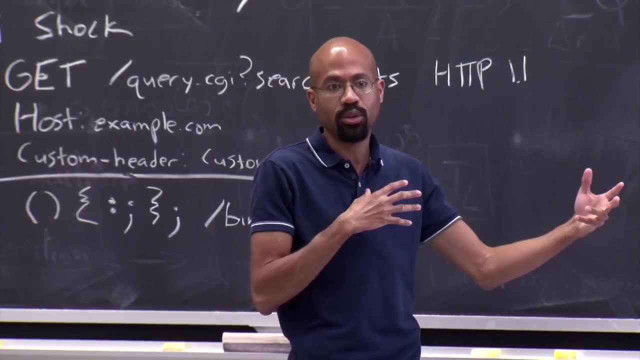 that stuff in the message. It's the attacker who's specifying the alert- XSS or something like that- And so essentially what's happening is that the victim page is executing code on behalf of someone that is not that page. Can you explain exactly what the browser role? 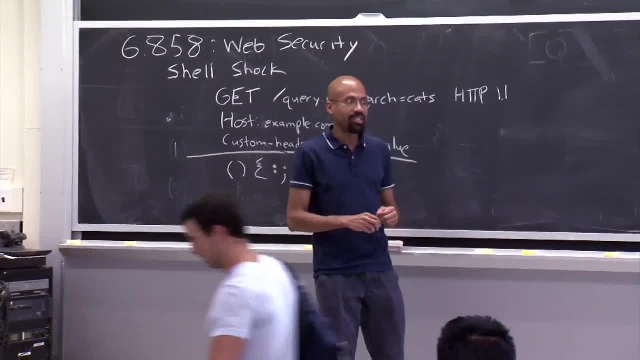 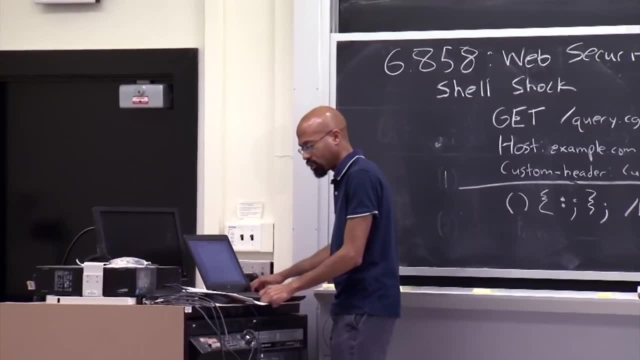 is for sanitizing the game's script page. Yeah, yeah, So we'll get to that in a second. Yeah, So we'll get to that in a second. OK, So that is all for story time And let's see here. 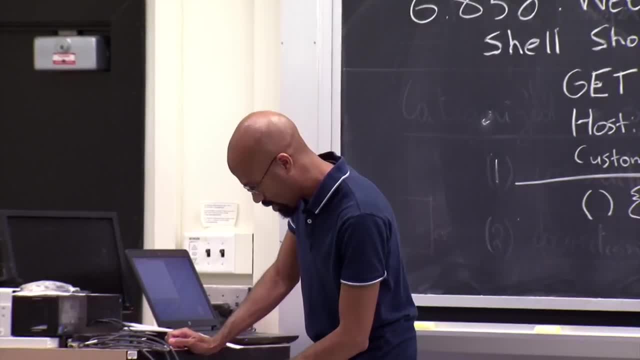 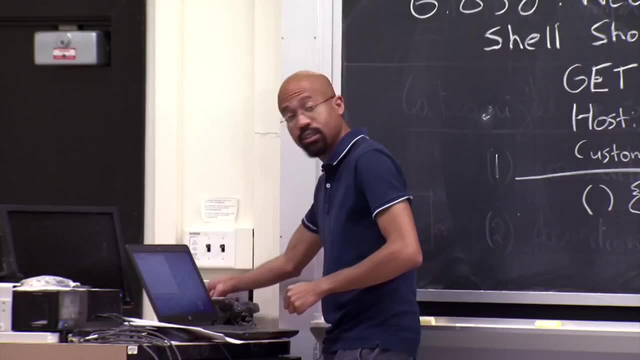 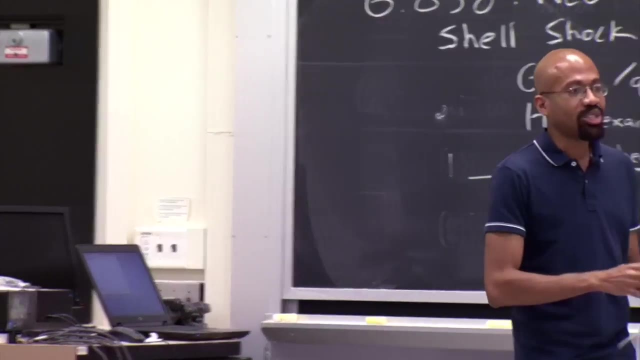 So I guess I can turn this guy off And then maybe he will. this guy here, this guy here. I'm trying to go off. OK, There you go. All right, Time's a charm. OK, Thanks OK. 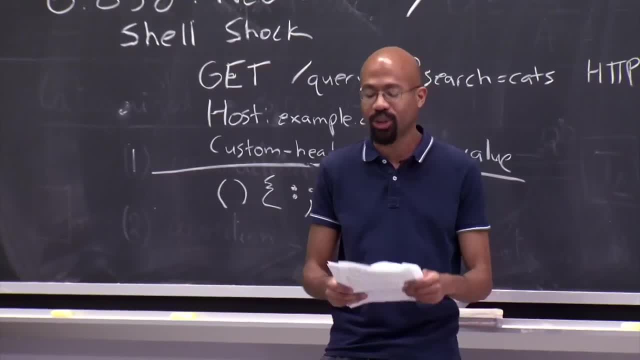 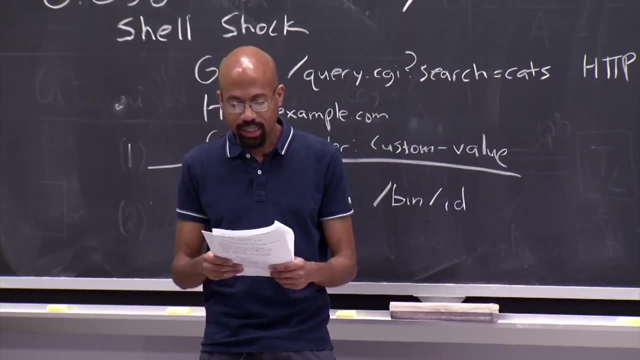 So yeah, So those are just two quick demos to show you the sort of filthy and dirty world that we live in right now. So why is cross-site scripting so prevalent? Why are these problems such a big deal? Well, the reason is that websites. 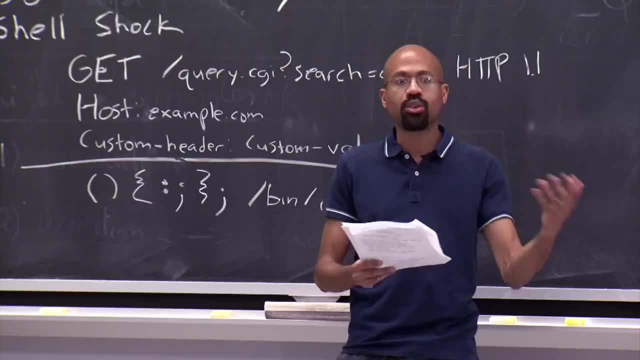 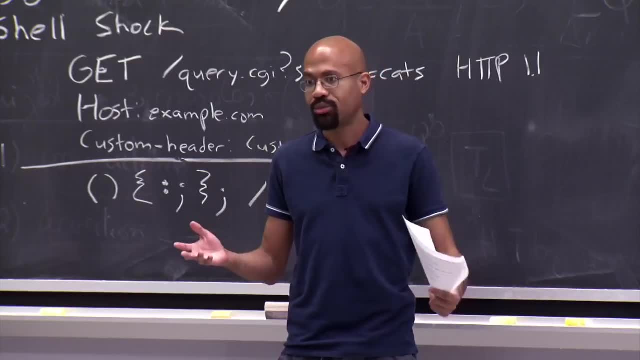 are increasingly more and more dynamic And they want to incorporate user content a lot of times, Or they want to incorporate content from other domains. So think about the comment section on a news article. Those comments come from untrusted folks from the user. 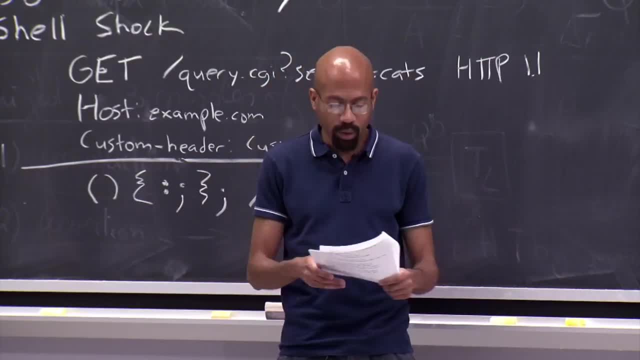 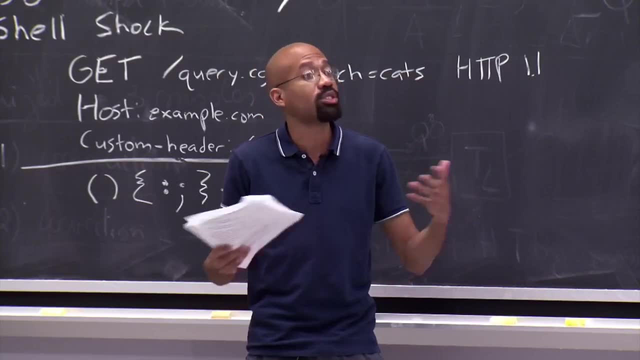 So somehow these sites have to figure out what are the rules for composing those types of things And also know that websites might host user-submitted documents. So think like Google Docs or Office 365,, for example, Those documents all come from untrusted folks. 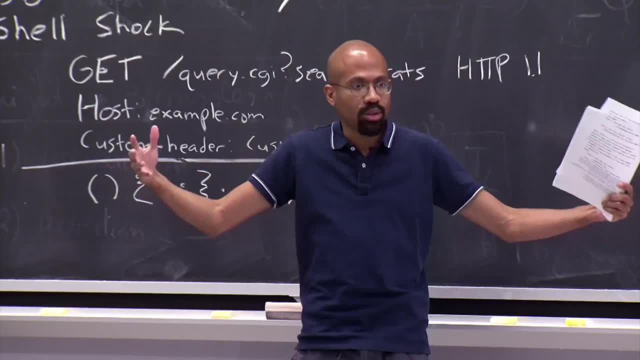 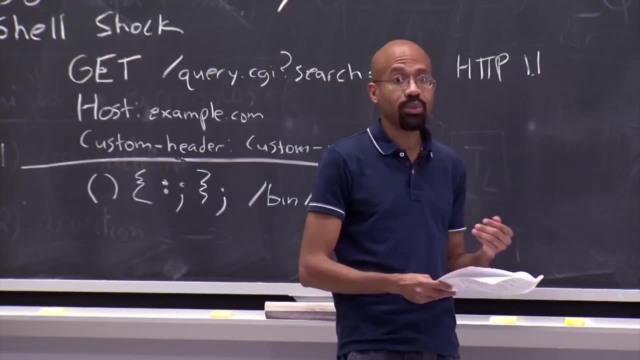 But somehow they have to live with each other and with the larger infrastructure from Google or from Microsoft or whatnot. So what are some of the cross-site scripting defenses we can use? This kind of gets to your question, So we'll actually look at some of those now. 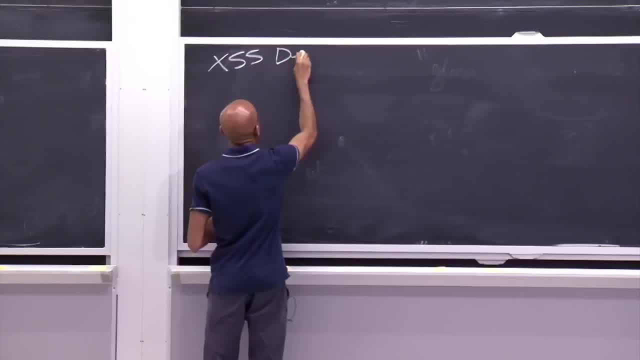 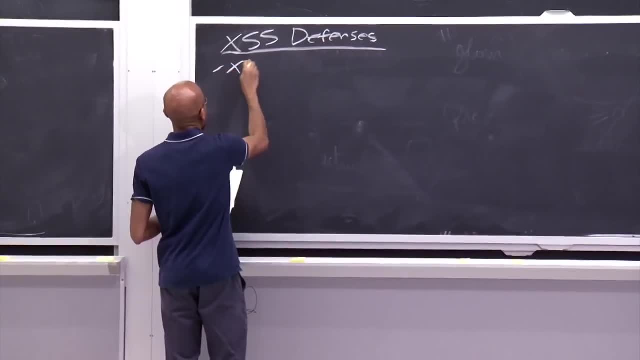 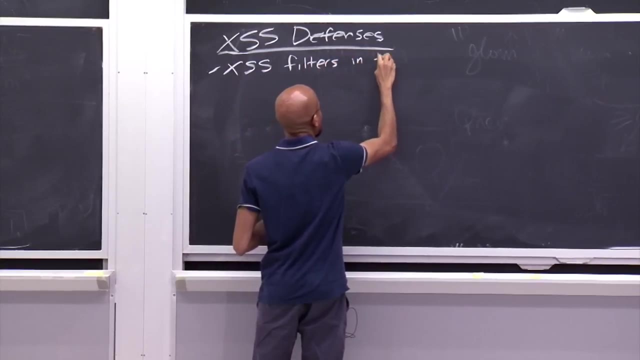 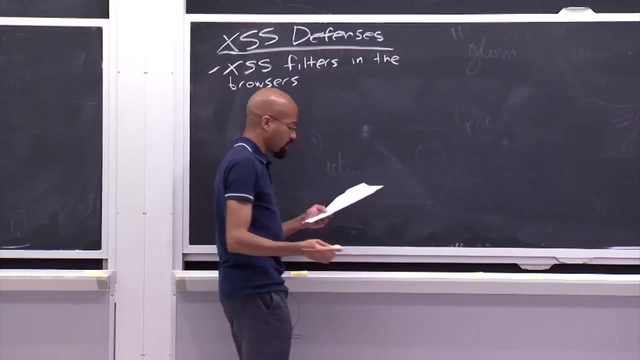 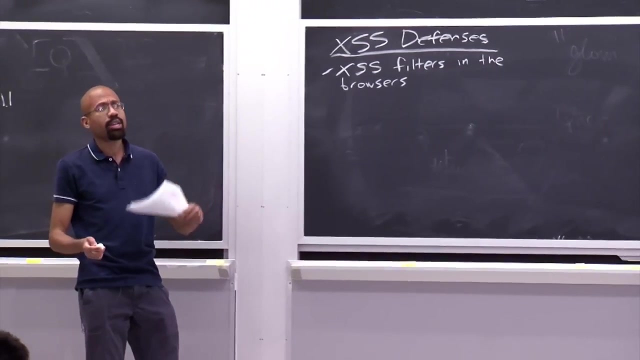 So one type of defense is to basically have cross-site scripting filters in the browser itself, And so these filters will essentially try to detect when there's a potential cross-site scripting attack. And so we actually saw one of those filters in action, And I think that was the third example that we looked at. 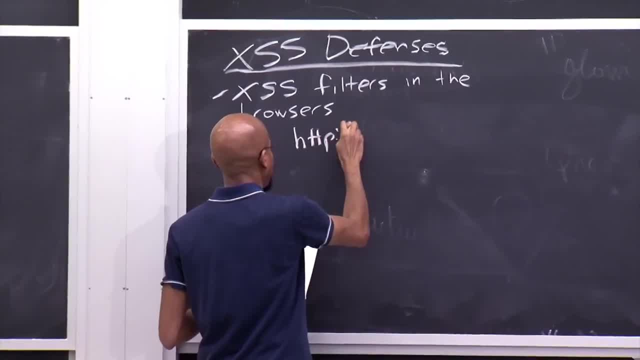 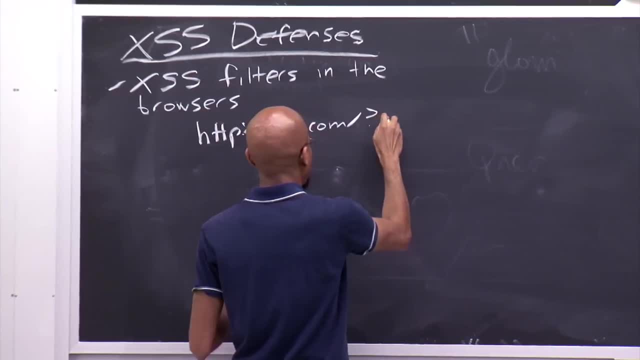 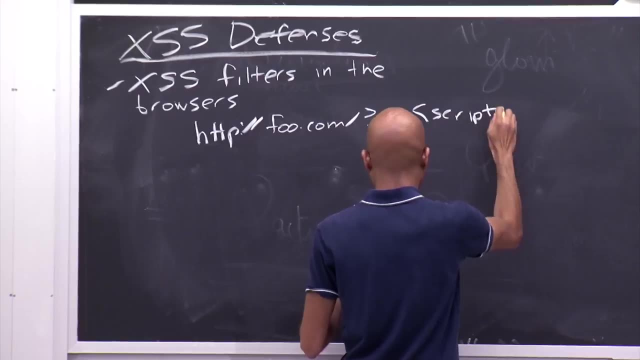 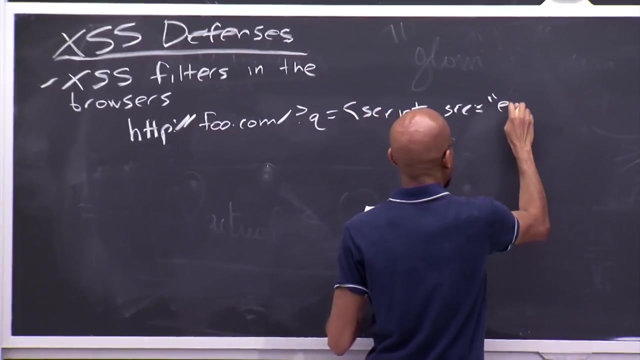 So if you have some URL that looks like this, so foocom, and then you have some question mark and then some query string you're going to submit. This is very similar to the example that I tried. third, So I just set this source to something like evilcom. 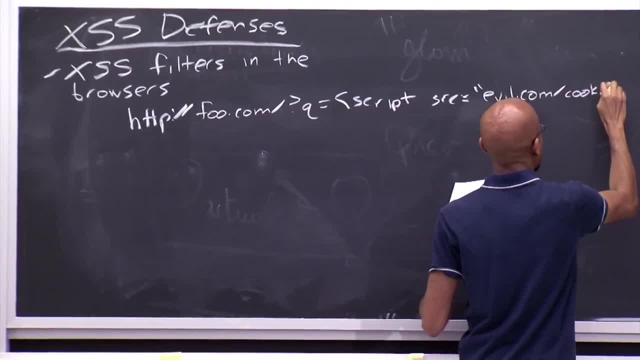 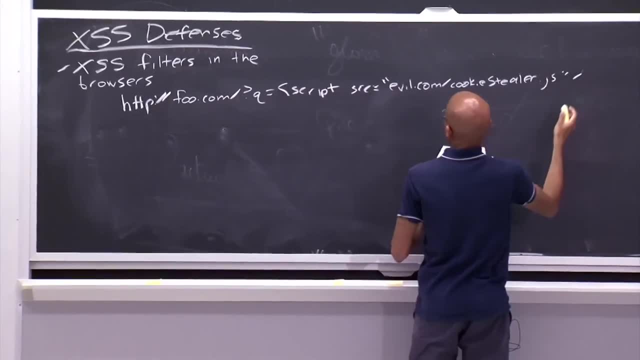 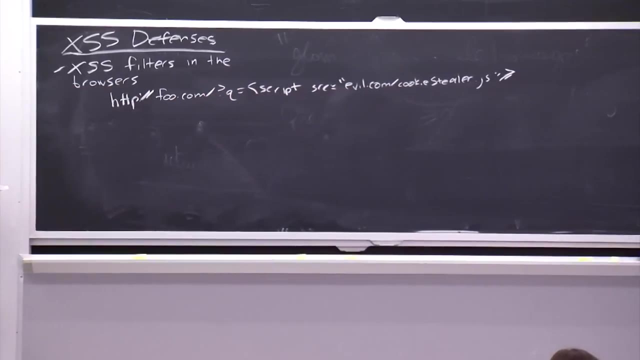 CookieStealerjs right, And so what ended up happening is that when I tried an example similar to this, the browser actually rejected it out of hand. So we saw that it didn't even work And the reason why it didn't work. 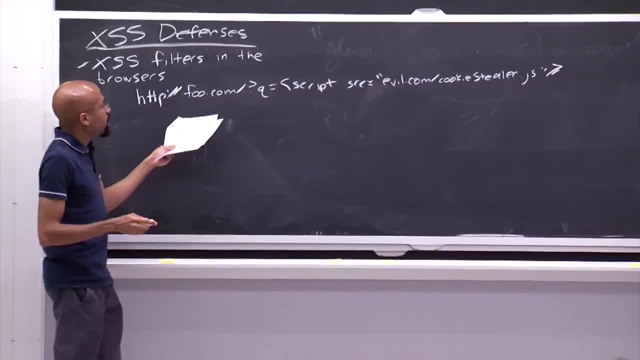 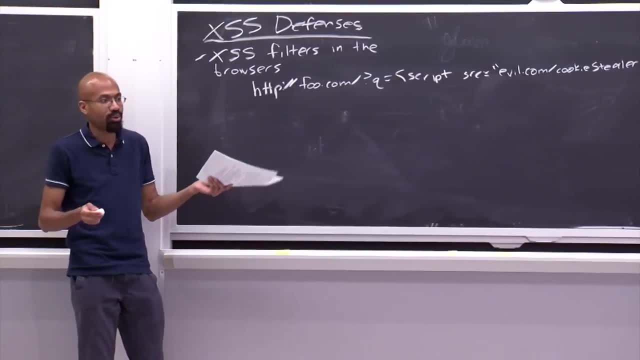 is because the browser looked and said: is there an embedded script tag in a URL, Right? So basically it's a very simple heuristic for figuring out if something evil has probably gone on. Because no legitimate developer or no developer. that's sane. 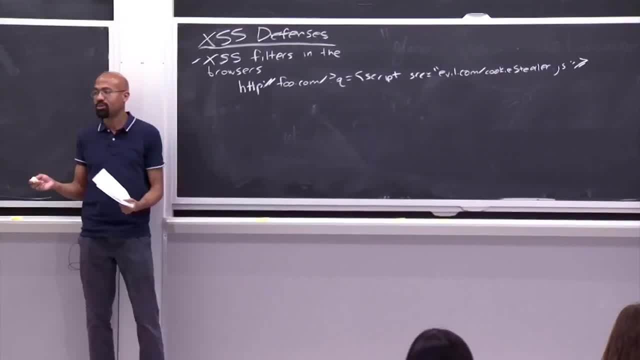 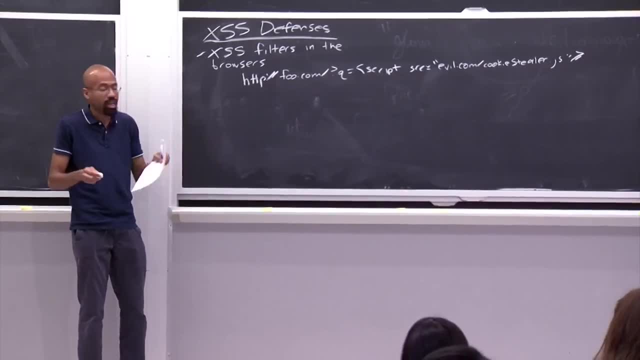 should be doing stuff like this, Right? So there's actually these configuration options in your browser you can use to turn these things on and off Occasionally. this is useful for testing, if you just want to inject some JavaScript really quick and dirty, But this is almost always a sign of chicanery. 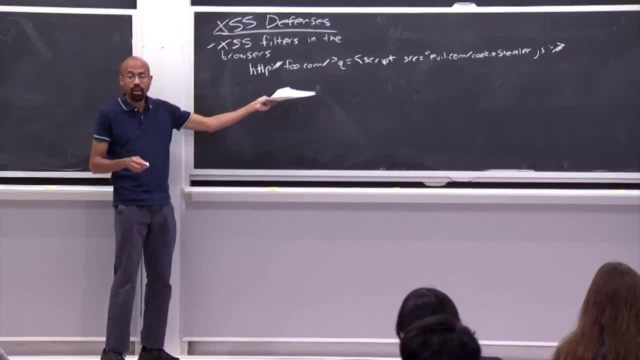 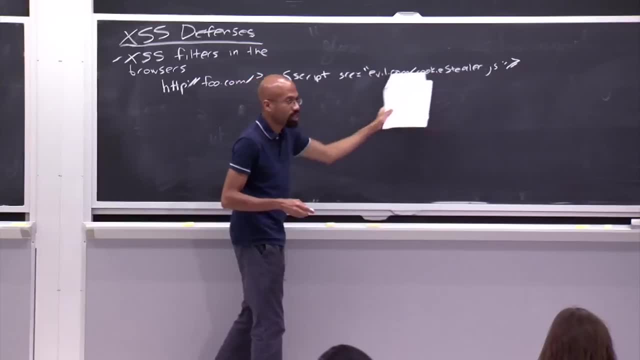 So, for example, Chrome and IE have a built-in filter that will look at your URL value in the address bar. look for things like this And if it's there, they will do things like: maybe delete this whole thing completely. They will maybe change the source to be empty. 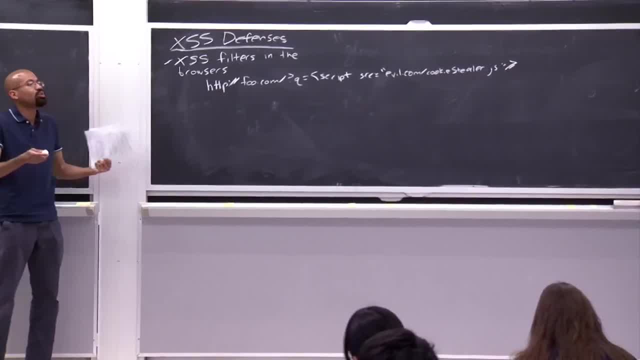 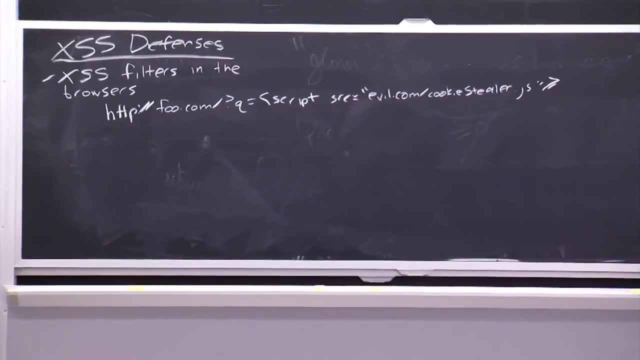 stuff like that, And so essentially to get to your question, there's a bunch of heuristics that the browsers have to identify things like this, And if you look at the OWASP site, they actually collect examples of heuristics you can use to detect cross-site scripting. 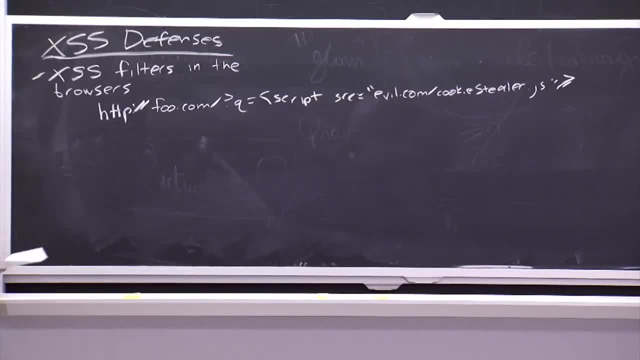 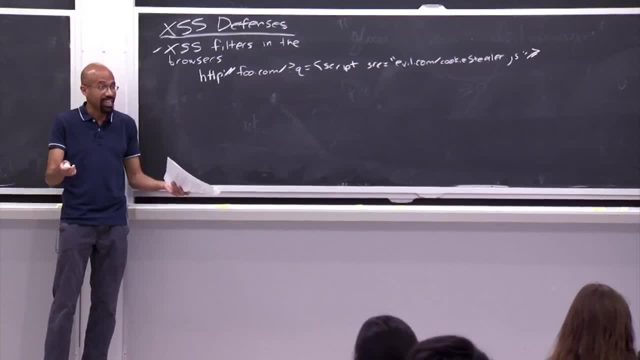 as well as tricks you can use to bypass those filters. Right, So it's very funny. So the first thing I wanted to do for the demo is do something like this, and it didn't work. So then I went to the OWASP cheat sheet. 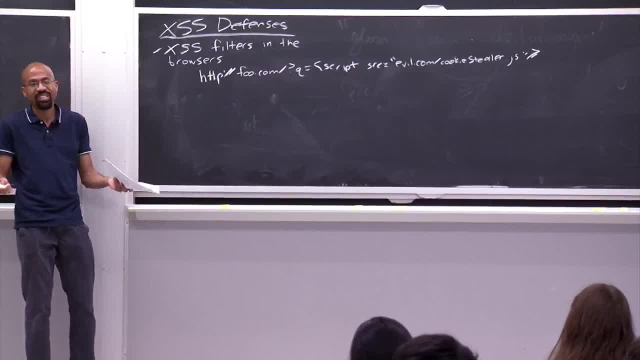 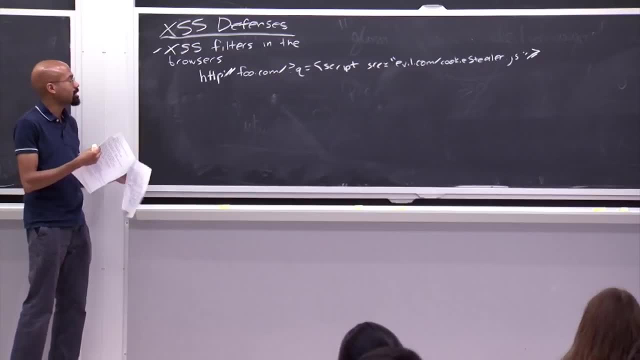 I looked at the third thing they suggested, and the third thing they suggested worked, which was that sort of broken image syntax type stuff. So the basic problem with just relying on this is that, like I said, there's a lot of different ways. 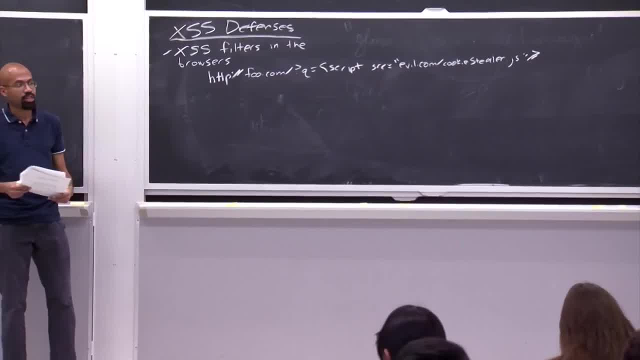 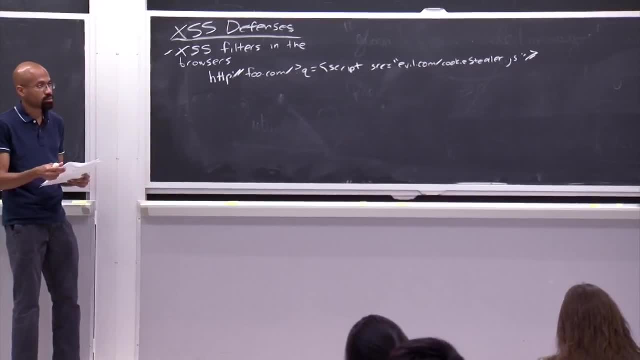 to force the CSS and HTML parsers to mal-parse something. So these things are sort of not complete solutions. They don't have the perfect coverage. Shouldn't this just be deleted from browsers, Because it seems like it's not the browser's job to do this? It's not the browser's job to sanitize This kind of stuff. I mean, you can imagine sort of having the browser sit atop a proxy, for example, and maybe the proxy did sort of cleaning like this. I mean intuitively one reason why it might make sense. to do it inside the browser is because so many of the legitimate parsing engines are inside the browser, right? So presumably if you're closer to where the actual parsing is being done it's better. But you're right that in practice you can imagine there being sort of like defense in layers. 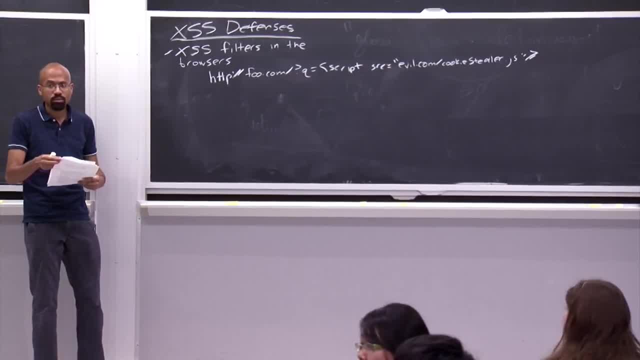 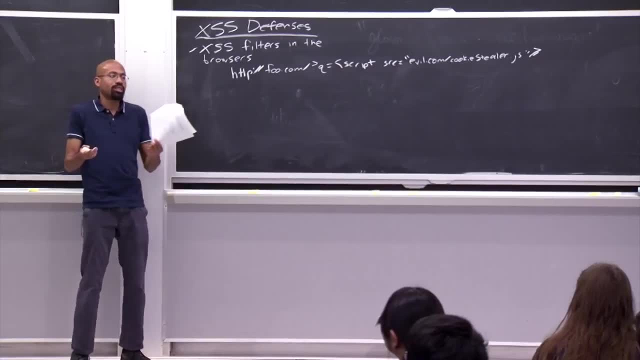 basically, I think what you're saying is like it's the developer, the web developer's job, not the client's job. to sanitize, Yeah Well, but I mean that's kind of like saying so. in a certain sense we could say that about processes too. 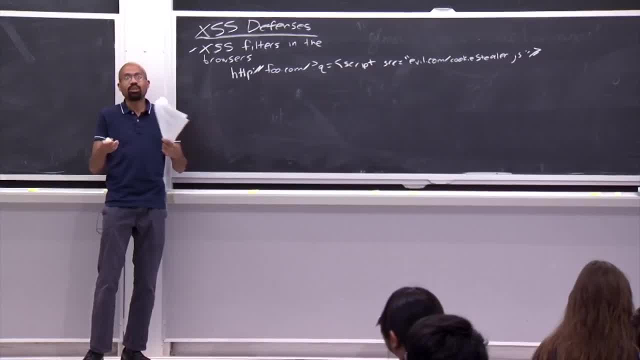 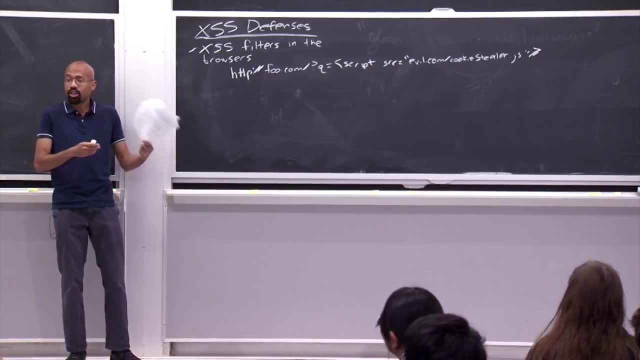 in Unix or Windows right. So we could say it's sort of developer's job to make sure that those things stay isolated. But in fact the OS, and the hardware as well, has an important role to play because presumably it's trusted whereas any two arbitrary programs written. by any two arbitrary developers may or may not be trusted to sort of implement security correctly, But you're correct. in fact, frameworks like Django or whatnot, they actually try to help you to get around some of these problems. So anyway, so yeah. 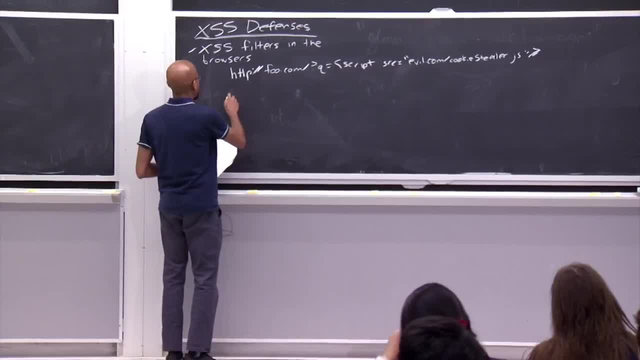 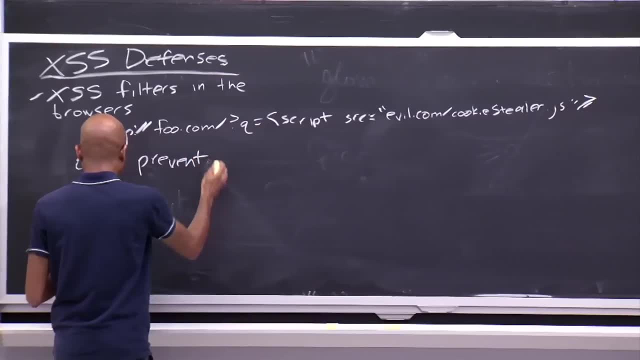 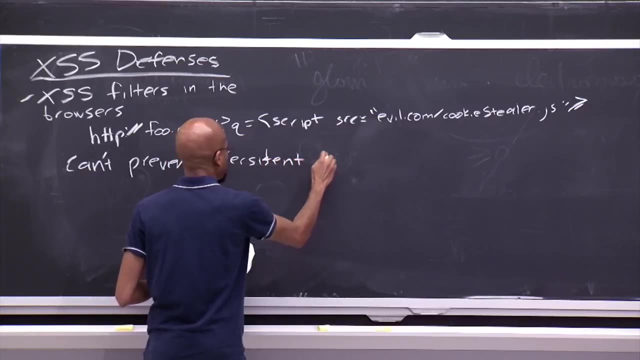 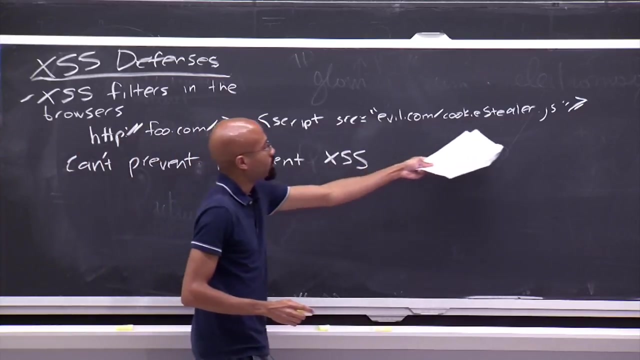 So filters are not a perfect solution And also filters can't prevent what's known as persistent cross-site scripting attacks. This is known as sort of a reflected or transient one, because this script code just sort of lives in the URL. Then, once the user's closed, that URL, basically the attack's. 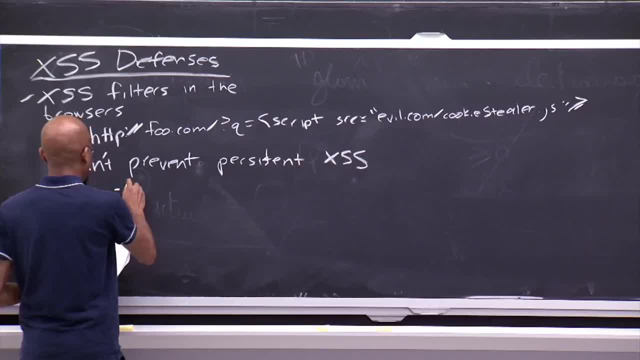 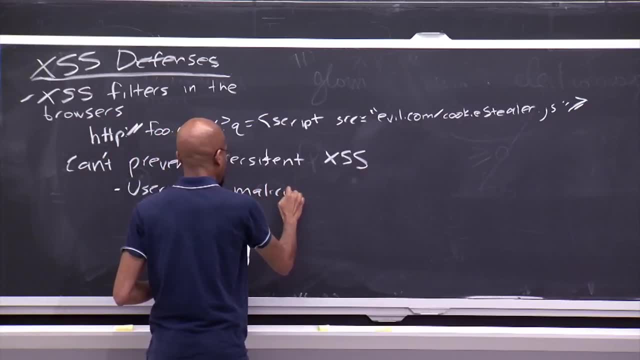 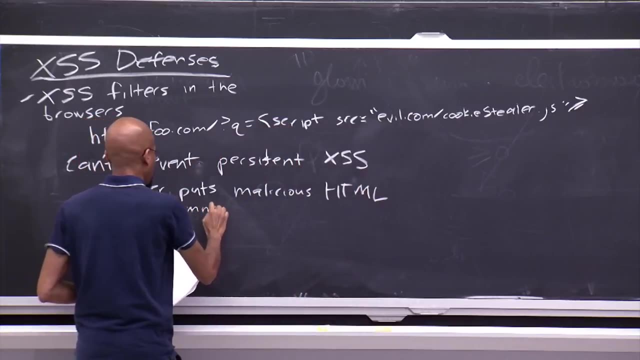 gone. But you can imagine that you could have someone who user puts malicious HTML in the comment section for a website And if the web server actually accepts that comment as valid, then that comment with this malicious payload can essentially live there forever, right. 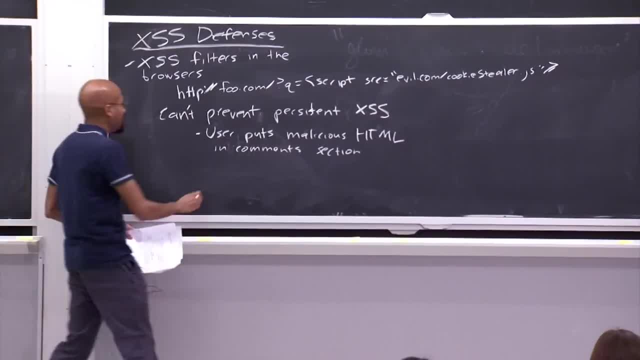 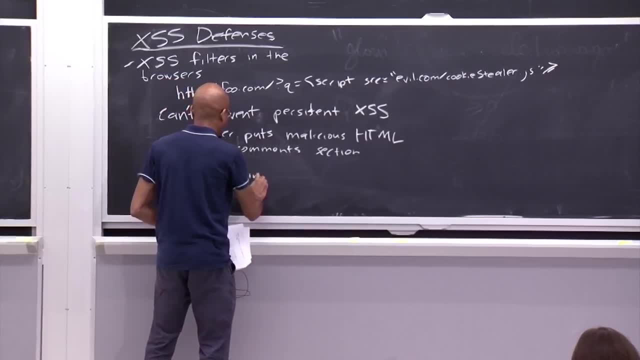 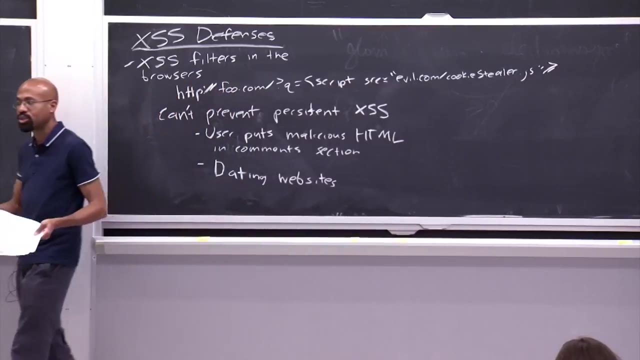 So whenever any user goes there, They would be exposed to that malicious content. Another example, which is sort of funny and sad as all these things is like, if you look at dating websites. So some dating websites actually allow users to put full-blown HTML in their profile. 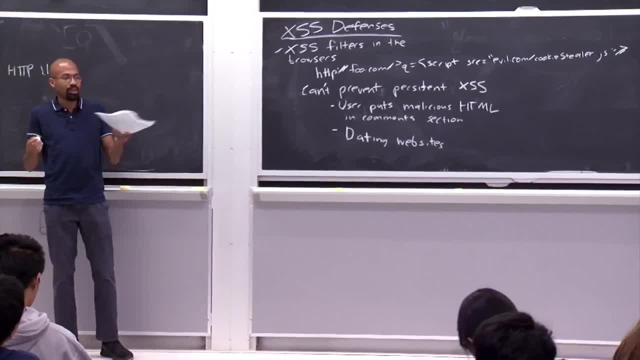 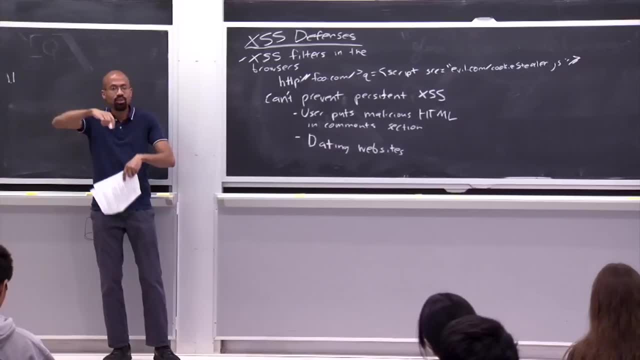 So what does that mean? So when someone else is lonely, presumably they're looking to find the one true soul match- they go to your website. They're going to run HTML that you've crafted in the context of like their session, right. 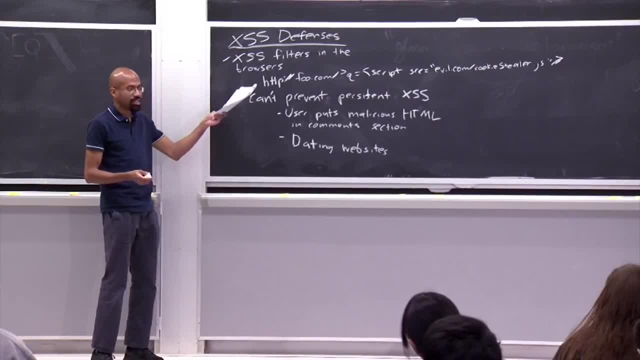 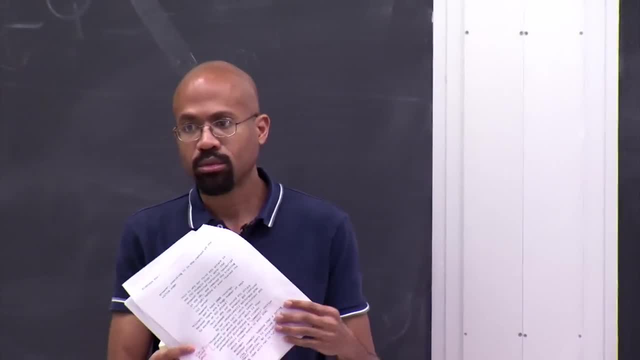 So that can also be a very damaging attack as well, And so just doing these kinds of filters don't protect against things like that. So, for example, when you use it for something in the comment section, presumably does that by sending like a post that information goes. 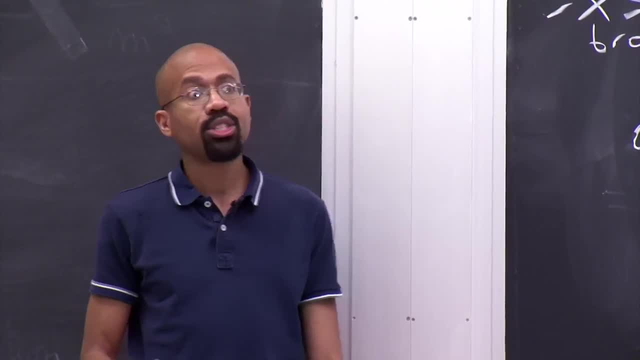 to the server's post variable or something like that. So there's a bunch of different ways you can imagine doing it. Yeah, so one way you can imagine doing it is a post. Another way you can imagine doing it is a dynamic XML HTTP. 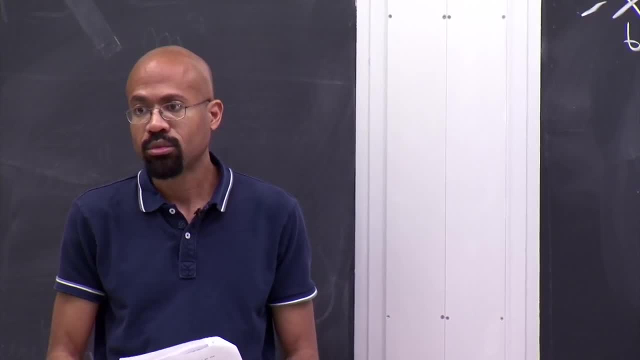 request: OK, But if it's like a post, why can't you just scan through it, Do the same thing that you have in the browser? Yes, So you're exactly correct about that, And we'll discuss some of that in a second. 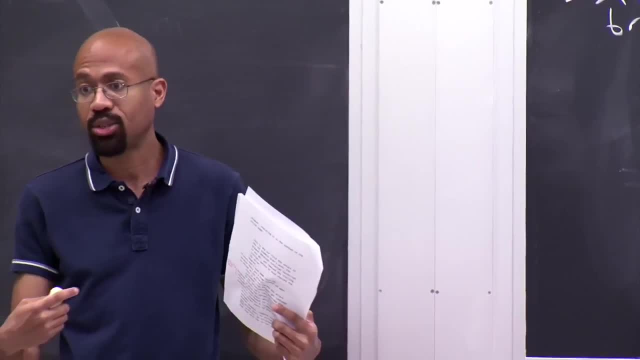 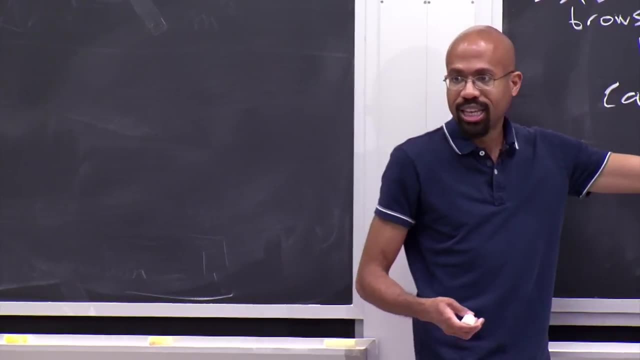 But you're exactly correct that the server side of the application should be very defensive and mistrustful of this stuff. So you're exactly right. So you can imagine that when the server maybe saw something like this, it would perform some type of filtering on its side. 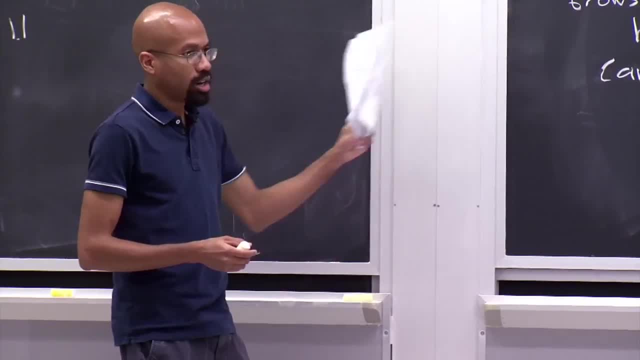 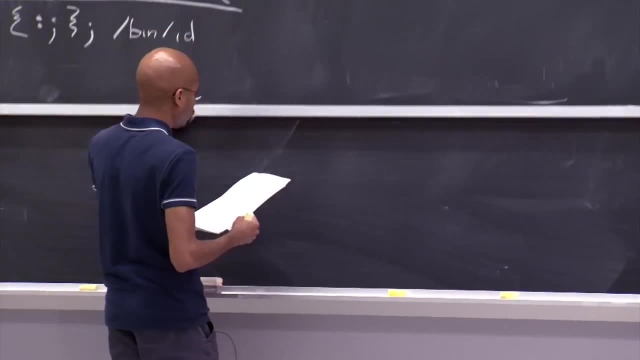 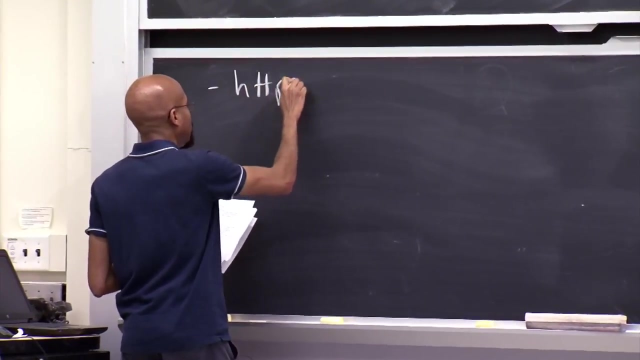 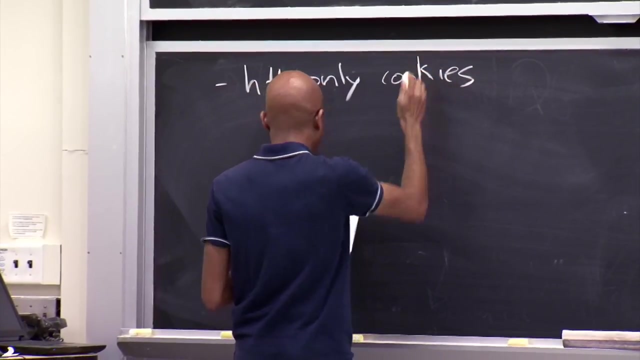 even if the browser did not. You're correct about that, All right, so that's basically a survey of these cross-site filters in the browser. So another defense against cross-site scripting is something known as HTTP only cookies, And so the basic idea behind this. 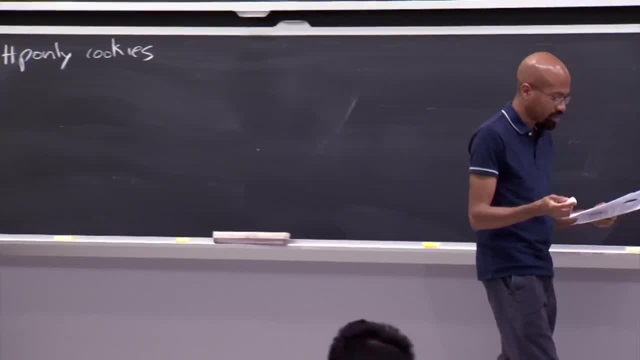 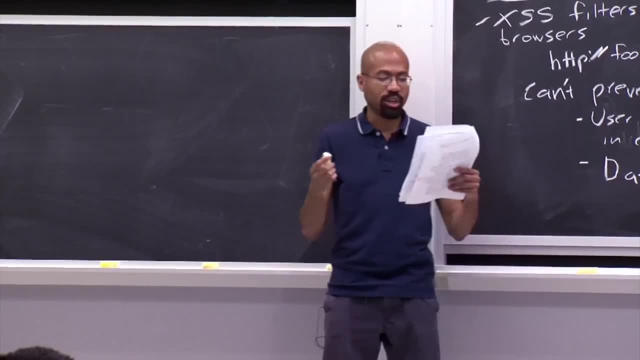 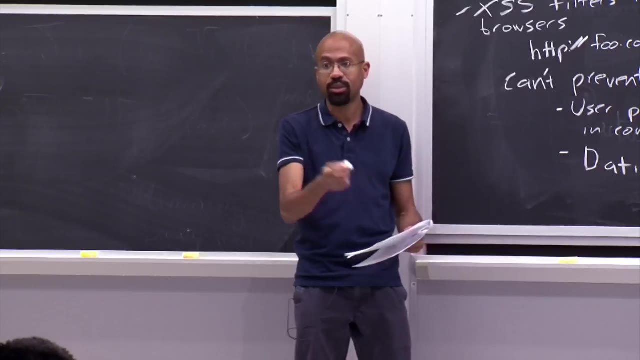 is that a server can actually tell the browser that client-side JavaScript should not be able to access a particular cookie, And so basically the server can just send a header value in response. in the set cookie field It can say: hey, don't let client-side JavaScript 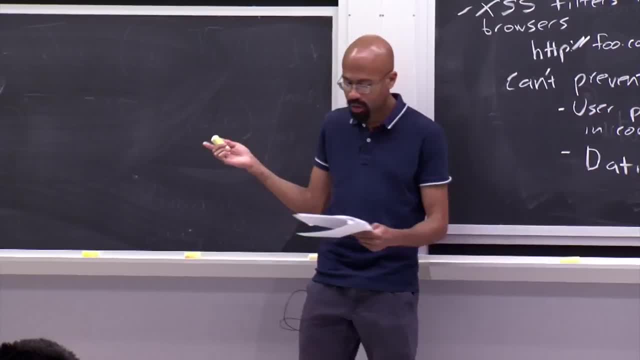 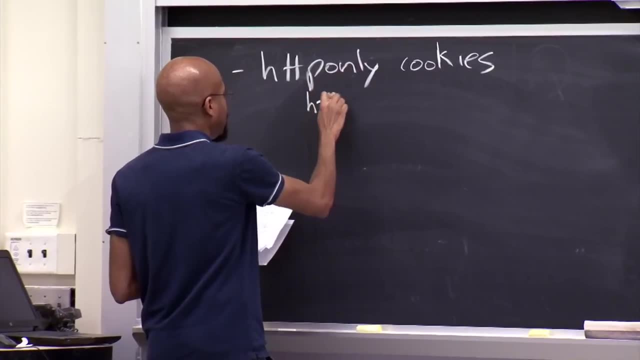 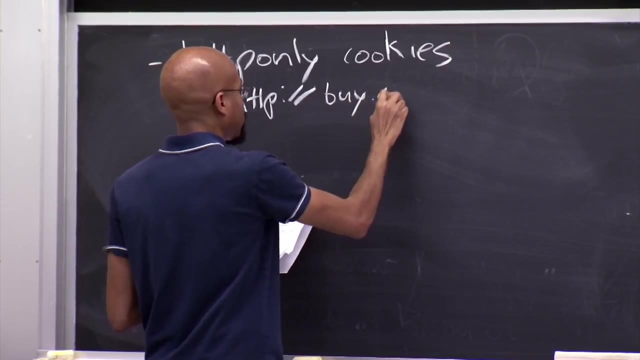 manipulate this cookie, So only the server can do this, And so this is only a partial defense, though, because the attacker can still issue requests that contain the user's cookies. So this was the cross-site request forgery that we looked at in last lecture. 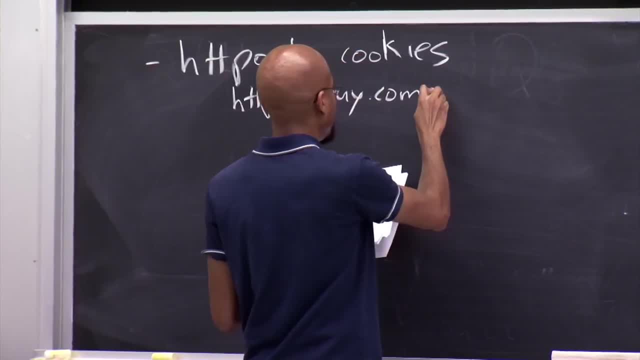 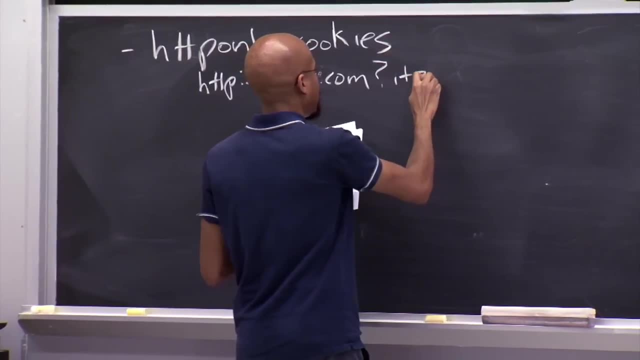 So even if JavaScript code can't manipulate cookies, the attacker can still do things like conjure up a URL to some e-comment- OK, OK, OK, OK. site, let's say buycom, the attacker can put whatever item the attacker wants to buy. 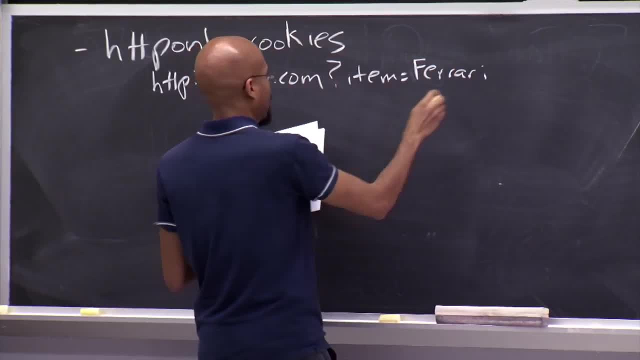 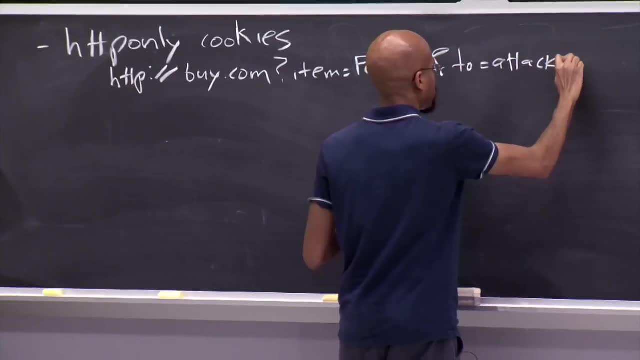 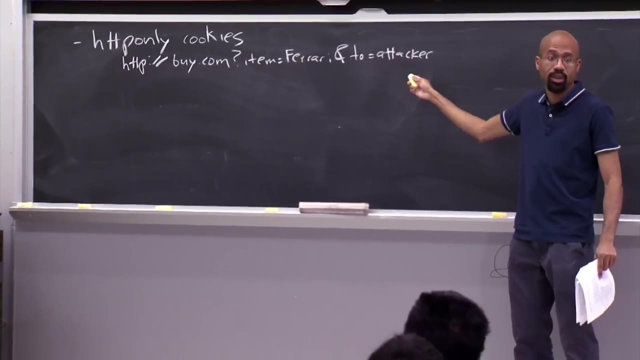 So it puts a Ferrari, for example, And then the attacker can then say: who should this go to? This should go to the attacker, And so, even though client-side JavaScript can't access the cookie, there's nothing that prevents the attacker from just conjuring up a URL like this. 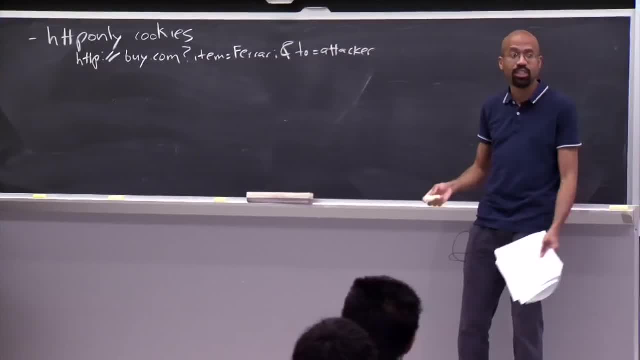 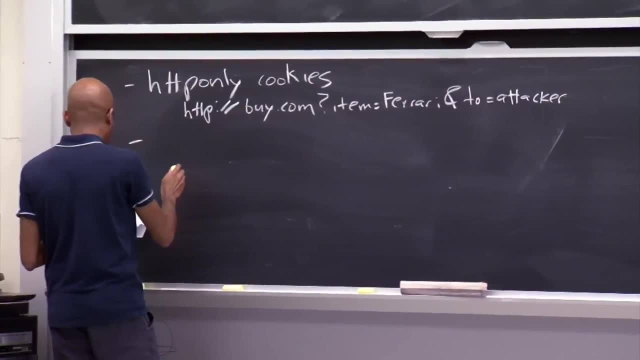 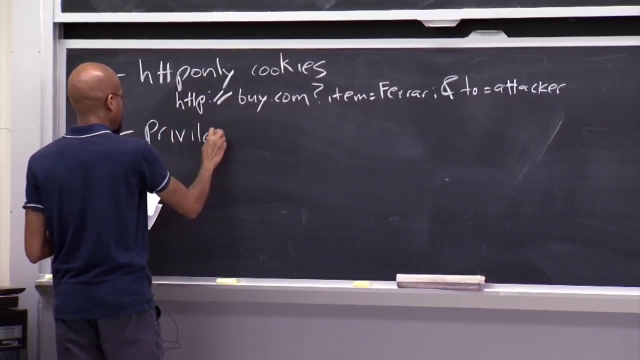 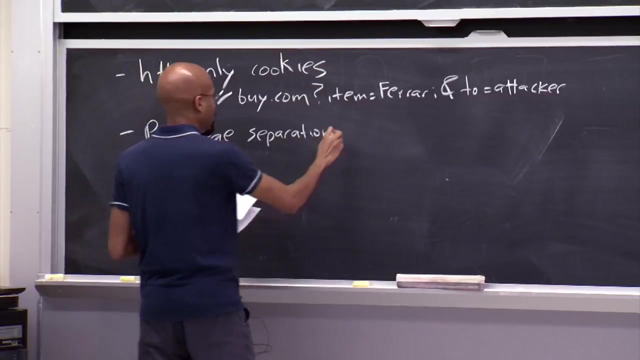 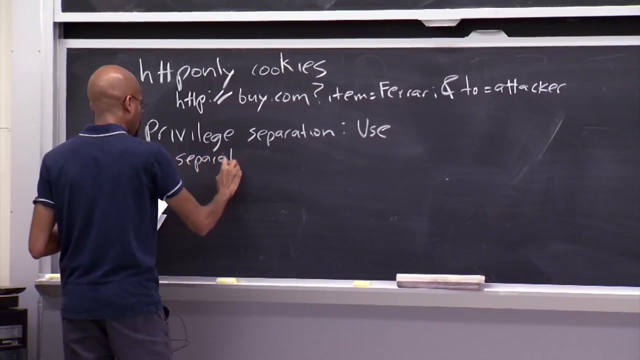 This is what some of the CSRF tokens help to prevent against, which we'll talk about a little bit later. So another thing that you can try to do to prevent these cross-site scripting attacks is privilege separation, And so the idea here is basically that you want to use a separate domain for all the content. 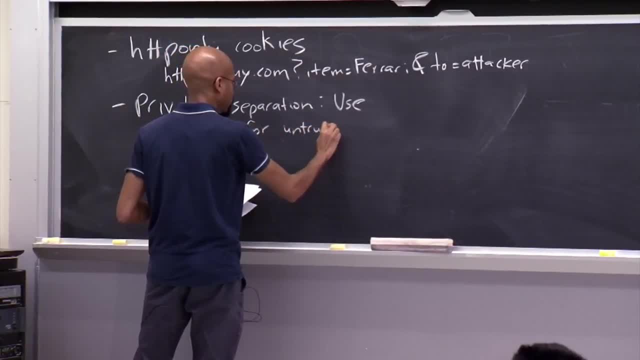 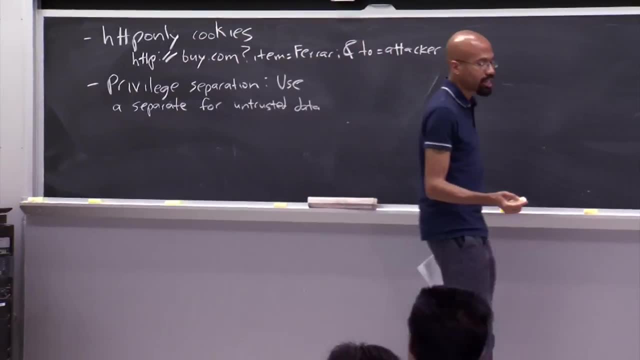 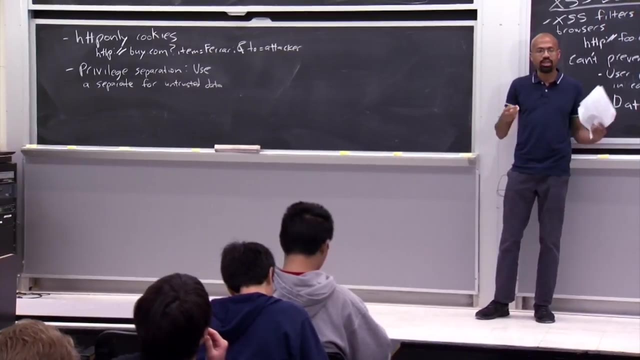 that is untrusted, And so, for example, a lot of the online service providers for things like email or online productivity suites, so think like Google Docs, Office 365, so on and so forth- they actually use a separate domain to host user-submitted content. 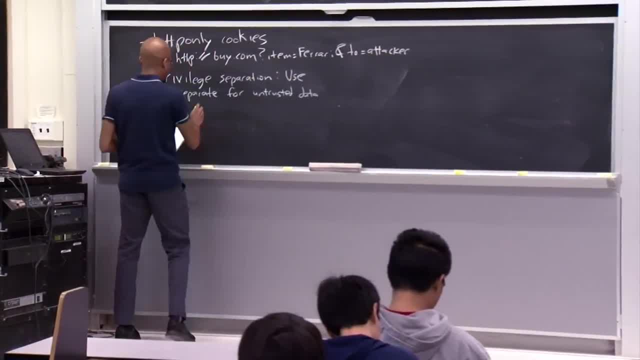 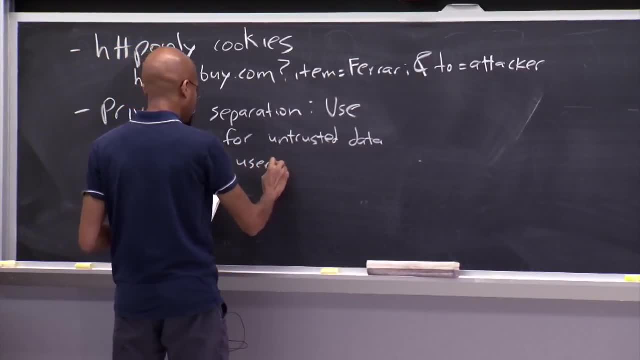 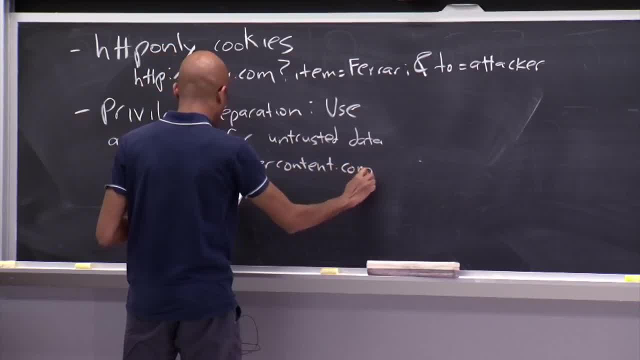 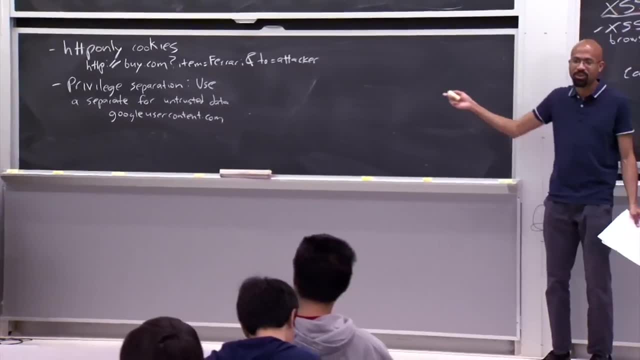 Googlecom, Googlecom, Googlecom, Googlecom, Googlecom. And so here they would put things like cached copies of pages, your Gmail attachments and things like this. And at least as of a year or two ago, this was one of the top 25 Alexa visited domains. 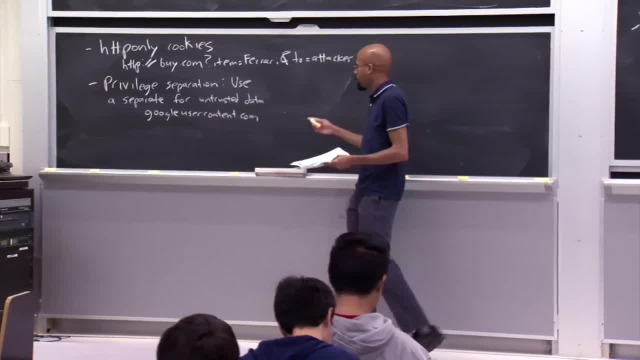 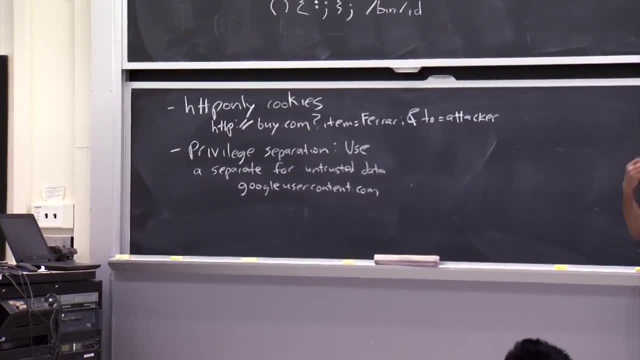 because Google services are so popular. So what's the advantage of putting stuff in here? Well, the hope at least, is that if there is some type of cross-site scripting vulnerability or something like this Googlecom in the user-submitted content, then hopefully the damage 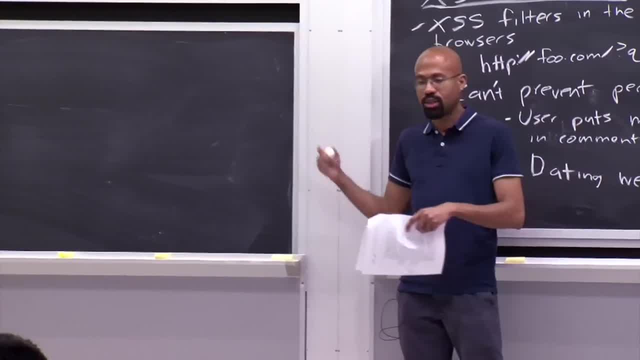 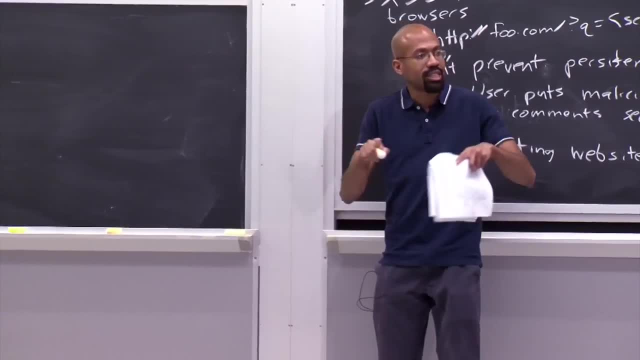 would just be limited to that domain. It wouldn't actually affect the full-blown googlecom. This isn't a perfect defense, though, because user-submitted content may have references to things from googlecom, And so, once again, this is only sort. 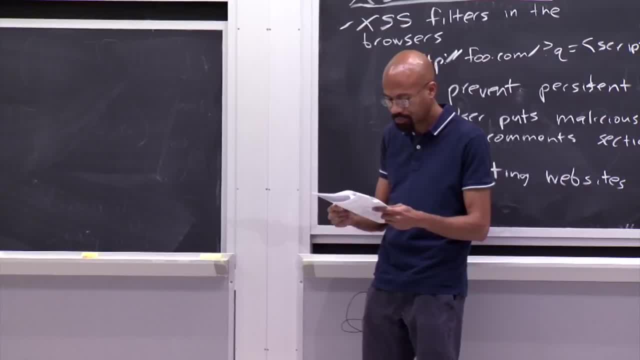 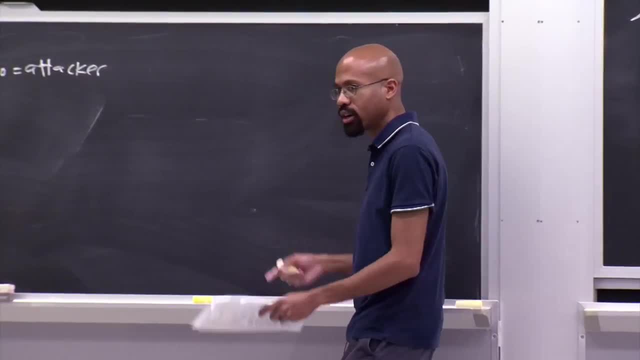 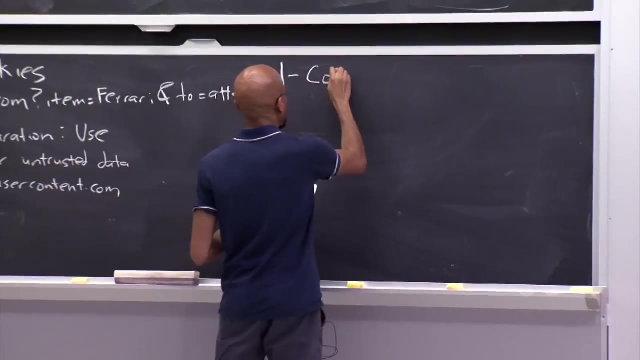 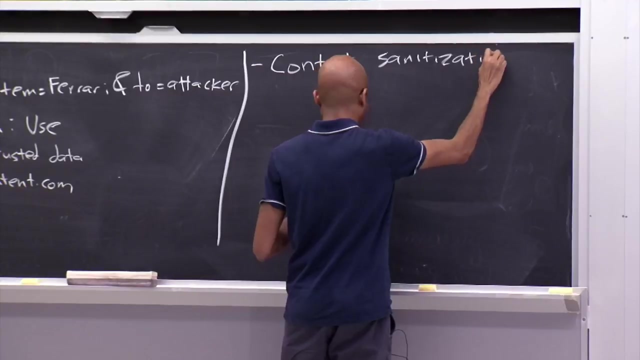 of like a partial fix for a much more pervasive problem. Now, another thing you could do- and this gets back to the gentleman's suggestion over here- is that we can actually do content standardization, And so the idea here is that, essentially whenever you 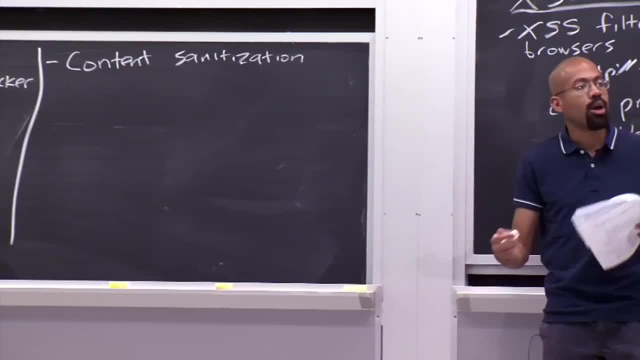 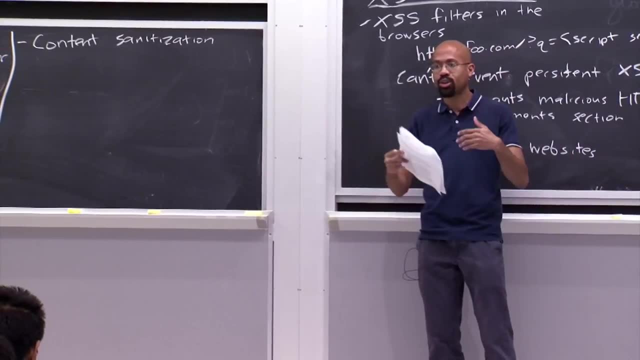 where you can be the browser, where you can be the web server, whatever. whenever you receive untrusted content, you don't trust it at all, And so you go through it and you do things to sort of render it sort of neutral. 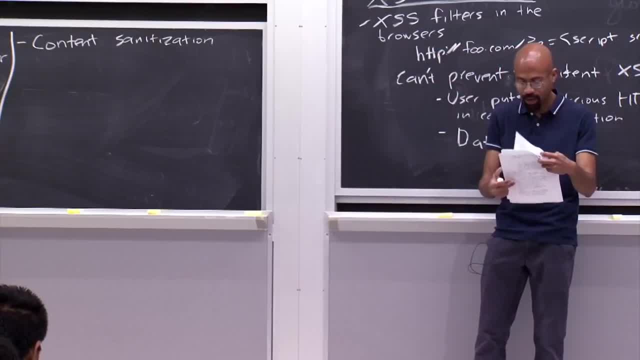 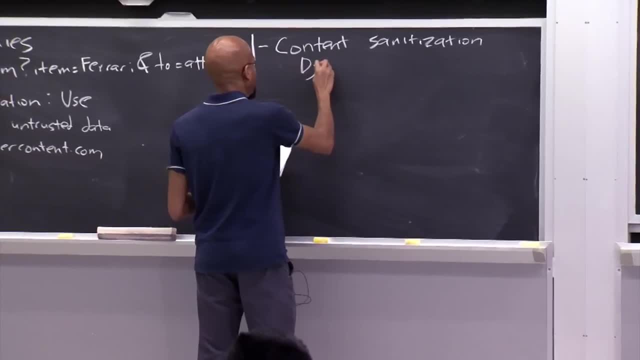 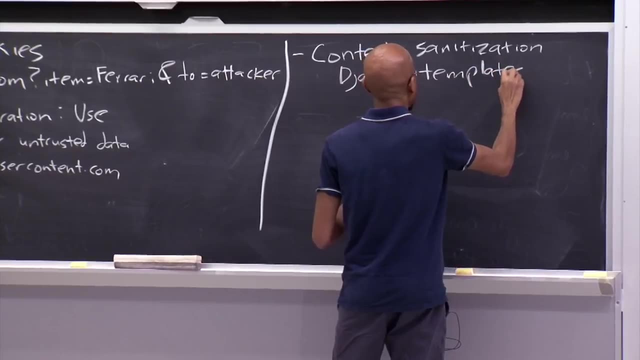 Such that it can't actually execute code or subvert your system in any way, And so an example of this is the Django template system, And so Django is an example of a web framework. So, basically, at a high level, a web framework. 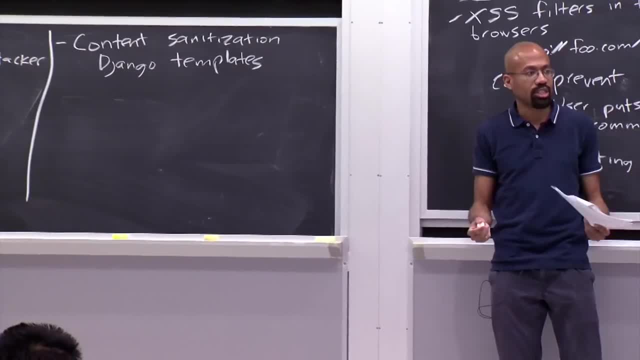 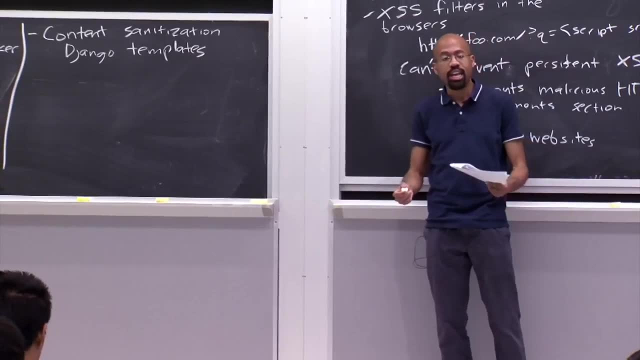 is something that helps to automate and secure some of the sort of tedious tasks of developing a website. So, OK, OK, OK, OK, OK, Great. It will help you with making database access easier. It will help you with doing things like session management. 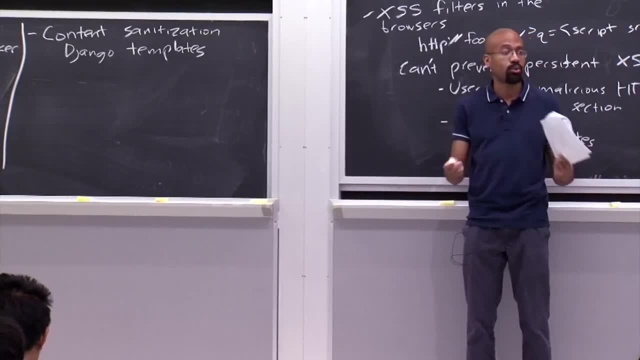 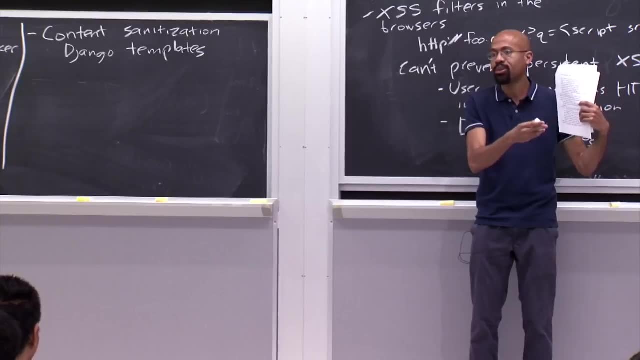 And it will also help you with maintaining a consistent look and feel across your website, And so one way to maintain that consistent look and feel is to use this notion of templates Right, So all of your pages automatically start out with the same CSS and things like that. 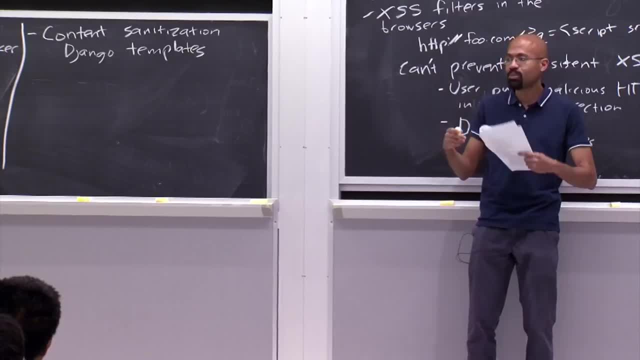 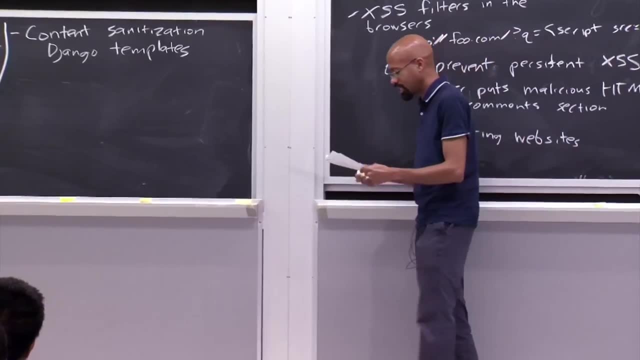 the same styles. But then there's these portions in the web page where you can specialize it with the particular news article that's at the top of the top of everybody's mind, or something like that, or user-specific content. So, for example, in Django, you can look at a template. 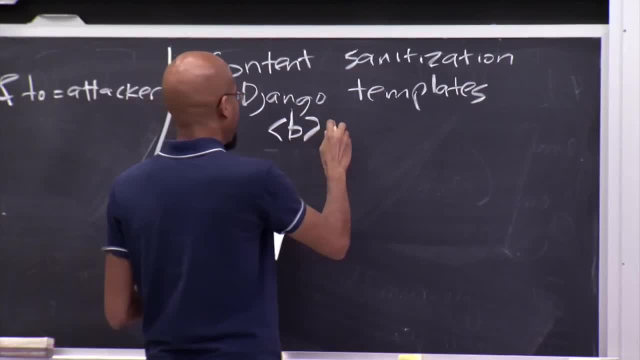 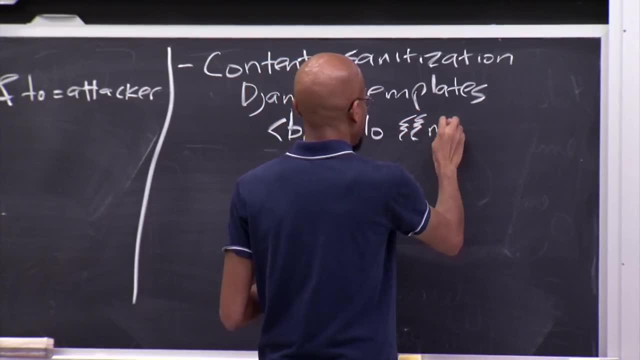 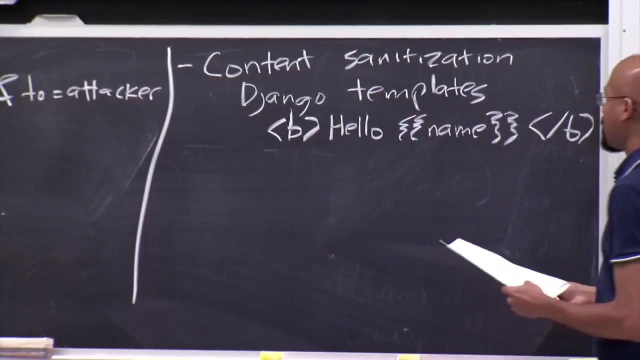 and it might look like something like this: So you have a bold tag, it says hello, and then you have these braces here, these double braces, and it says name, And so essentially, what this means is that this is like a placeholder variable. 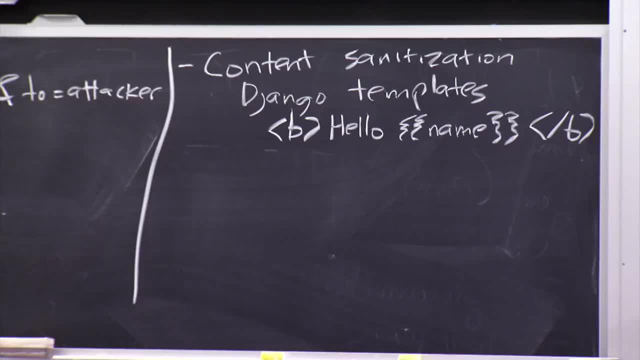 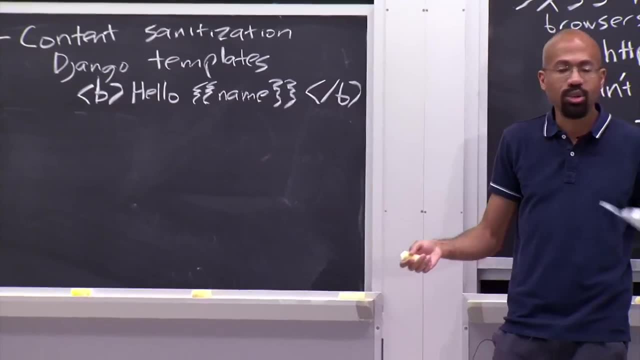 So essentially these pages get dynamically generated. So when the user goes to a Django site, the Django server says: OK, well, this name is going to be somewhere, who knows, in the cookie. maybe it's going to be in a CGI string, whatever. 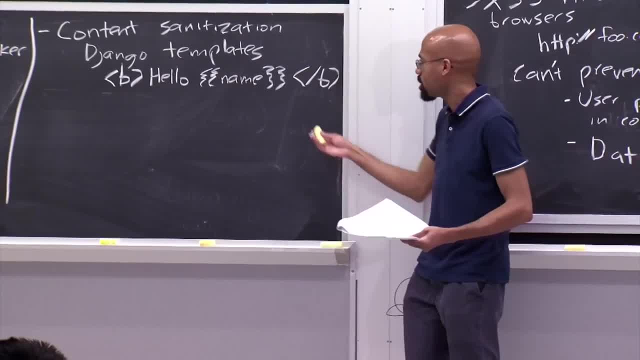 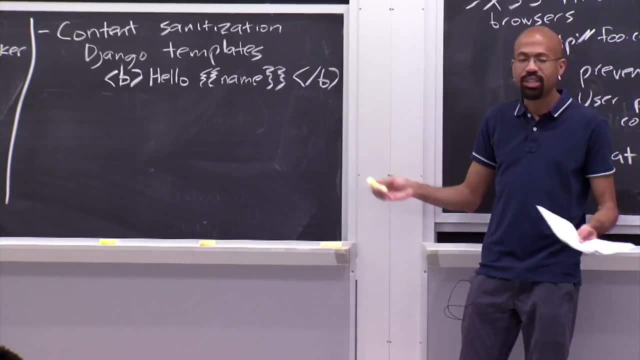 And so, as the Django server dynamically generates the page to return to the user, it replaces the special reference here with whatever the value of this variable is. So it's pretty straightforward. This is kind of like that dinky CGI server I showed you. 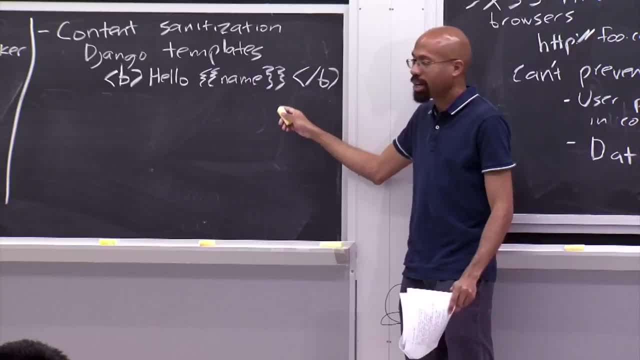 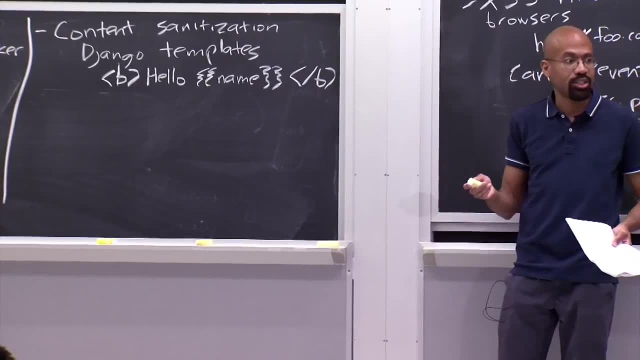 So just reflecting user-submitted content right here. But Django actually does it better than the silly CGI server that I showed you, because it uses this notion of content standardization. So Django expects that users may be adversarial, So it's not just going to directly put the value. 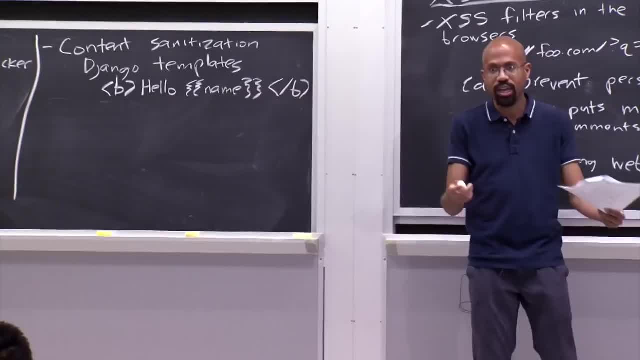 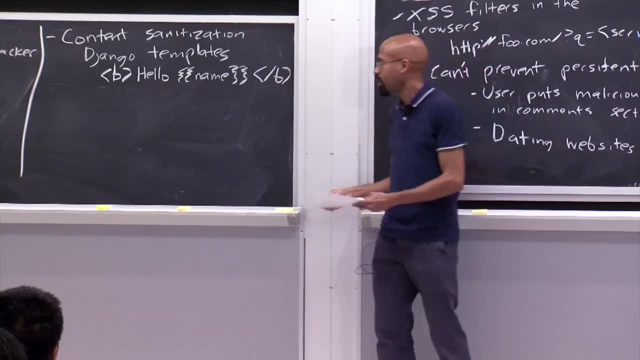 of the name variable here. Instead, it is going to encode it in such a way that this content will never be able to escape out of the HTML context and execute JavaScript or something like this. So, for example, one thing it will do is it will take the angle brackets. 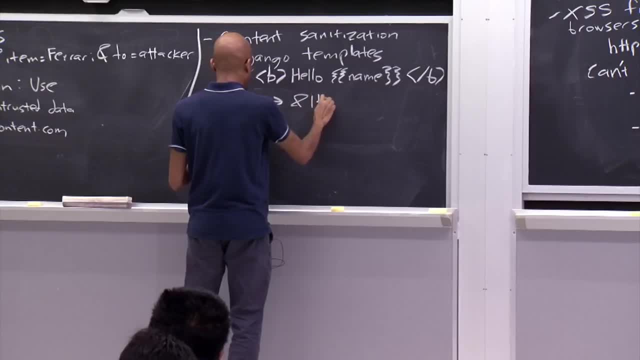 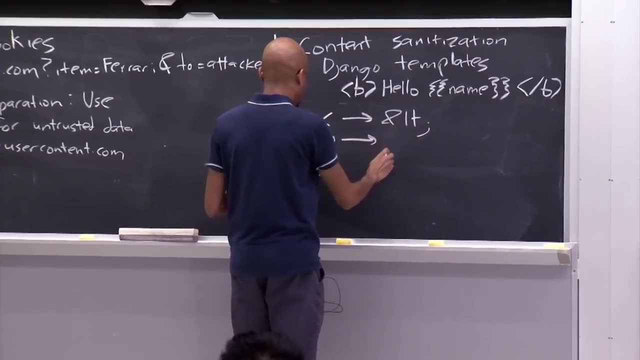 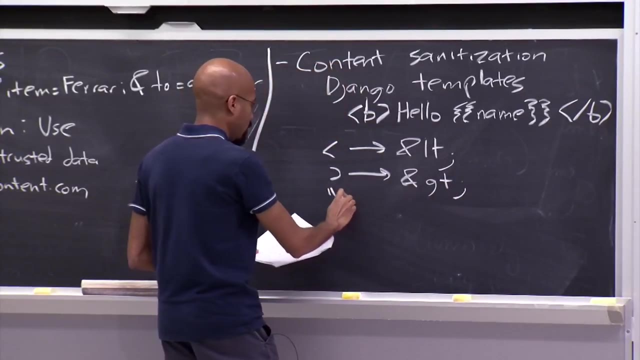 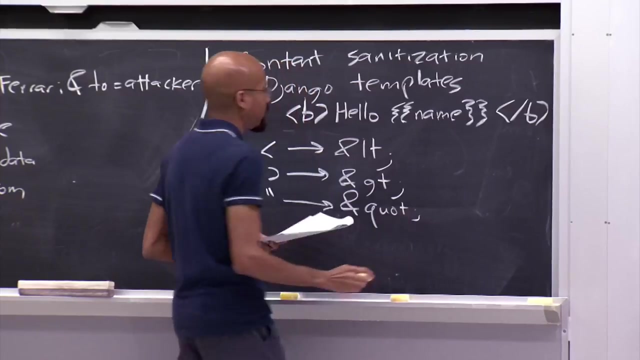 and it will translate them into these HTML entities. So the less than character gets transformed into this, The greater than character gets translated into this. Double quotations get translated into ampersand quote, and so on and so forth. And so what this ensures is that if the content the user put in 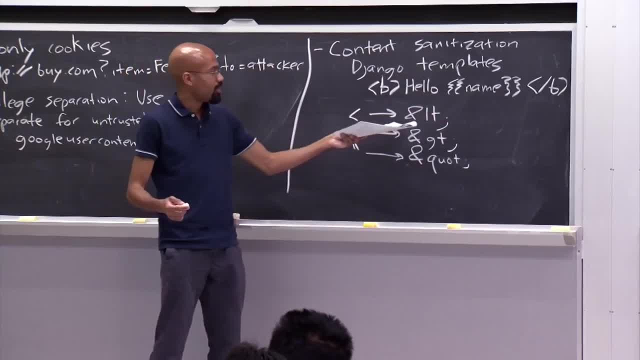 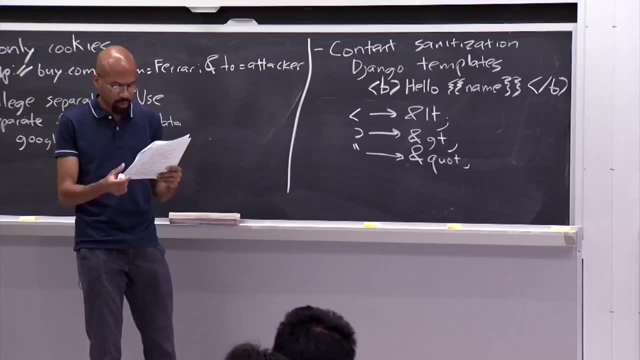 put in name, actually tries to contain angle brackets or things like this, then it will basically be neutered And it will be translated into something that will not be interpreted as HTML on the client side browser. So does that make sense? So now note that this is not a completely foolproof defense. 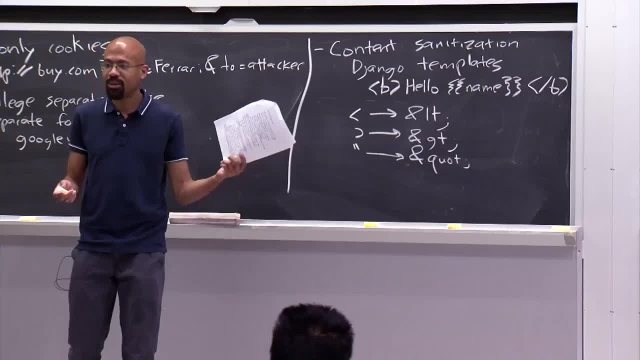 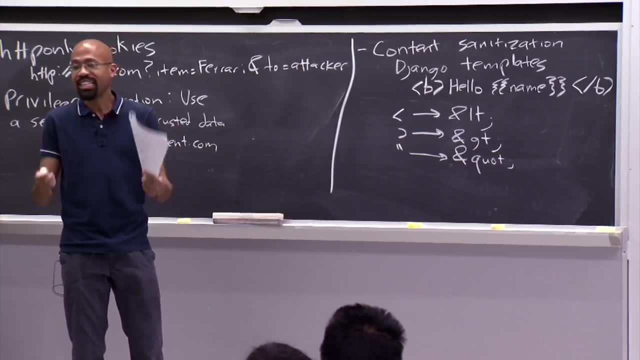 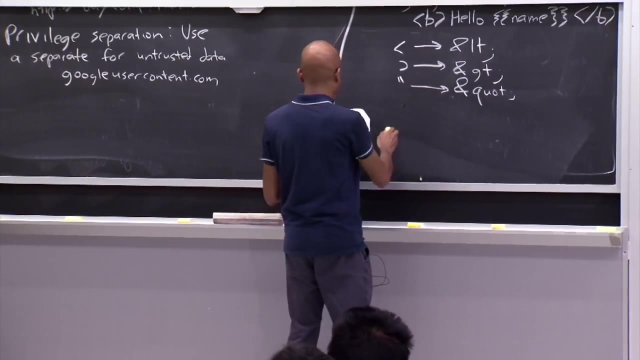 against some of this cross-site scripting stuff, And the reason, as we show in the example, is that these grammars for HTML and CSS and JavaScript are so complicated that it's very easy to confuse the browser's parser. So, for example, let's say that you had something like this: 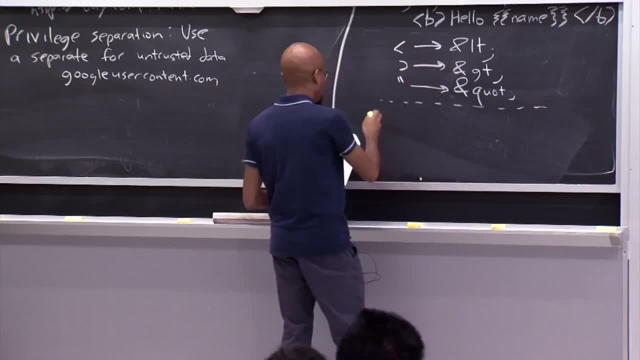 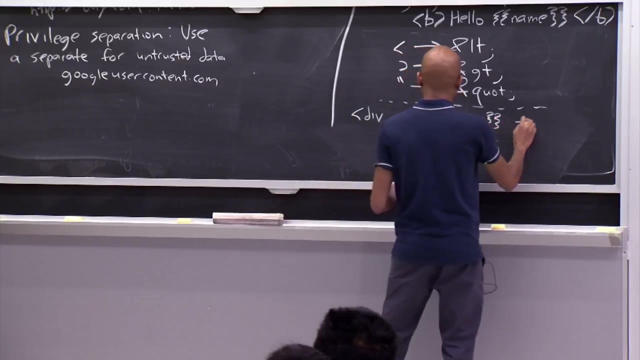 And this is a very common thing to do in frameworks like Django. So you have some div and then you want to set its class dynamically, So you set its class to some var, so on and so forth. So the idea is that when Django processes this, 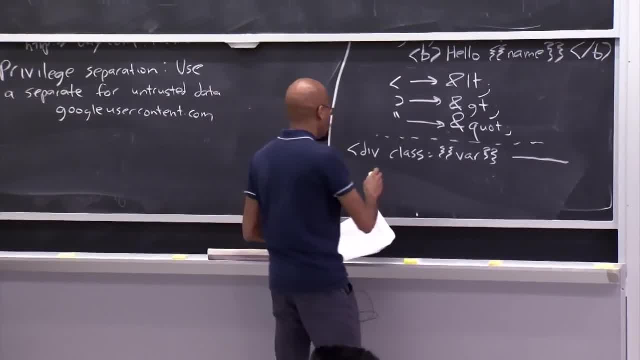 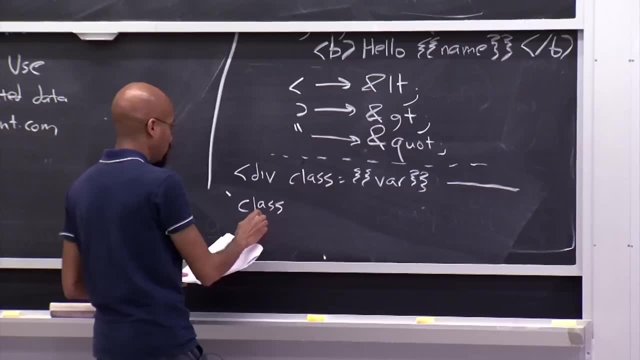 it should figure out what the current, what the current styling is and then put it in here. Well, one thing you can do is maybe the attacker supplies something like a string like this, So attacker will say: class 1.. OK, so far, so good, because that seems like a valid CSS. 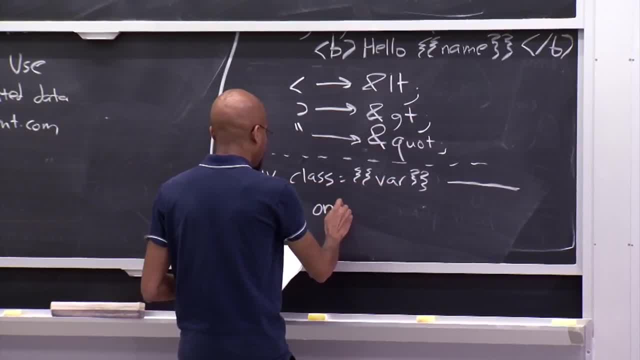 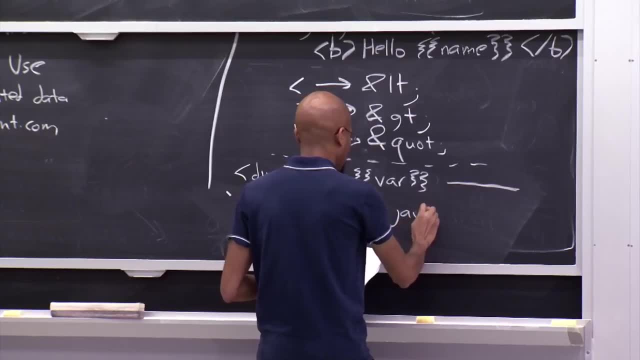 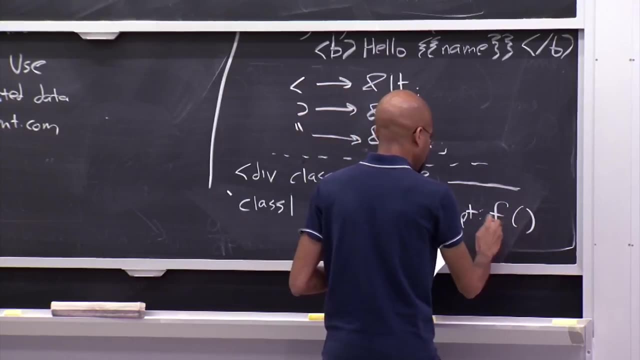 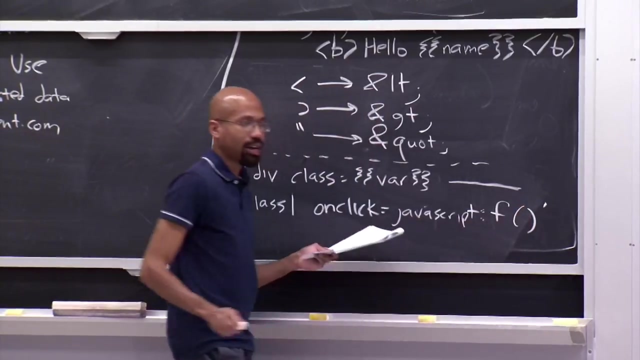 expression, But then the attacker will then try to put some JavaScript here, So it might say: onClick equals and then put JavaScript URL And then put some function call here. So this is malformed. The browser should probably just do a fail. stop here. But the problem is that if you've ever looked at the HTML for a real web page, all of it's broken. even for legitimate benevolent sites, People just can't hack HTML. So if the browser were to be fail, stop. literally no site that you enjoy would ever work- ever. 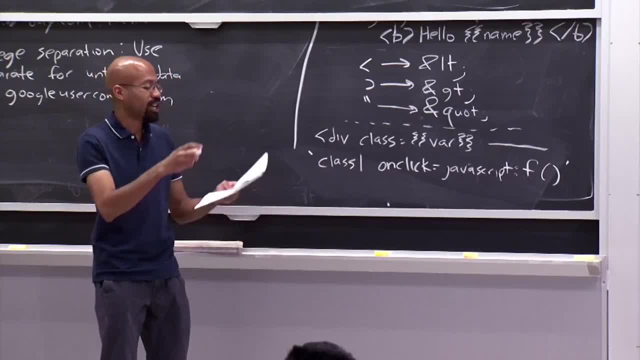 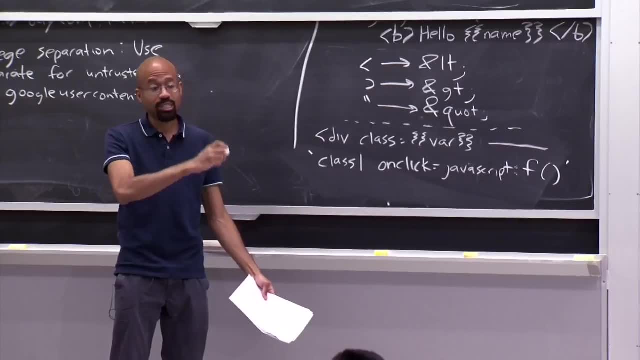 If you ever want to be disappointed- disappointed by the world, if I haven't helped you do that enough- open up your JavaScript console when you browse a website and see how many errors get spit out. Like, go to CNN and just see how many errors get spit out. 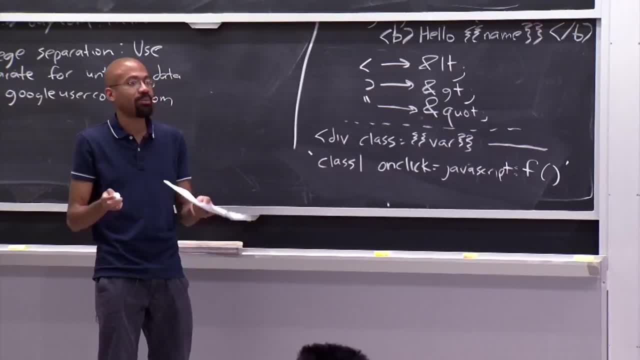 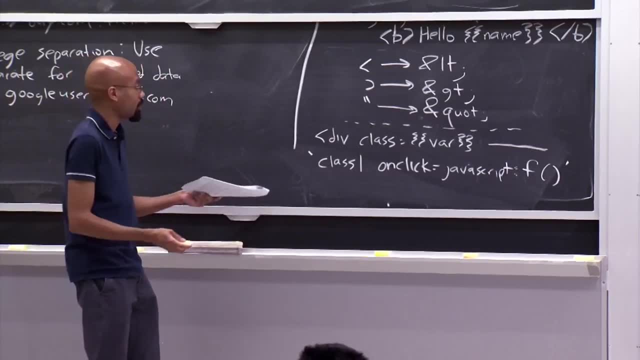 CNN basically kind of works. but it's very disturbing Because if you were to open up Acrobat Reader and you're just constantly throwing null pointer exceptions, you would feel a bit cheated by life. But in the web apparently we've learned to accept this. 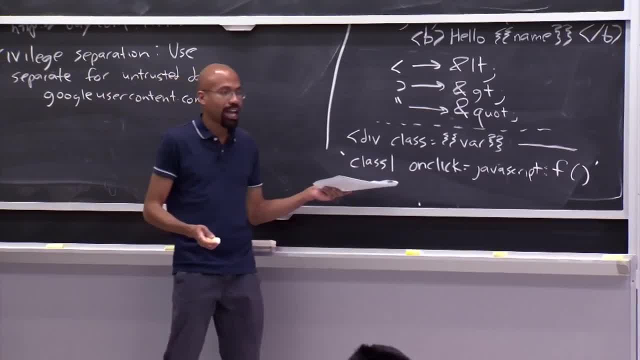 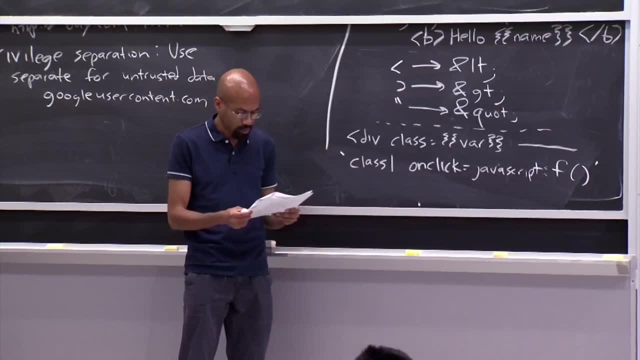 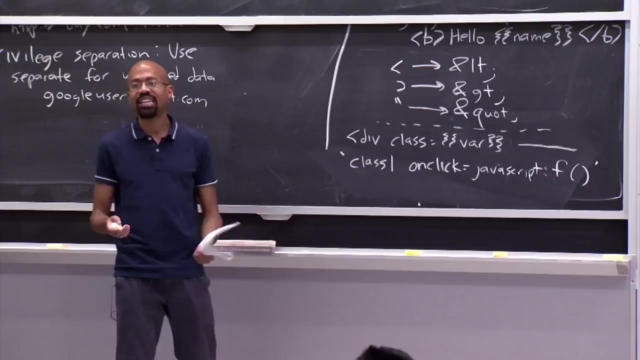 So because browsers have to be so tolerant of these things, they will actually try to massage malformed code into something that's seen as reasonable, And therein lies the security vulnerability. So I guess the take home point for this is that content sanitization kind of works. 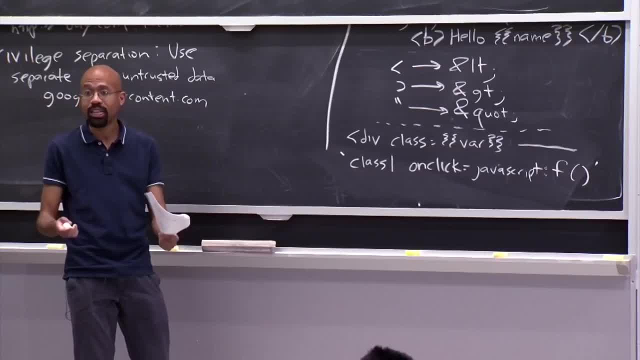 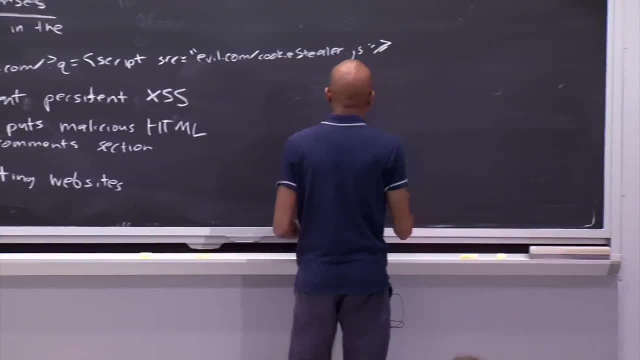 So it is literally better than nothing. It can actually catch a lot of cases, But in many cases it is not sort of a full defense, And so one thing you might actually think about doing is actually- I'll just put this over here- is, you might think, 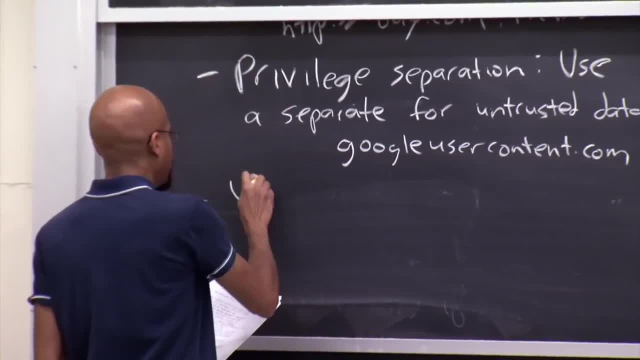 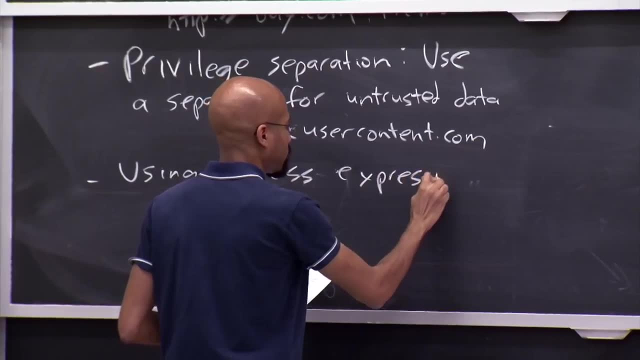 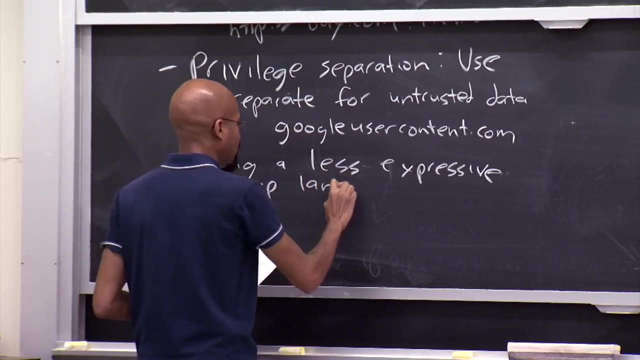 well, I'm going to do this. I'm going to do this. So you might think about sort of using a less expressive markup language. So what do I mean by that? So HTML and CSS and JavaScript are Turing complete. They allow you to do all kinds of fun things. 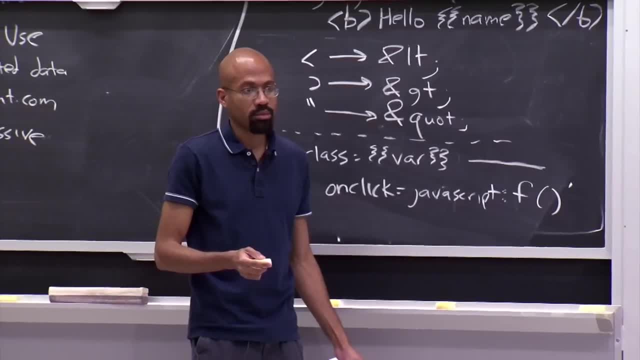 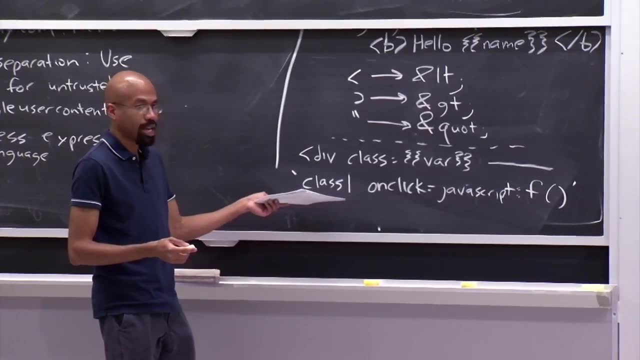 But yeah, Sorry about it. When does content sanitization not work? When does content sanitization- In many cases it doesn't work, Oh yeah, So, like in this case, for example, we're going to do this. For example, Django will probably not. 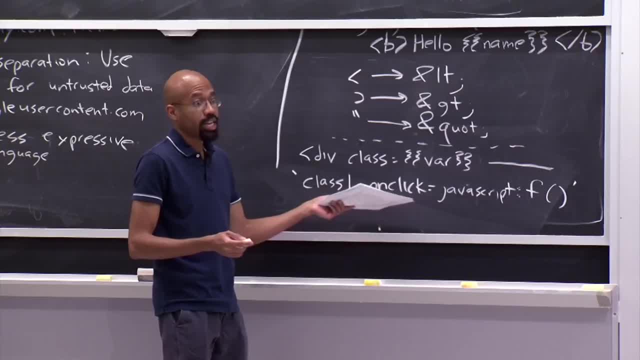 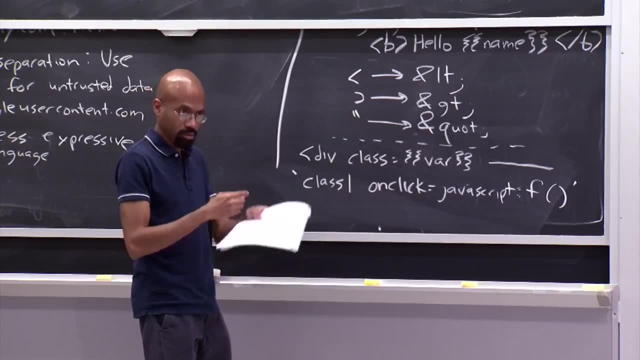 be able to statically determine. this is a bad thing, like in this particular case. Or like in the case where I inserted that malformed image tag. I basically said: like in that particular case, I would expect the class equals assignment to be in quotes. 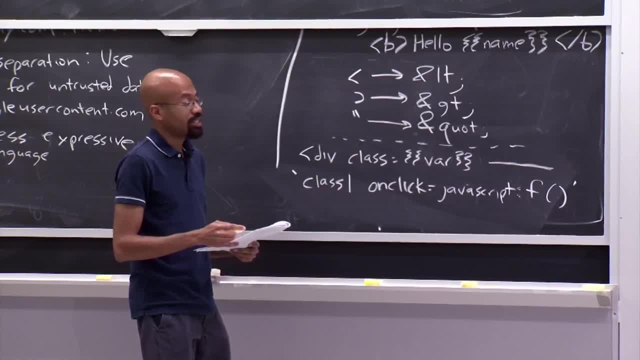 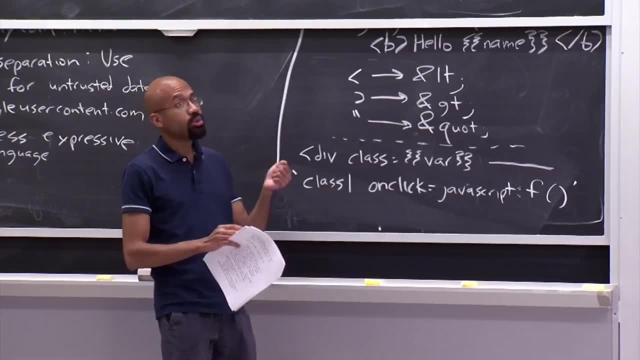 And then so that thing would not have any effect. So Django could enforce quotes on the class. Well see, there's a little bit of trickiness there, Because if we assumed that all pages were written. well, let me back up. 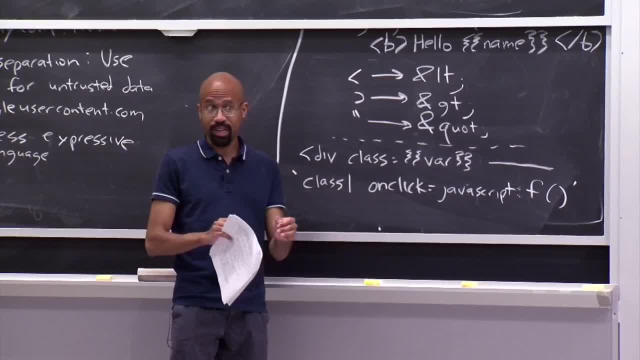 Let me back up a little bit. If we assumed the HTML grammar was well-specified and the CSS grammar was well-specified, and so on and so forth, then you could imagine a world in which perfect parsers would be able to sort of catch these problems. 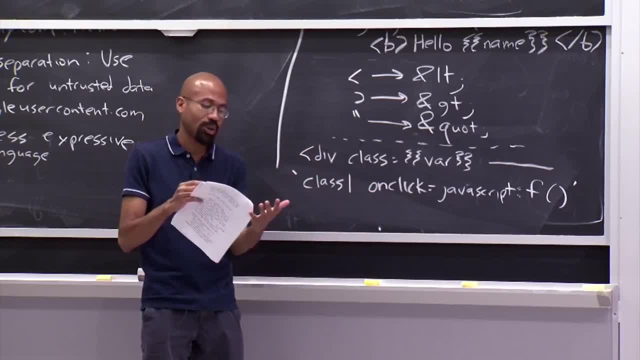 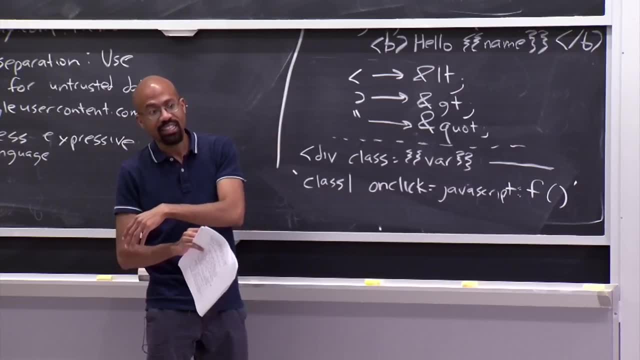 or somehow convert them to normal things, But in fact the HTML grammars and the CSS grammars are not well-specified, And then, on top of that, browsers don't implement specs, So it's like babushka dolls of terror. 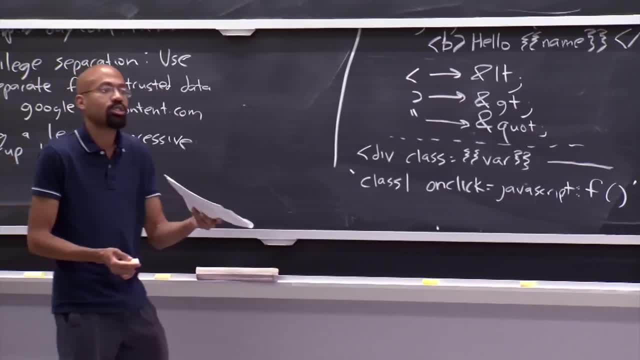 So I mean this in fact gets into sort of this notion here, right? Because I think essentially what you're saying is: well, look, if we have the grammar for something, that should mean something, right, And as it turns out, if you stick. 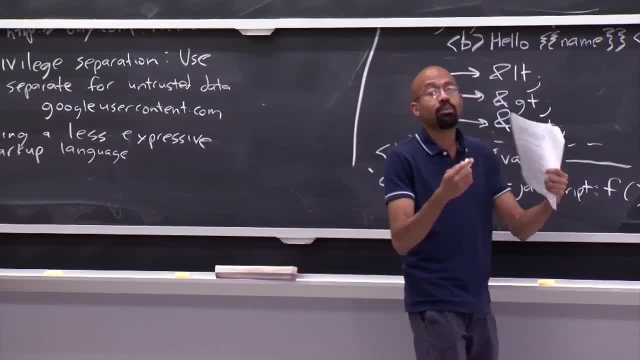 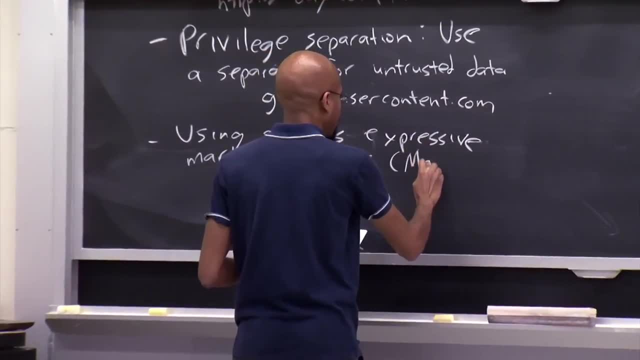 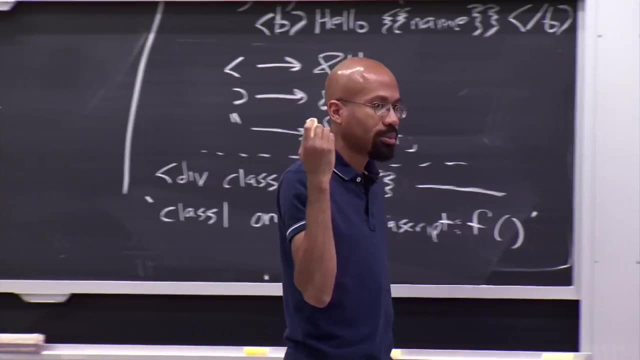 to a less expressive grammar, then it is actually much easier to do content sanitization. So there's actually some language It's called markdown instead of markup. lol, right, And so with markdown, the basic idea is that it's designed to be a language that allows 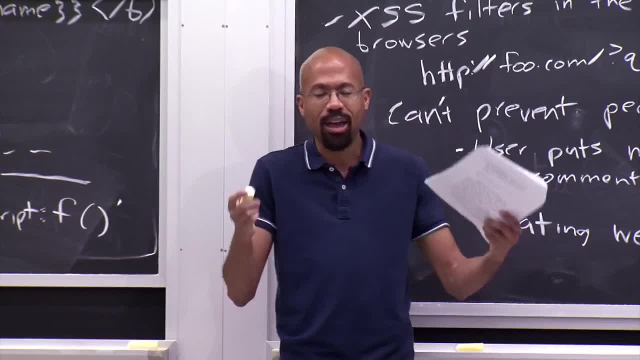 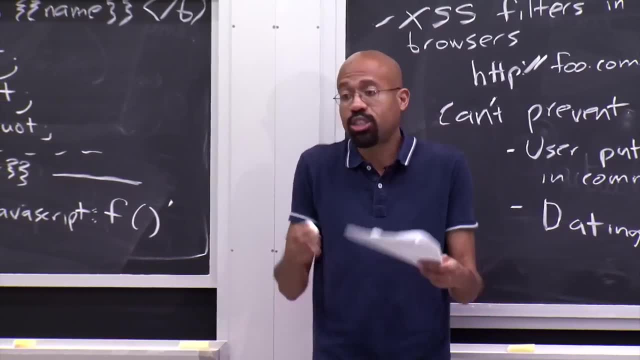 for example, users to submit comments, but it doesn't actually have things like the blank tag and applet support and stuff like that, And so in markdown it's actually much easier to do what you suggested, which seems like a reasonable thing at first glance. 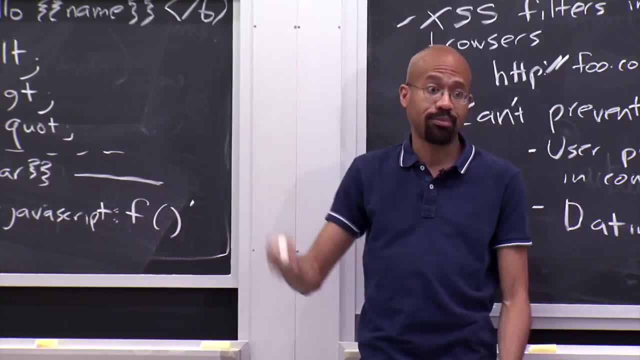 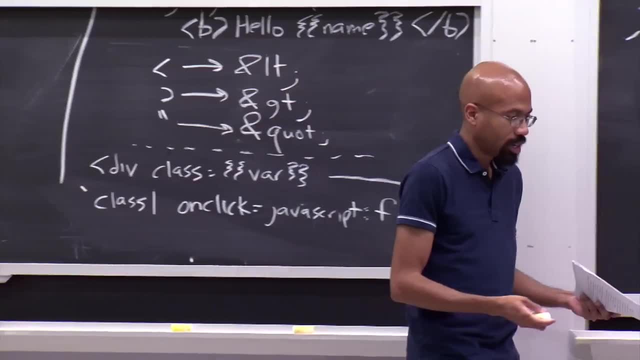 Just define the grammar unambiguously and then just enforce that grammar. So it's much easier to do sanitization in a simpler language than in the full-blown HTML, CSS and JavaScript And in a certain sense think about it. 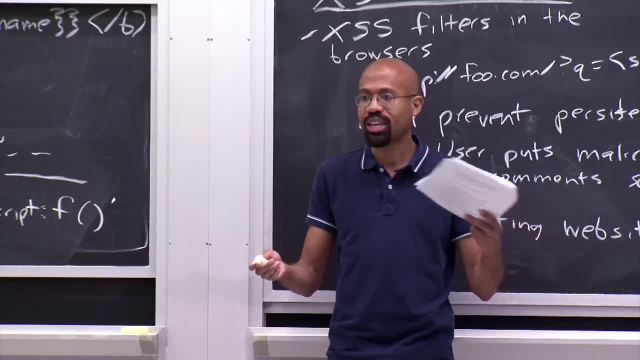 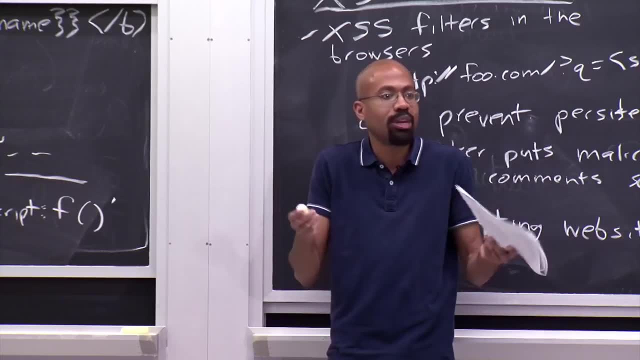 like the difference between understanding gnarly C code versus gnarly Python code. There's actually a big difference in trying to understand that much more expressive language, because it can do many more things. By constraining expressivity you oftentimes improve security. 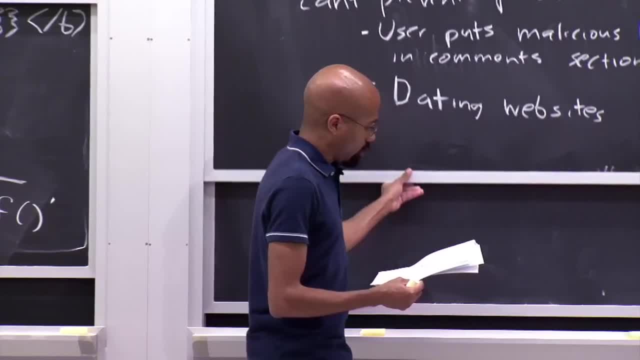 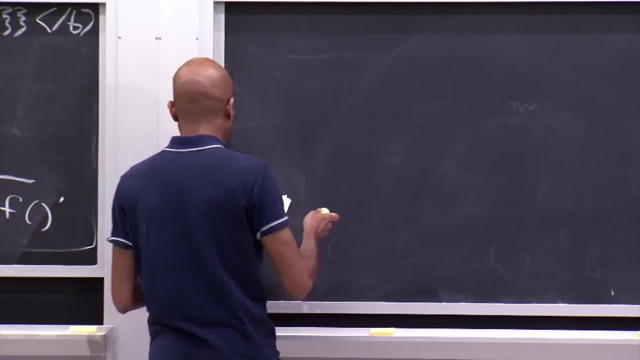 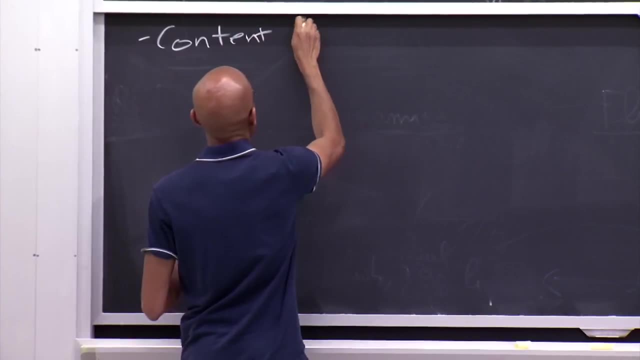 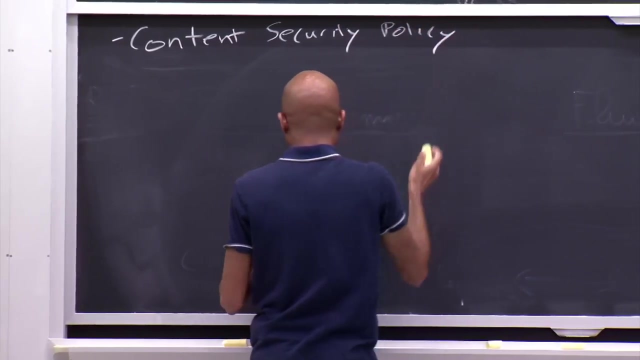 Does that all make sense? So another thing that you can imagine doing to protect against cross-site scripting attacks is to use something called CSP- CSP, Content Security Policy- And so the idea behind CSP is that it's going to allow a web server to up. 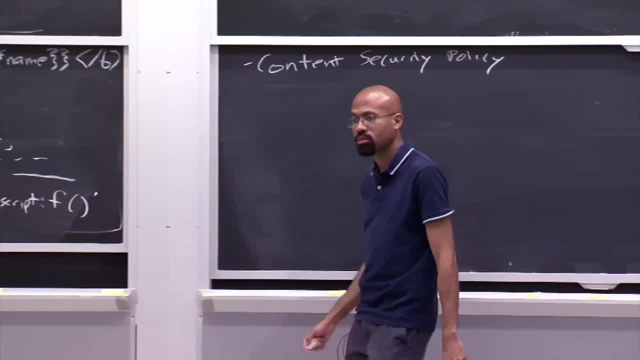 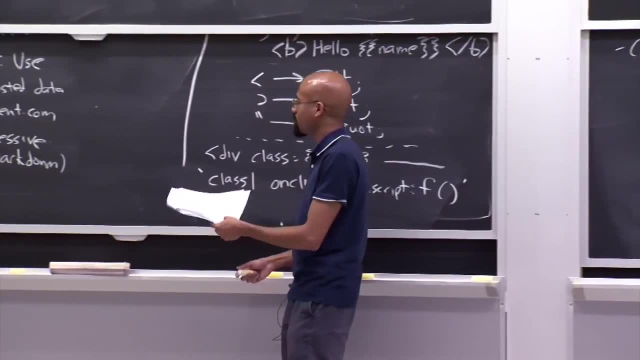 I'm just curious about this markdown thing. So all browsers know how to parse? No, no, no. So what happens with a lot of these types of languages is that you, essentially, you can convert them, You can compile them, You can compile them down to HTML. 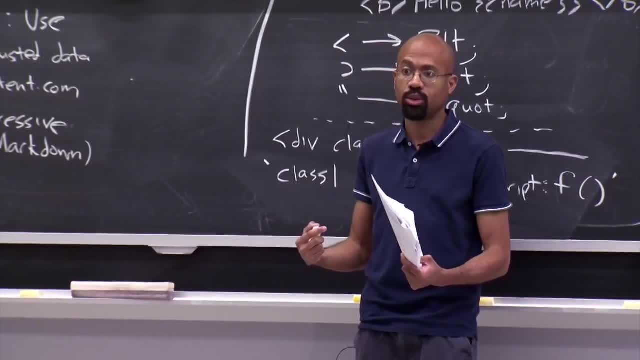 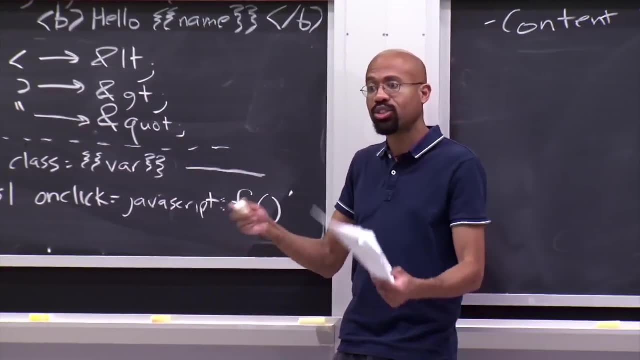 But they're not natively understood by the browser typically. So in other words, you've got some comment submission system. It internally expresses stuff in markdown, But then, before it can be rendered to the page, it essentially goes to the markdown compiler. 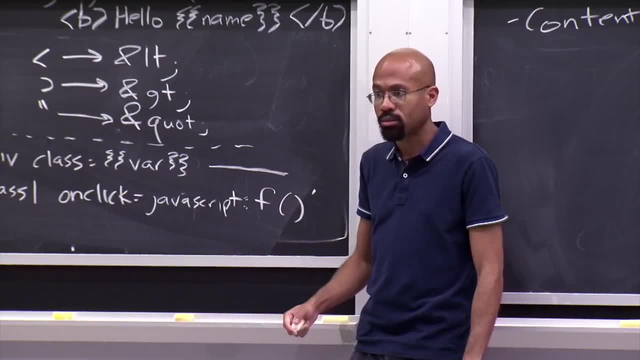 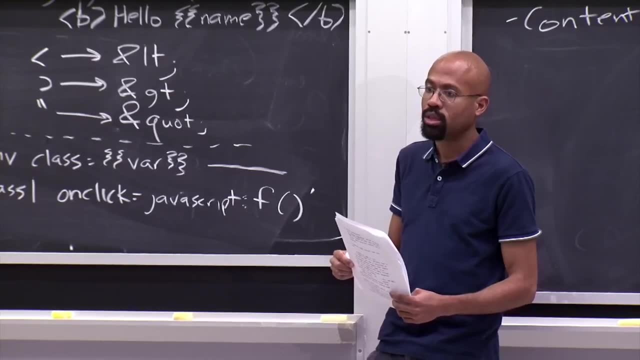 The markdown compiler then translates it to HTML. Thanks, Just as a useful point. markdown might not be the best way to use markdown analysis, So markdown might not be the best way to use markdown analysis. So markdown does allow inline HTML. As far as I know, there's a way to disable that in the compiler. 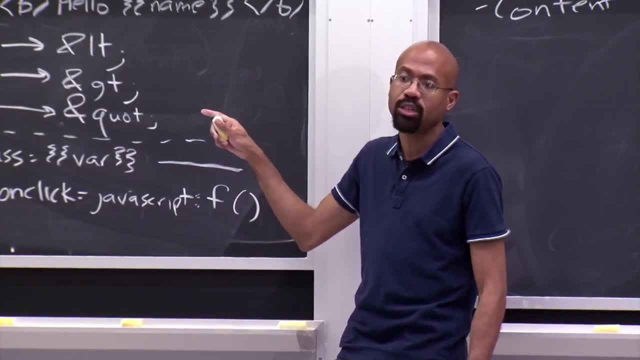 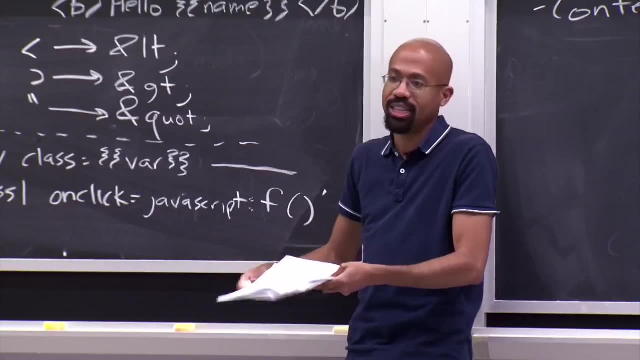 I could be wrong about that, But I believe that there's a flag you can pass to get rid of it. But you're correct that if you use a constrained language but then you embed an unconstrained language, then that I mean the terrorist of one. 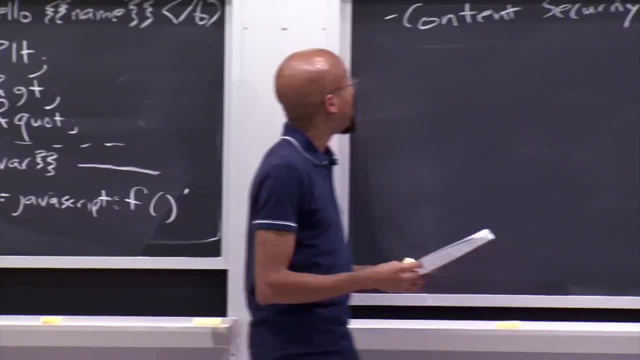 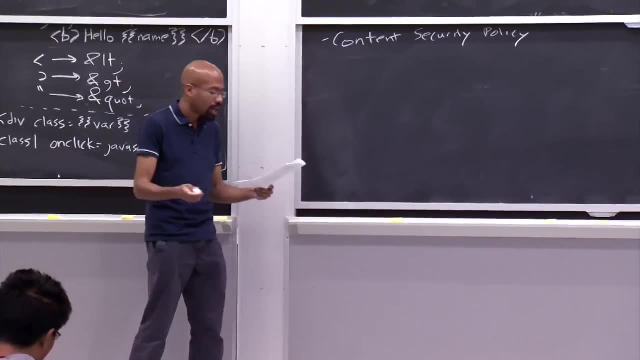 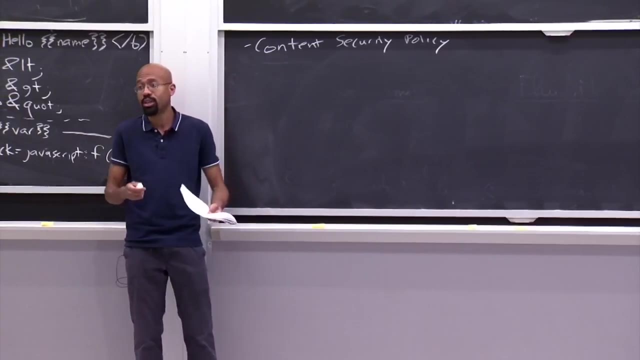 So you're right about that. OK, so another thing you can do to improve security is this thing called content security policy. So, like I was saying, what this allows the server to do is to tell a web browser what types of content can be loaded in the page it's sending back. 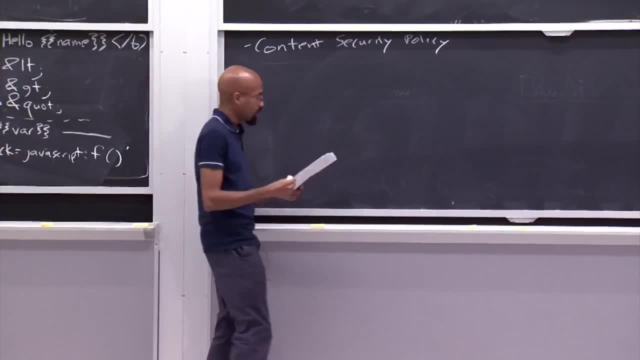 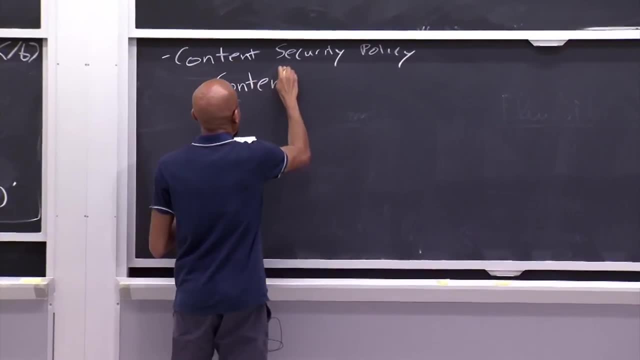 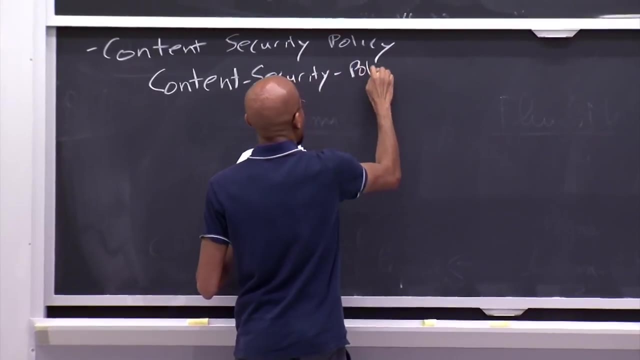 and also where that content should come from. So, for example, in an HTTP response, the server might be able to say something like this: It include the content security policy header, and then it might say something like the default source. OK. 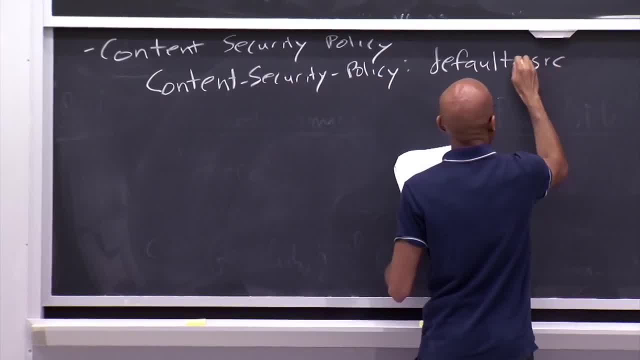 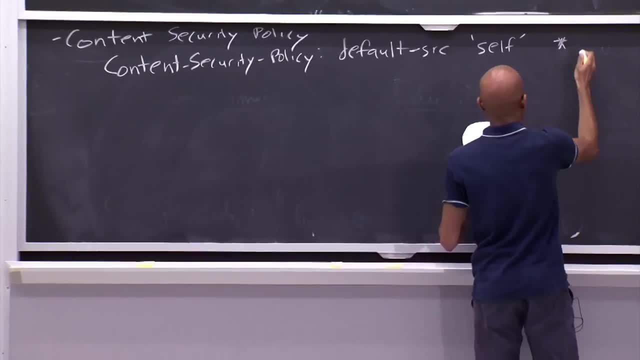 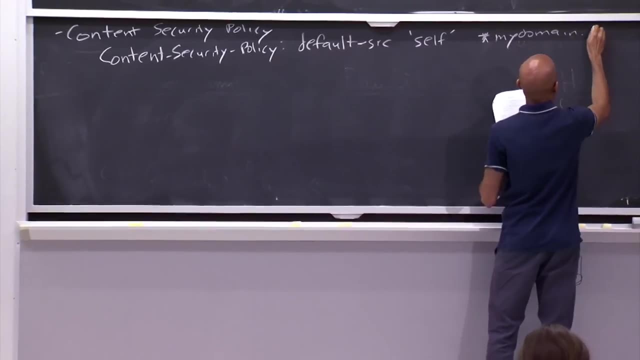 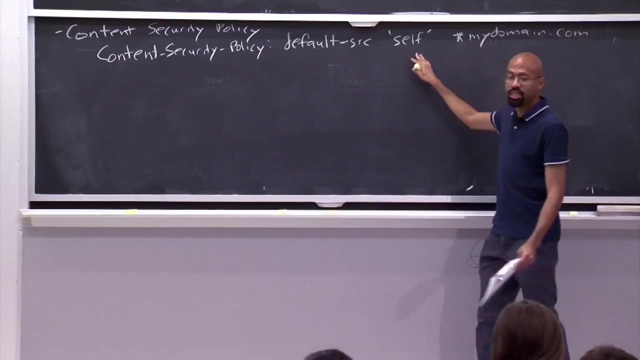 That's cool. That's cool. Source is going to equal self and it will also accept things from asterisk, my domain dot com. So what does this mean? So, essentially, the server is saying the content from this site should only come from whatever it is that the domain is. 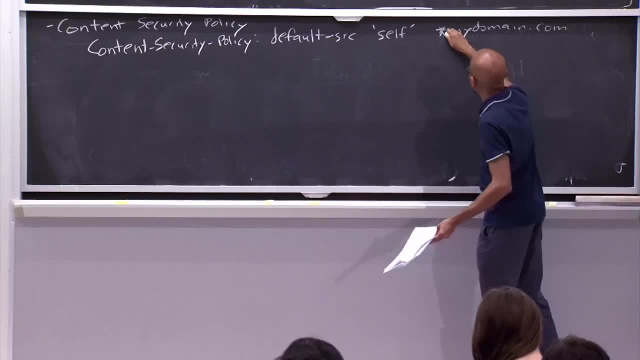 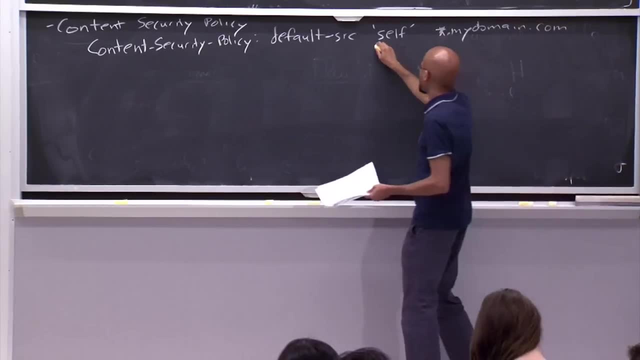 for the particular page And then any other subdomain from my domain dot com. So what that means basically is that let's say, if self was bound to foo dot com, let's say that's the origin of the server, that's sending. 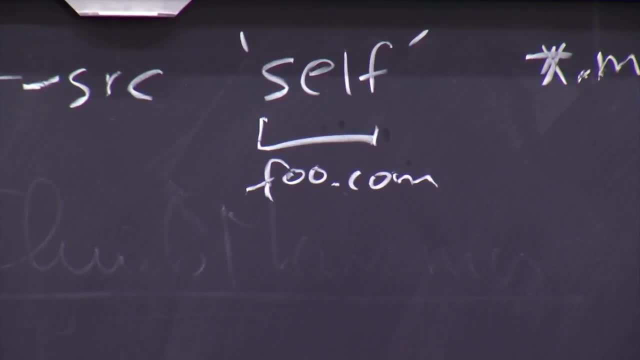 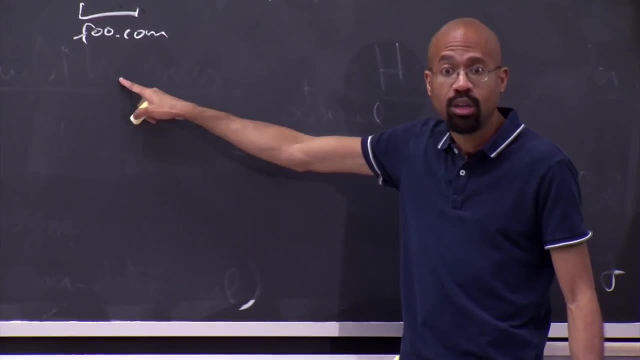 this thing back to the browser. So if somehow there is a cross site scripting attack and the page tries to generate a reference to, let's say, bar dot com, the browser would say, OK, bar dot com is not self. Bar dot com is also not in this sort of set of domains. 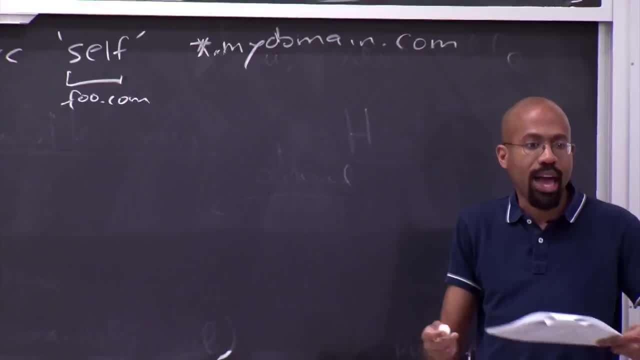 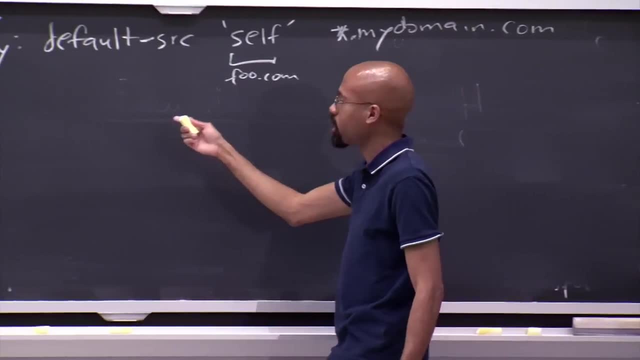 So therefore the browser can just say: I will not allow that request to go forward. So this is actually a pretty powerful mechanism. You can actually specify more fine grained controls here. You can say: my images should come from here, my script should come from here, so on and so forth. 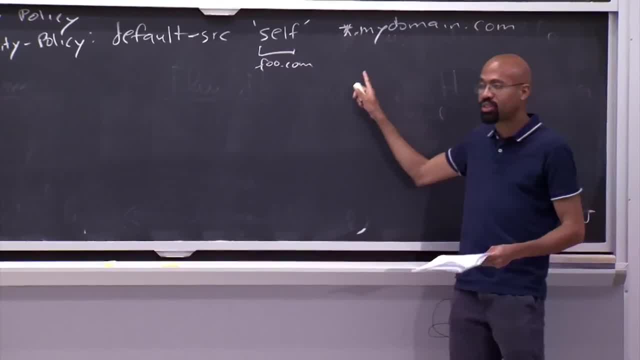 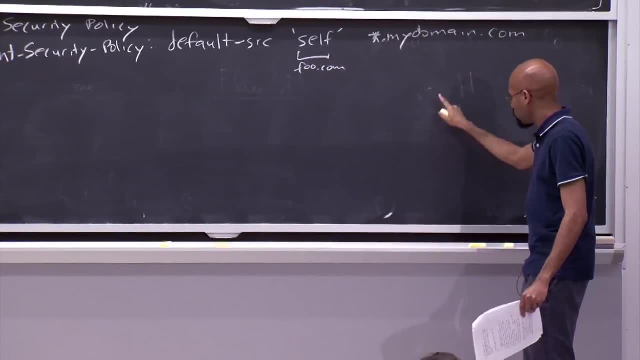 This is actually pretty nice, And one nice thing about this, too, is that it actually prevents inline JavaScript. So you can't have script tag and then some literal JavaScript, then closed script tag. Everything has to come from a script tag with a source. 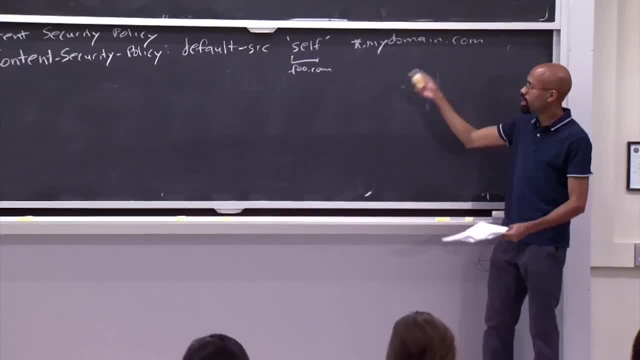 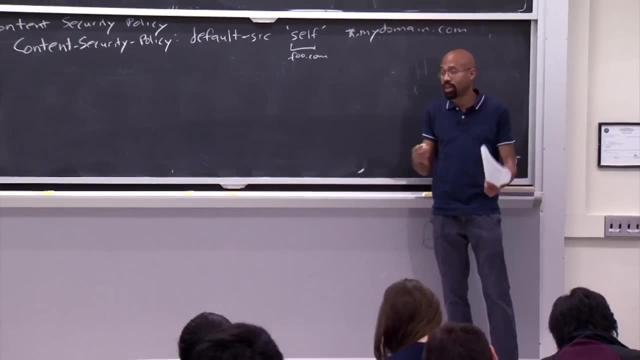 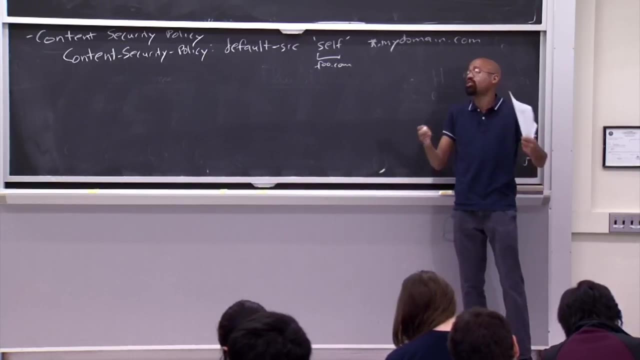 So it can be validated through this, And also content security policy prevents these dangerous statements like eval. So eval basically allows a web page to dynamically generate JavaScript code, And so if the CSP header is specified, the browser does not execute evals. 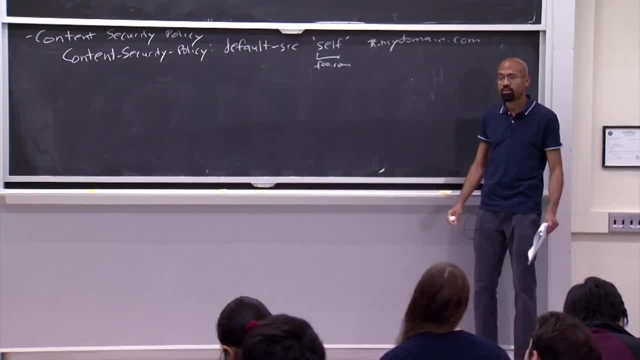 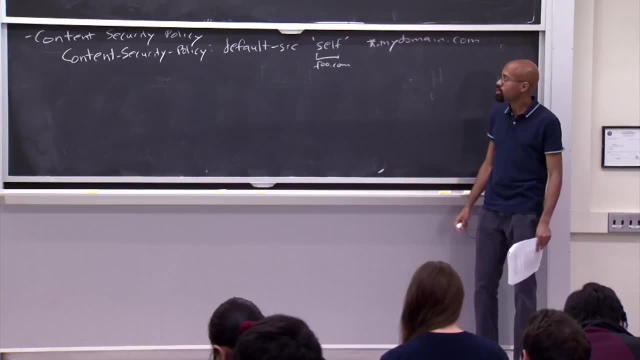 So does that all make sense? So it seems like kind of an ad hoc set of things. Is that like a complete set of things that you're talking about? It's not a complete set of things, No, so there's a whole list of resources. 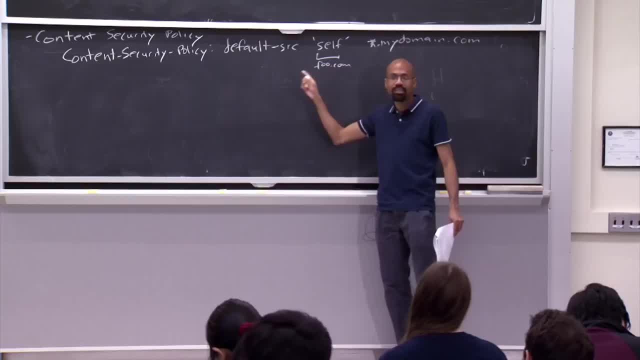 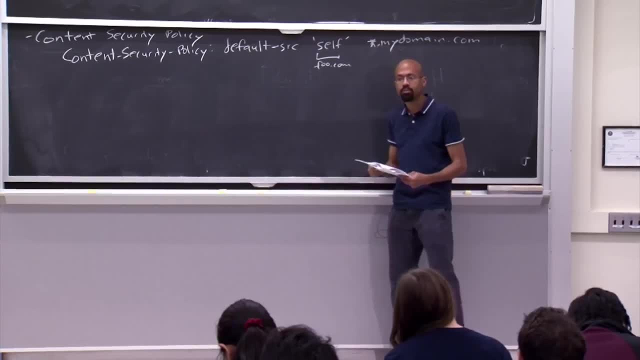 that it actually protects. So this is sort of like the most blanket type protection you could get, But, like I said, it actually allows you to specify, I think, where CSS can come from, like a bunch of different things. But I was like preventing evals. 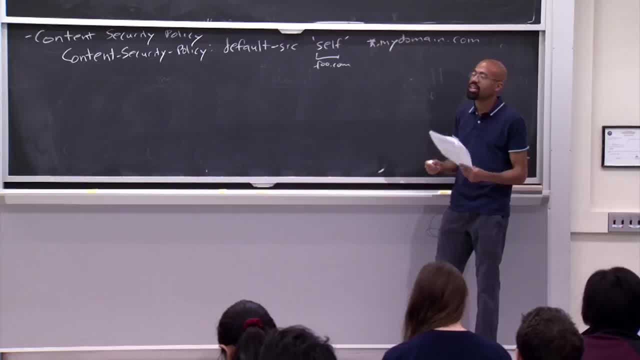 that seems like some sort of like. are there other things, like random things like that? So, yeah, there are. So there's always this question of completeness, Right? So, for example, eval is not the only way JavaScript can actually, you know, do something. It's the only way to generate code dynamically. There's the function constructor, for example. There's certain ways you can call set time out, You pass in a string and it can evaluate code that way. So I believe that CSP actually shuts down those vectors. 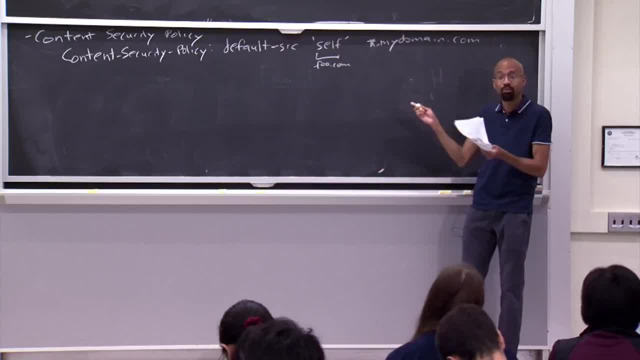 as well. But if you're asking, you know, is this sort of provably complete in terms of what it isolates? No, and I don't think that any of these solutions are provably complete. One really interesting thing about CSP is the fact that you can sort of disallow all inline JavaScript. 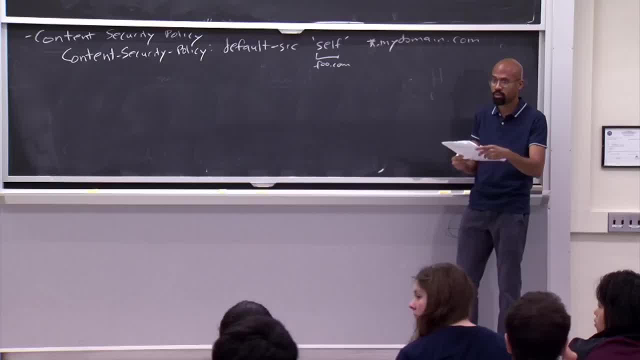 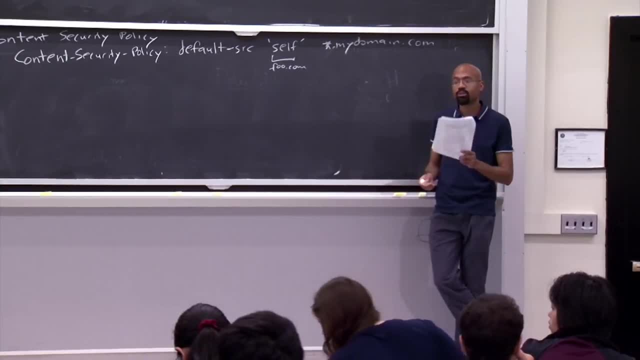 from the page. That's right. Which help can you of these kind of things? Yeah, that, yeah, I mean that helps. It's also going to outlaw eval, but it prevents an attacker from, So that helps with some things. 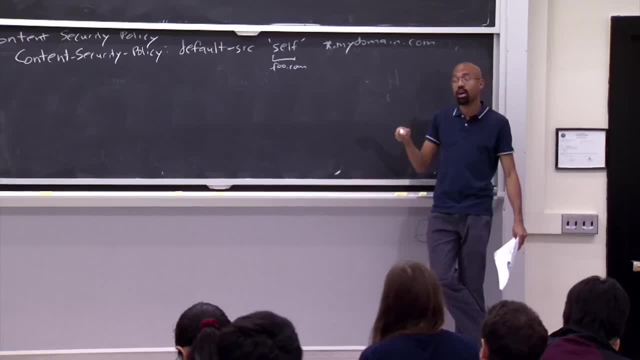 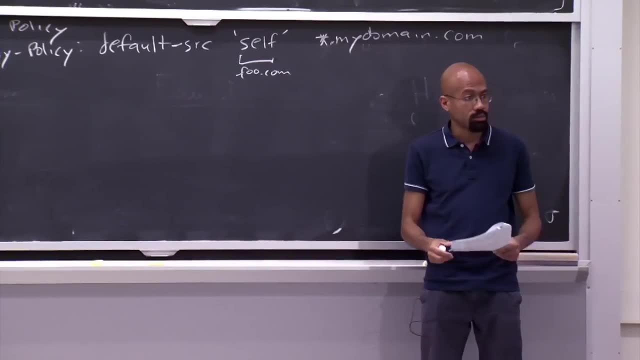 but you know that still would allow, like a fetch script, to use eval, right. So that's why it's important to try to get rid of all of those dynamically, all those interfaces for dynamic code generation If you have a script tag with a source. 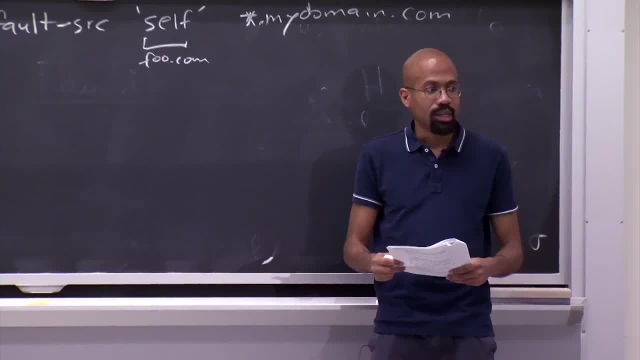 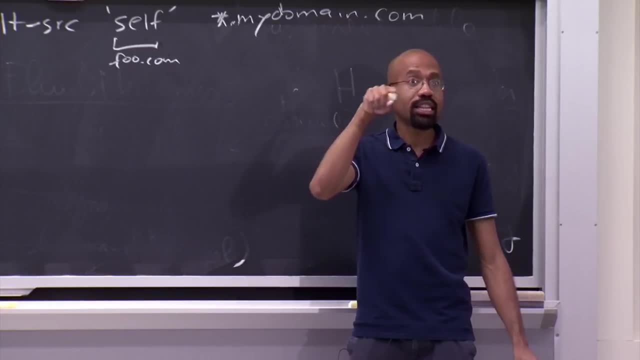 but then also inline code is there, like standardized invoker that all browsers do with. Yeah, So what should happen? So what should happen is that the inline code should be ignored, right? So the browser should always get the code from the source attribute. 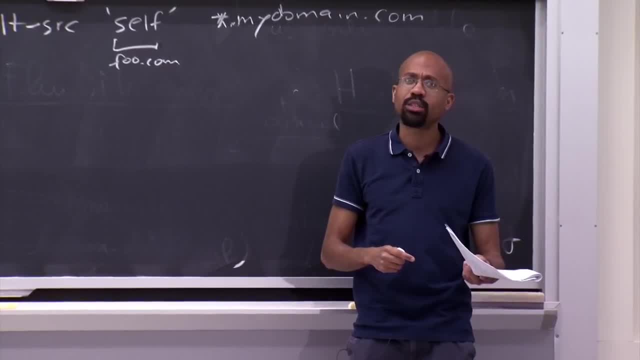 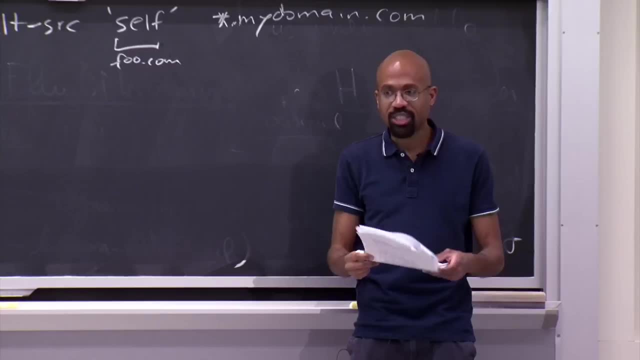 I actually don't know if all browsers do that. I've actually personally experienced browsers exhibit different behavior. in that This was a couple years ago, so I'm not sure, And so yeah, so one thing to keep in mind about sort of doing. 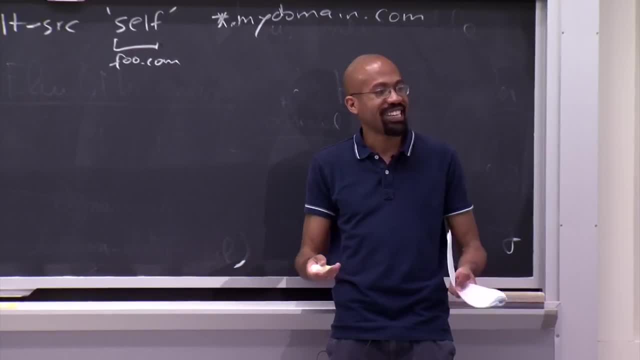 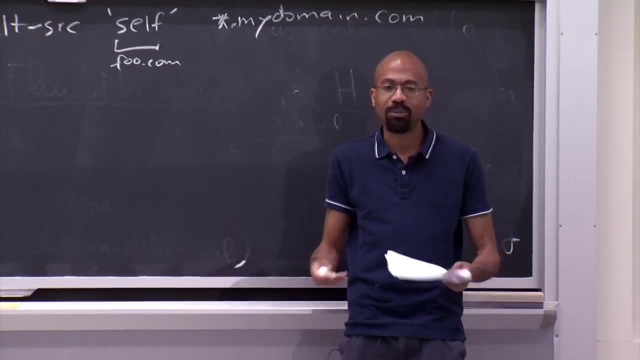 work in the web security is that in a sense it's almost like a natural science, So it's like people actually propose theories about how browsers work and then you go see and you do that right, And so that can be a little bit disappointing. 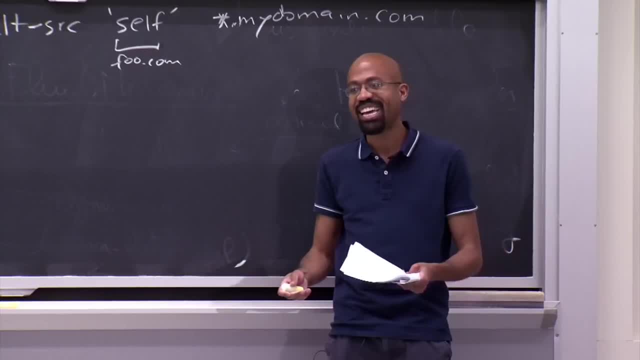 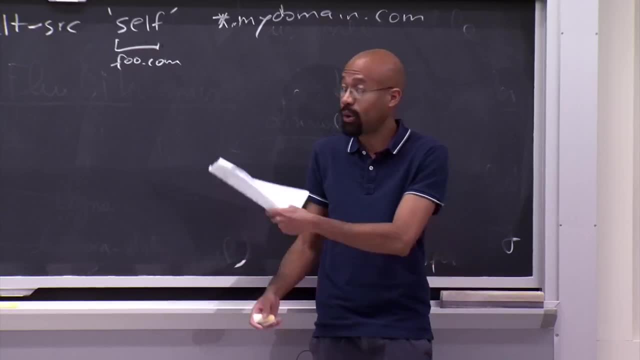 because we're taught like yay, algorithms and proofs and stuff like that. But these browsers are so ill-behaved that a lot of times the answer is like maybe or maybe not, And then you go out and you go see. 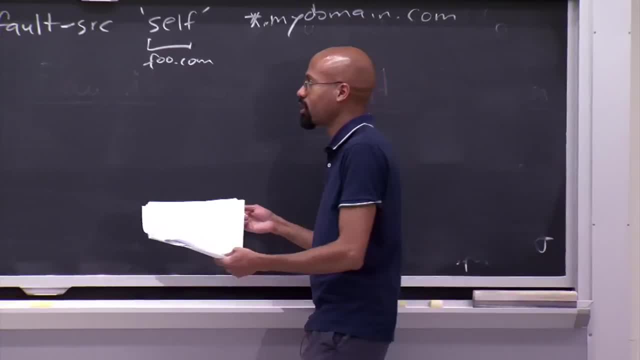 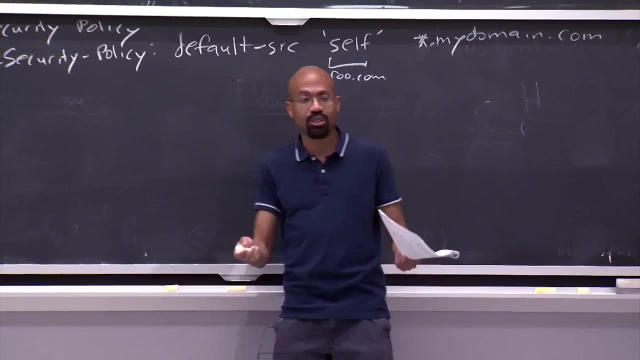 And so, as we'll see, as they keep on adding features. it gets back to your question about: are these things provably complete? I think web vendors have punted on this notion of creating a browser that is provably foo. Basically, what they try to do is just: 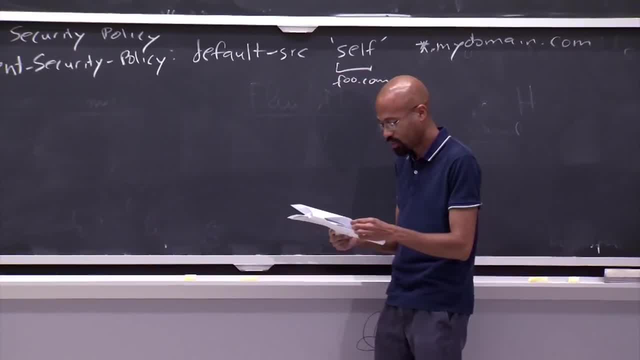 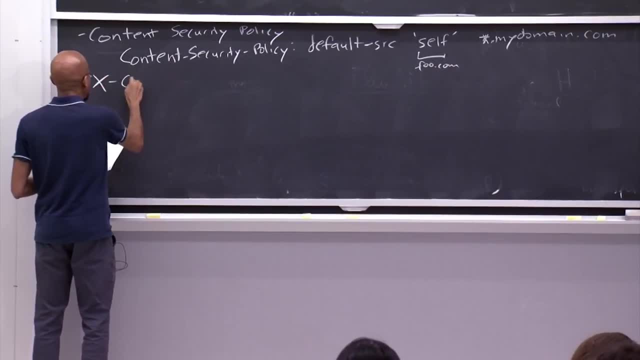 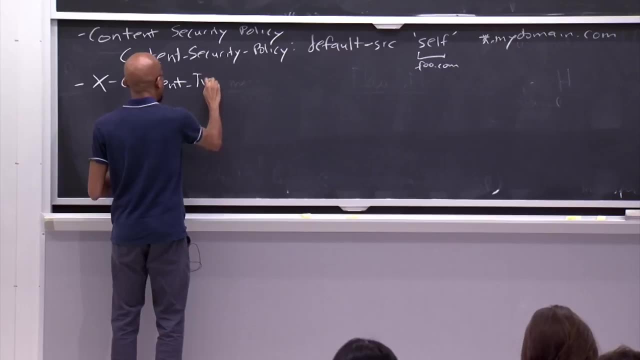 try to keep one step ahead of the attackers, And we'll see some examples of that further in the lecture. So yeah, so CSP is actually pretty cool. Another thing that's useful is that the server can set this HTTP header called X, content type options. 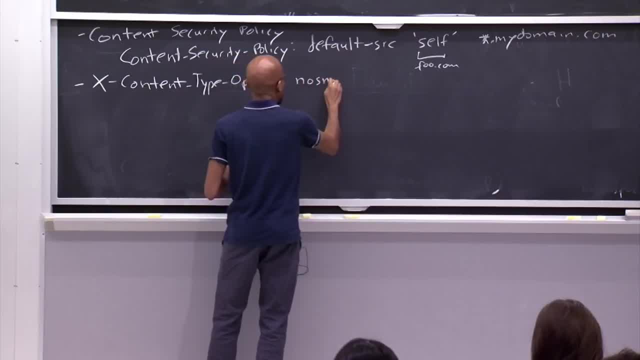 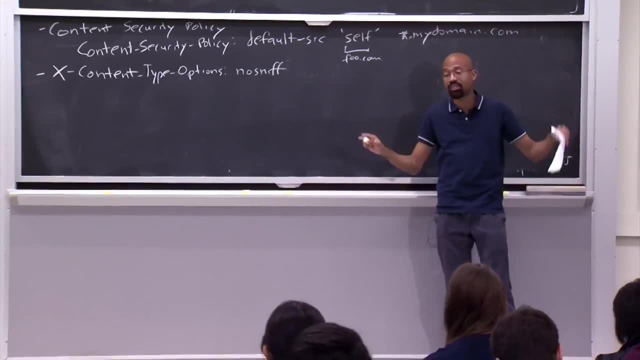 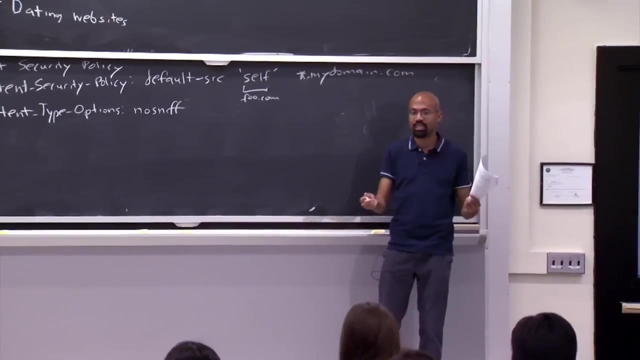 and then can say no sniff. And so what this means is that this prevents the browser from doing some of those quote unquote helpful optimizations, like we discussed last lecture, where it will say: aha, there's a mismatch between the file extension and the actual bytes that I've sniffed in the content. 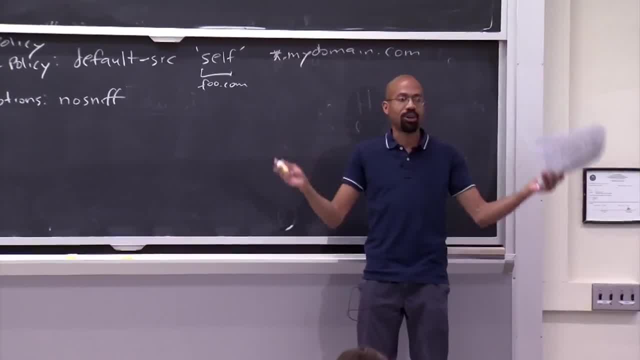 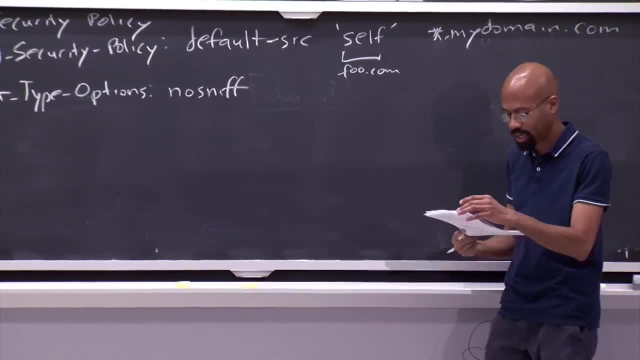 So let me somehow massage this content to some different thing. And then all of a sudden you've given the barbarians the keys to the kingdom, So you can set this header and basically say: browser, do not do that. And so that can be useful in mitigating some types. 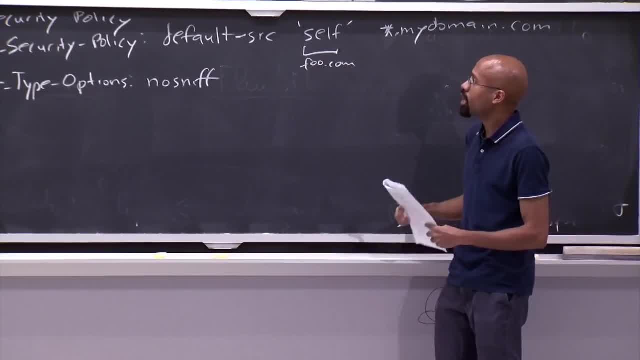 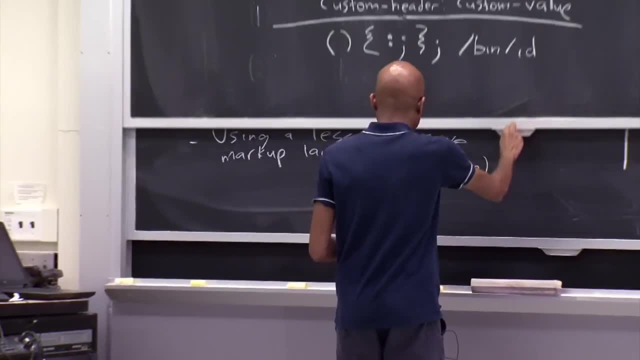 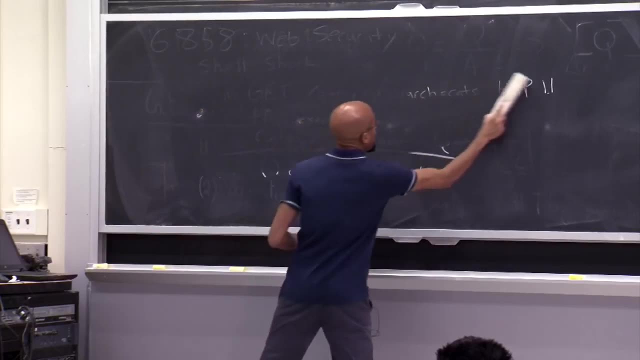 of attacks as well. All right, so that's kind of a quick survey of some of these cross-site scripts. All right, So, scripting vulnerabilities. So now let's look at another popular vector for attacks, And that vector is going to be SQL. 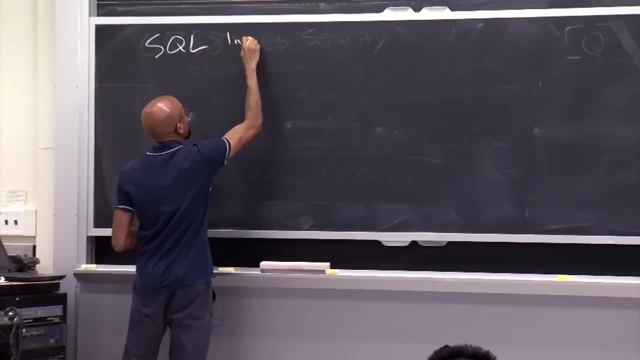 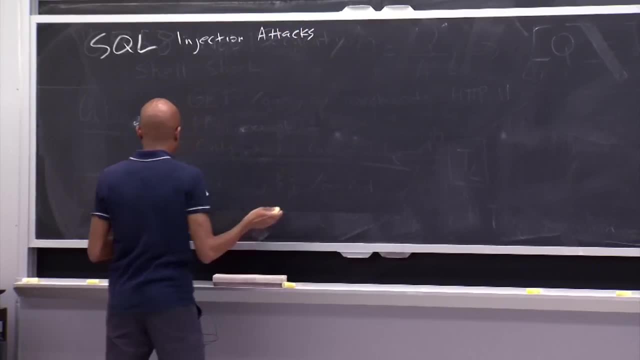 And so you've probably heard of these SQL injection attacks, And so what these attacks do is they take advantage of the fact that on the back end for a lot of websites there's some type of database, And so to dynamically construct the page that's. 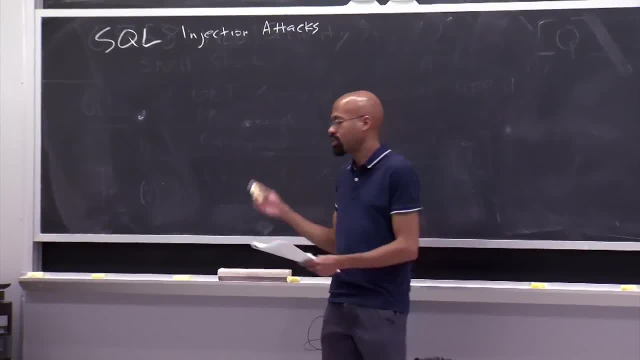 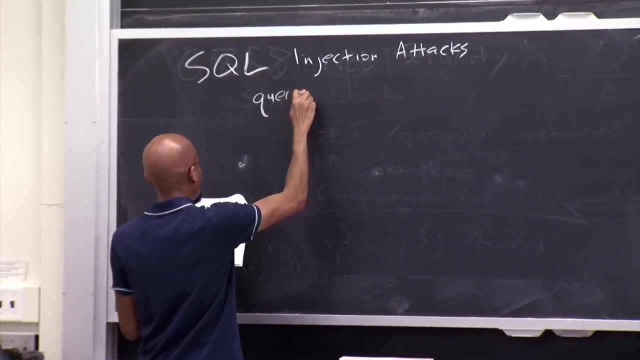 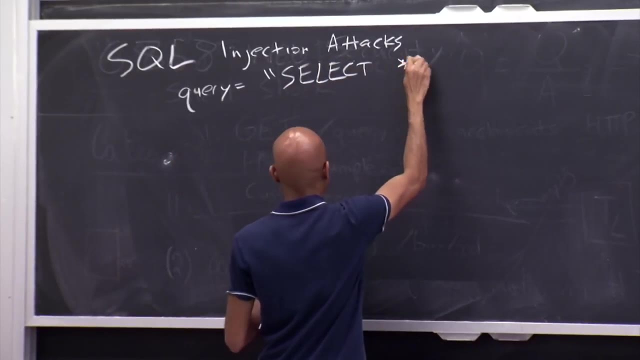 shown to the user. there have to be some database queries that are issued to that back end server. So imagine that you had some query that looked like this. So you do a select asterisk, So give me all the values from this query, from some particular table. 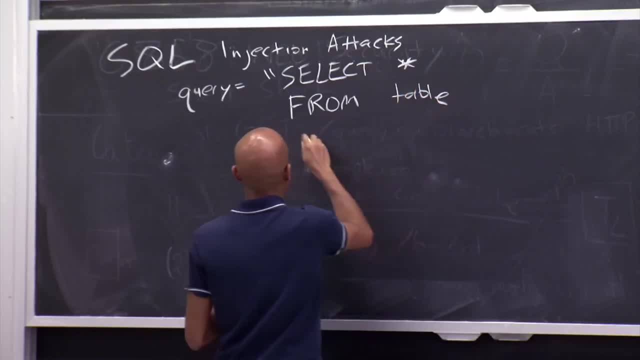 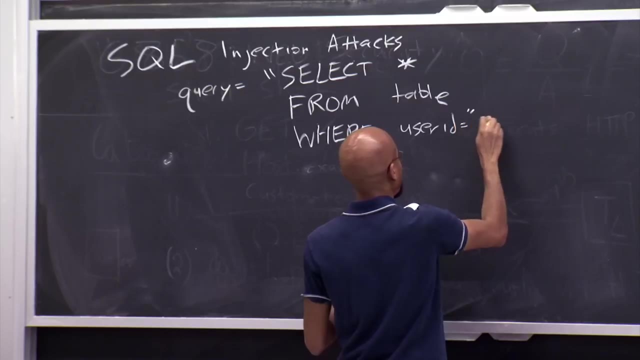 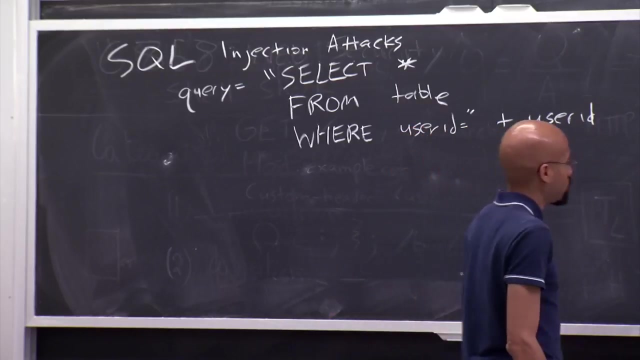 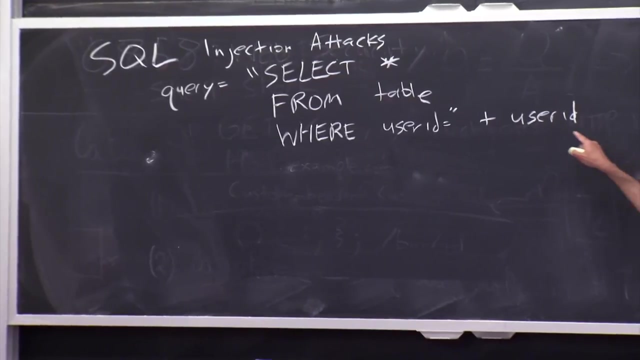 Where The user ID field is equal to something that is specified over the web from some potentially untrusted source. So at this point I think we all know how this story ends. It ends very badly. There are no survivors. So basically, if this comes from someone untrusted, 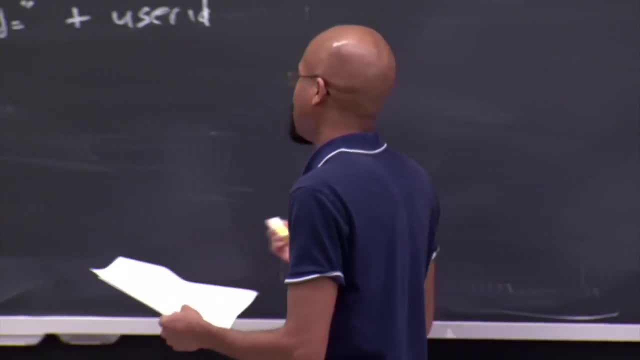 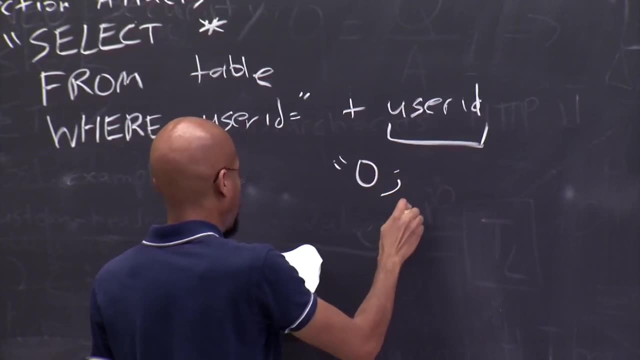 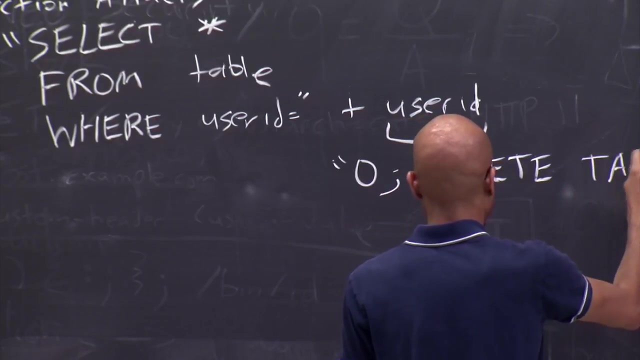 then you can do all kinds of chicaner stuff here. So one thing you could do is, if you want to be a jerk, you could just set this to the string 0, and then something like delete table. So what happens here? 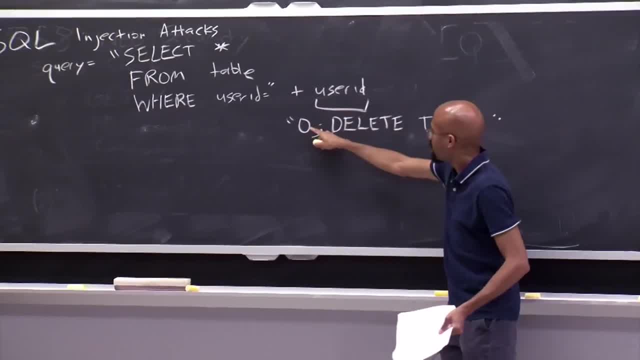 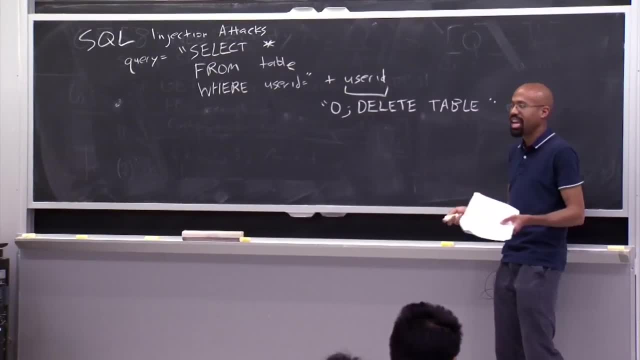 So basically, the database server is going to say: OK, I'll set the user ID to 0, semicolon. Here's the start of a new command: delete table. OK, cheers, There goes your table Right and you're done. 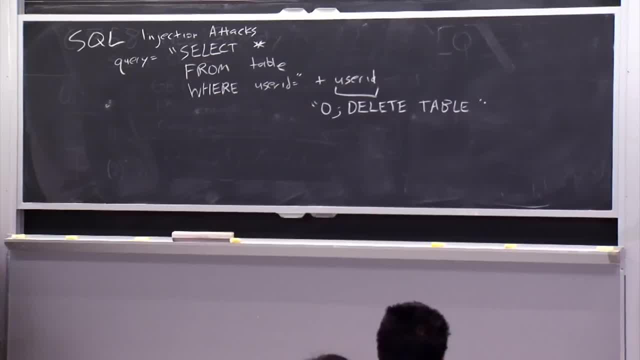 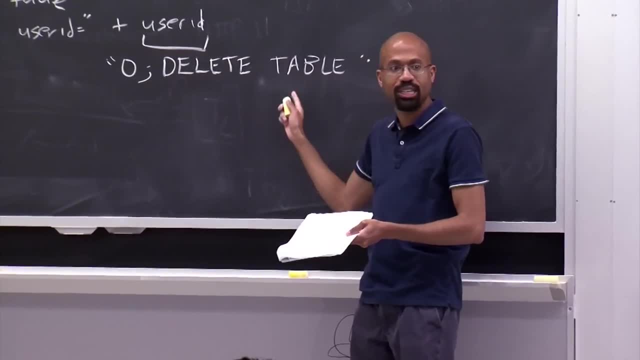 And in fact there was a viral image that went around a couple years ago. It's unclear if it's true, like many of these viral images, But it was that people in Germany had license plates that actually said 0, semicolon delete table. 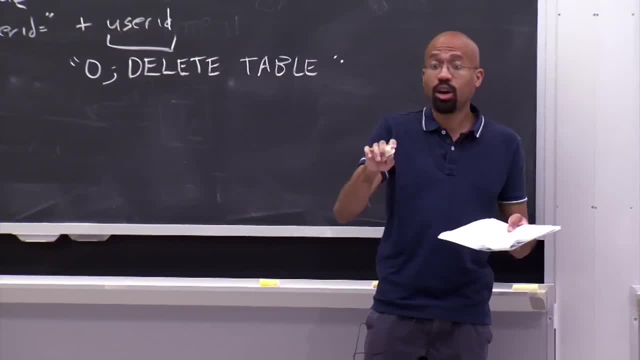 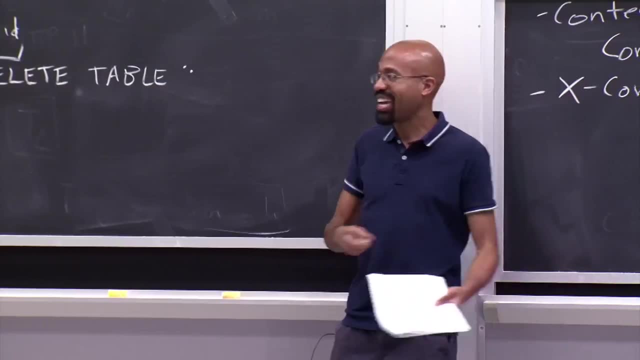 Because the idea is that the security cameras, they would use OCR, optical character recognition- to figure out what your license plate was and then put it in a SQL database. And so there are images floating around these Volkswagens. People would have this as their license plate. 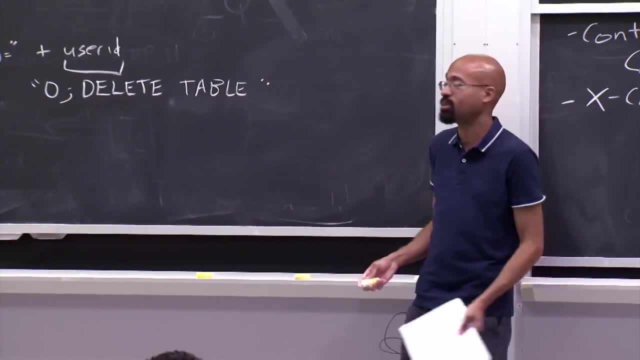 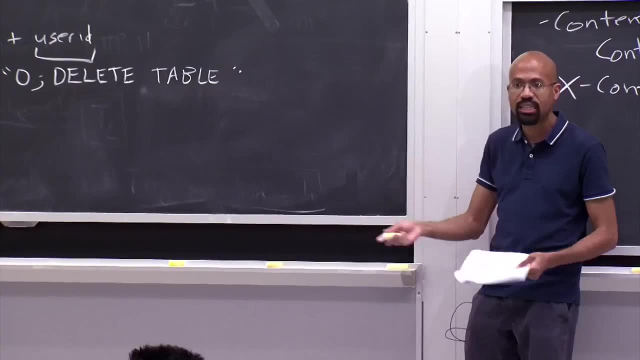 People sometimes I don't know if that works. It's funny, so I like to believe that it's true. Who knows? But I mean you get the basic idea behind that. So, once again, the idea is: you want to be sure to sanitize this content, that you're. 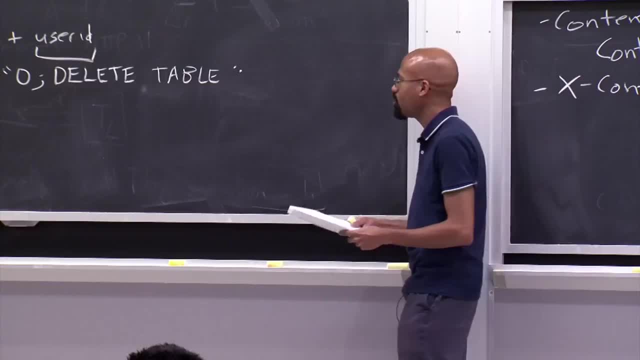 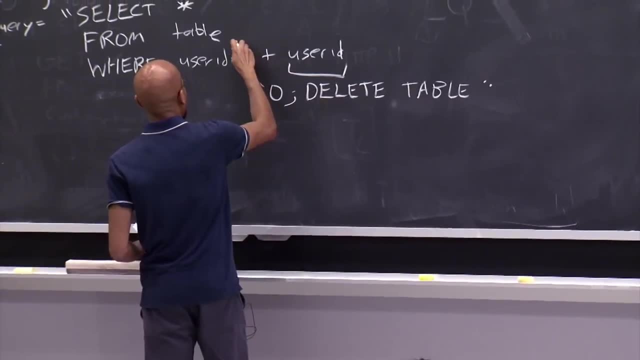 getting from these untrusted sources, And so note that there may be some sort of straightforward things that don't quite work. So you might think, OK, well then, why can't I just put another quote here and then put another quote here? 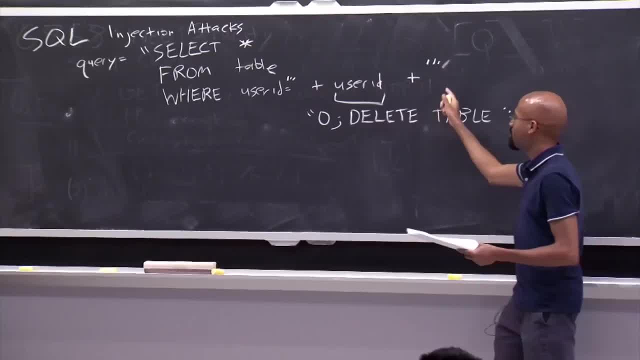 such that whatever it is that the attacker submits there's going to be- It's going to be a good thing- It's going to be enclosed in a string. So this doesn't work, because then the attacker can always just put a quote inside his or her attack. 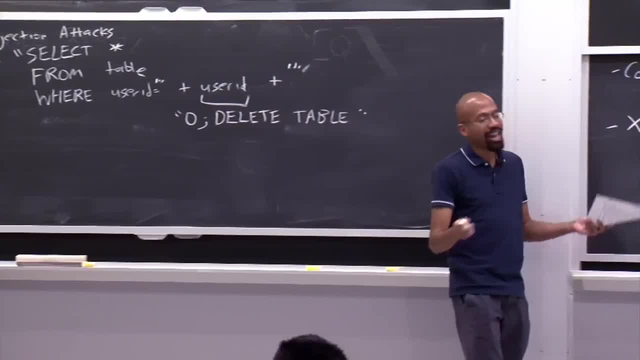 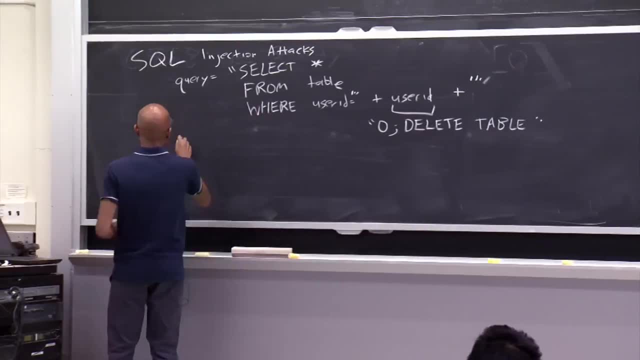 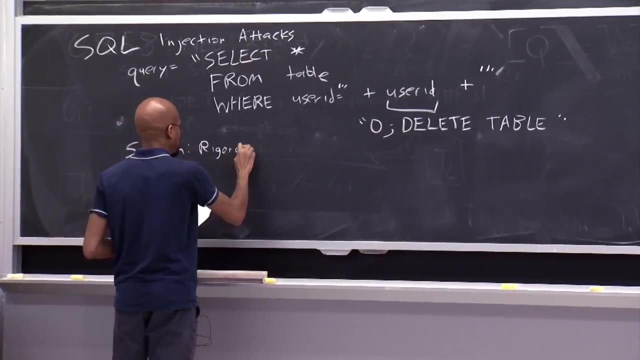 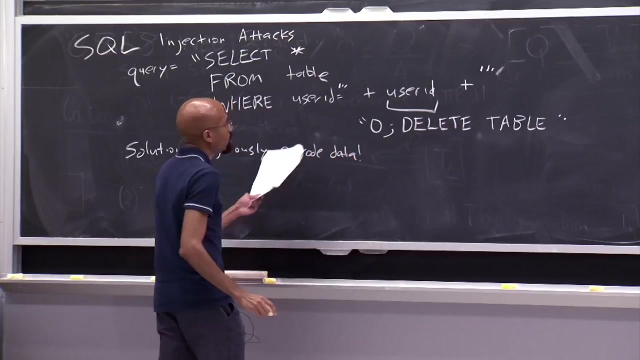 string. So a lot of times, these sort of half-hearted hacks don't really get you the security you think they might. So the solution here is that you need to rigorously encode your data, And once again, that just means that when you get information from an untrusted source, 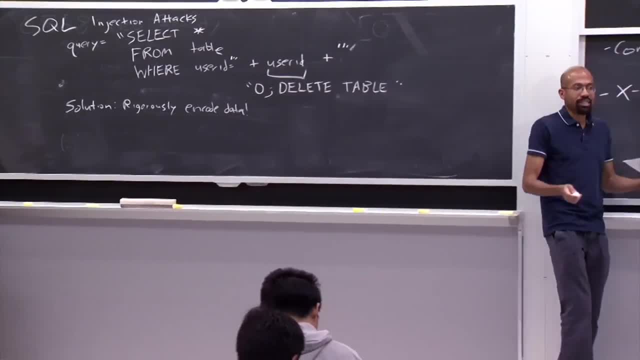 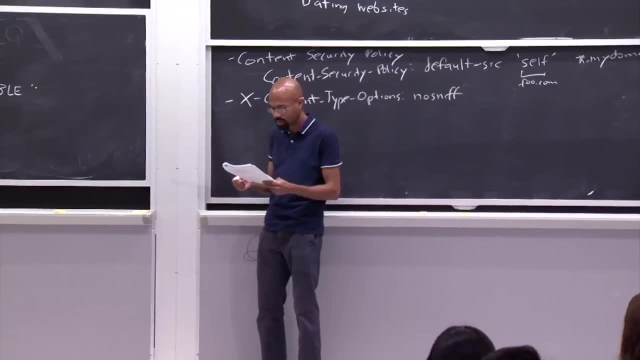 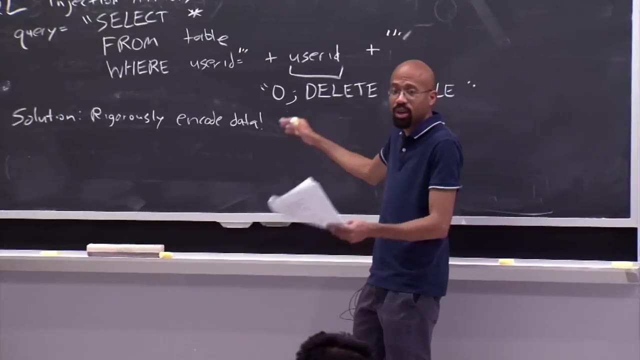 don't just stick it in the system as it is. Make sure that, for example, it can't actually escape from whatever sandbox or whatnot you think you're actually putting into. So, for example, you want to put in escape functions that would prevent, maybe, the semicolon operator. 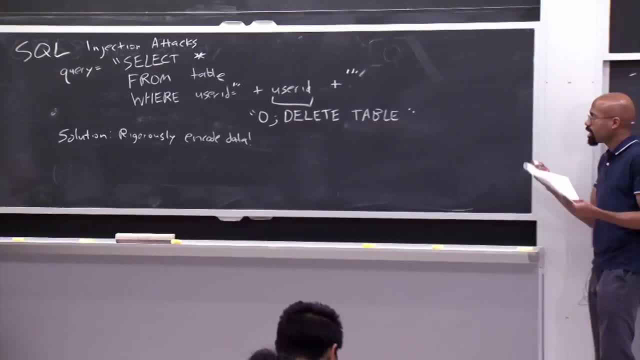 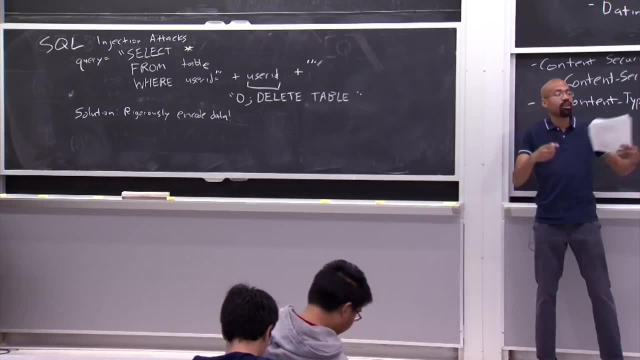 from showing up in raw form or things like this, And so a lot of these web frameworks like Django actually have built-in libraries And you can actually put in a lot of these things. They have built-in libraries to do things like character escaping for SQL queries. 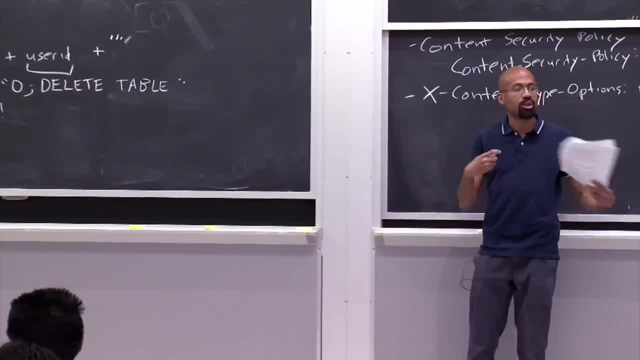 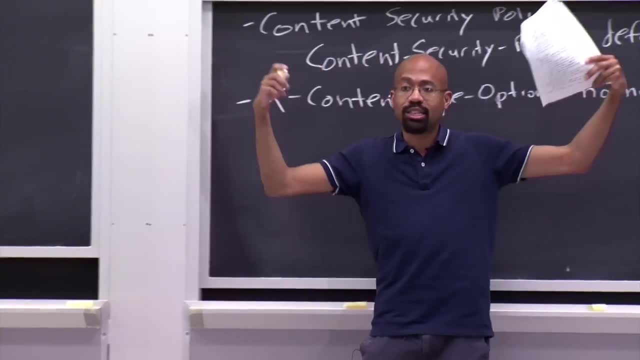 to try to prevent some of this stuff, And a lot of these frameworks actually encourage developers not to ever directly interface with the database. So Django itself will provide some higher-level interface which does standardization for you and takes care of some of these icky corner cases. 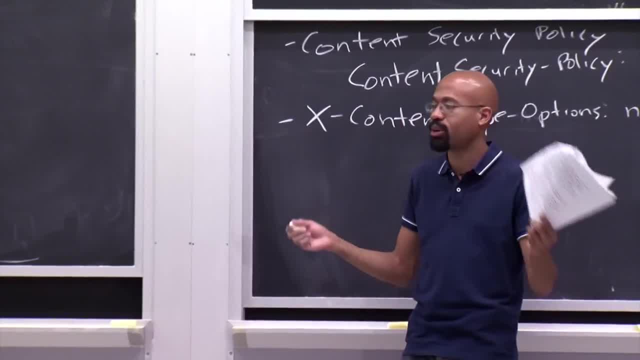 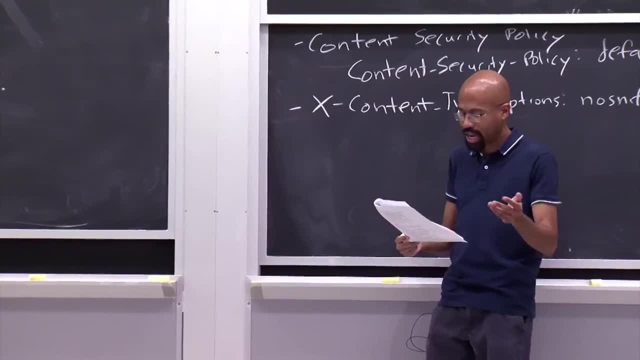 But performance, performance, performance. Sometimes people think that these web frameworks are too slow, So you will still see on the back end a lot of time. people will still make these raw SQL queries and that can lead to problems, So you can also imagine that there. 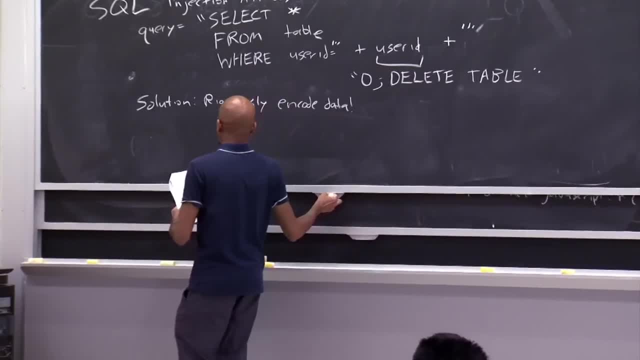 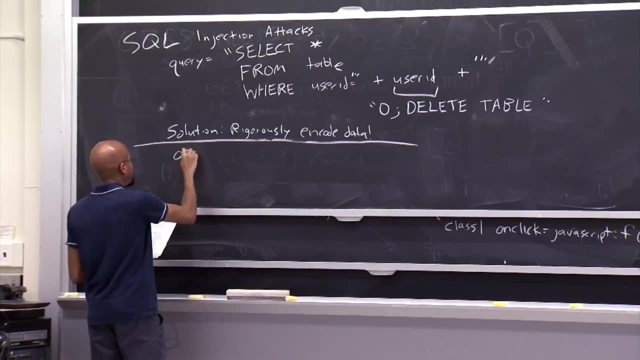 are problems if the web server takes in path names from untrusted entities. So imagine that somewhere in your server you do something like this. You have an open call and then you say that you're going to read from the www directory, You're going to read from the images subdirectory in there. 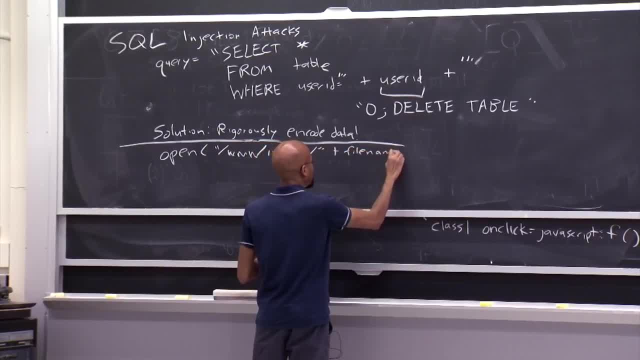 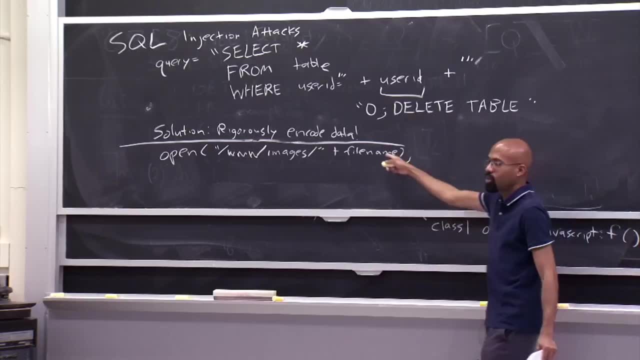 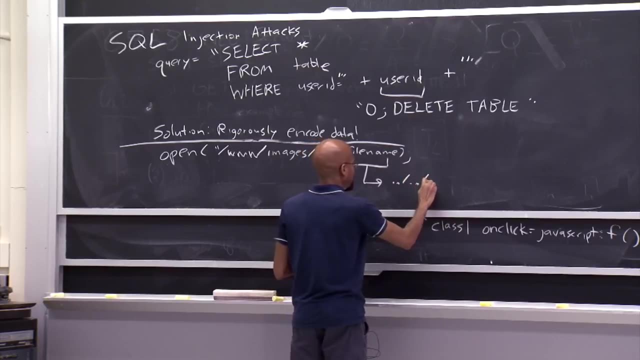 You're going to read from some file name that, once again, is supplied by the user. So, as we saw in some of the discussion of Trute and things like this, what if this file name maps to something like a bunch of instances of the dot dot? 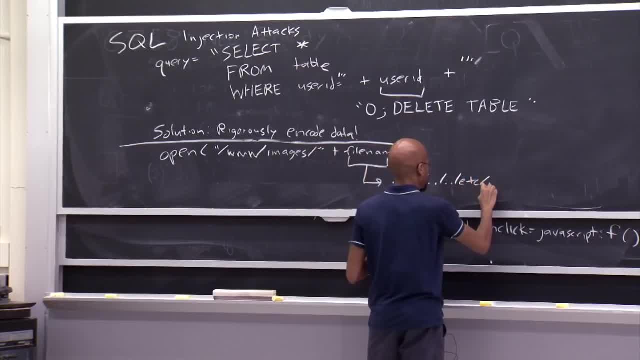 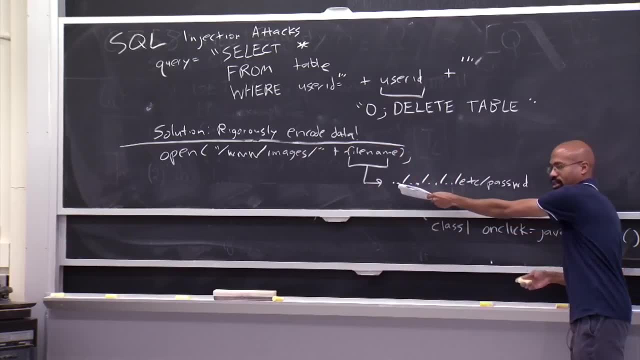 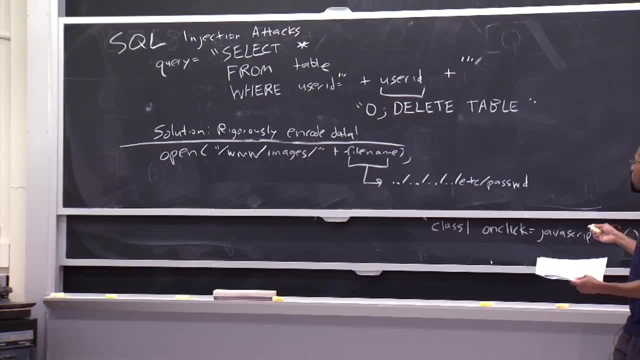 So, once again, you want to be able to use the web server or the web framework. You need to be able to detect these dangerous characters, escape them in some way to prevent those raw commands from executing. So I think that's all pretty straightforward. 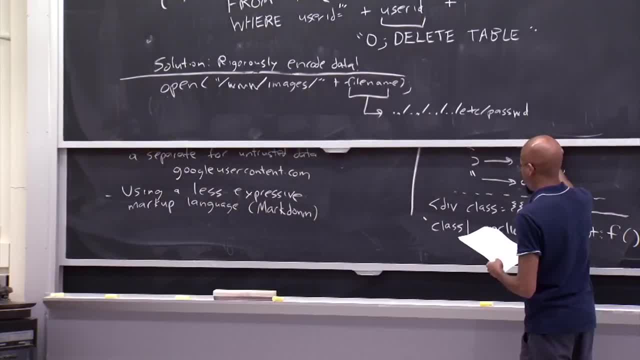 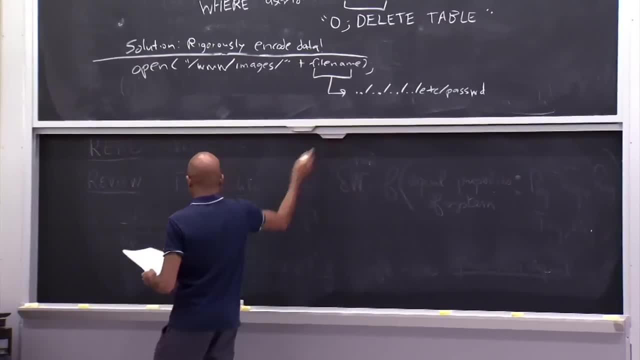 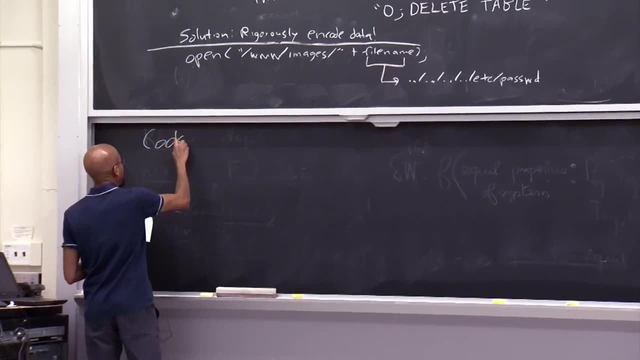 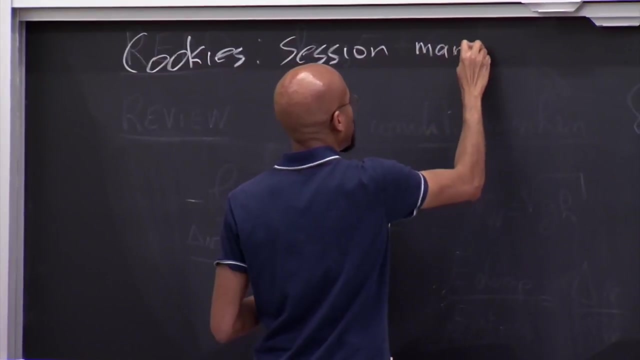 So let's move on from the discussion of content sanitization and now let's talk a little bit about cookies. So cookies are a very popular way to do session management: to bind the user to some set of resources that exist on the server side. 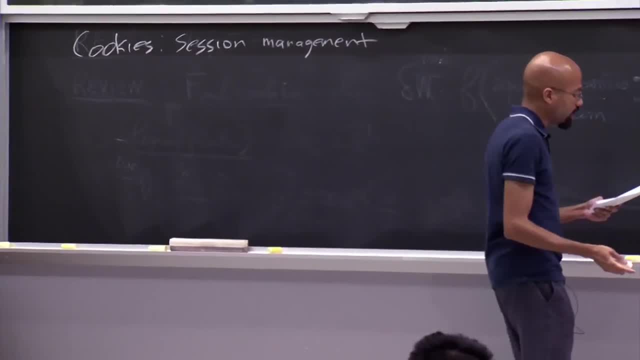 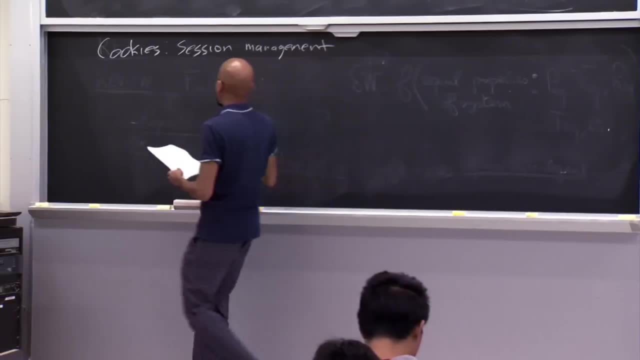 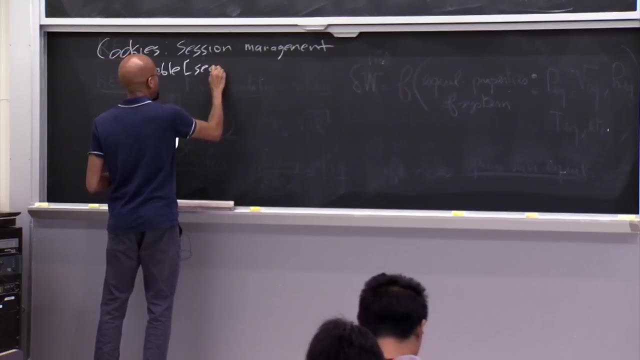 And so a lot of frameworks like Django, like Zubar that you see in this class. they actually put a random session ID inside the cookie, And so the idea is that this Session ID is the index in the sum server site table. 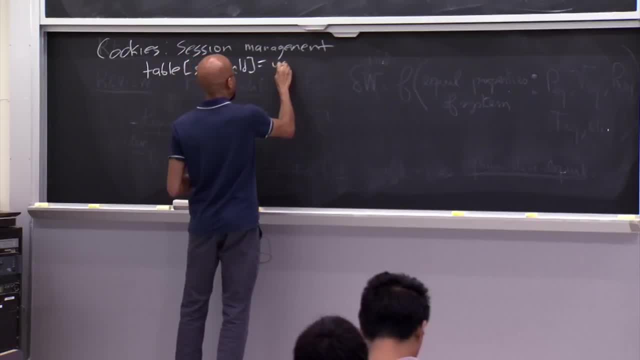 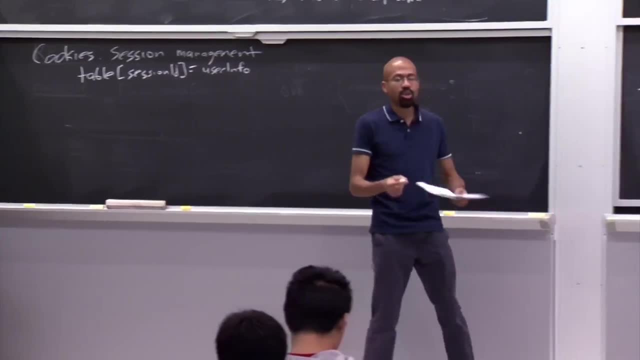 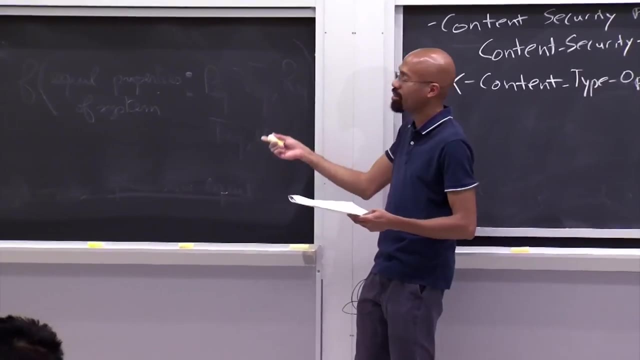 So you just apply the session ID there, and then this is where your user info lives, And so, as a result, this session ID, and cookies by extension, are very sensitive entities, And so this is why a lot of attacks involve stealing of the cookie in order. 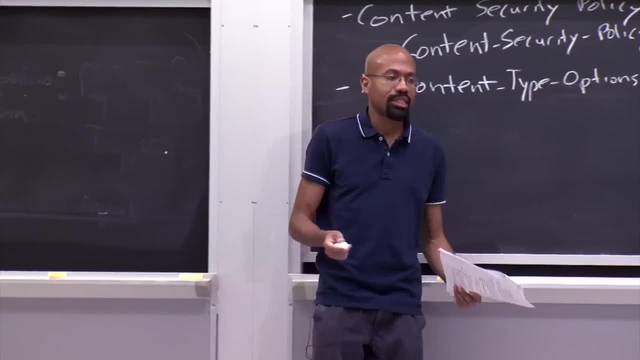 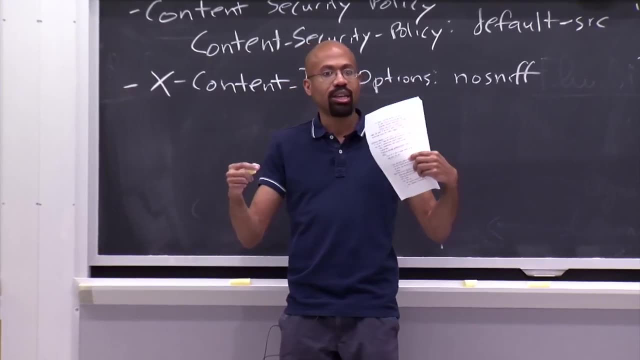 to get that session ID. And so, as we discussed in the last session, in the last lecture, the same origin policy can help you to a certain extent against some of these cookie-stealing attacks, Because there are origin-based rules that prevent arbitrary tampering with cookies. 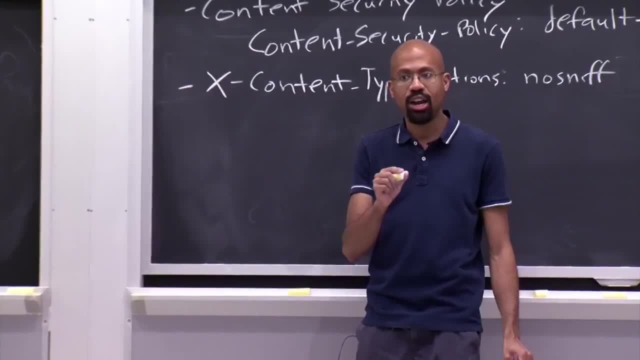 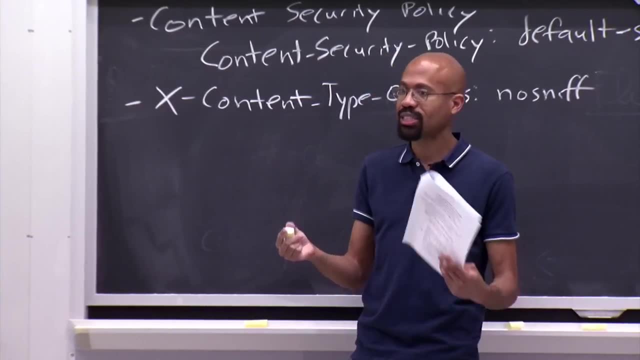 But one thing that's a little bit subtle is that you shouldn't share a domain or a subdomain with someone that you don't trust, Because, as we discussed in the last lecture, there are these sort of very subtle rules in which two origins with the same domain. 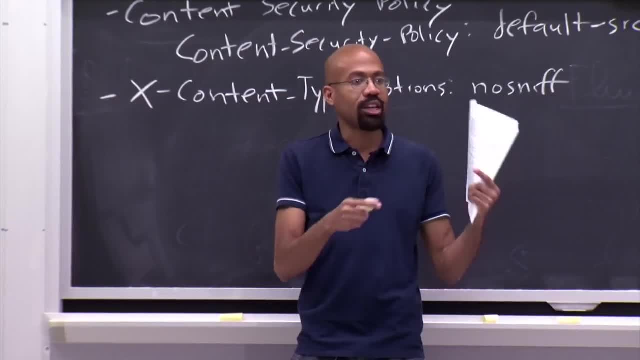 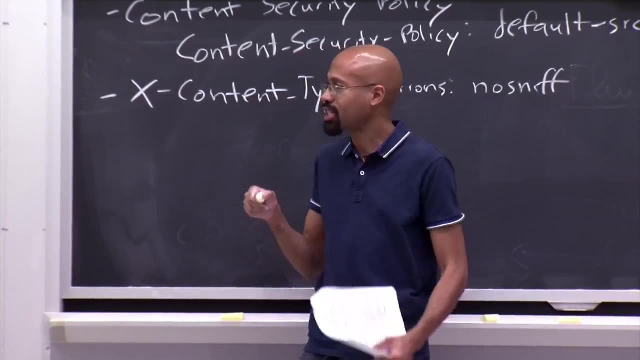 or possibly some subdomain relationship. they can actually access each other's cookies And so if you trust a domain that you shouldn't, then that domain may be able to do things like directly set the session ID in that cookie that both of you can access. 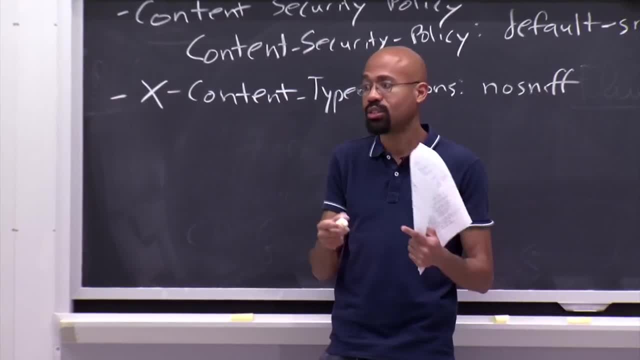 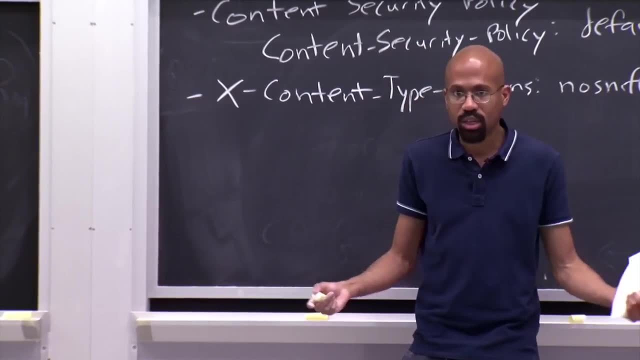 And that can do things like allow the attacker to force the user to use a session ID of the attacker's choosing. And then, for example, let's say the attacker sets the user's Gmail cookie. let's say The user goes to Gmail types some emails. 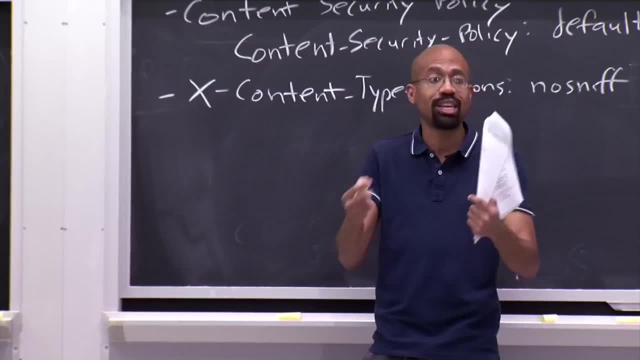 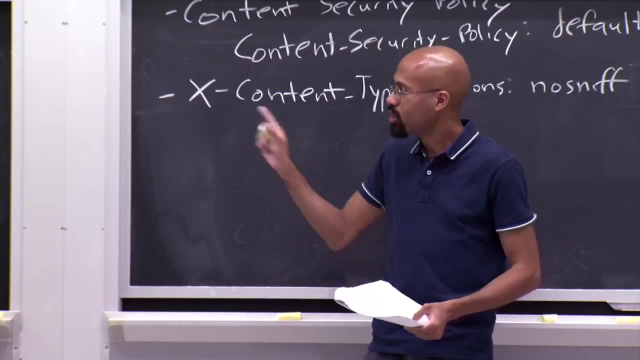 The attacker later on can then use that cookie or, more specifically, use that session ID, load up Gmail and then access Gmail as if he or she were the user who was victimized. So there's a lot of subtleties with using these cookies. 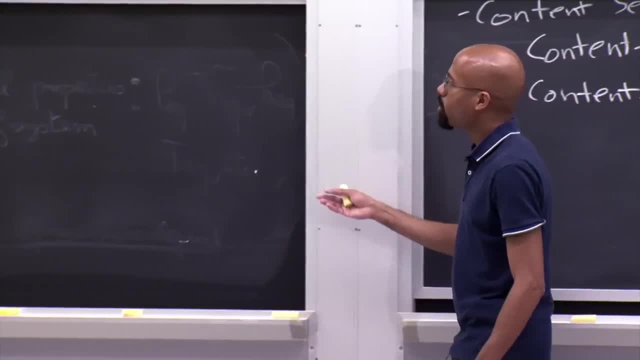 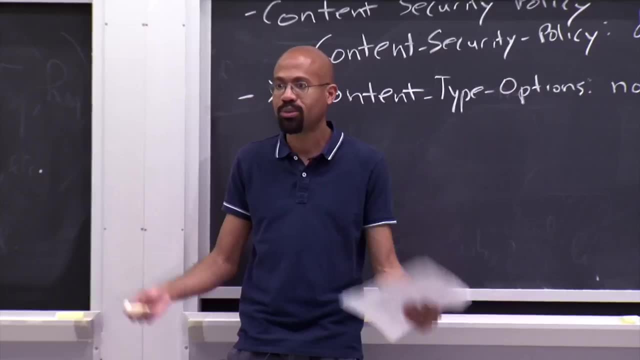 for session management. So there's a lot more we could talk about cookies. We've discussed some of it today in last lecture, So you might be thinking, well, can we just get rid of cookies? Cookies just seem more trouble than they're worth. 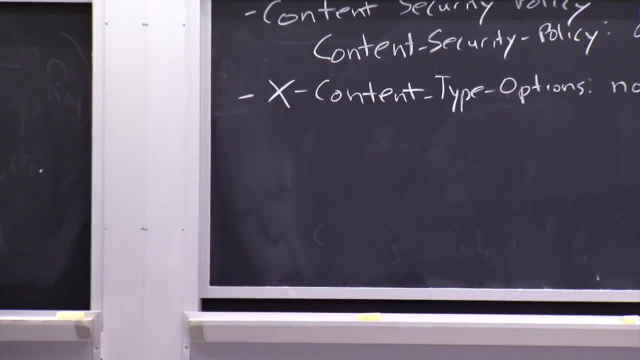 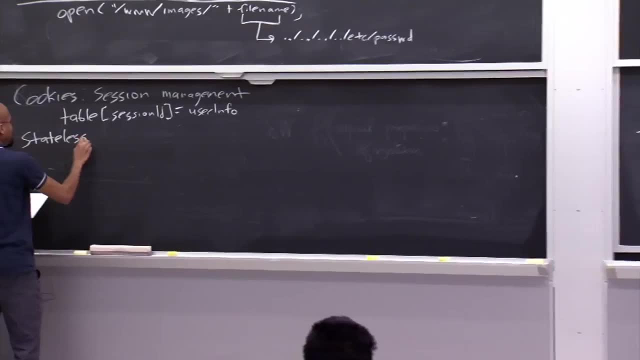 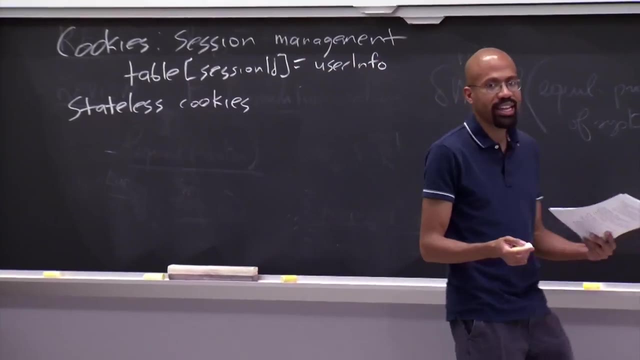 just like triples. So can we just not have these cookies? So one thing you can imagine is you can imagine basically having Some notion of stateless cookies, of somehow getting rid of the notion of sessions altogether and preventing this nasty attack vector that seems to be sort of prevalent in all these discussions. 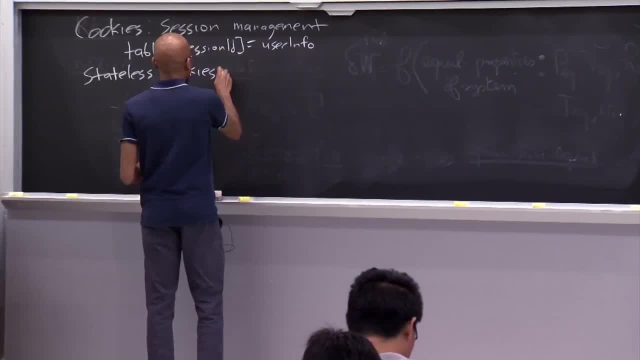 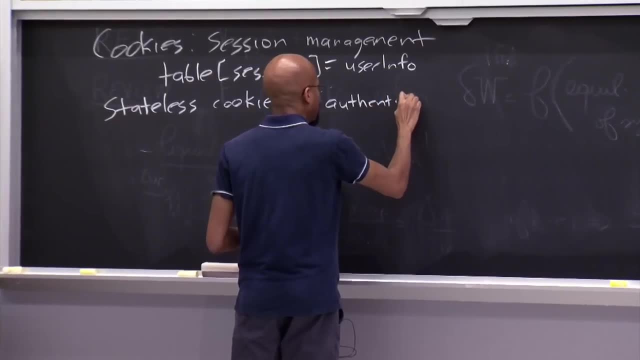 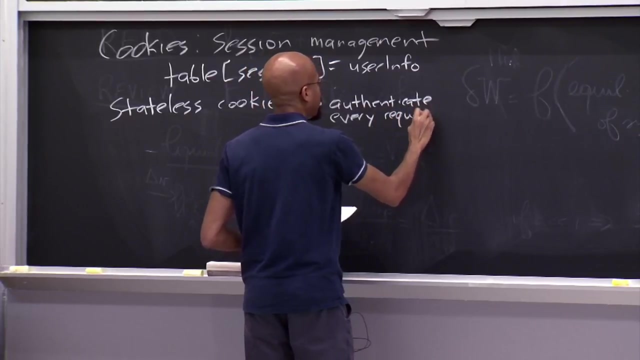 that we have. So the basic idea here is that if you want to go sort of stateless, then this essentially means you have to authenticate every request. Right, Because the nice thing about cookies is that they basically follow you wherever you go. So you authenticate once and then. 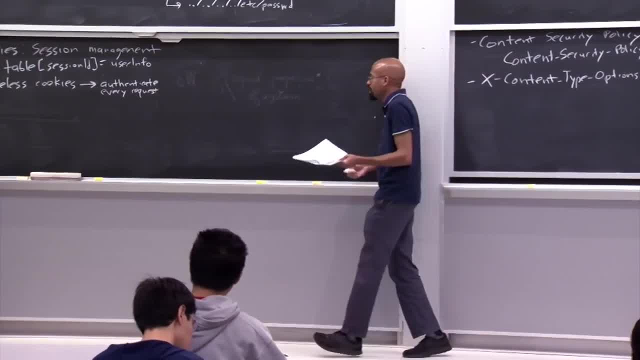 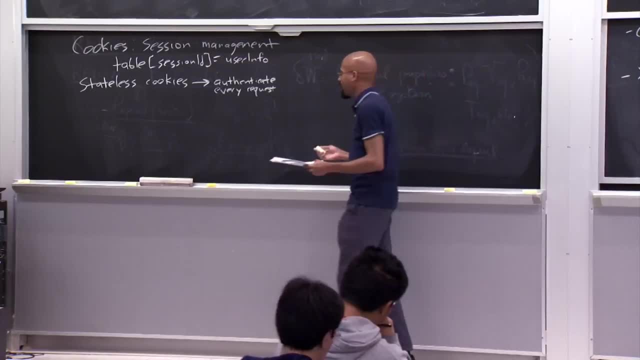 every subsequent request you make has this little token in it. But if you want to get rid of those things, well then now you essentially have to have some proof of your authority in every request that you make, And so one way you can imagine doing this. 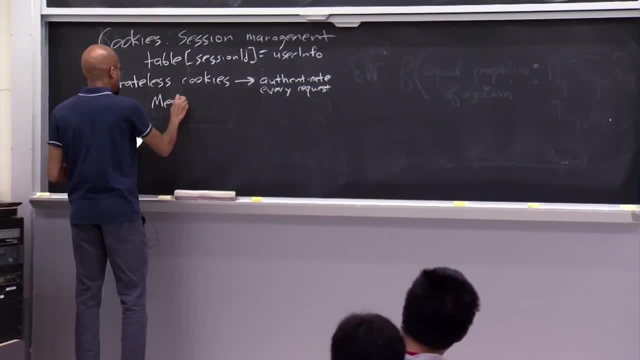 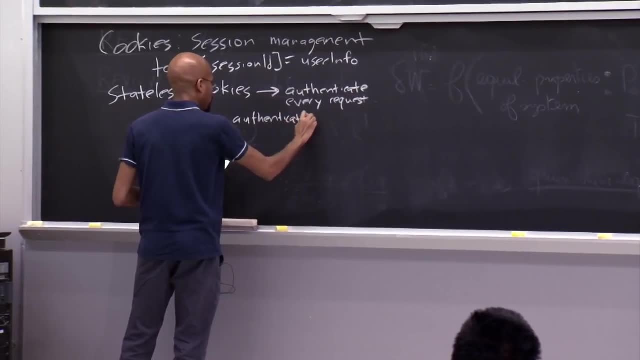 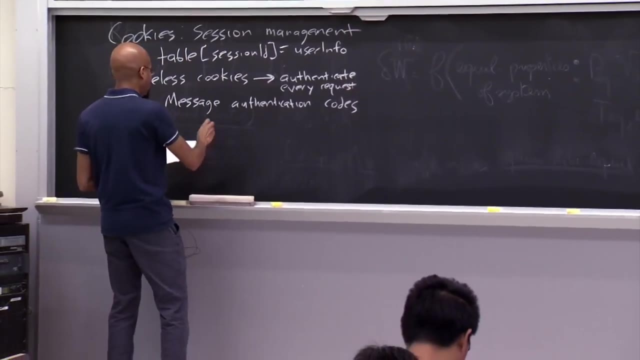 is by using something they call MACs, or Message Authentication Codes, And so the basic way to think about this is to think about one of these MACs. It's like a hash that takes in a key as well, So the authentication code is the hash of some key. 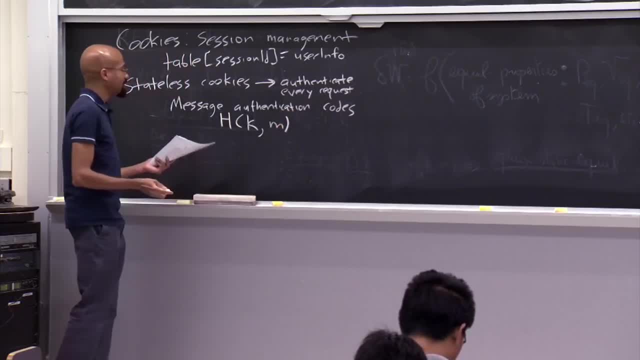 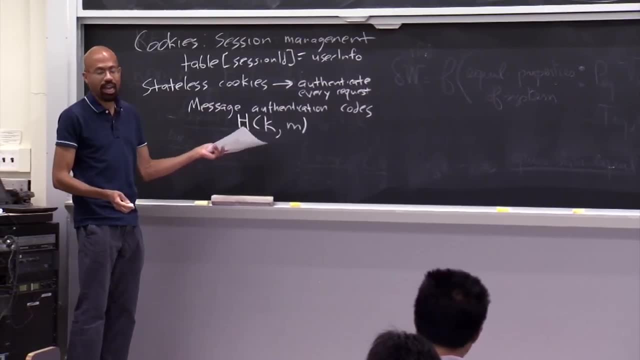 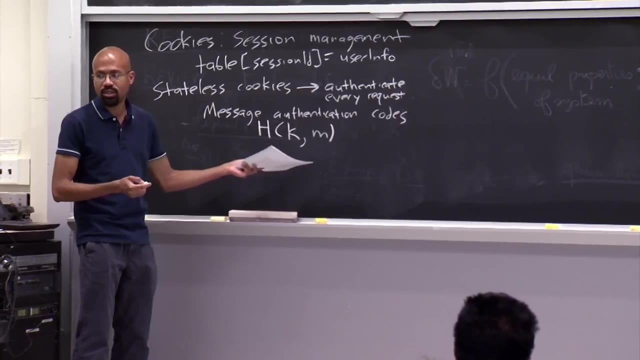 and then some message. And so the basic idea is that the client, the user and the server are going to share some secret key K, And so the client uses that key to sort of produce a signature over the message that it sends to the server. 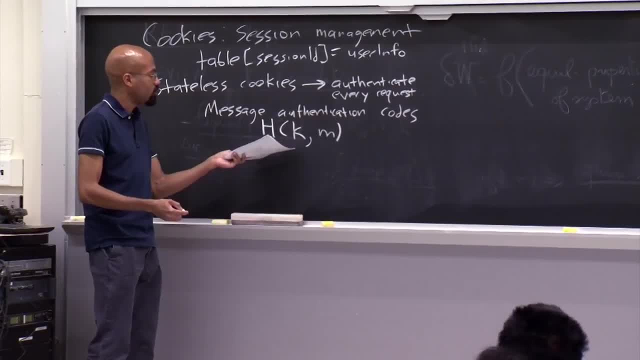 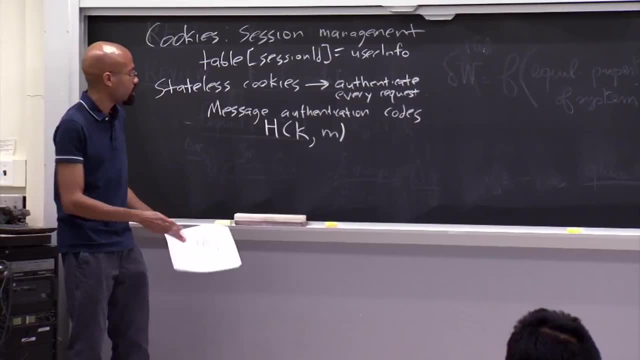 And then the server, who also knows the key, can then use this same function here to validate that the signature is correct. So let's look at a very specific example of how this works. So one real service that uses these types of stateless. 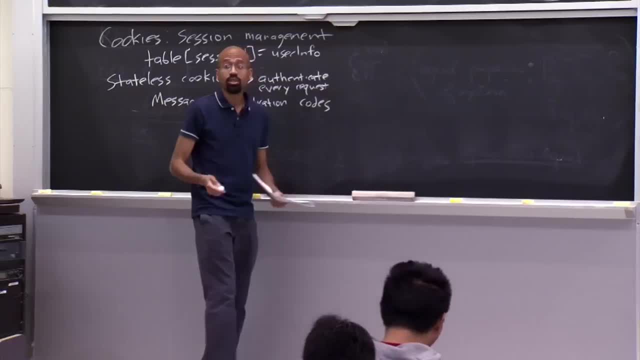 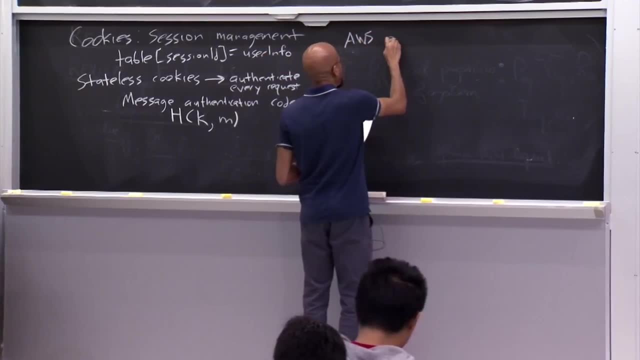 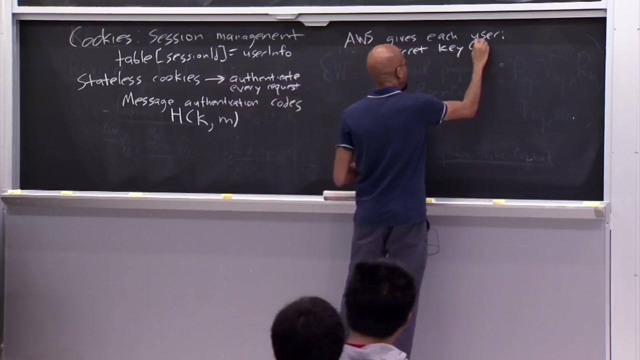 cookies is Amazon Web Services. It's like S3,, for example, And so, basically, Amazon AWS gives each user two things. It gives that user a secret key, and so this is equivalent to the K that we were discussing over there. 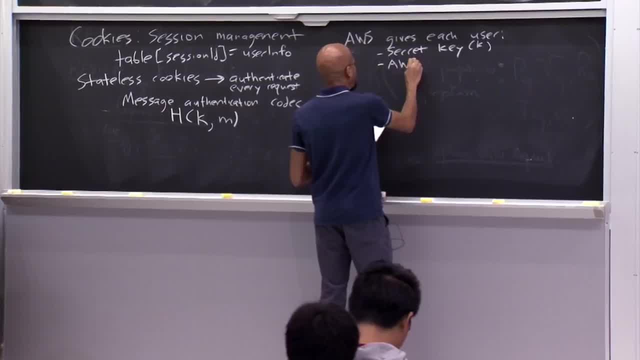 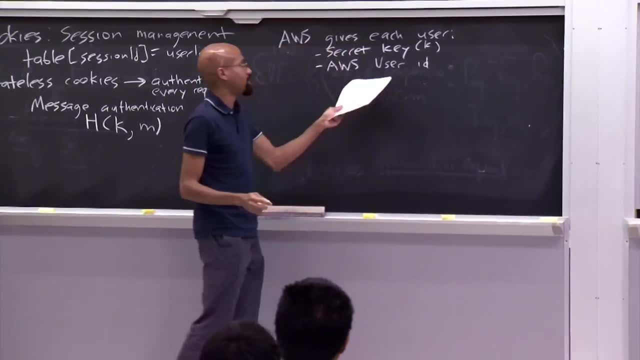 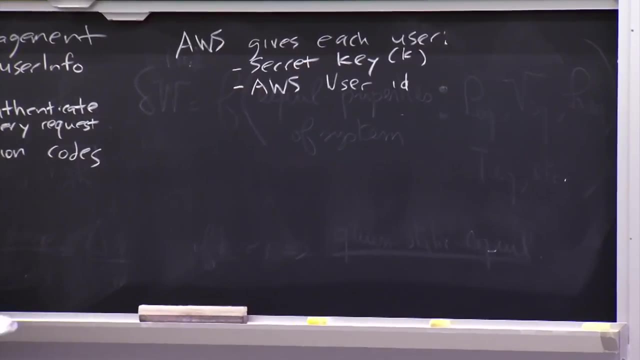 And it also gives them- let's think of it like an AWS user ID. So this part is not secret, but this part is, And so every time you want to send a request to AWS via HTTP, you have to send it in this special format. 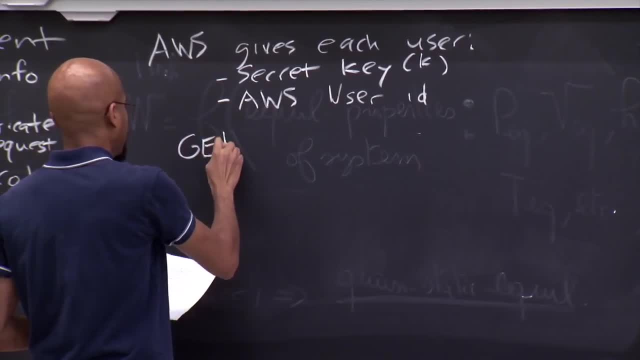 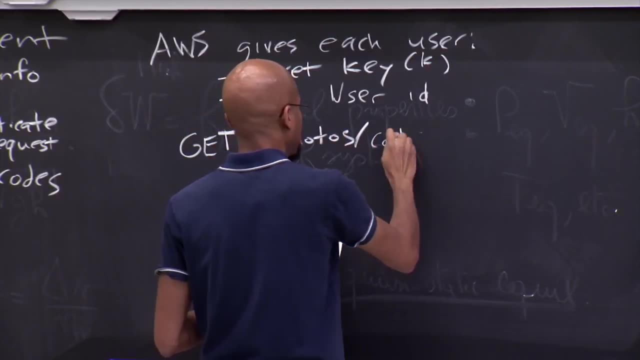 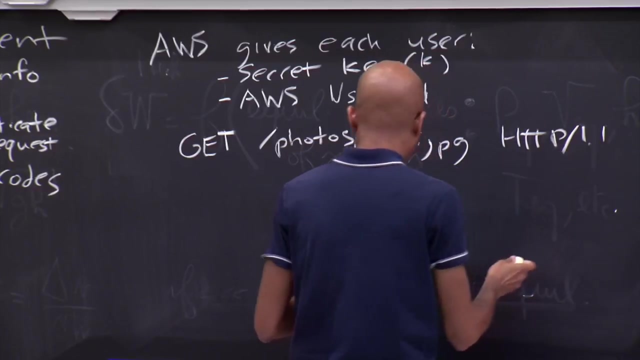 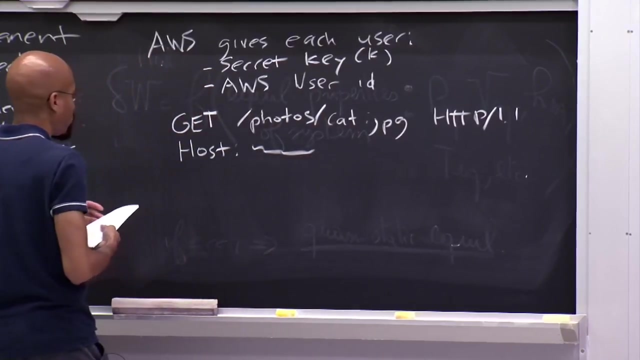 So you'll have the first line of the get request: So you want to access some photos- No surprises here- And then you'll put the host from which you expect to get it. That's not super important. so this is just some AWS server. 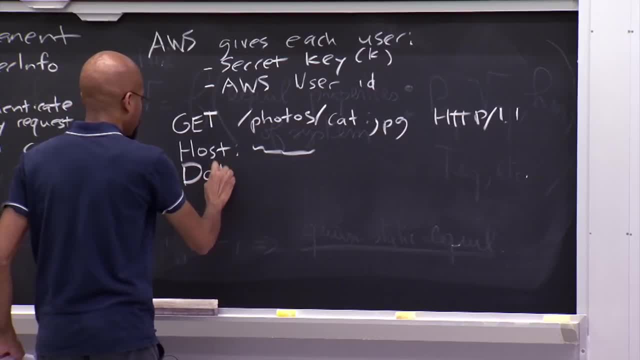 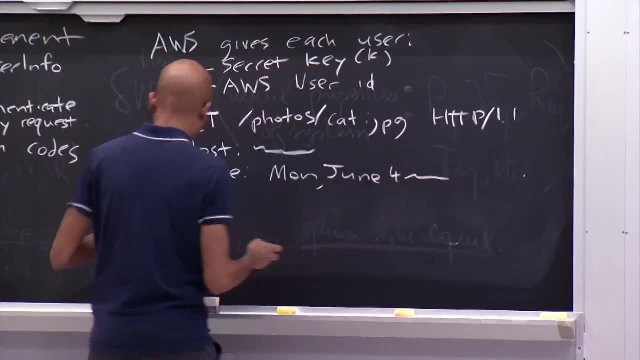 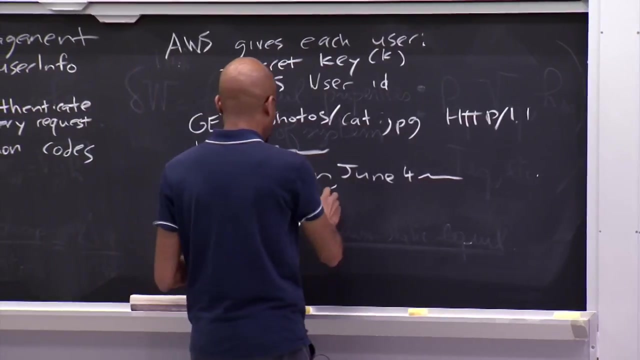 that's there. You'll have a date, so maybe this is Monday, June 4,, whatever- And then you have this thing. that's essentially the authorization field And this is where the message authentication code comes in. So essentially, what this looks like is: you've got some string. 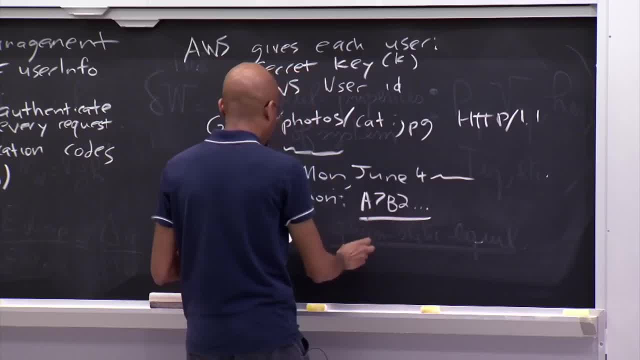 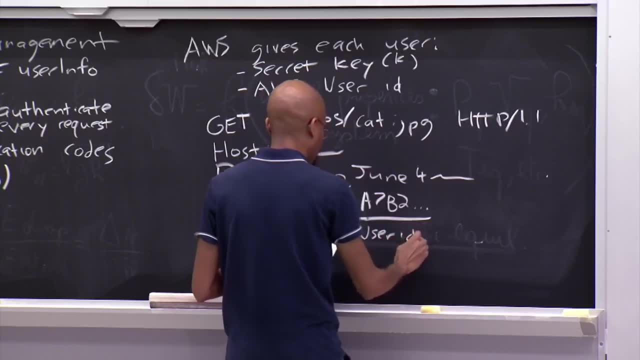 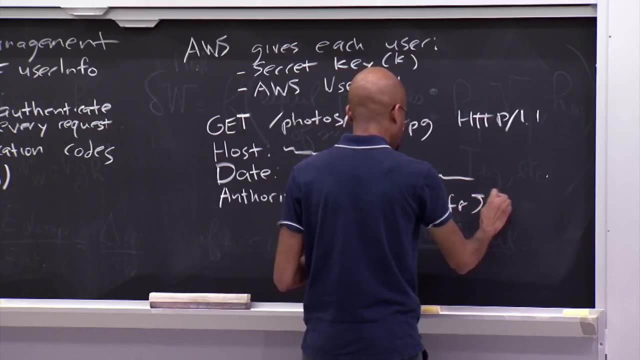 here. This represents your access ID or the user ID, And then you've got something here, some other seemingly random letters, And then these things are a signature that use this method- authentication code here. So what does that signature look like? 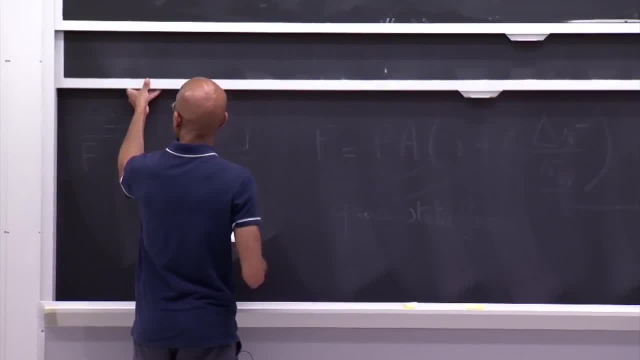 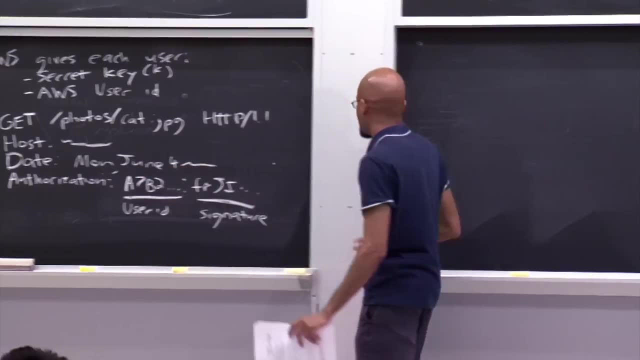 So the details are a little bit complicated, but basically this signature is over a string that encapsulates a bunch of details in this request. 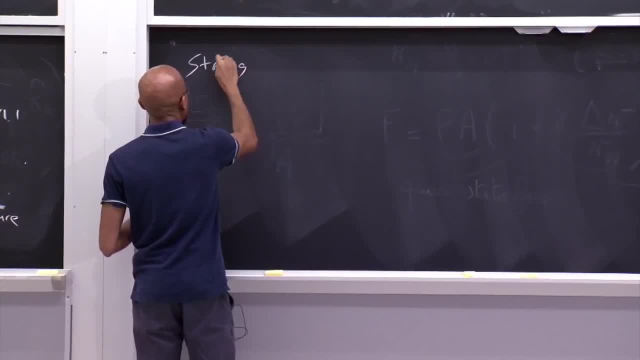 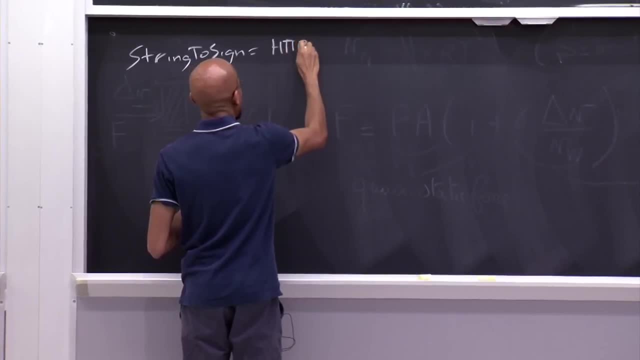 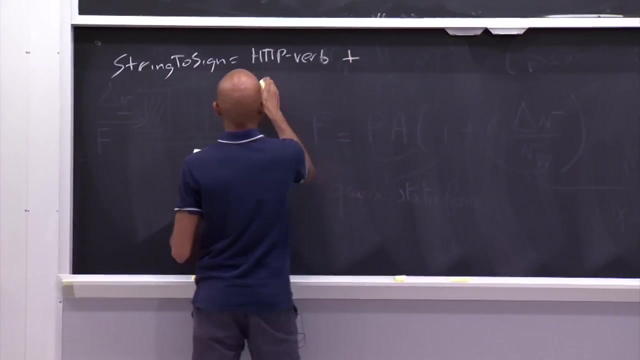 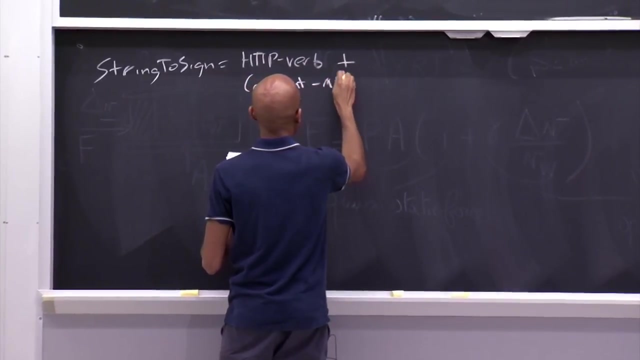 So essentially the string, the sign looks something like this: So you put the HTTP verb in there, So in this case that verb is get, and then you put a md5 checksum of the message content. 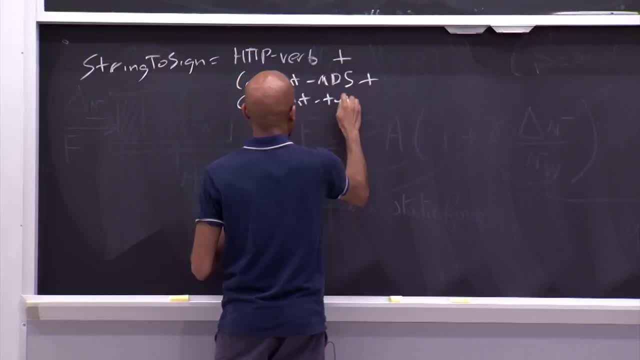 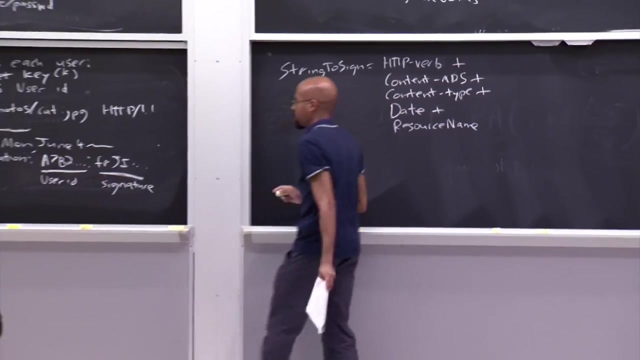 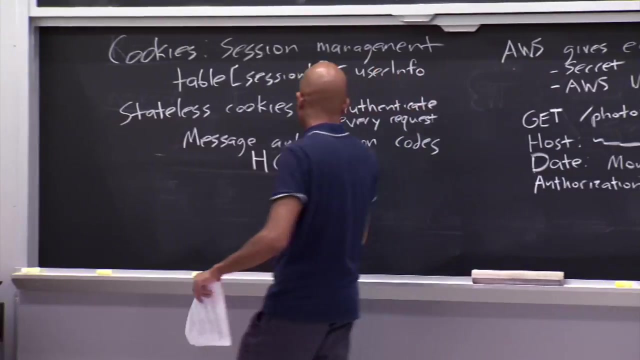 And then you also put the content type, so it's HTML or image or whatever. You put in the date and then the resource name, which is essentially the path that you see over here. So, in other words, this string here is the message that you pass into the HMAC over here. 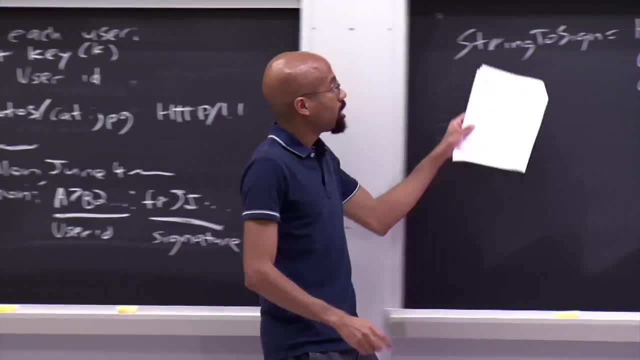 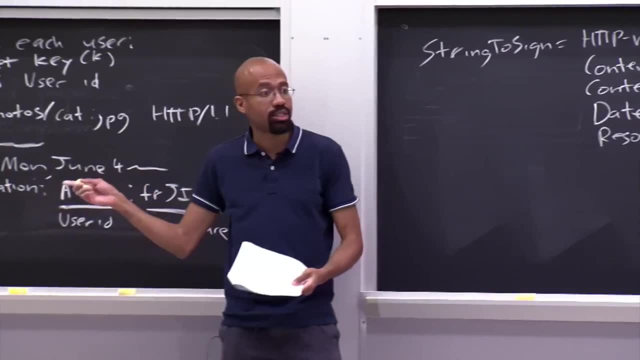 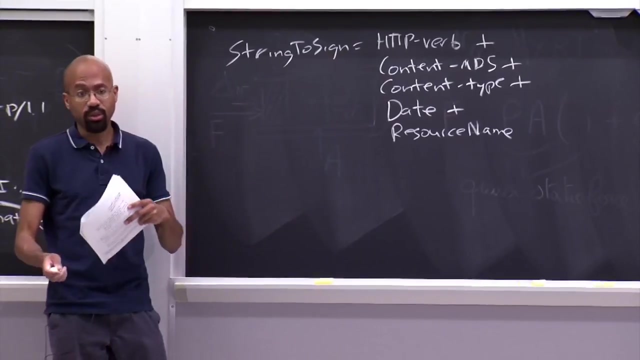 And so note that the server can see all this stuff in clear text in the request, And so that's what allows the server to validate that message. authentication code is correct, Because note that the server shares that key with the user, So that allows the server to validate that kind of stuff. 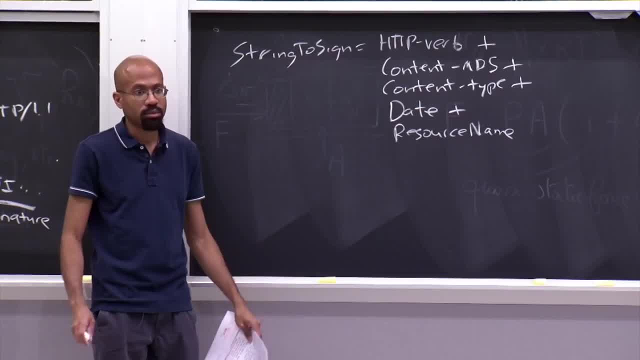 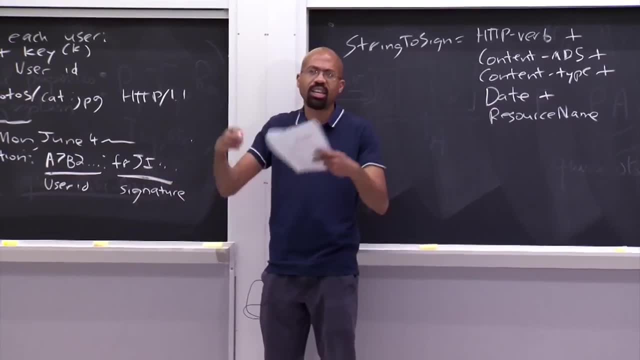 So does that all make sense? So what would be the content here? Oh, so, in this case, for the content, that's probably going to be nothing like the empty string, But you can imagine if it was a post or something like that. you'd actually have the data of the HTTP. Do they really use md5, which is kind of an unfortunate choice now? just So, I believe that they do So. I checked the Amazon documentation yesterday So I believe they do use it. 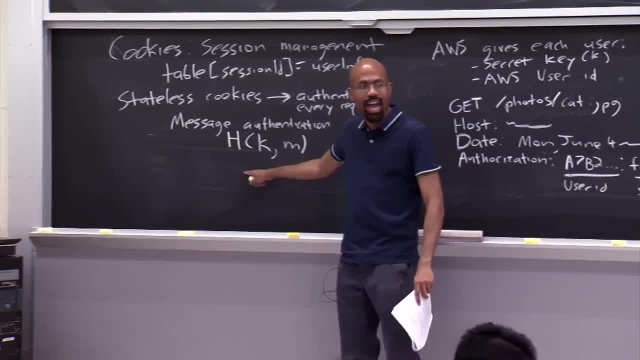 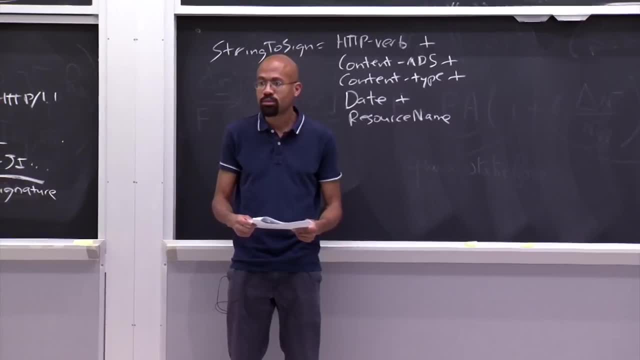 But I think I could be wrong. but I think they actually use a stronger hash here, So that helps a little bit. but you're right, md5 is not the best. I didn't entirely follow how you guys would do that. 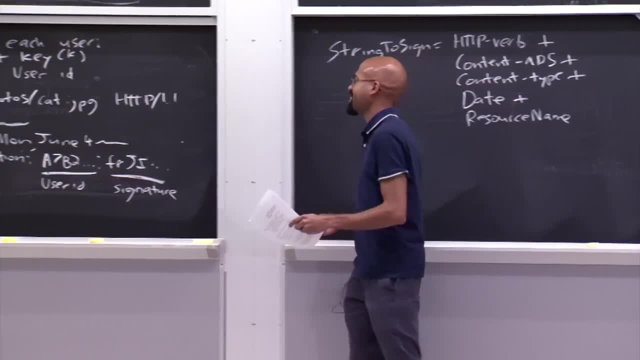 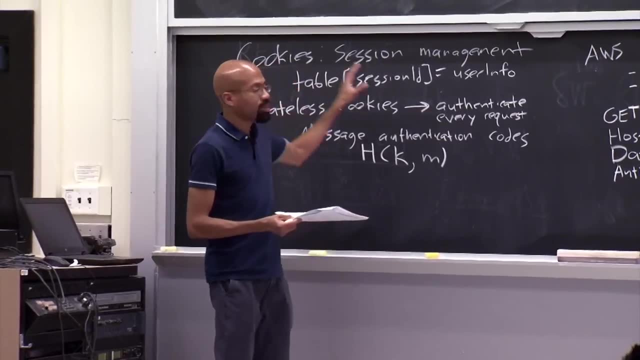 This works OK, so allow me to help you. hopefully So, even though I'm the guy who confused you in the first place. The basic idea is that we want to get rid of this notion of this persistent cookie that's always following the user around. 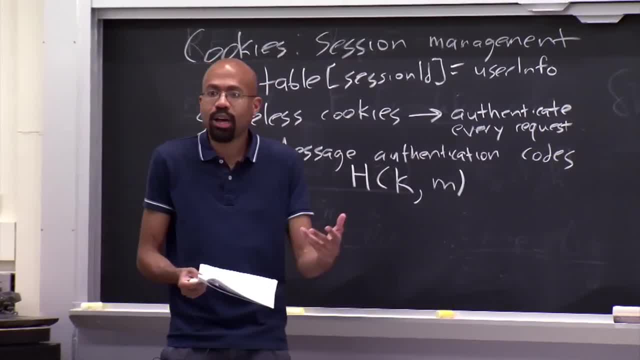 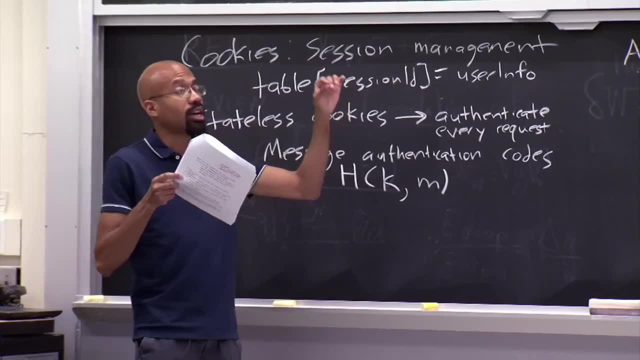 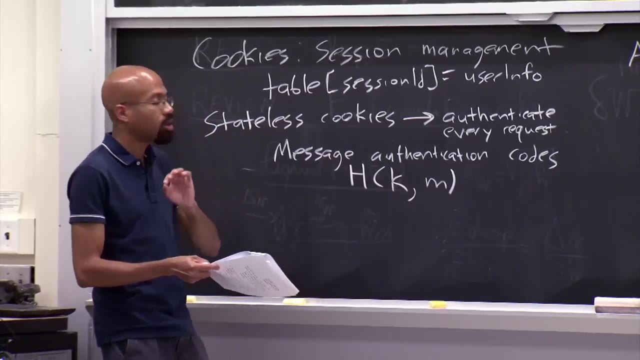 Now. the problem, though, is that the server needs some way to identify which client it's talking to. So what we're going to do is we're going to ensure that each client shares a unique key with the server, And so, basically, whenever the client 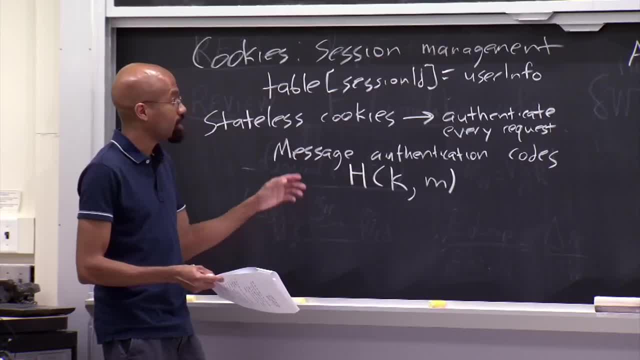 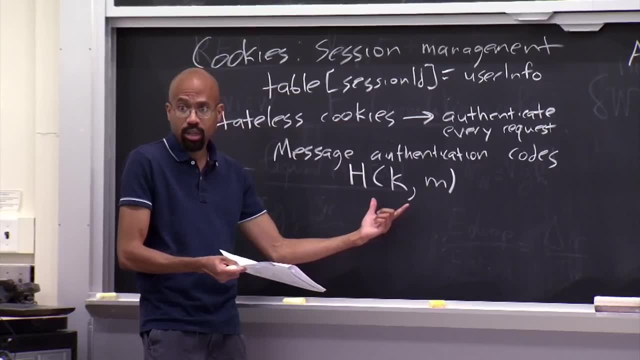 sends a message to the server. the client is going to send the messages before and then also send this special cryptographic operation. the result of this operation here, Oh OK, So normal message in clear text, and then again you hash it. 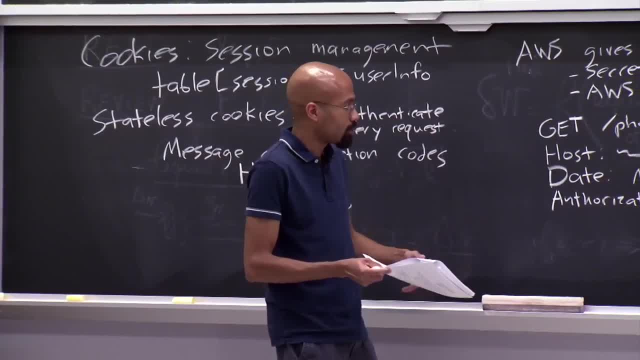 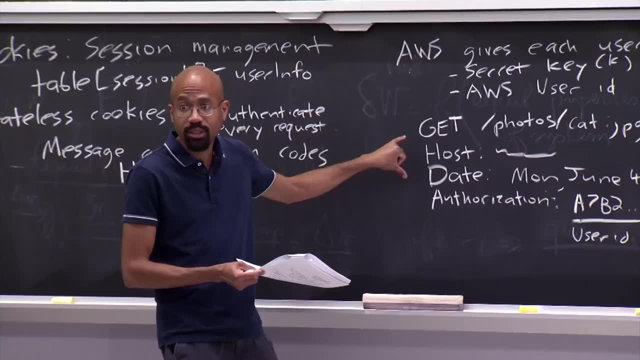 Yeah, so basically to first approximation. imagine that in the regular world this would be some cookie here Instead of the authorization. But now we're getting rid of the cookie and we're saying: here's this clear text message, Then here's this crypto thing which basically: 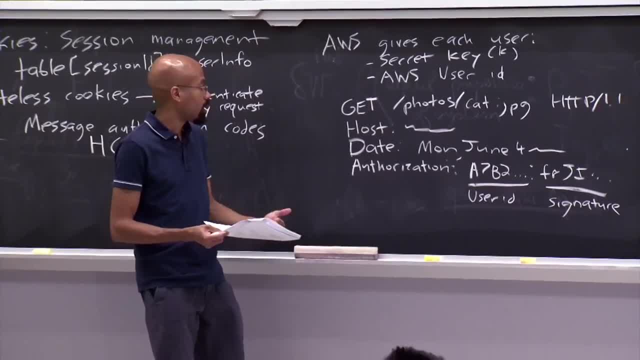 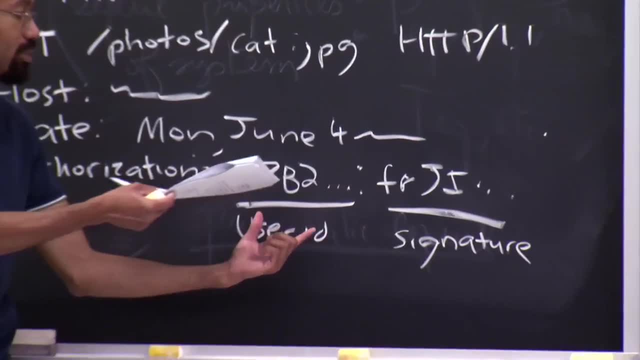 allows the server to figure out who this thing came from, And so the server knows who the user is, because that's embedded in the clear. That's not a secret right. But this basically allows the server to say: aha, I know which secret key this user should. 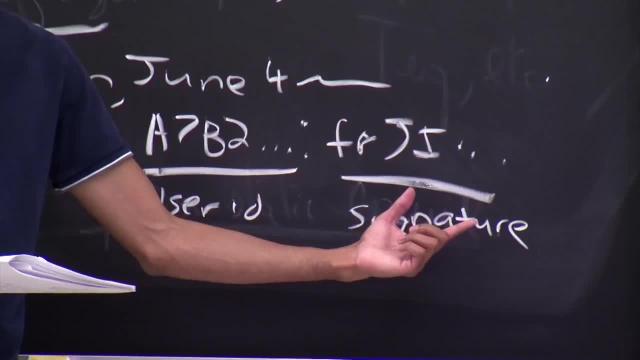 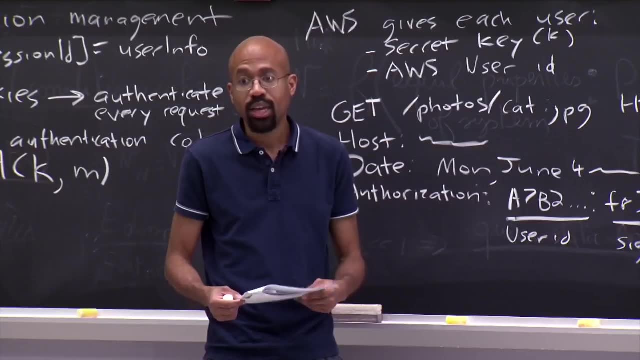 have been using to create this. if that is in fact the real user, Nice, OK, Thanks. So what preventive measures? What prevents the attacker from finding the key, Like where is the secret key? Yeah, that's a good question. 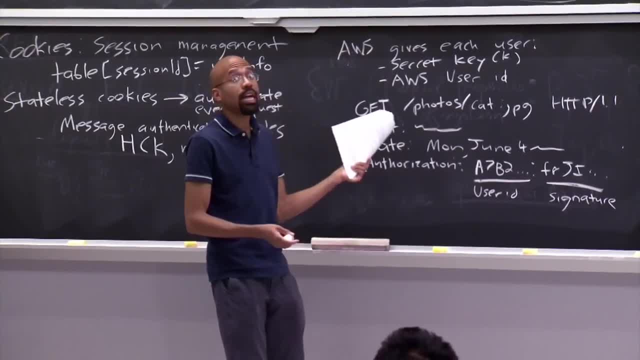 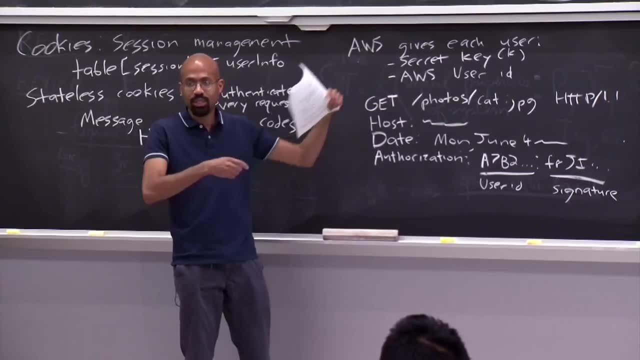 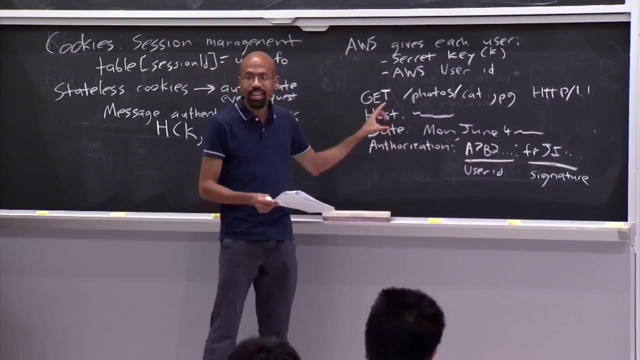 So in a lot of cases the client for AWS is not a browser, but some VM running in the cloud, for example. So you'll see VM to VM communication. You can also imagine, too, that users can sort of hand out these links or embed them somehow in HTML. 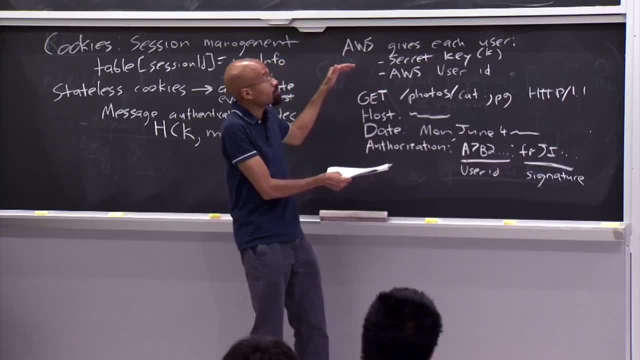 So it's like you just have sort of this in the- how do you say it? Like inside the HTML or JavaScript source code, you'd have the code to create a request like this. So it's almost like me giving you a capability, right. 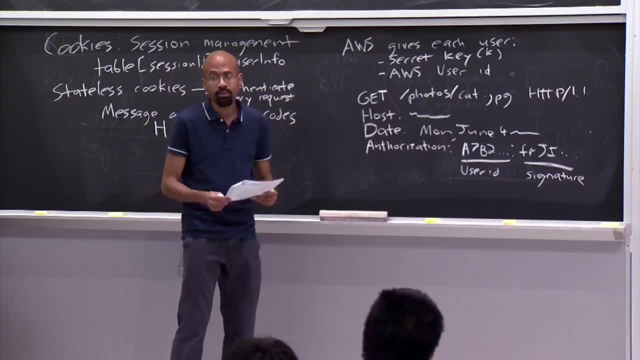 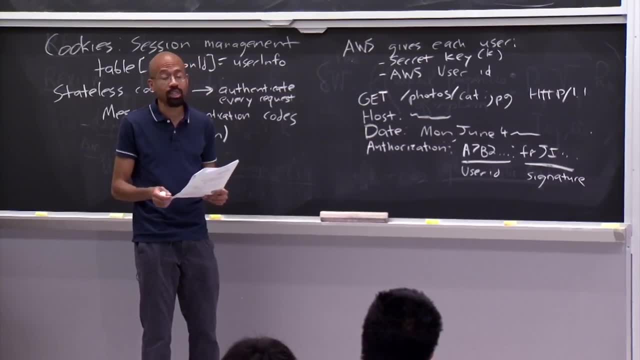 So if I give you one of these things, you can make that request on my behalf. basically, So would it be possible to use Max on the normal clients for the? For normal, you mean like browsers For normal users at home? Yeah, well, I mean you get into these questions. 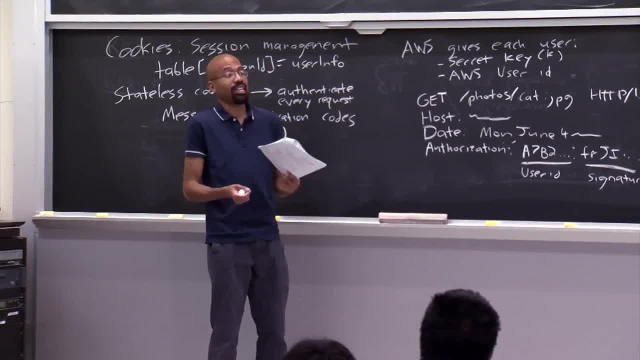 like: where does the key live, right, Which is kind of like he was asking. So in a certain extent, the issue of where the key lives is actually super, super important, right? Because if the key can be stolen just as easily as the cookie, 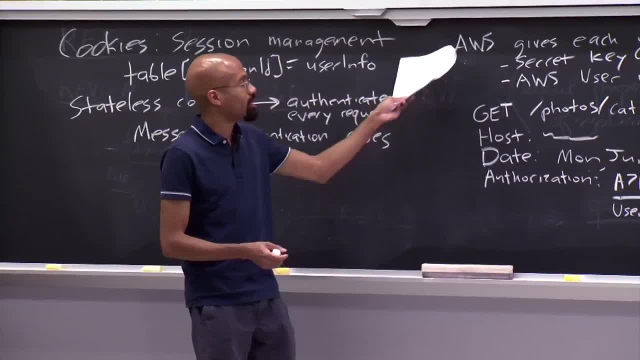 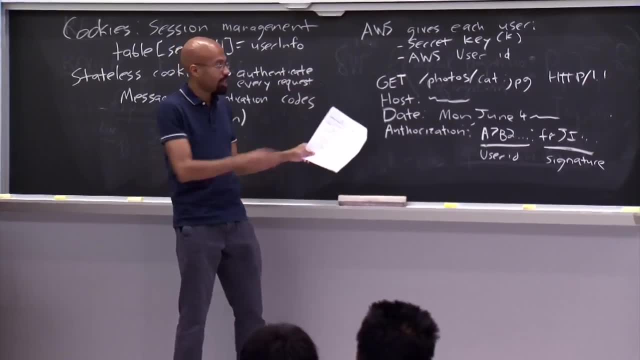 well then we're sort of back to square one. So in many cases this stuff is actually used, like I said, sort of server to server, like a VM to VM somewhere in the cloud. So the application developer runs a VM that sort of outsources a bunch of storage stuff to AWS. 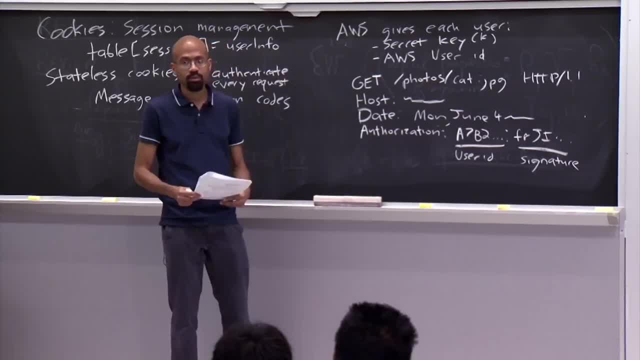 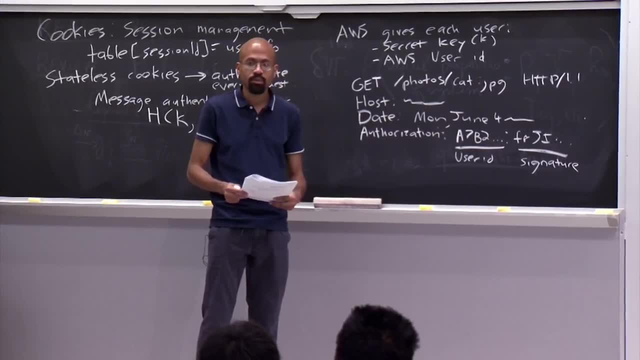 So they're using things that you play it back or whatever. but it's not kind of a bad thing for any Because they have network latency, so it can't be like too fine-grained of a constraint that they're putting into the application. 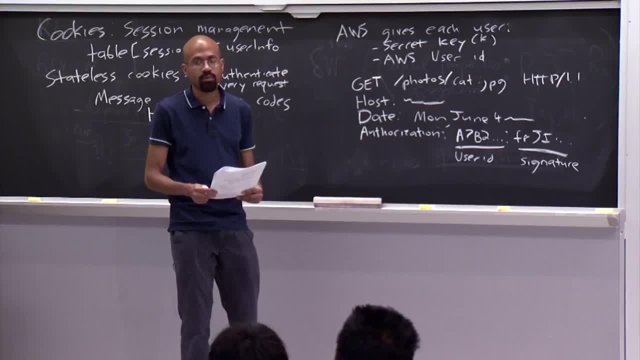 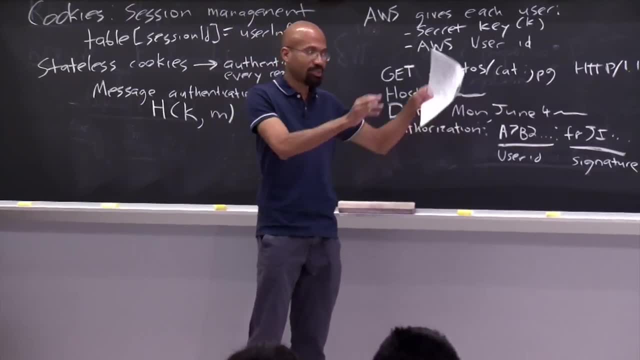 So if an attacker sent the same request again really quickly after the user, wouldn't they be able to server execute the request? Yeah, yeah, yeah. So suffice it to say that secure time stamping is like several people's PhD thesis. But you're exactly right that if this were just 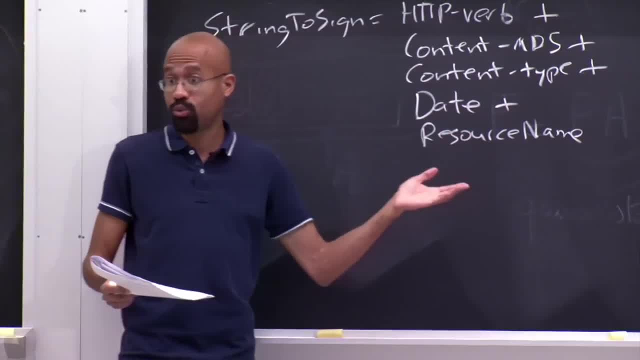 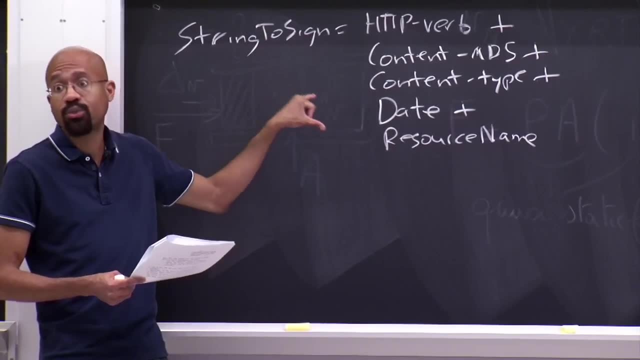 as a crude example, right? So imagine this, just said like Monday June 4th, right? Then if somehow the attacker could get access to this entire thing and there was nothing that was different about it, right? So there's no nonce, no randomness. 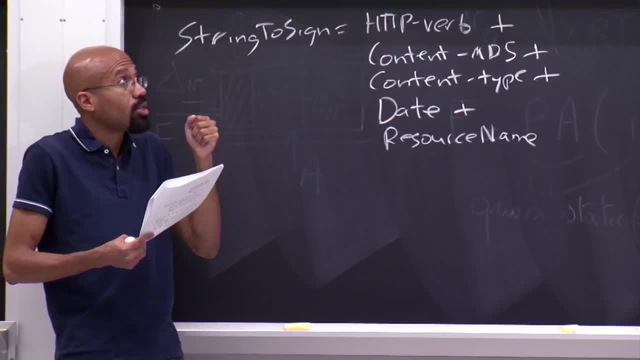 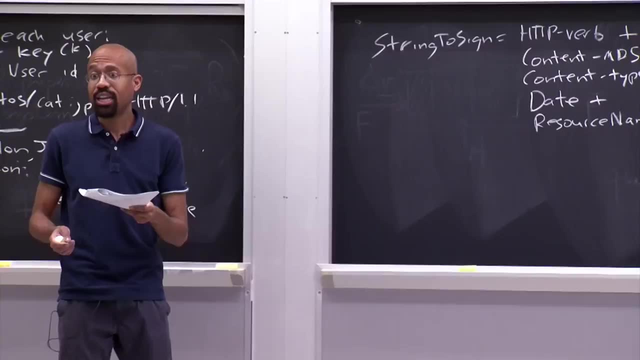 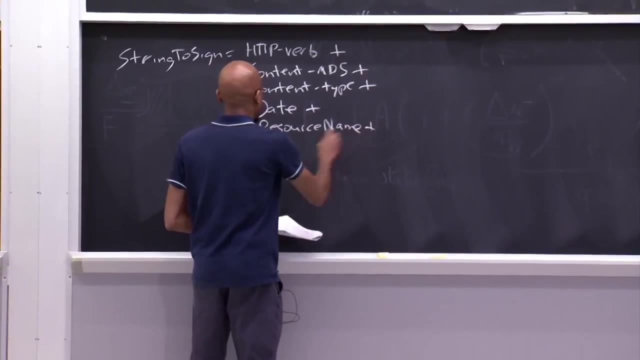 And stuff like that, And that's right and that request could be replayed. Now, one thing that AWS actually does is you can actually include an expiration date in these things. So one thing you can actually do is add sort of expires field. 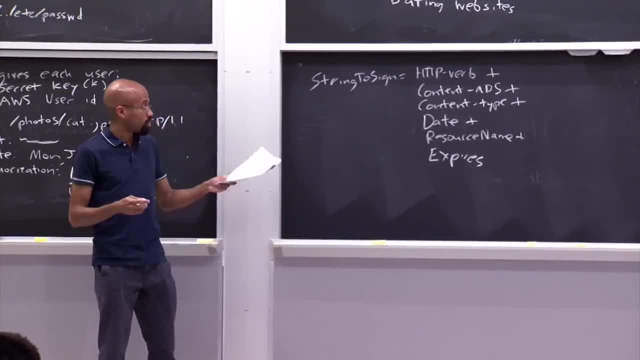 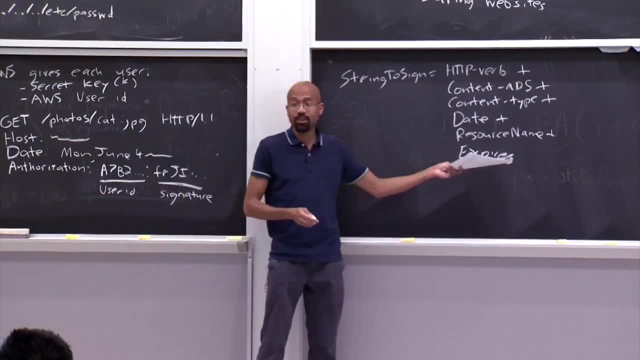 essentially Have that thing be signed, Then I can hand that reference to a bunch of different people. kind of like I was saying in response to his question, It acts as a capability, but the browser- sorry, the server- can then check that expiration date. 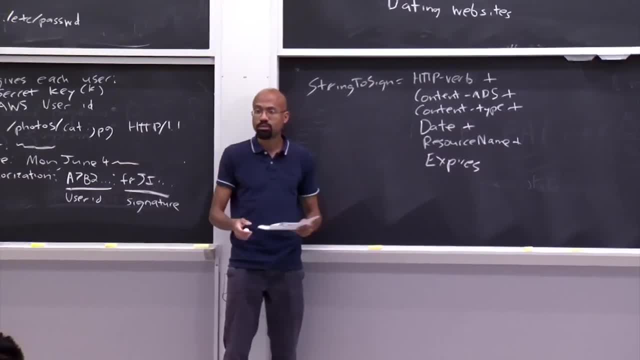 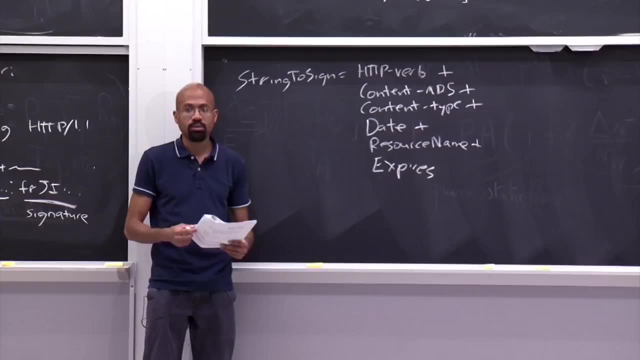 for when it actually sees it and then not actually. But even if the expiration date is like 200 milliseconds in the feature or something, as long as the attacker has really low latency, then they can send two copies instead of one. Yeah, that's exactly right. 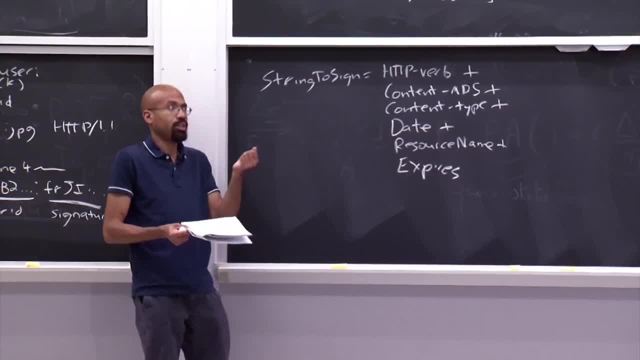 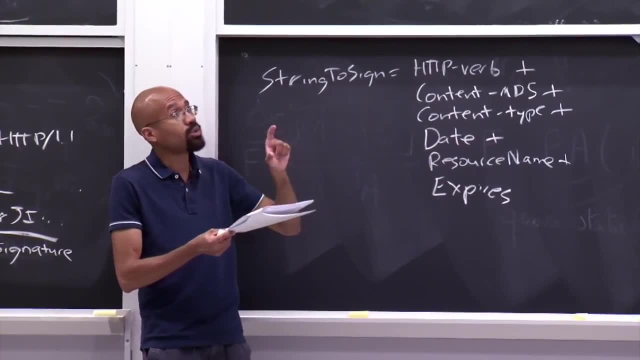 That's exactly right. So yeah, if the attacker can somehow like a network attacker, for example, is seeing these things go over the wire. and you're right, if there's enough sort of wiggle room in the expiration date, then they. 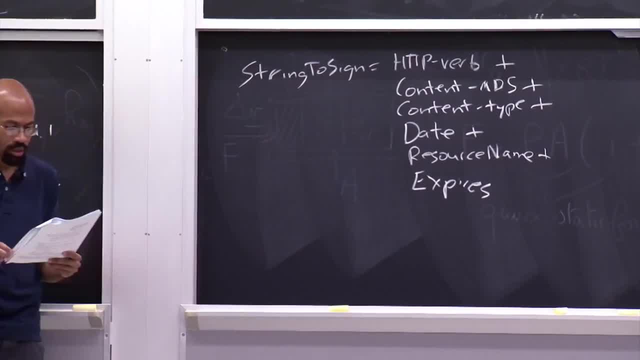 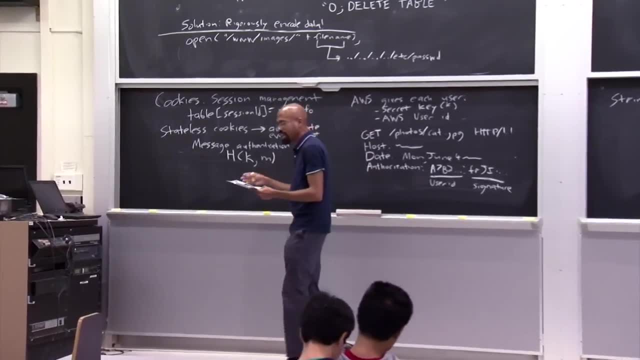 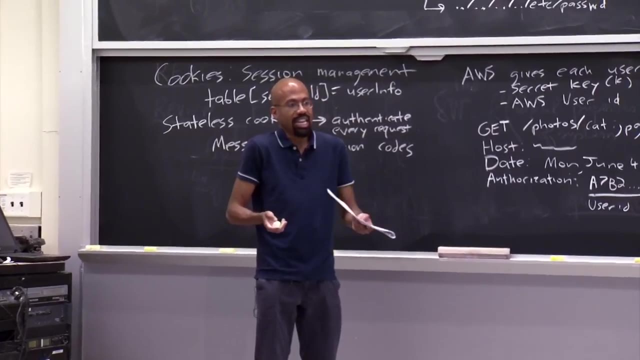 can exactly do that attack. That's right. OK, so that is sort of an overview of how these stateless cookies work, And so one question that's interesting is: you might think: well, what does it mean to log out with this type of cookie? 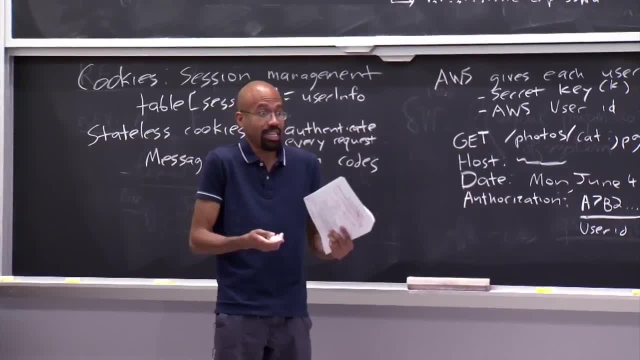 And the answer is that you don't really log out, right. I mean, you have this key and so whenever you want to send a request, you just send it, You include this dude right here and then you're ready to go. 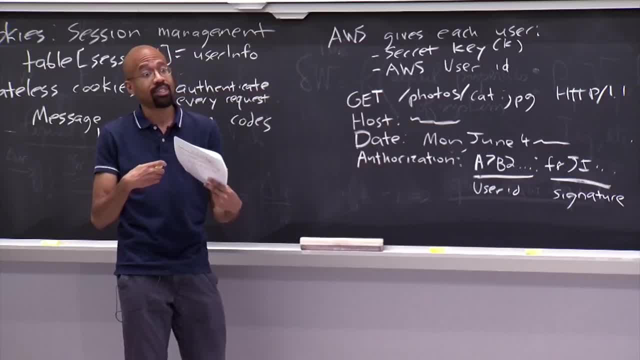 Now, one thing the server could do, for example, though, is revoke your key right. So if the server revokes your key, then you can generate one of these things, But when you send the message over there, the server's going to say: aha, I. 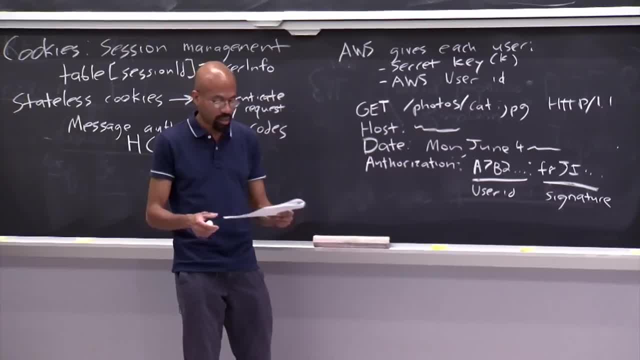 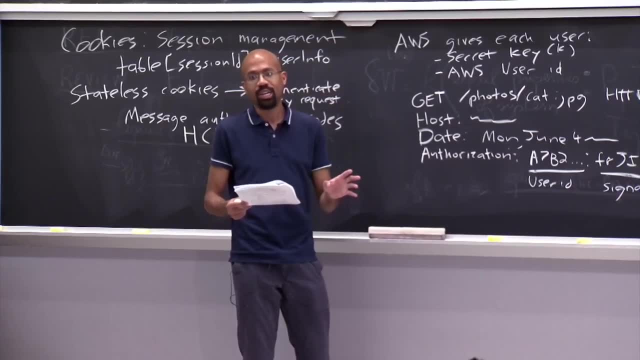 know what your user ID is. You've been revoked, so I'm not going to honor your request, But it's a little bit interesting, right? And revocation- as we'll talk more about- with things like SSL- is always a tricky issue, right. 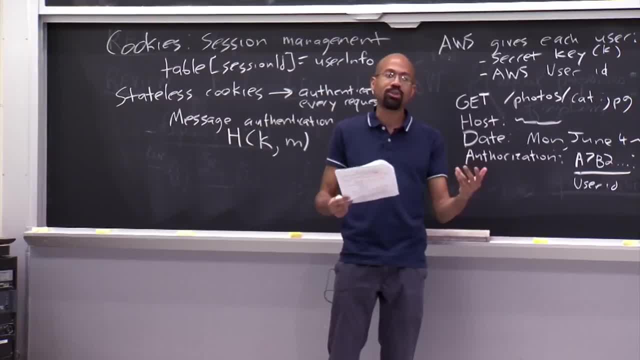 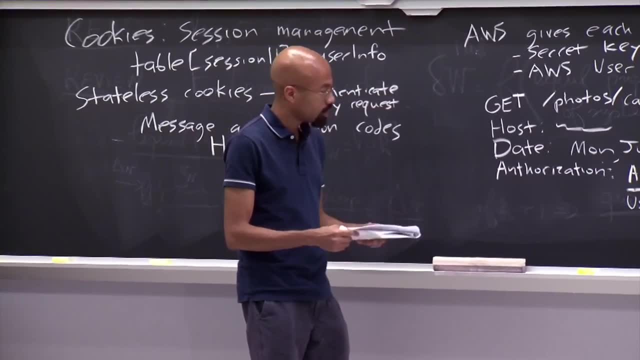 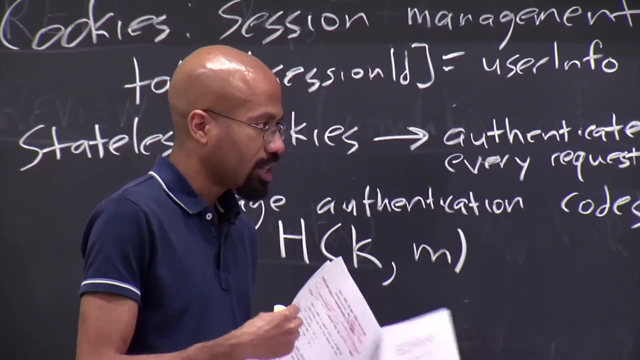 Because, as it turns out, taking authority away from human users is often much more difficult than giving it to them in the first place. So that's the basic idea behind These sort of stateless cookies. So there's also a couple other things that you can use if you want to avoid traditional cookies. 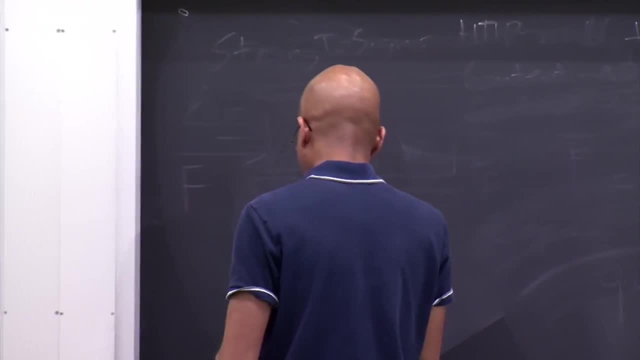 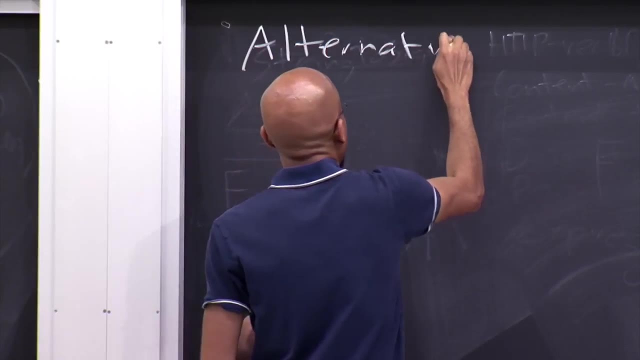 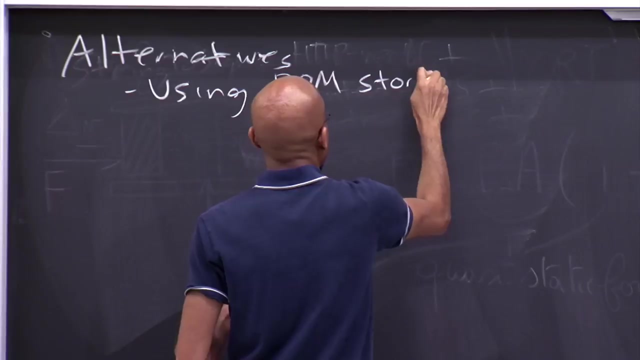 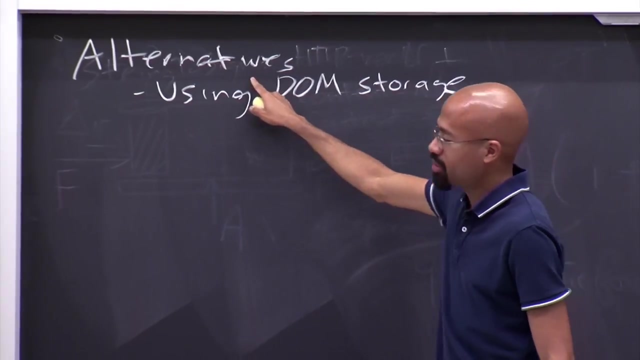 for using. sorry for implementing authentication. So one thing you can imagine doing is actually using DOM storage. You can use DOM storage to hold client-side authentication information. This says alternatives in case you can't read that. So one thing you do is use DOM storage. 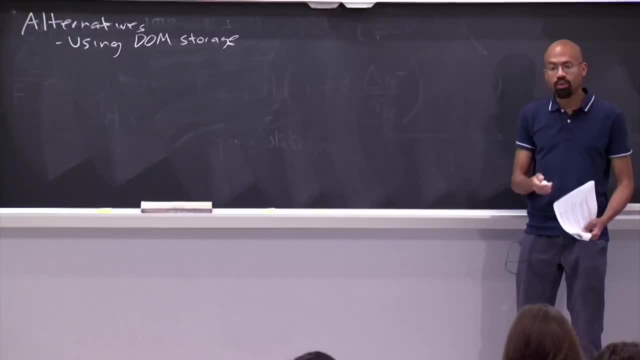 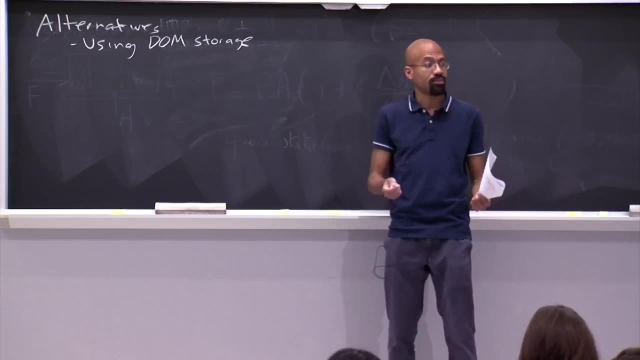 to hold some of that session state that you would ordinarily put inside of a cookie. So, if you remember from last lecture, DOM storage is essentially a key value interface that the browser provides to each origin right. So you can just say get and put and both the key. 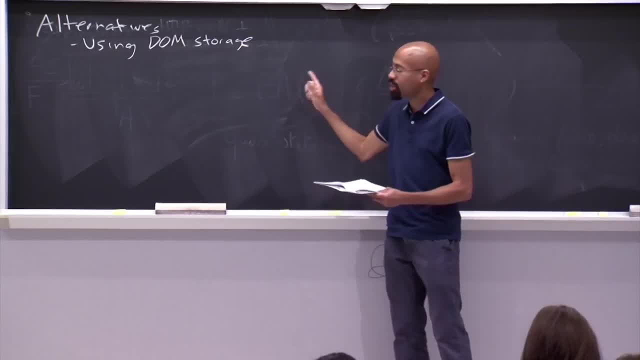 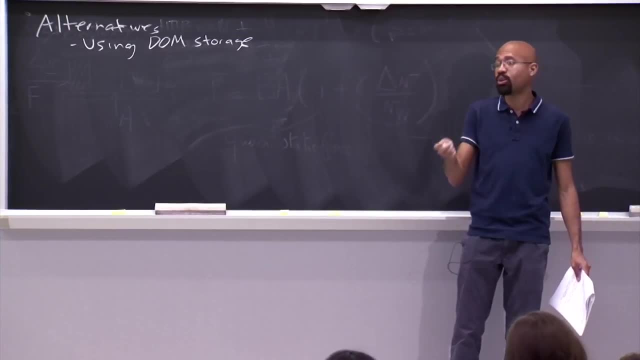 and the value are strings right, So you can imagine putting your authentication stuff inside there. What's interesting about this is that DOM storage actually has much less wacky rules with respect to the same origin policy. So if you remember cookies, you can do all these tricks. 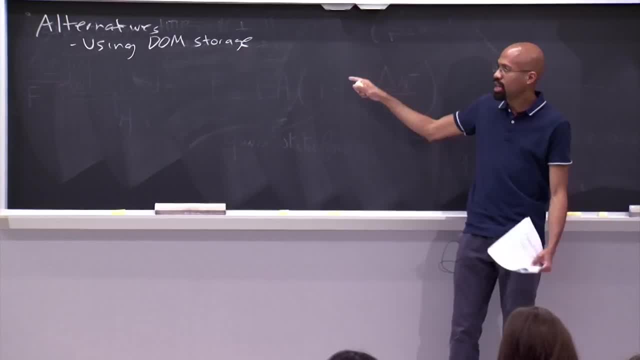 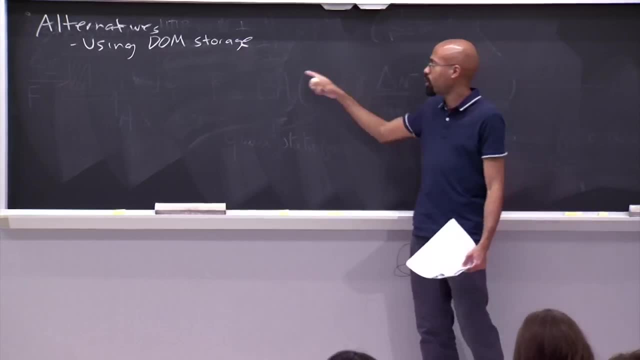 with subdomains and stuff like that, It got kind of weird. DOM storage is actually strictly tied to a single origin. You can't do any of this subdomain expansion or all that kind of stuff, And so frameworks like Meteor use DOM storage for this very reason. 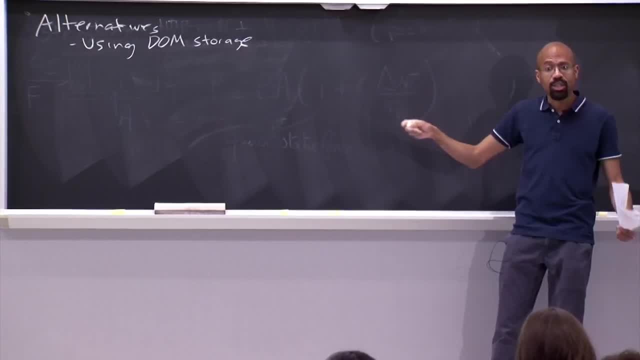 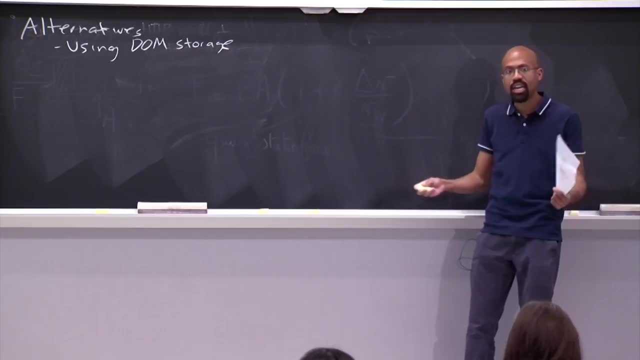 But now note that if you want to store authentication information in DOM storage, then you have to write JavaScript code yourself to actually pass that authentication information to the server to do any crypto that's necessary, so on and so forth. So that's one thing you could do. 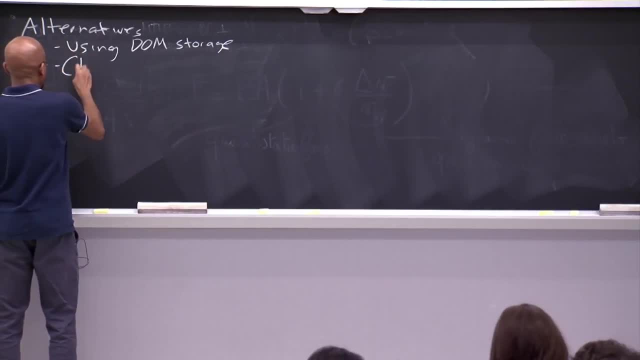 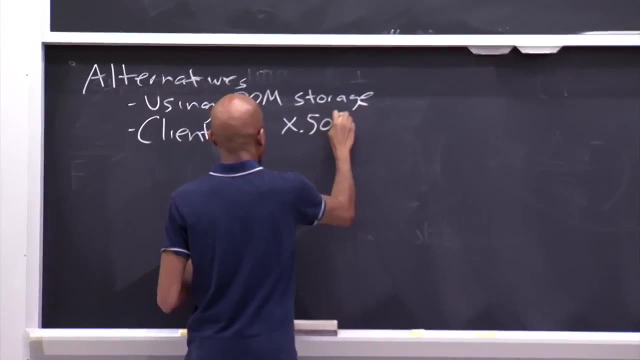 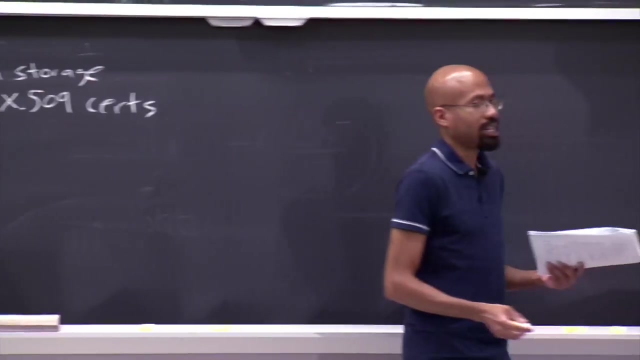 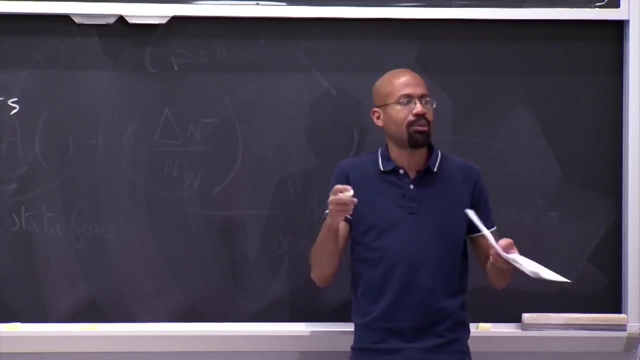 Another thing that you could do is actually use client-side certificates, So, for example, like in X.509 format, And so what's nice about these certificates is that, basically, JavaScript has no explicit interface to access these things. So, unlike cookies, There's always this arms race to find these weird. same origin. 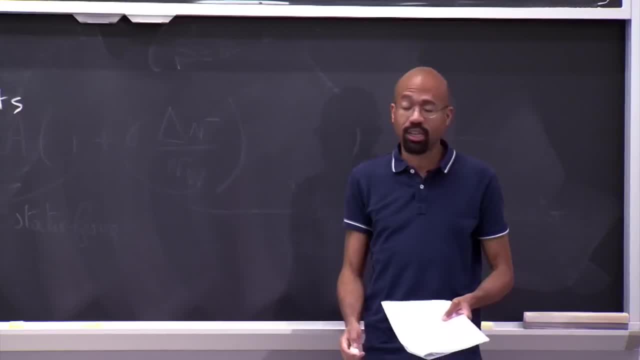 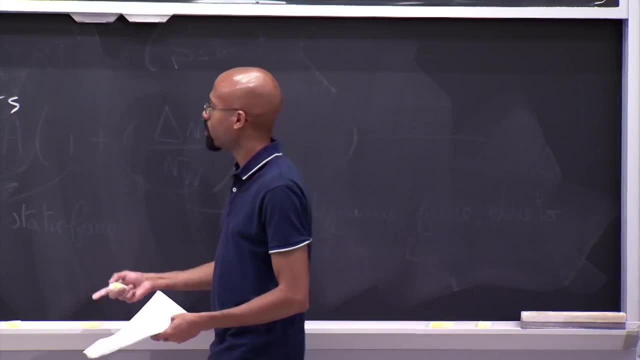 bugs. There's no explicit JavaScript interface for that stuff, So that's very nice from a security perspective. One problem that I mentioned very briefly that we'll look at in more detail in later lectures- is that the revocation story is kind of hard for these. 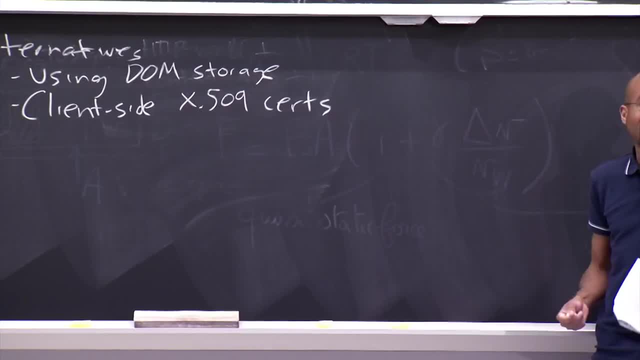 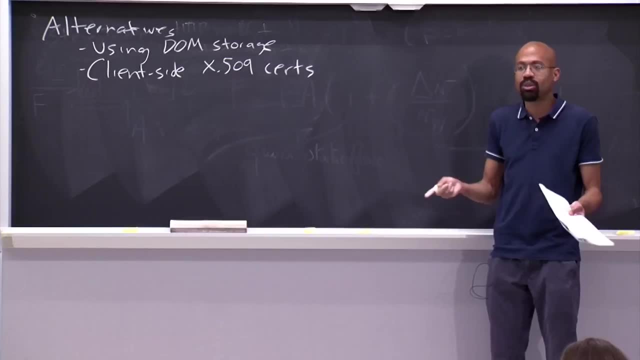 So once a user leaves your organization, how do you take back their certificates? It becomes a little bit tricky. Also, these things don't have great usability, Because who wants to install a bunch of certificates for each site that you go to? So, as a result, these things have a lot of friction. 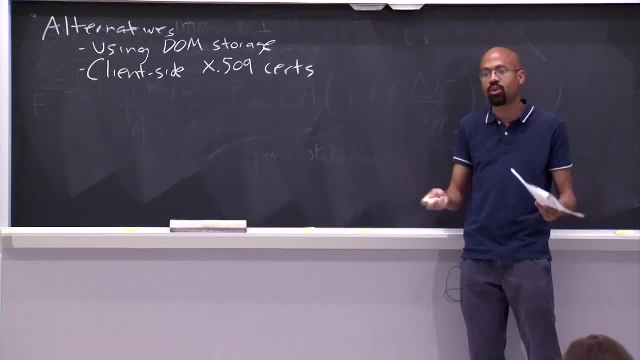 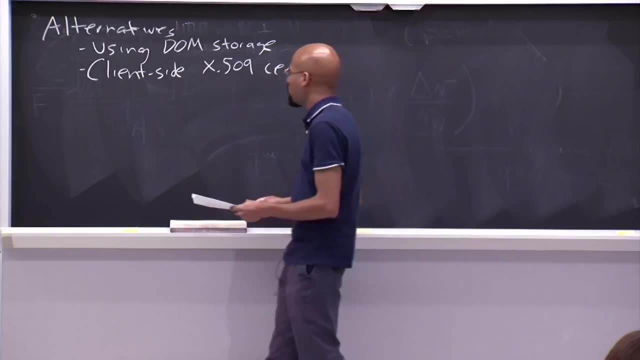 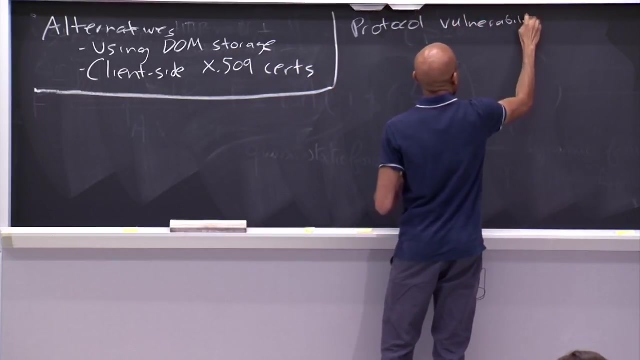 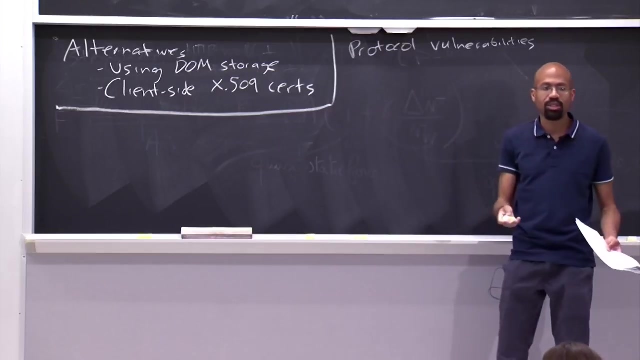 And these are not super popular, except in companies or organizations that are super security conscious. So that concludes our discussion of cookies, And so now let's talk about protocol vulnerabilities in the web stack, And so one kind of interesting attack is that there are all these sort of bugs in the way. 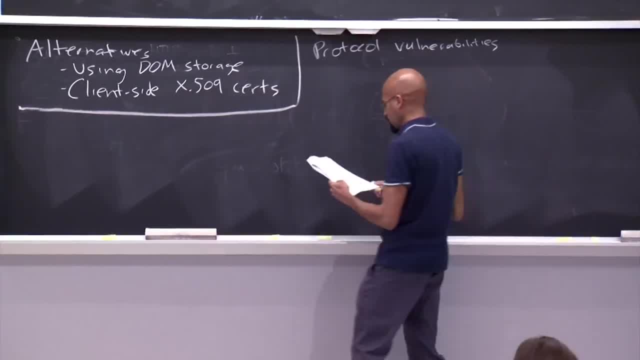 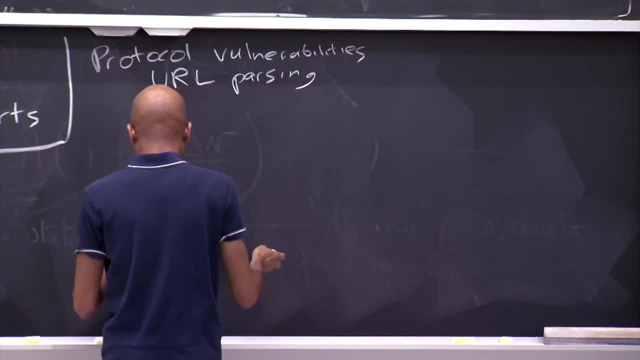 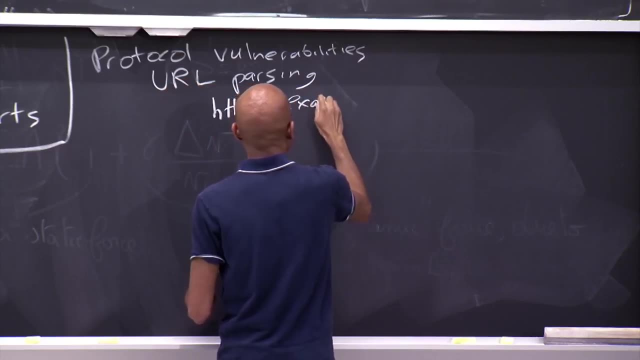 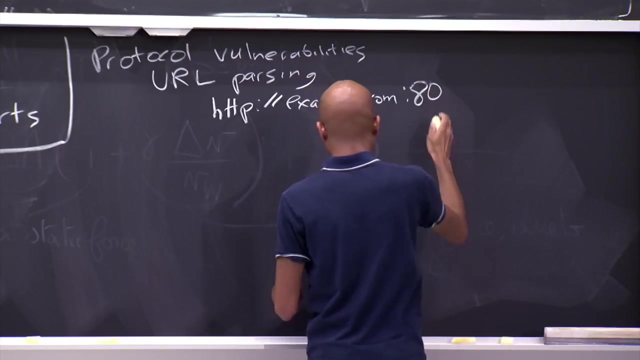 that different browser components parse URLs, for example. So how can URL parsing get us into trouble? So suppose that you have a URL that looks like this: HTTP comes from examplecom and then it's got an explicit port that specifies of 80.. 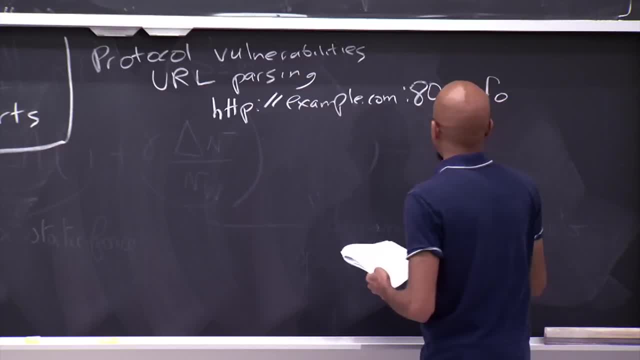 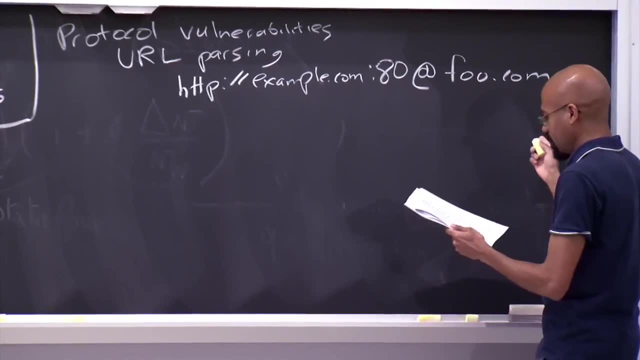 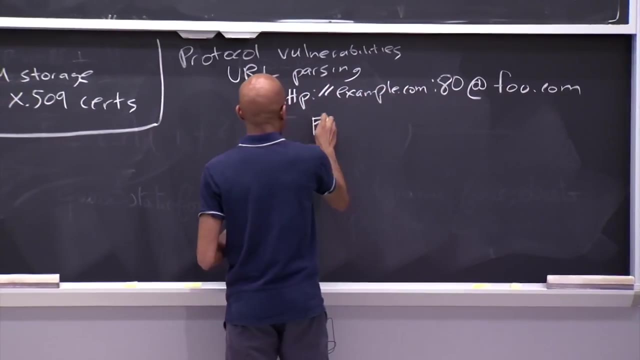 And then, for some unknown reason, it embeds this at character here. So the question is: well, what is the origin of this particular URL? So, as it turns out, so Flash would say: well, this is a URL, This is a URL. 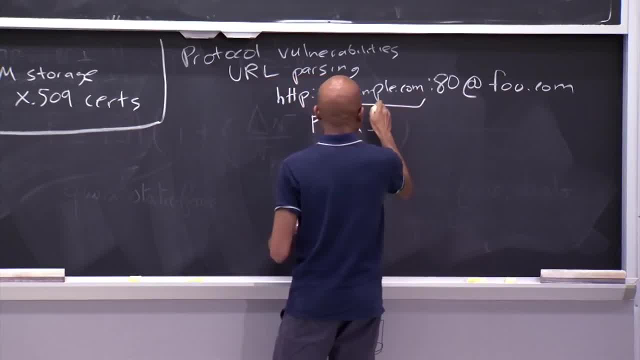 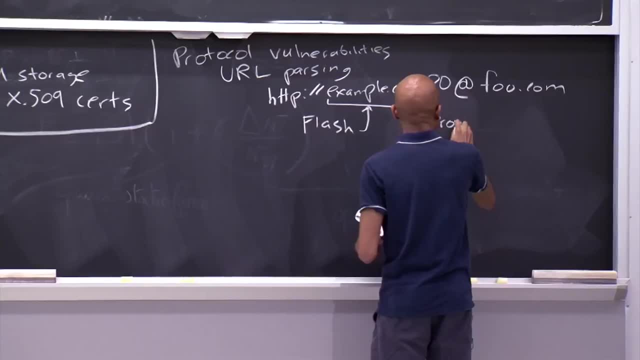 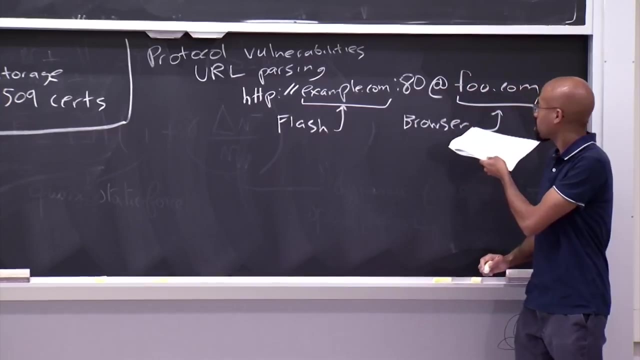 So it would say that the hostname portion of this was examplecom. However, when the browser would parse this, it would say that the hostname part of the origin was actually foocom. So this is clearly a bad thing, Because once you have two different entities, who? 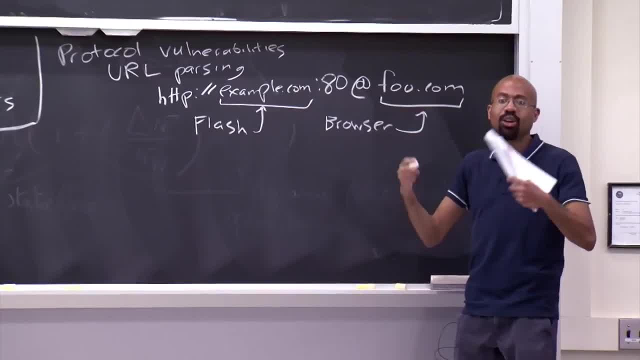 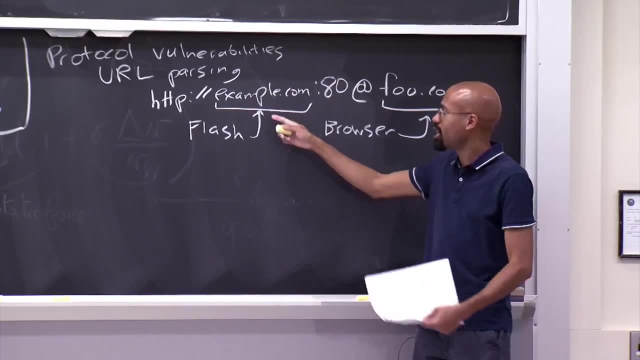 are confused about the origin of the same resource, then you can get into all kinds of nasty problems. So, for example, Flash. The Flash code could be malicious. It could download stuff from examplecom If it was embedded in a page from foocom. 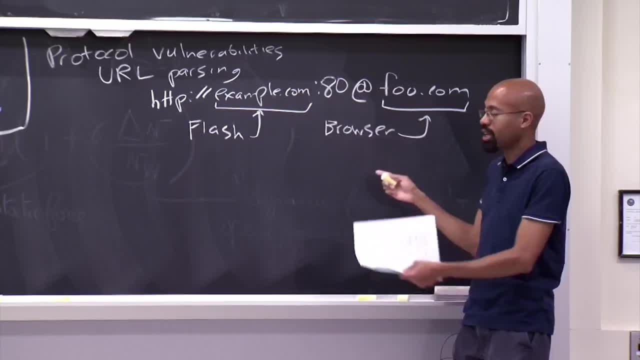 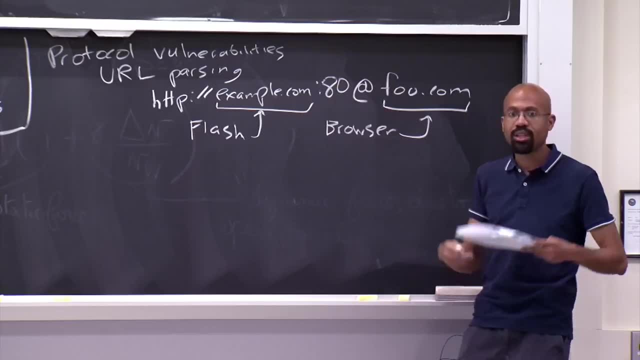 it could then do some evil things there, Take some code from examplecom and run it with the authority of foocom. So there's a lot of complex parsing rules like that that make life very difficult. This is a continuing theme, like as we just 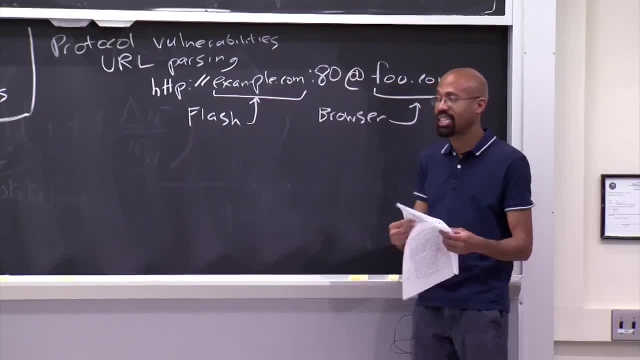 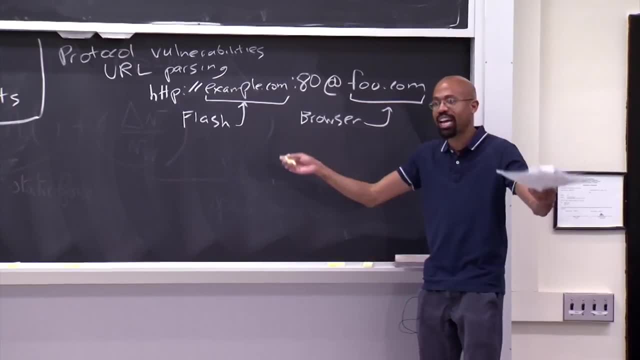 saw with the content sanitization. So the basic idea is that it's oftentimes much better to have simpler parsing rules for this kind of stuff. It's difficult to do that in retrospect, though, because HTML is already out there. so all aboard the Wambulance. 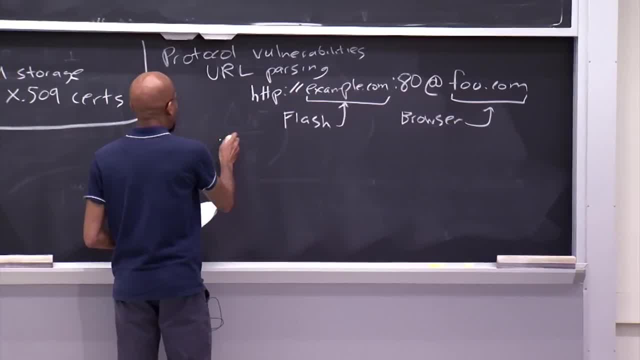 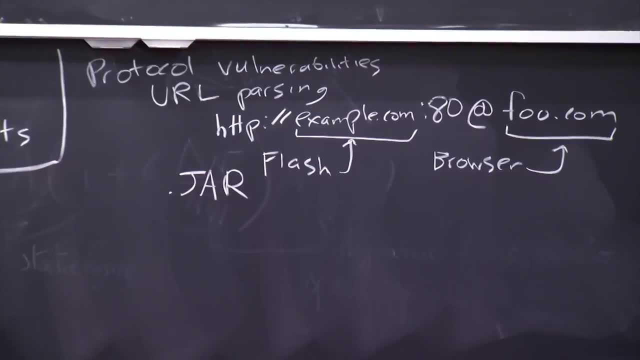 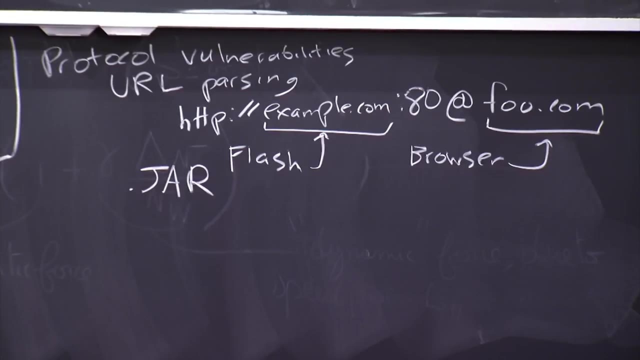 So this next one. this is actually my all-time favorite security vulnerability. So it basically attacks the way that the browser will run JAR files, basically Java applets. So in 2007, I think, yeah, 2007,. so lifehackercom. 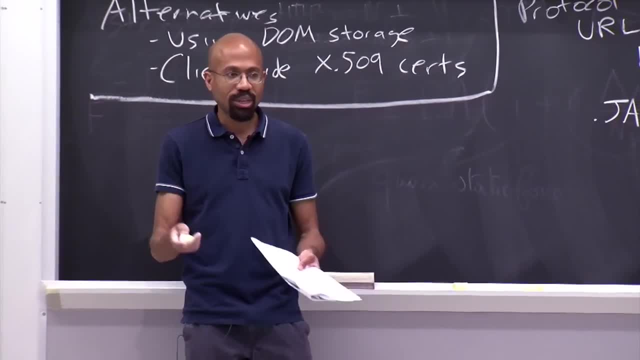 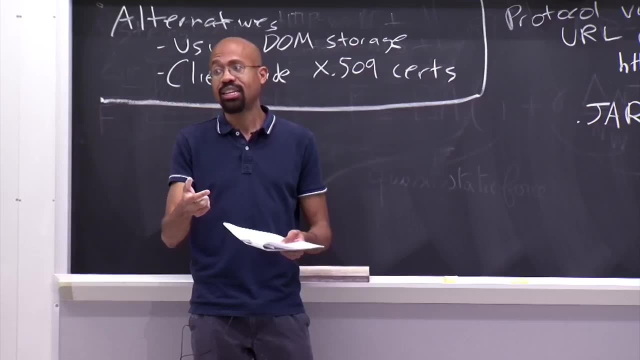 great website if you haven't been to it. lifehackercom com. com basically explains how you can embed zip files inside of images. Now, it's not quite clear who you're trying to hide from by doing this, but lifehacker says you can do it, so hooray. 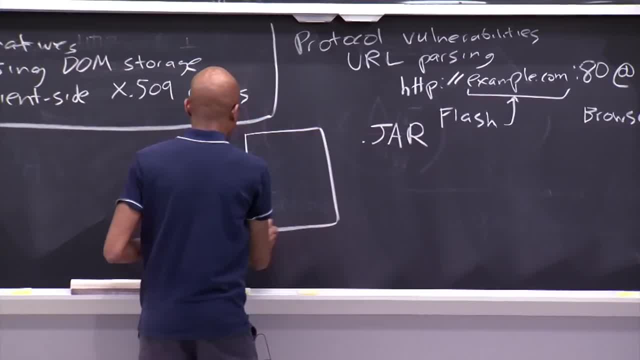 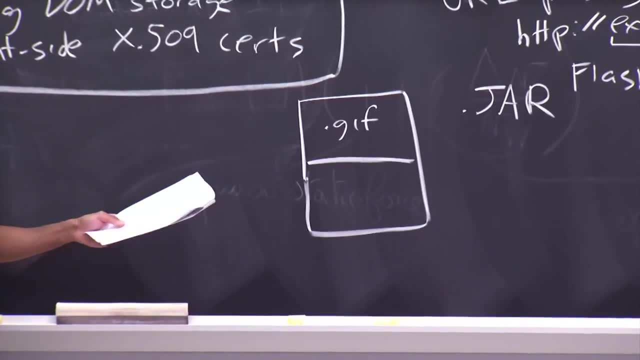 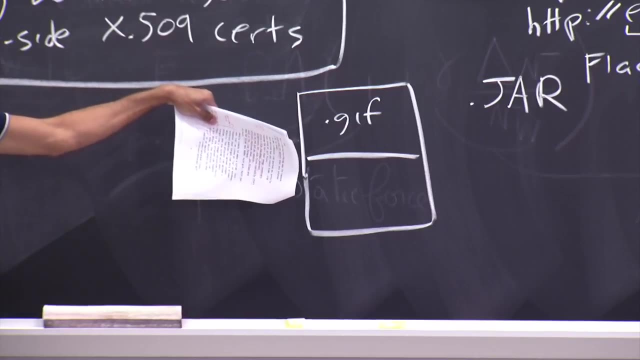 So basically, what they take advantage of is the fact that if you look at image formats like GIF, for example, typically the way the parser works is the parser works from the top down, So it finds information in the header and then it sort of computes on the rest of the bits here. 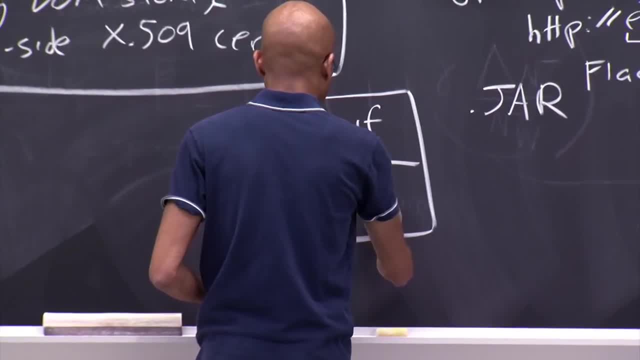 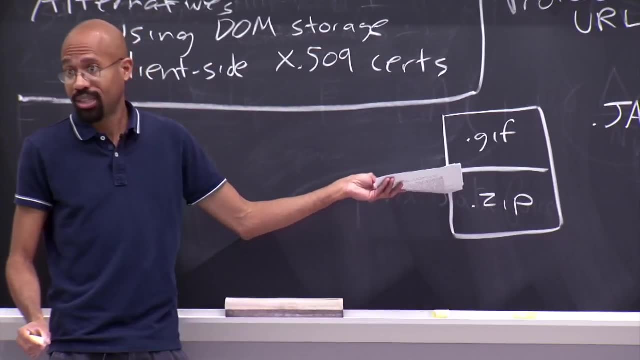 Now, what was interesting is that, as it turns out, programs which manipulate zip files typically work from the bottom up, So they find some information in the footer of the file, then they work up to try to extract what's inside of it. 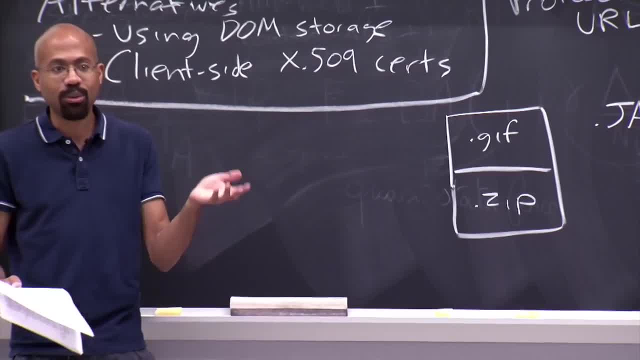 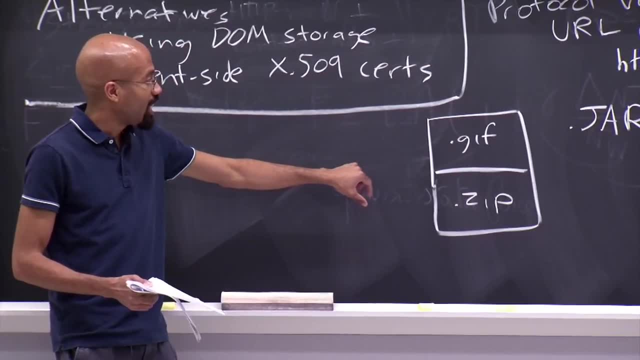 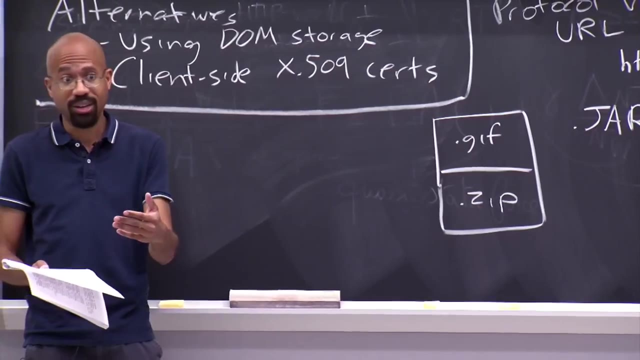 So what lifehacker basically said is that if you wanted to hide a zip file on a merger or something like this, then you could actually post a GIF there, right? So if you have a file that has this zip file here, it will pass all the validation checks on Flickr or whatever. 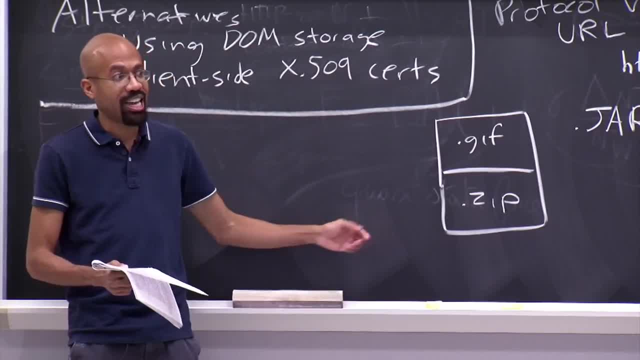 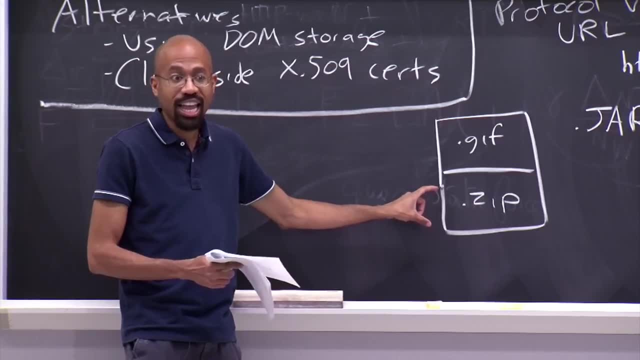 as an image. It will actually display as an image in your browser. Aha, but only you know the hidden truth that if you take this file here, you can pass it to unzip and it will unzip. You will actually get information there. 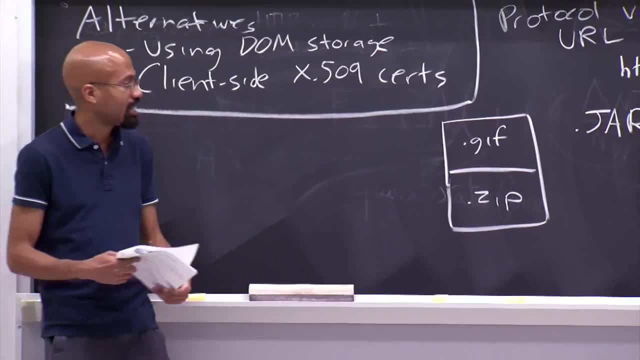 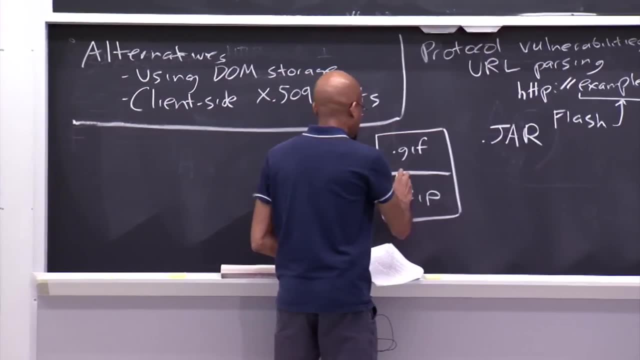 OK, fine, This seems like a cheap parlor trick. OK, that's nice. Now attackers, of course, never sleep and they want to ruin our life. So what did they realize They realized? They realized that JAR files are basically. 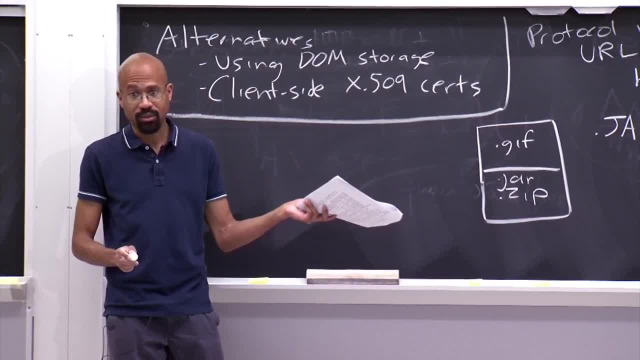 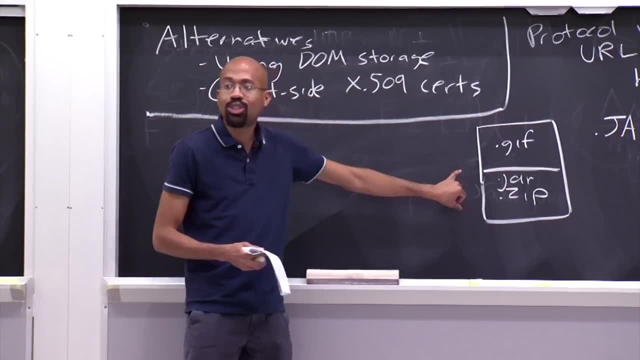 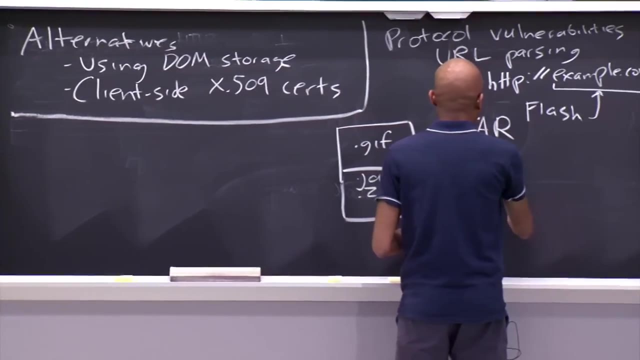 derivatives of the zip format, right. So this meant that you could actually create a GIF or an image that had a JAR file, executable JavaScript code at the bottom of it. OK, and so then people called this attack. they called it the GIFAR attack. 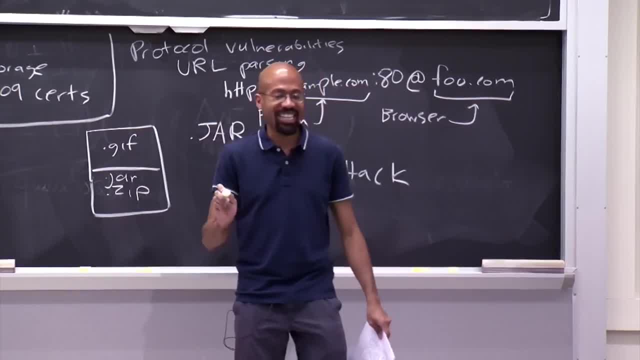 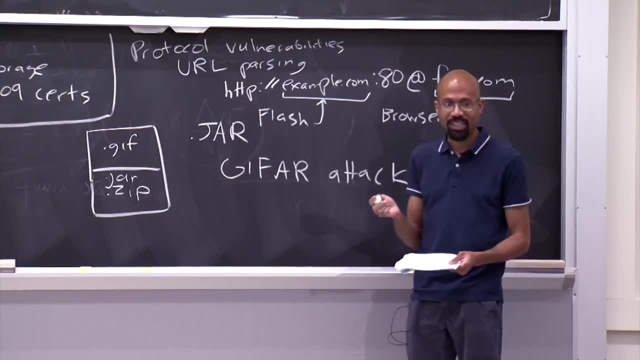 Half GIF, half JAR, all evil, And so this was amazing. And so what did this mean that you could do? Well, it's actually quite subtle, Because people first discovered this they thought it was amazing, but they didn't quite. 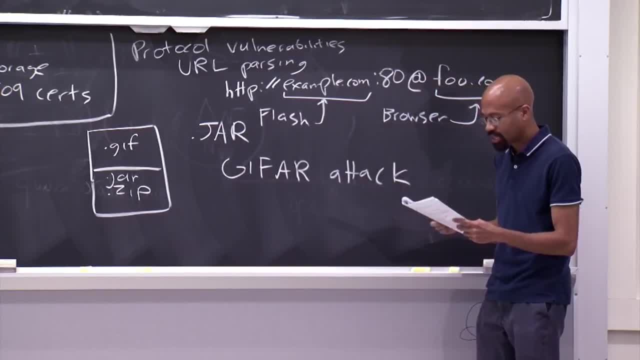 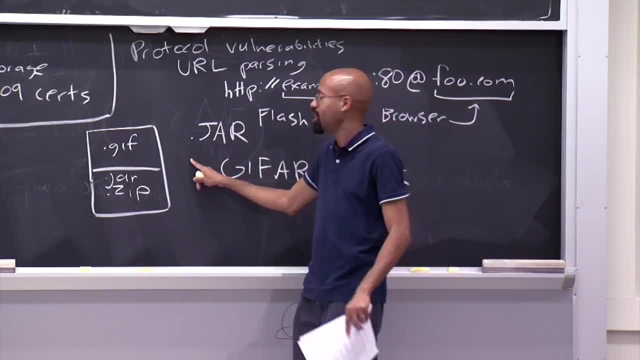 know how to exploit it right, But as it turns out, you can do things like the following. So, first of all, how do you make one of these things? You just use cat. There's literally no trickeration you have to do. 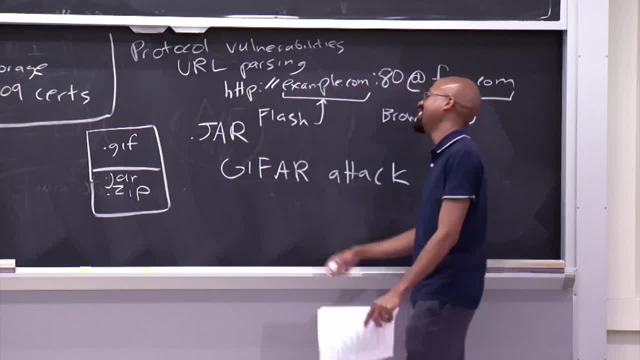 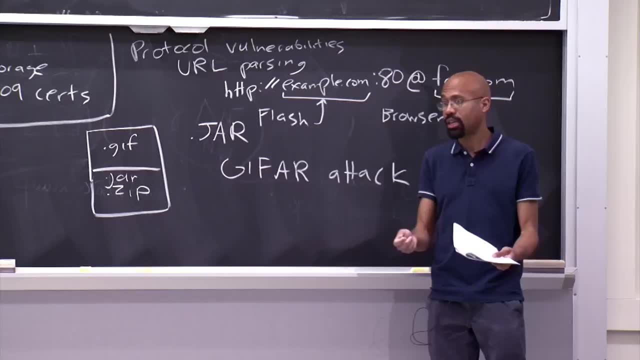 Take this, take this, you cat it, boom, You've got a GIF jar. So once you have that, what can you do? Well, there are some sensitive sites that will allow you to to submit data, but not arbitrary types of data. 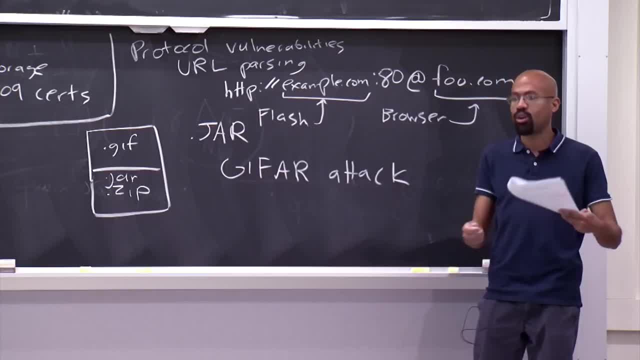 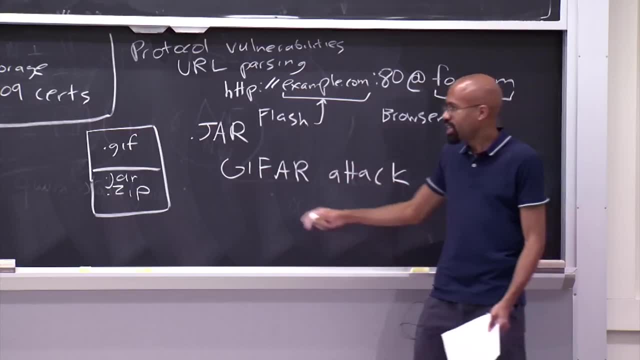 So, like, for example, Flickr or something like that, It may not allow you to submit arbitrary ActiveX or whatever arbitrary HTML, but it will allow you to submit images. So what you could do is construct one of these things, submit it to one of these sensitive sites. 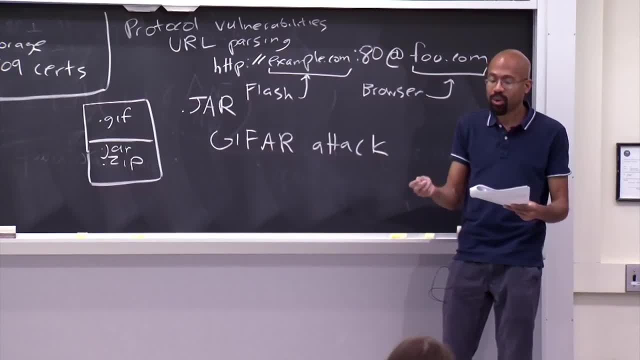 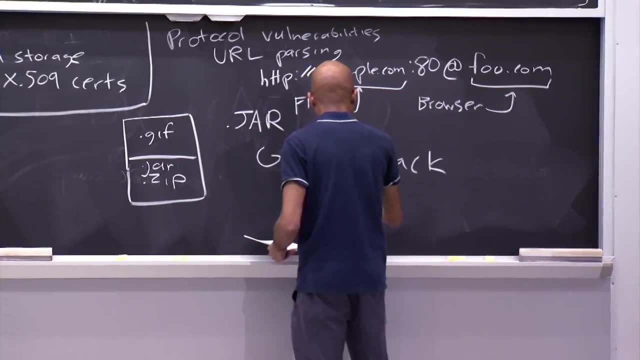 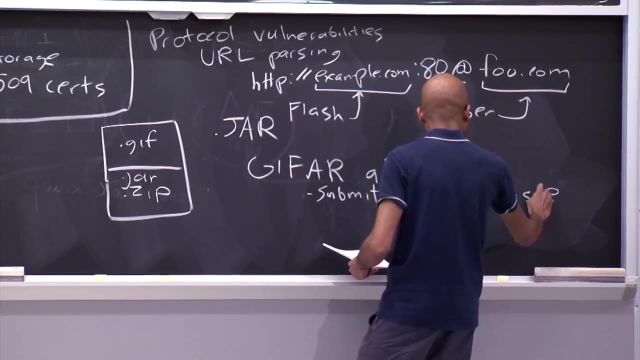 that does allow you to submit images. And then, what can you do? Well, the next thing that you need to do is: so, yes, the first thing you do is you Submit one of these things to the sensitive site, And then the next thing that you can do is: 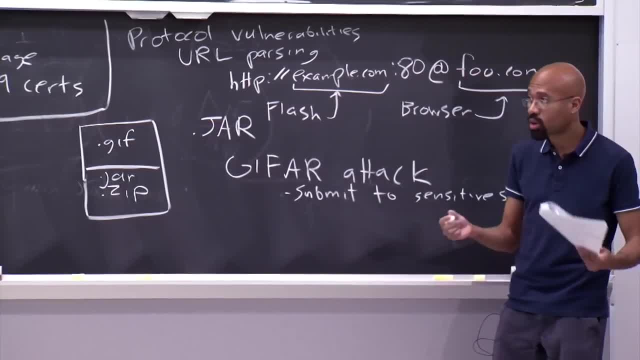 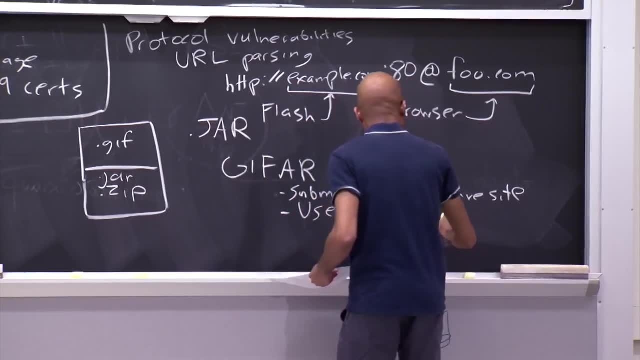 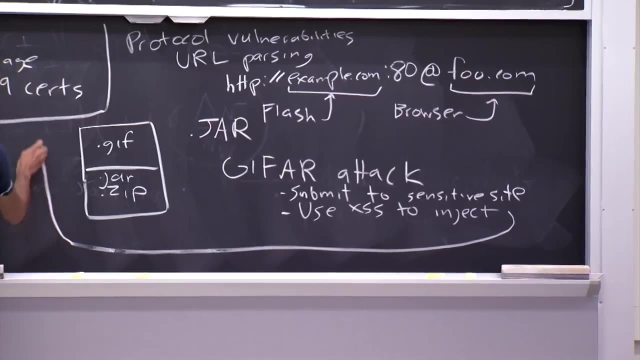 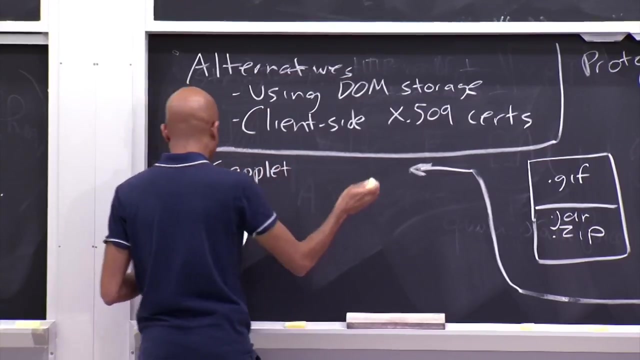 if you have a XSS attack, if you have a cross-site vulnerability, then you can use cross-site scripting to inject something like this And, due to poor board management, I will draw this over here, So you can inject an applet JavaScript code: 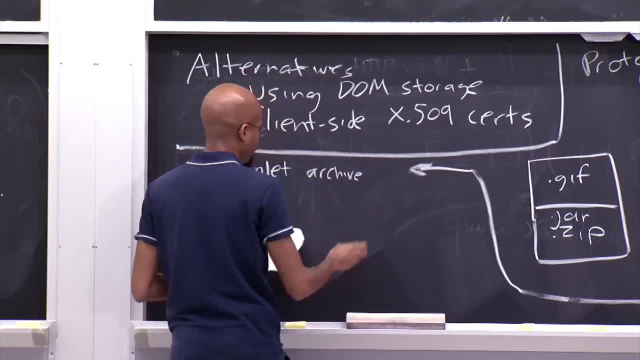 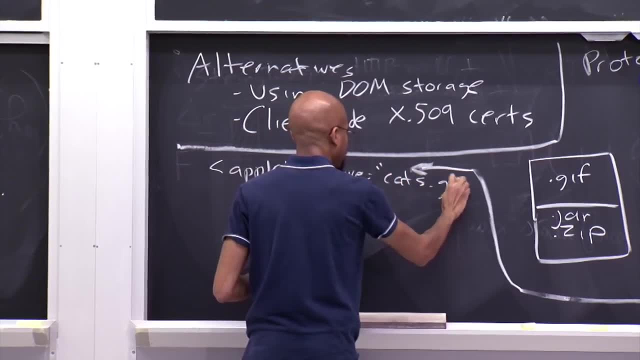 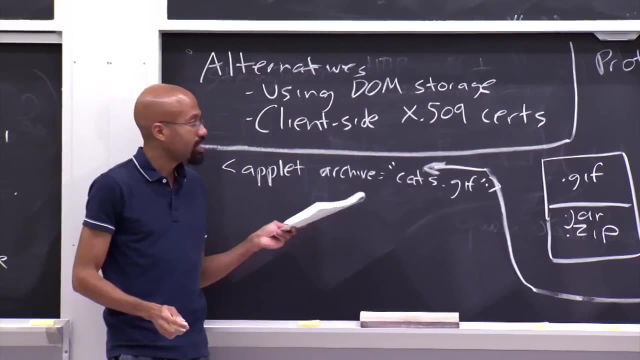 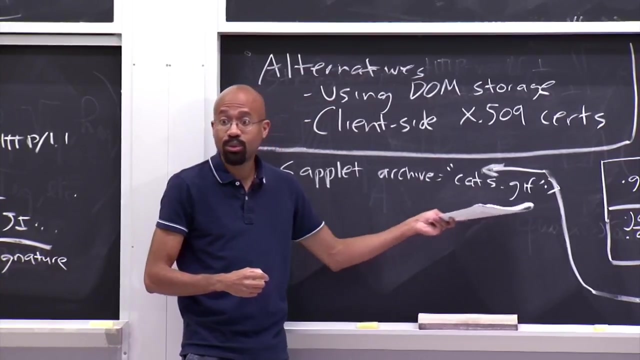 that has as its sort of source, you just say catsgif, And so what's interesting about this is that this code, because we're using a cross-site scripting vulnerability, runs in the context of the vulnerable site, Right, Right, then uploaded to the vulnerable site's origin. 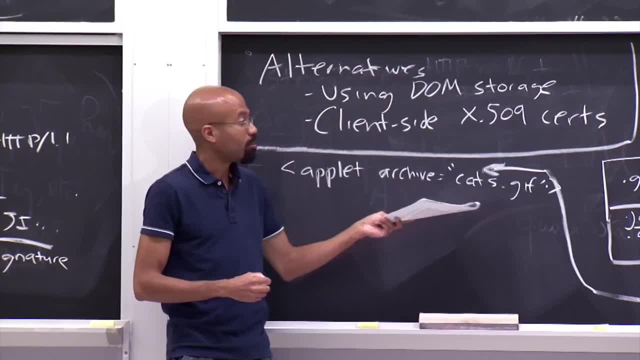 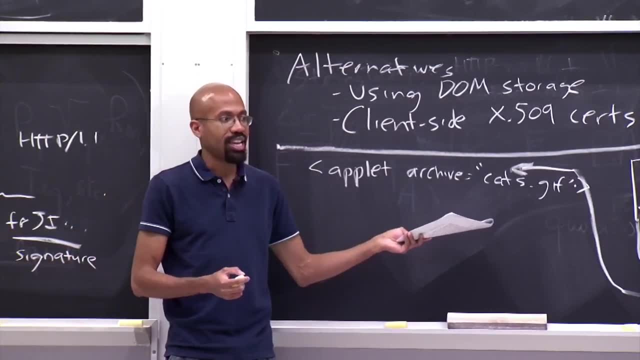 So this will pass the same origin test, right. But however, this code was specified by the attacker, And so now what's happened is that the attacker gets to run that Java applet in the context of the victim site, with all the authority of that origin. 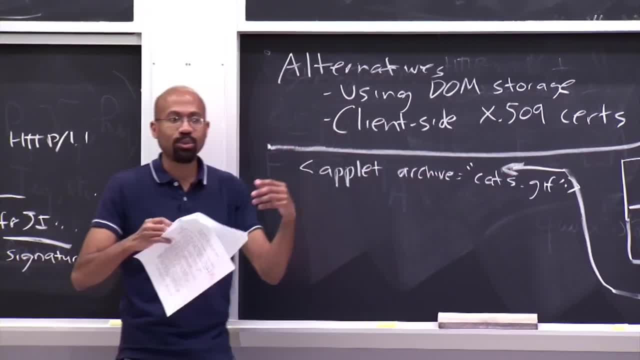 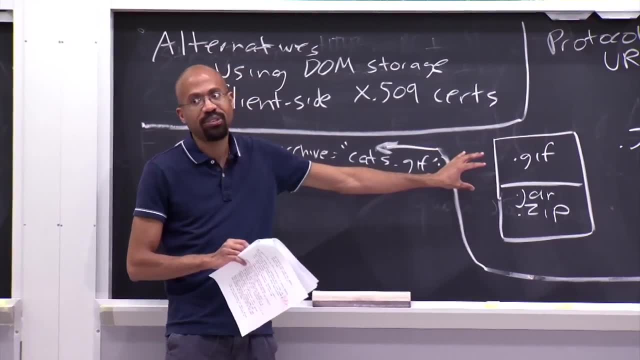 even though the Jifar passed the vulnerable site's image validation code right, Because one of these things will actually parse correctly as a GIF, right, But it has this hidden code in here And so, as a result, when the browser tries to execute the jar part of it once again. 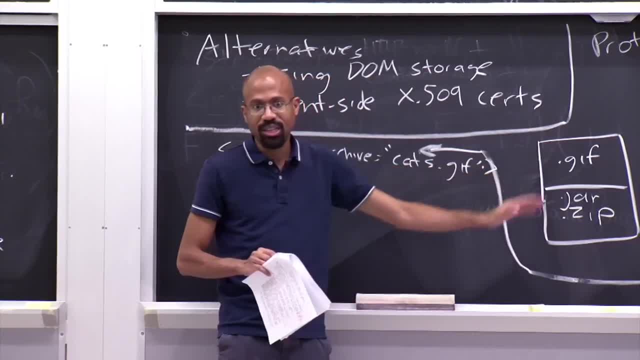 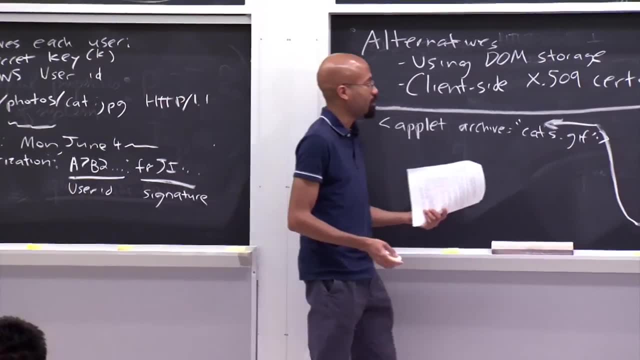 it starts at the bottom, comes up here and just ignores that part, right? So this is actually pretty amazing, right? And so there's some fairly straightforward ways you can fix something like this. So, for example, you can actually have the applet loader actually. 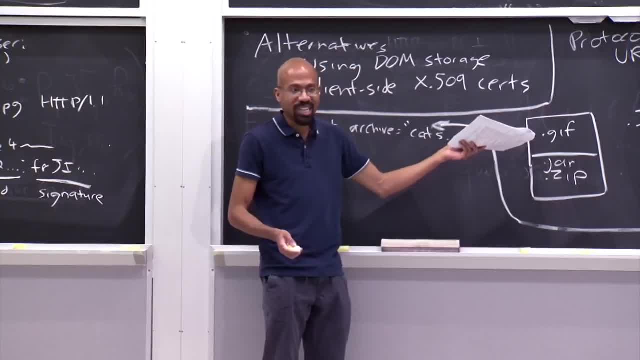 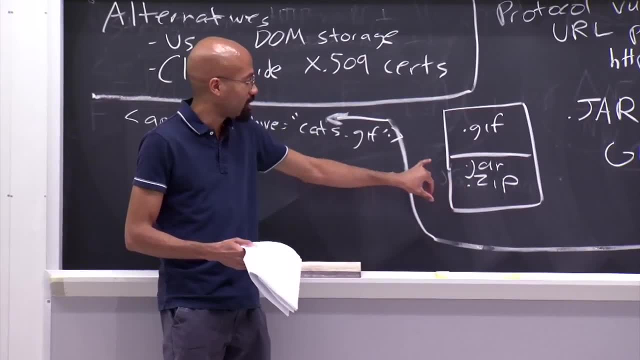 understand that there should not be random junk up here. for example, What was happening in many cases is that there was information in the metadata saying here's the length of this resource And then if it said the length is just, it stops here. 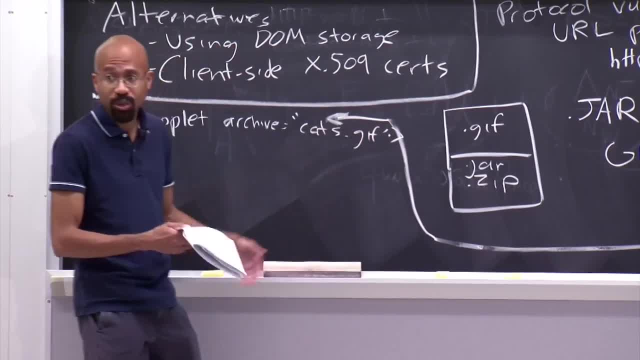 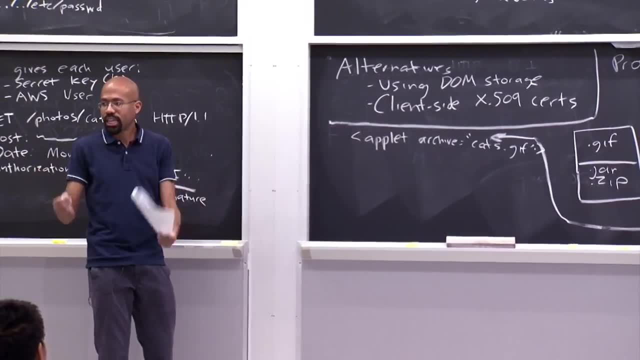 they would just say: who cares what's at the rest? It's probably zero, But in this case it wasn't, And so what I love about this is that it really shows how wide the software stack is for the web, right. 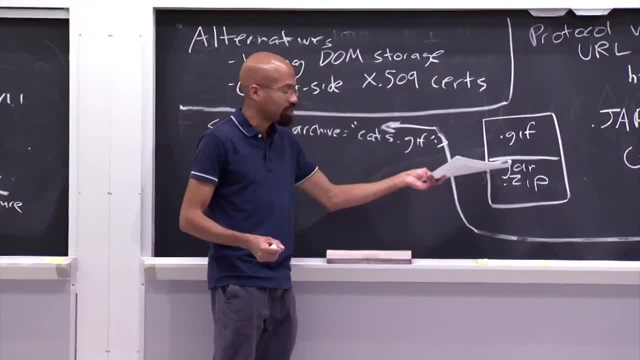 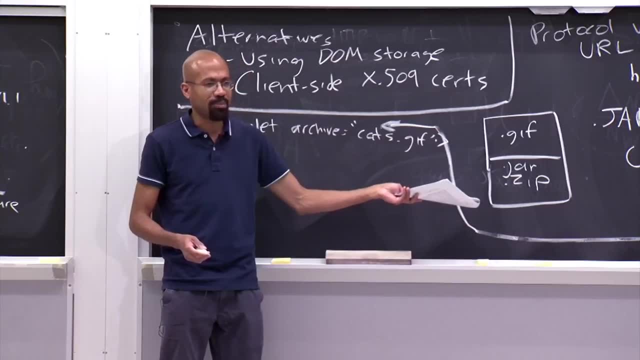 So sort of taking these two formats, GIF and then jar, we can actually create this really nasty attack, And you can actually do this for PDFs too. You can put PDFs here. I think that was called the PDFR attack or something like this. 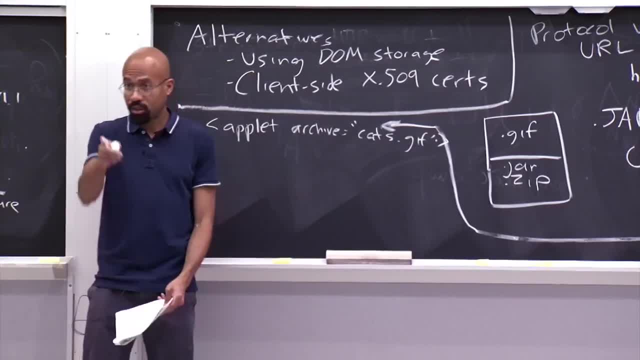 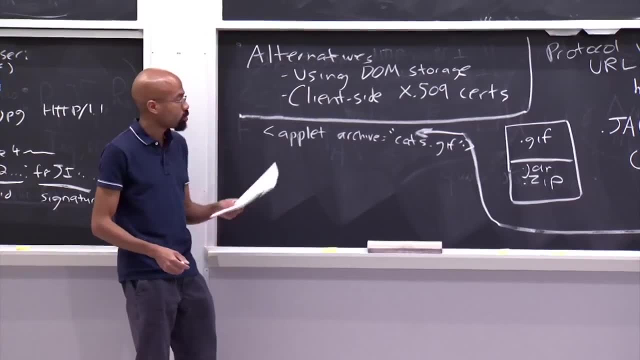 So people had a. They had a field day with this for a bit. These vulnerabilities have been closed down. So what can you do with this attack that you can't do with either the XSS or your own? So what's nice about this is that Java oftentimes 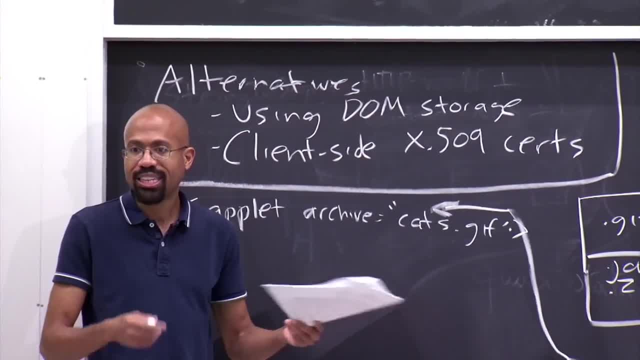 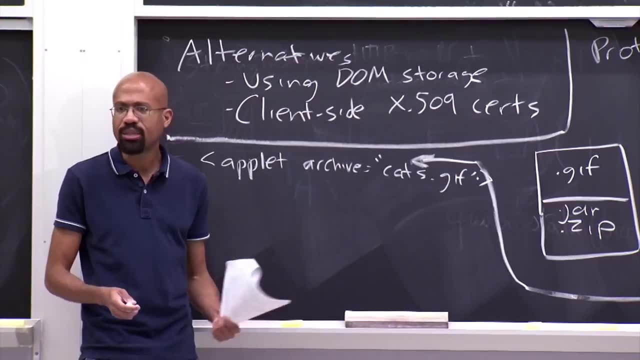 can be more powerful than just running regular JavaScript Because it has slightly different rules on same origin policy and stuff like that And sometimes you can get more lower level access to the file systems or things like that. But you're right that I mean if you can do cross-site scripting. 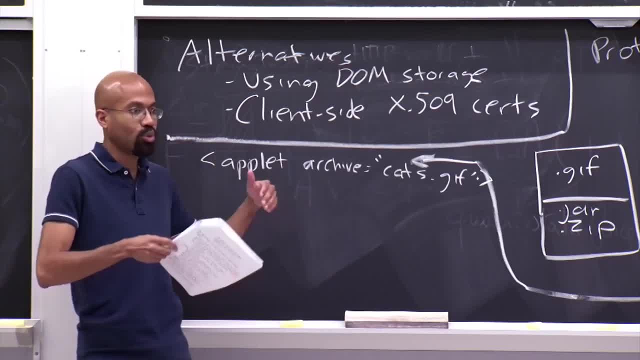 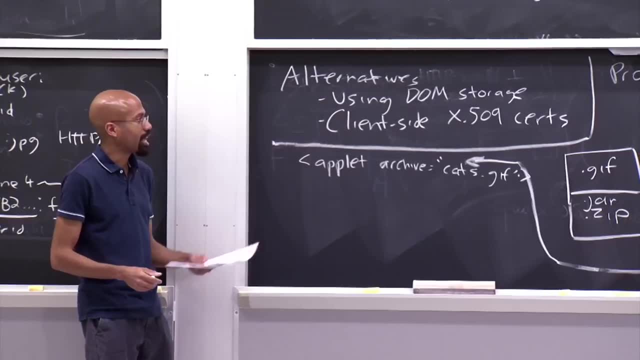 running JavaScript is already pretty damaging, But the main advantage of this is once again running inside the applet. All right, Yeah, so, like I said, that's my favorite attack of all time, Mainly just because it forced serious minded security. 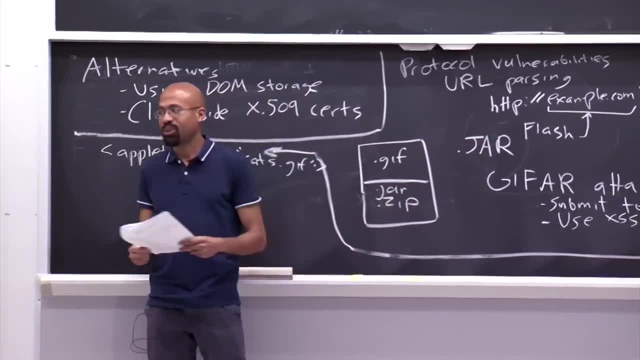 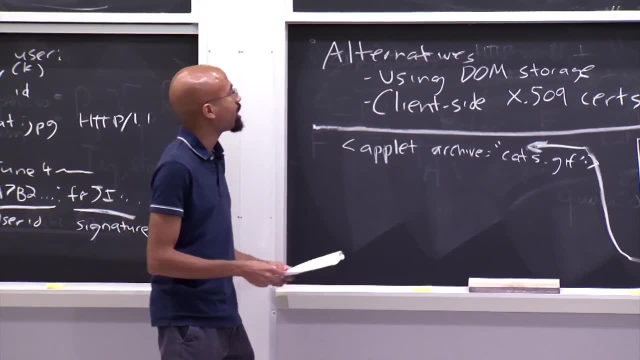 individuals to say GIFR all the time. So if you're easily amused, like myself, then this was a bonanza for you. So another thing that's interesting is that there are actually attacks that I don't know. I don't know if you've heard of it, but there are actually attacks that 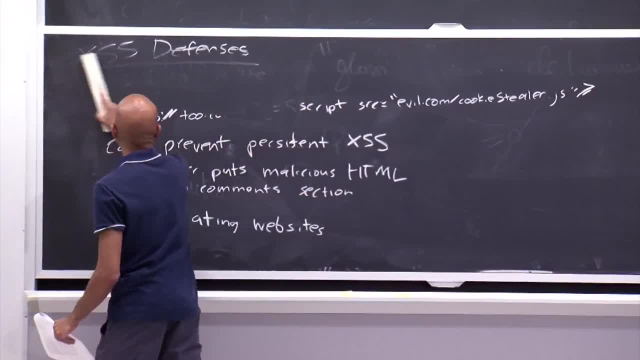 I don't know if you've heard of it, but there are actually attacks that. I don't know if you've heard of it, but there are actually attacks that that are based on time, right, So you might not think of time as a resource which. 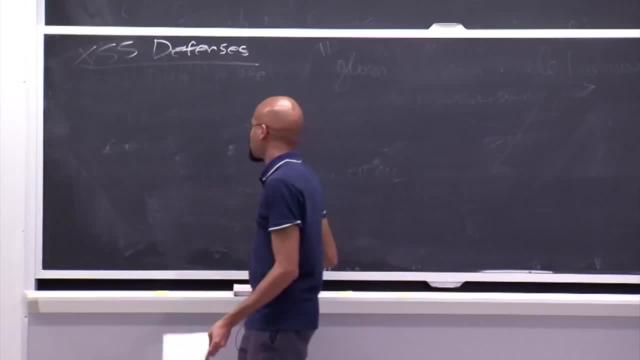 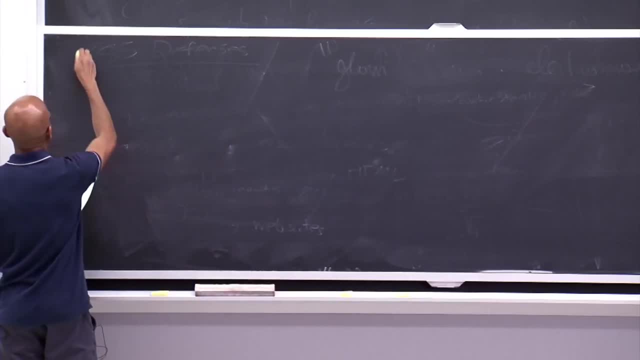 could be a vector for attacks, But, as I was discussing with someone a few minutes ago, yeah, time can actually be a way that a system can be exploited, And so these attacks are called. the particular attack I'm going to talk to you about is a specific example. 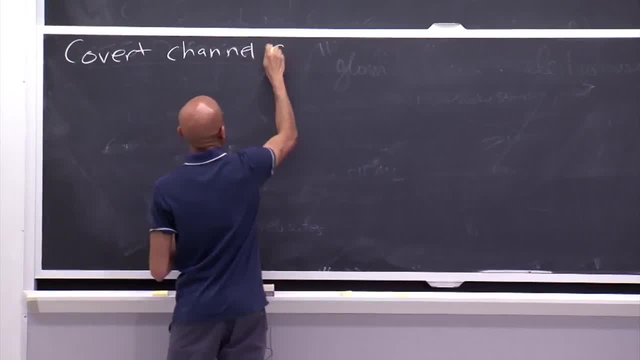 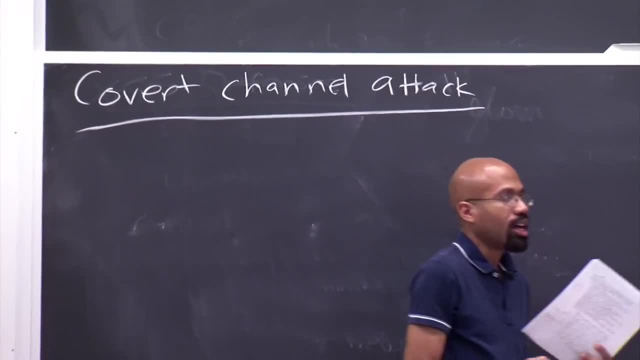 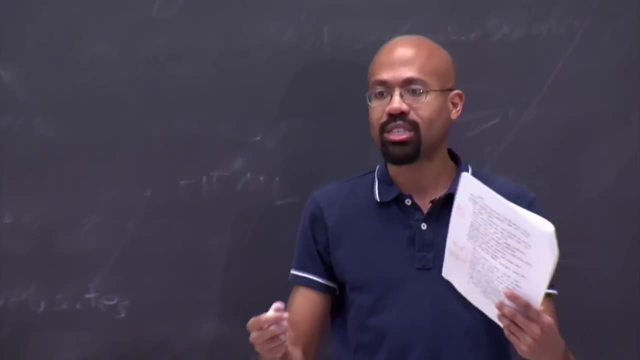 of a covert channel attack, And so the idea behind a covert channel attack is that essentially the attacker has found some way for two applications to exchange information, And that exchange vector is not sort of an officially sanction vector. The attacker is somehow leveraging some other part of the system. 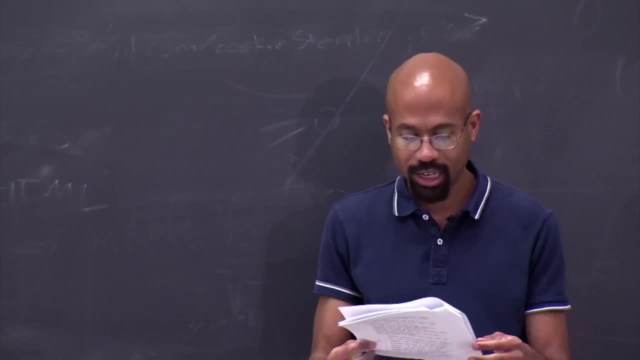 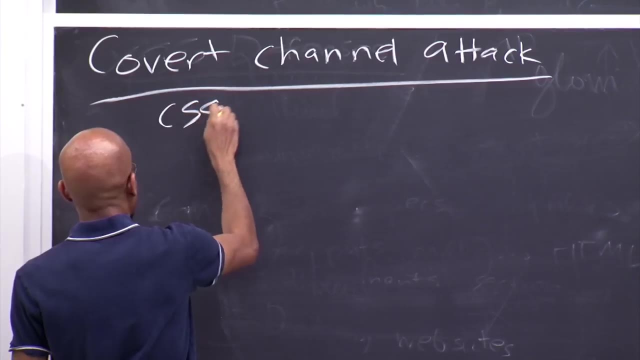 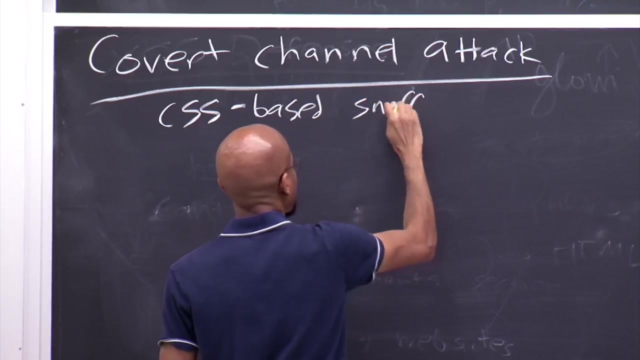 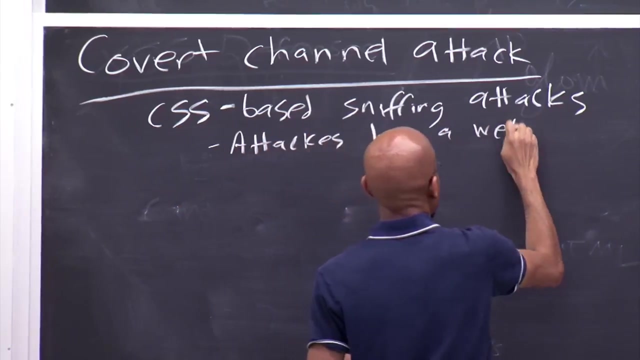 to pass bits of information between two different entities. So a good example of some of this stuff is something called CSS-based sniffing attacks. So what is this attack all about? So attacker has a website that the user can visit And once again getting a user to visit a website. 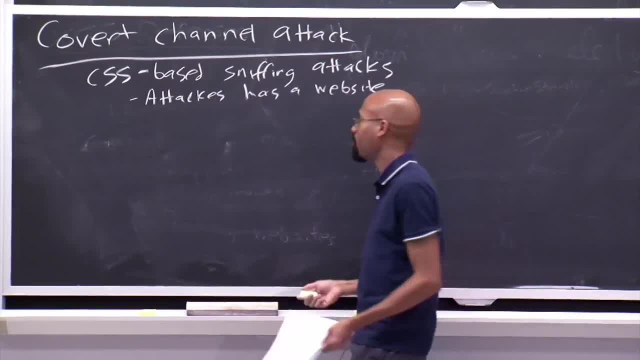 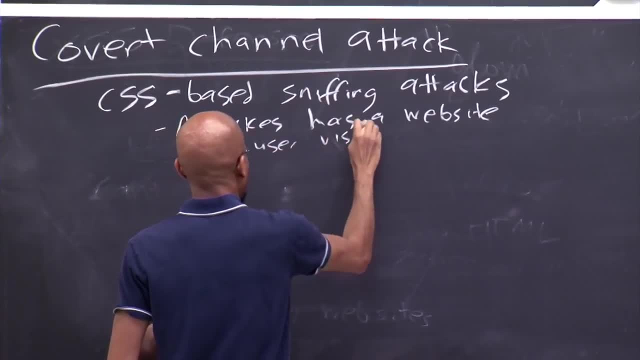 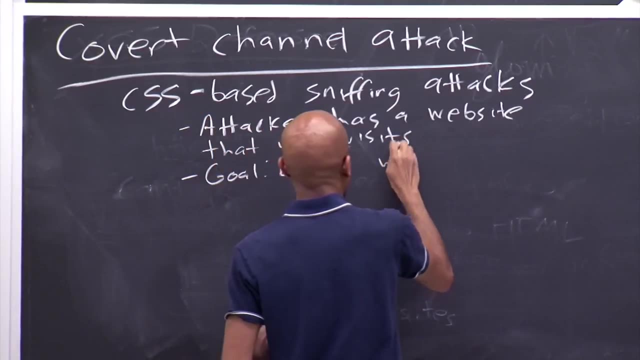 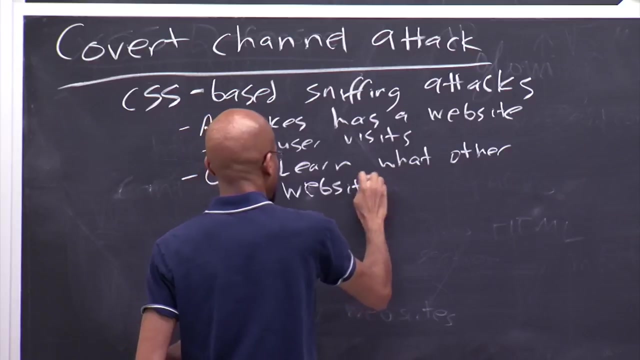 is actually usually pretty straightforward: You create ads, you send them a phishing email, whatever. So the attacker has a website that the user visits, and the goal of the attacker is to learn what other websites the user has visited, And so the attacker might want to know this. 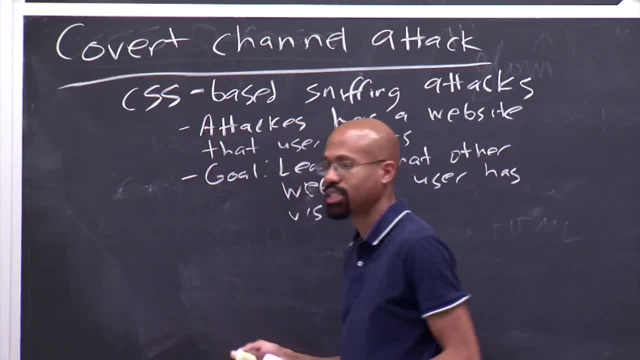 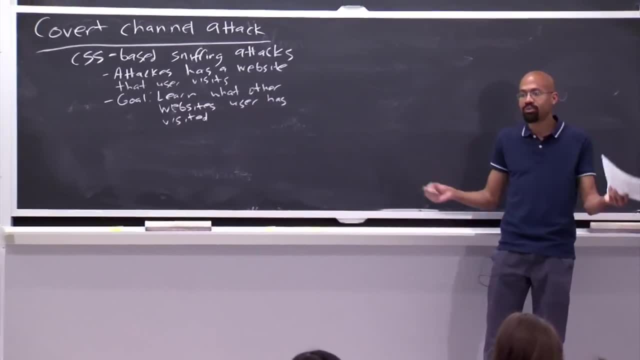 for several reasons. Maybe they're trying to figure out what kinds of search terms the user's looking for. Maybe they're trying to figure out where that person's employed. Maybe they want to know if they've accessed some type of embarrassing material, so on and so forth. 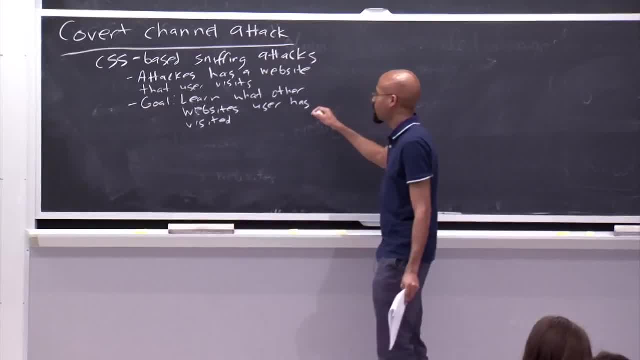 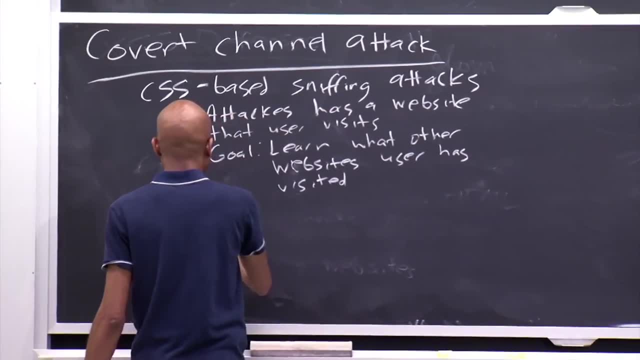 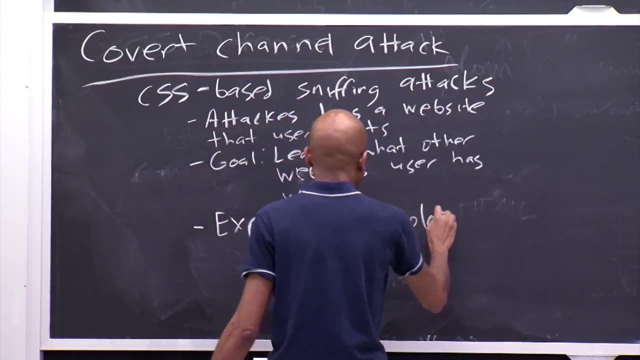 So how is the attacker going to do that? if the only thing that the attacker controls is a website that he or she can convince the user to visit? Well, the exploit is to leverage link colors. So you know when you go to a web page. 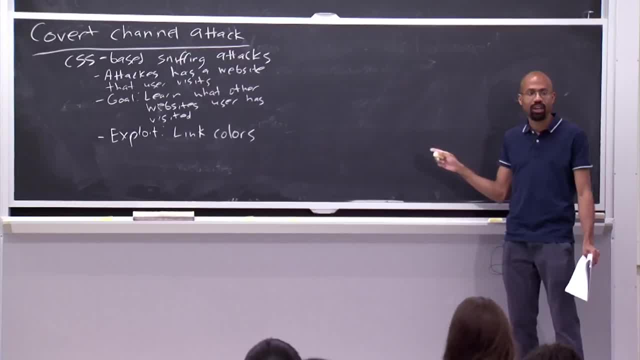 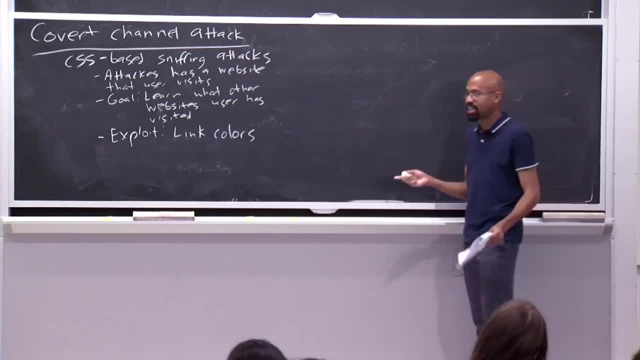 and you click on a link, the next time you see that link, it is now a different color. So, zoinks, That's actually a security vulnerability, Because what that means is that in this attacker website, if the attacker can trick you into visiting it, 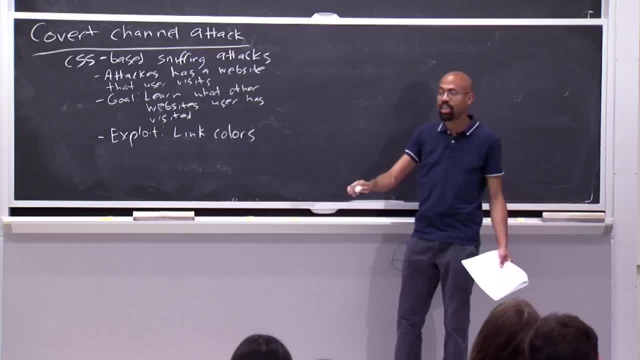 then the attacker can generate a huge list of candidate URLs that you might have visited And then use JavaScript to see what color those URLs are, And if the URL color is purple, then that's very subtle. That means aha, you have visited that site. 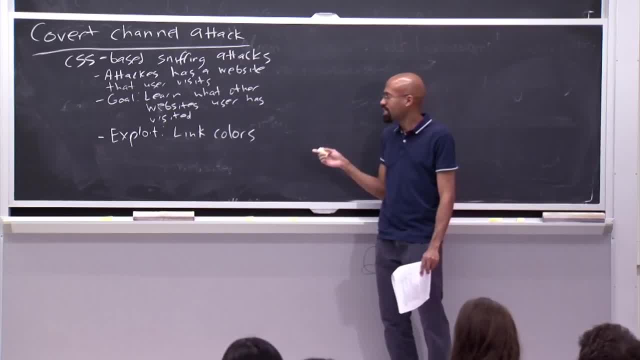 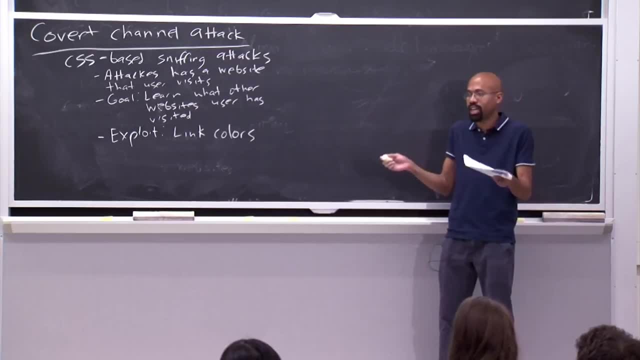 So this was very subtle, And what's interesting about this is that you don't even have to display the URLs in many cases to the user. You can just sort of conjure up a DOM node that has a particular href and then just look at its style. 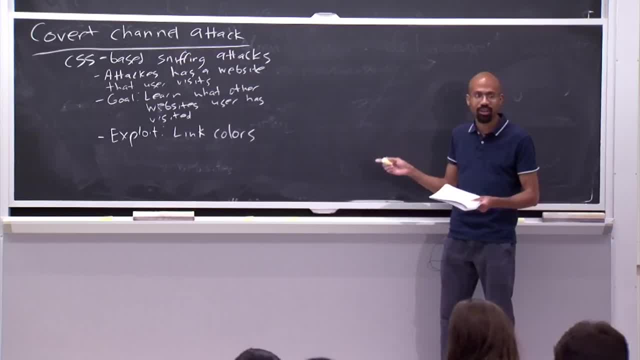 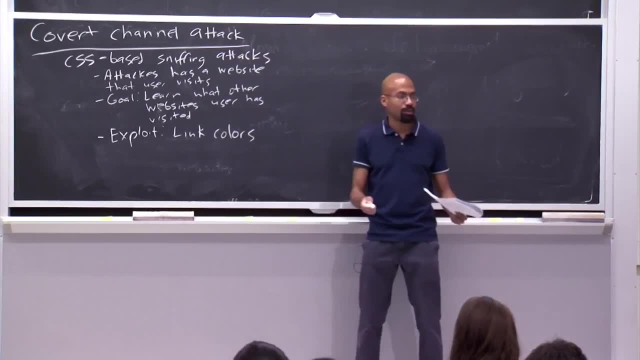 and then see if it has the visited color or not. This is actually pretty subtle, And so you might be thinking: well, but isn't it going to be inefficient to scan through all these candidate URLs? We can do all kinds of clever optimizations. 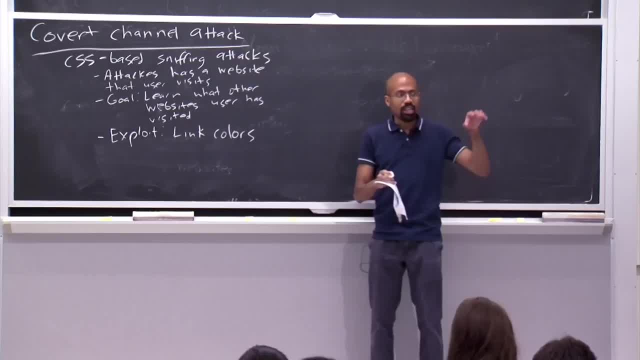 So, for example, you can have multiple URLs, You can have multiple passes. In your first pass, you could only see if the user had visited top-level URLs- cnncom, facebookcom, so on and so forth. If the answer is yes, you can, then 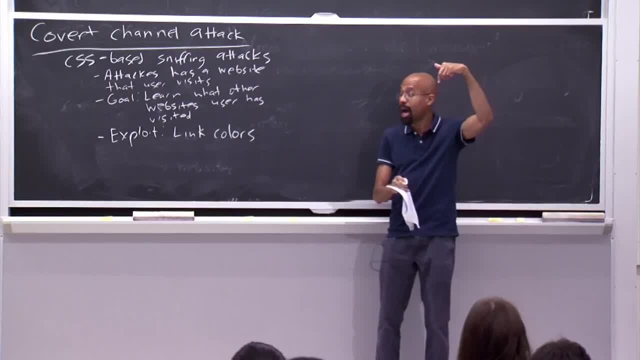 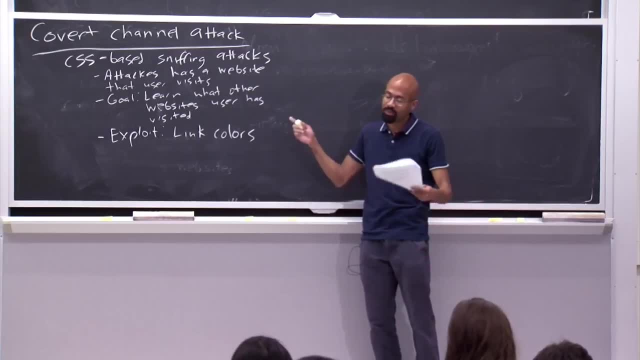 do sort of like a depth-first search on those hits that you found at the top level, So you can actually really constrain the search space this way. So this was really really funny too if you have a demented sense of humor. 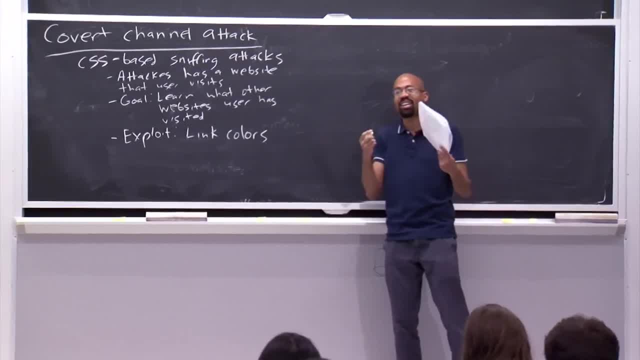 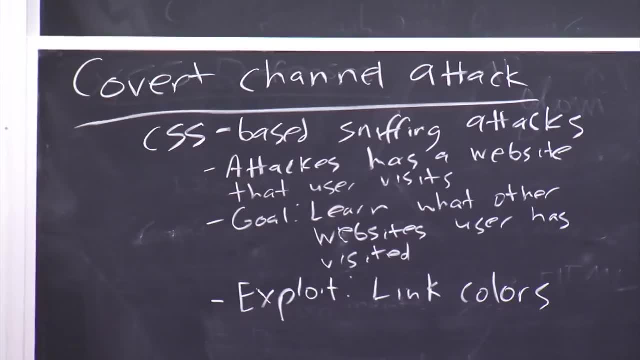 Because it showed that this very innocuous feature that browsers support- they're just trying to help you out, They're trying to say, hey, buddy, here's where you visited- It- can actually reveal this very damaging information here. So what is the solution for this? 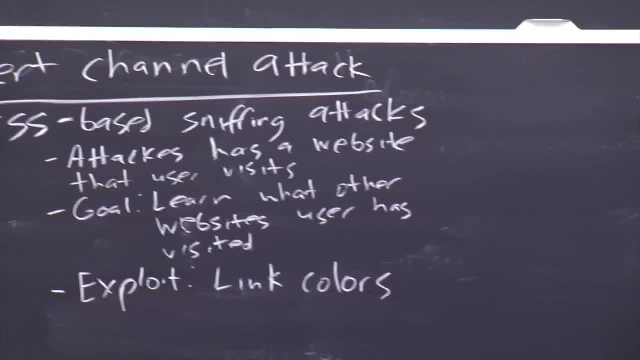 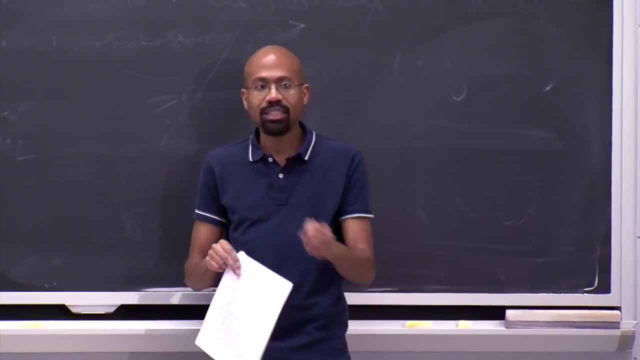 So, in practice, what people did, the browser vendors did, is that they made it such that the browser lies to JavaScript about the color of links. So basically, when JavaScript tries to look at the link and look at its styling, the browser always says unvisited. 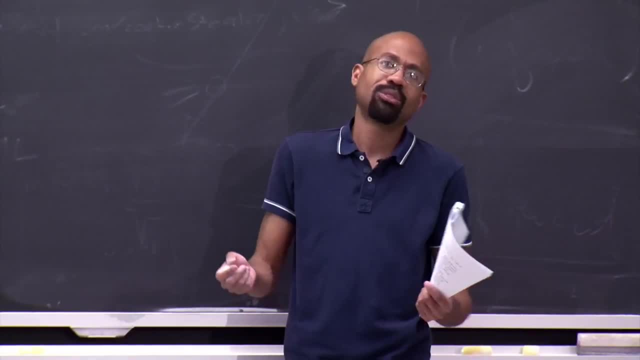 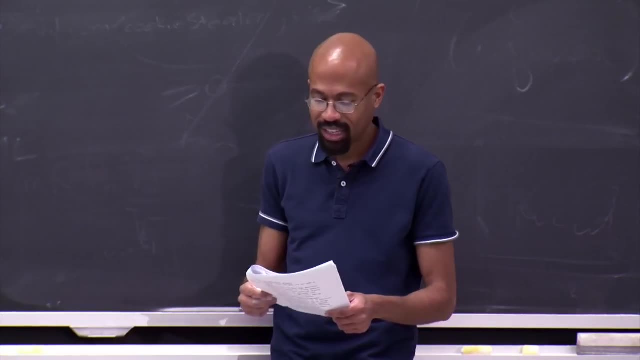 OK. so that seems somewhat unfortunate, but it prevents this attack, so I guess we can live with it. JavaScript not being able to read link colors and not the end of the world. So are we done, though? Does this fix the problem of the attacker? 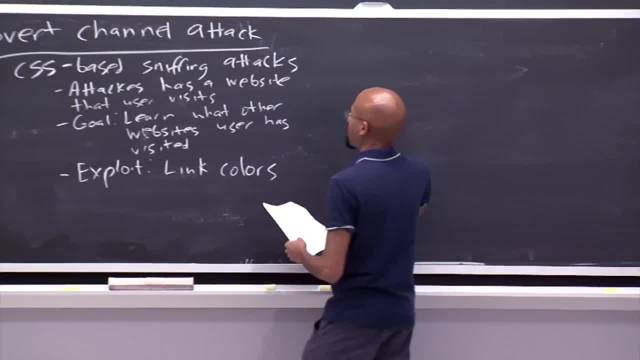 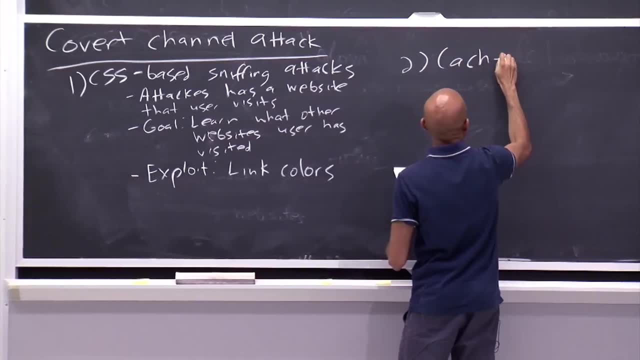 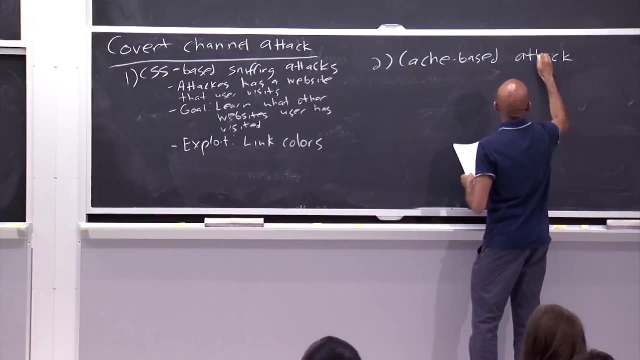 being able to figure out where you've been? The answer, of course, is no, So the next attack that the attacker can do is a cache-based attack, And so the intuition here is that, once again, the goals are the same. The attacker wants to know what sites you visited. The exploit vector is that information that has been cached is quicker to access. That, in fact, is the whole reason why you cached it in the first place. So, once again, the attacker can generate a list. 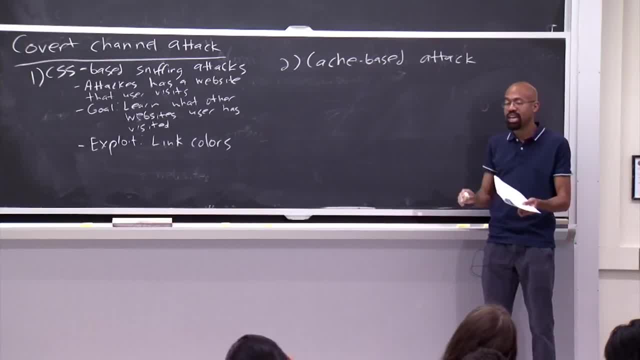 of candidate objects that the attacker thinks you might have visited, and then just time how quickly those objects come back to the attacker. And so if the objects come back quickly beneath some threshold, the attacker can guess that you in fact have been to those objects before. 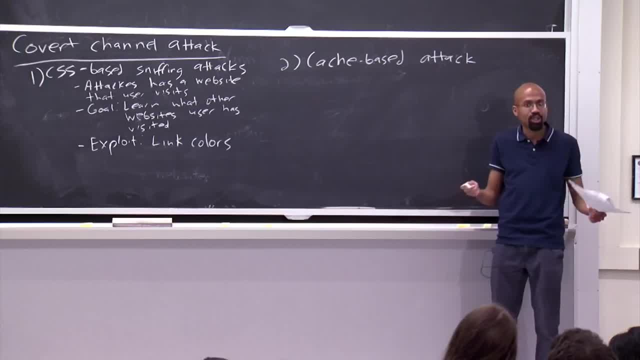 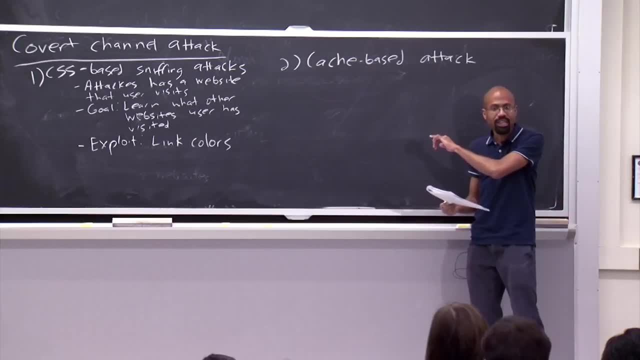 So does that make sense? Well, yeah, Once again, the browser is just trying to help you out, but you can leverage these techniques to figure out some evil knowledge. And what's interesting about this is that this attack can actually leverage some very interesting geographic location information. 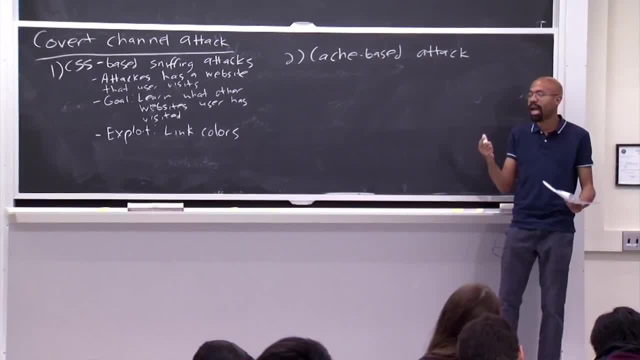 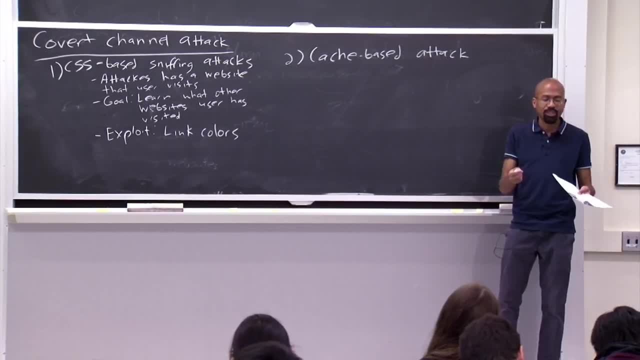 So imagine that we're doing attacks on Google map tiles, for example. So if I detect that you've actually accessed a series of Google map tiles, that probably means you're either in that place or you're interested in other people who might be in that place. 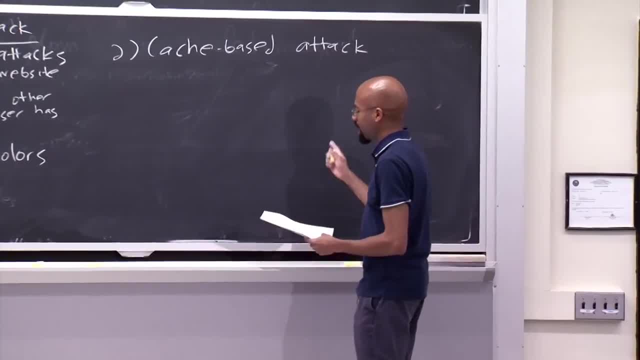 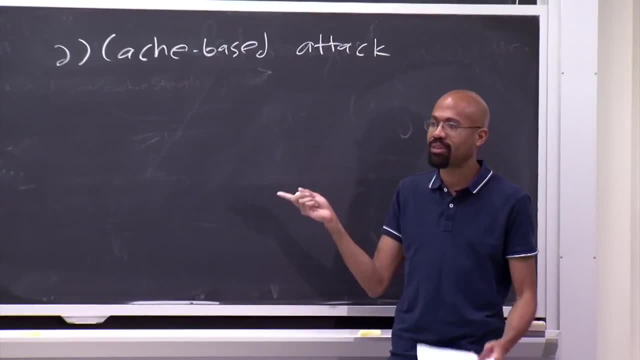 So it's actually a pretty powerful attack. So how can you fix this one? Well, this one is not quite clear. You could have a site that doesn't cache anything at all, but then your site's going to be slow, so that kind of sucks. 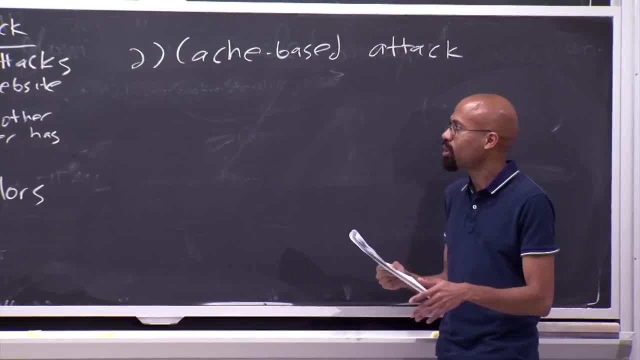 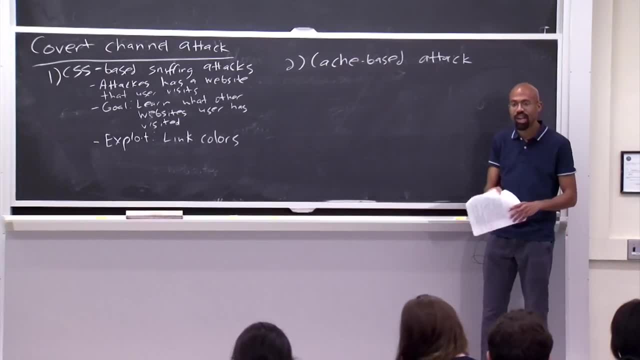 So it's not quite clear how you get around this. But OK, let's suppose that we have the defense we put in place here. JavaScript can't read link colors. Let's assume that the site is super paranoid: It caches nothing, So have we completely defended it? Have we completely defended ourselves against this attack? So the answer is no, because the attacker can actually launch DNS-based attacks. So the intuition is that, even if you don't cache anything, when you access a resource for the first time, you have to generate a DNS request for the hosting. that's. 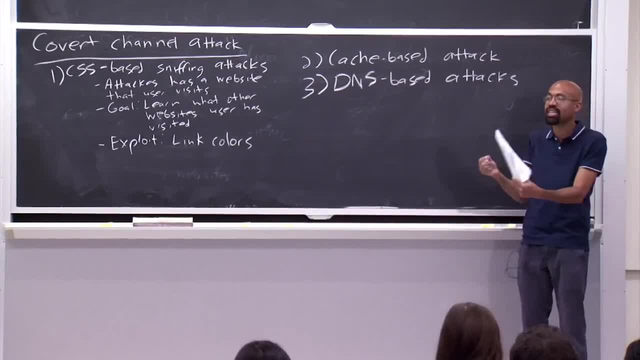 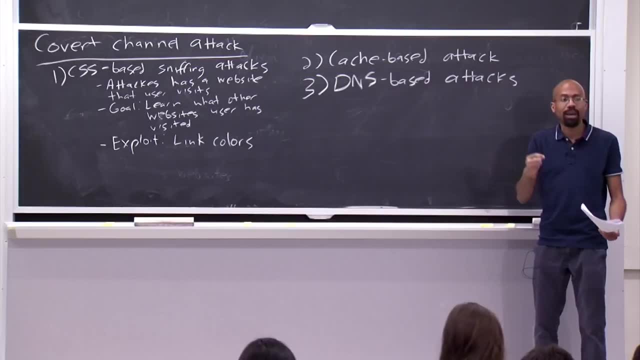 associated with that resource. So once again, the attacker can look in time and see how long it takes for the attacker to access these- a candidate The attacker thinks you may have accessed. If they come back quickly, then that's perhaps a good hint. 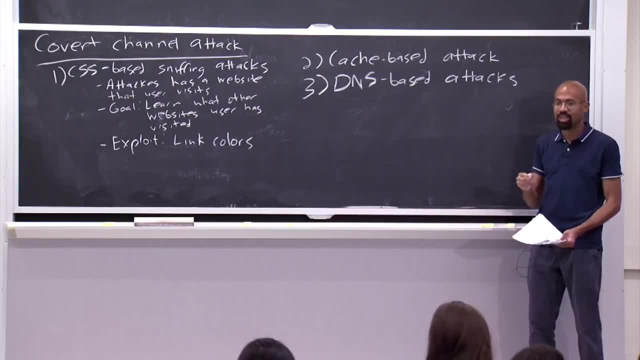 that you've resolved the DNS name for that host before, So this works even if you don't cache anything, because the DNS cache lives with the OS, not with the browser. You mentioned, I think, the ability to get JavaScript to take screenshots. 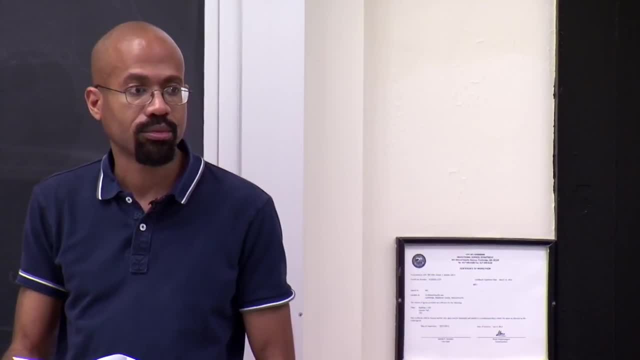 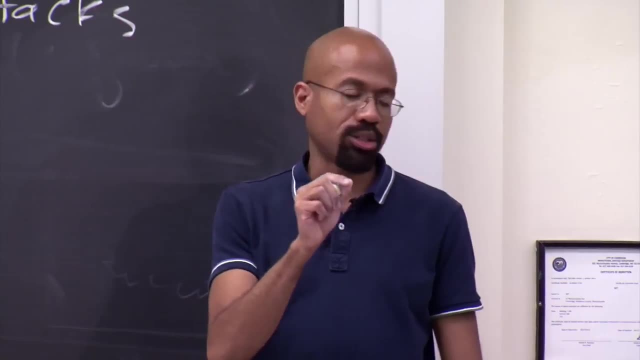 Yeah, I had to. So couldn't you just render the link as a single pixel and then take a screenshot and inspect that? Yeah, well, so you could. So rendering stuff is always a little bit tricky because you have to play these games with. 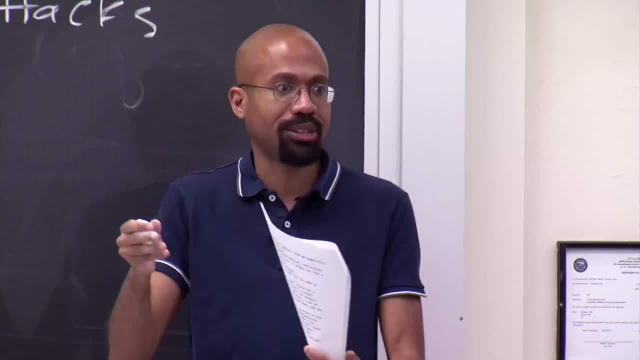 if you want to show something to the user, it has to flash really quickly, or else they might see that someone generated this huge list of URLs. But you're right, If you have access to the screen sharing API, a lot of this becomes a lot simpler. 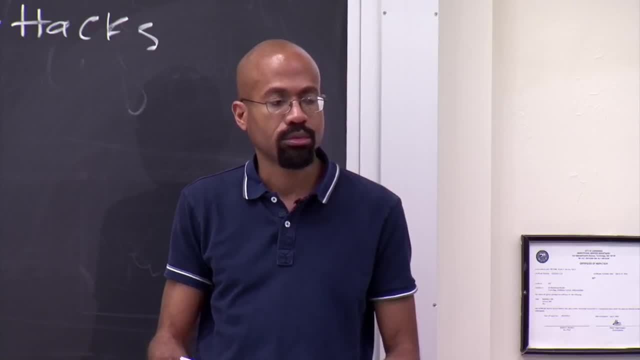 If you just have some kind of animated image that looks mostly random, do you just pay attention to one pixel of it? You're exactly right. I mean, in general, I think the screen sharing API is a bad idea. I'm not the president of the world. 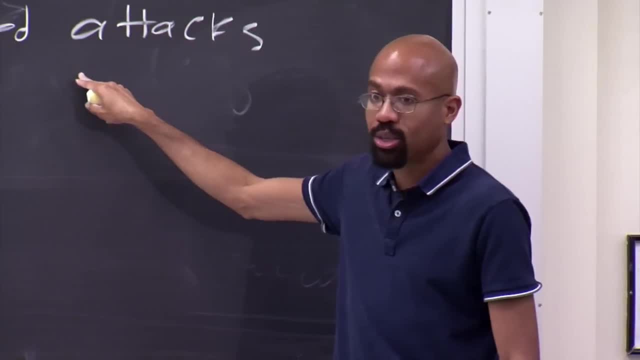 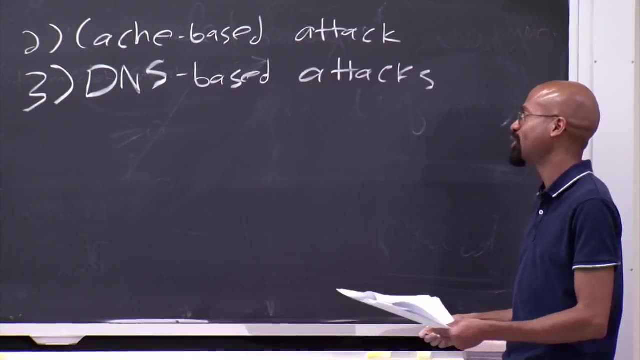 so what can I do? So, yeah, so anyway. so DNS-based attacks work even if there's no caching. that takes place OK. so as the final piece de resistance. so you might think: OK, what if we only use raw IP?